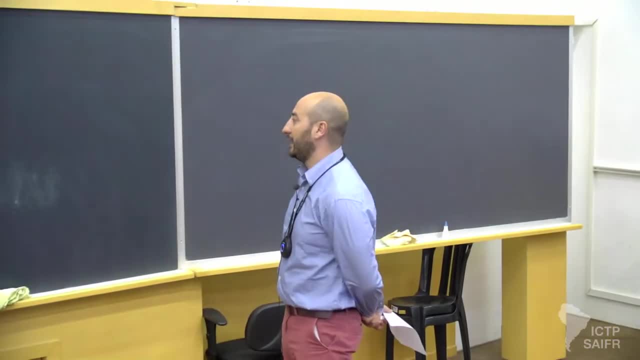 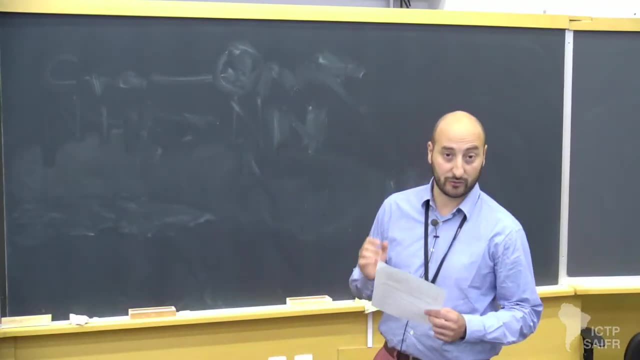 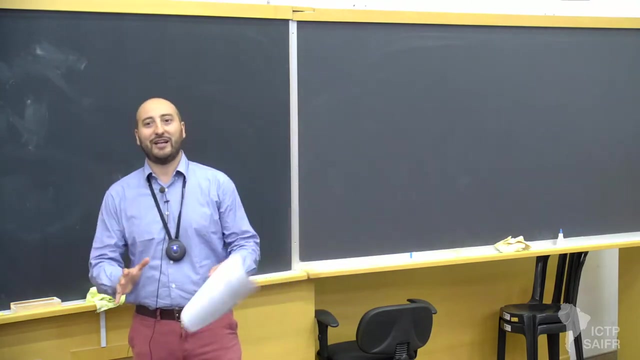 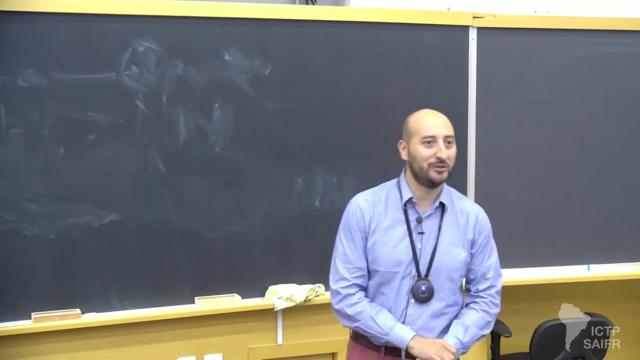 And just an information which will be useful for you. I plan to do everything on Blackboard and I also wrote some notes that will be available daily after the lectures. So don't stress too much. Don't stress too much in taking down the notes. If you miss one line, it won't be dramatic. You will find them back on the notes available, hopefully one hour or two after the lecture. 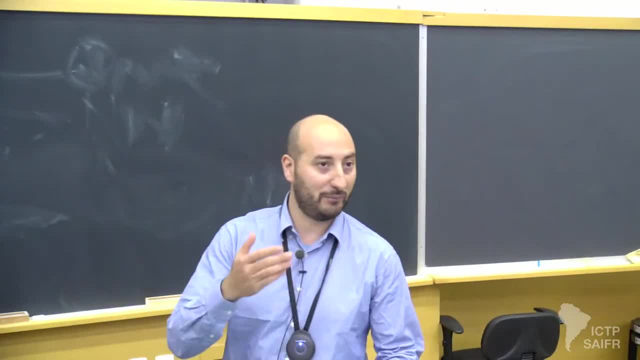 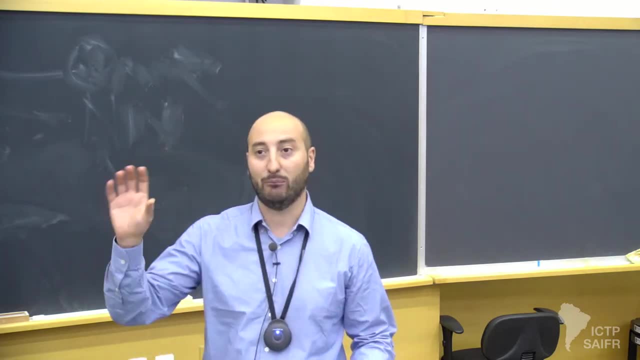 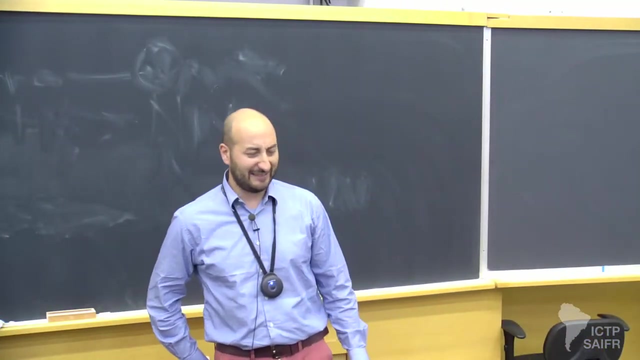 I also prepared some exercises that will be clearly identified as such in the notes, with some boldface blue character. I will briefly introduce them during the class if I have time, And they are not very difficult. At least I think they are not very difficult. 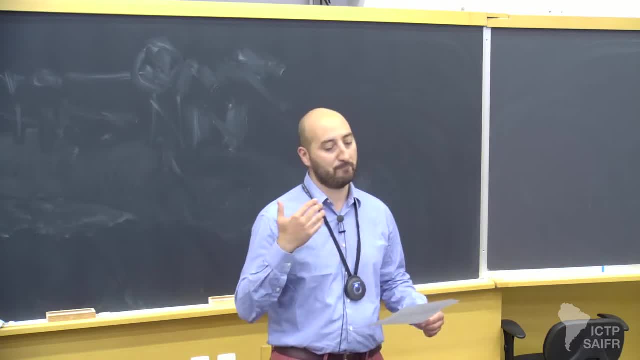 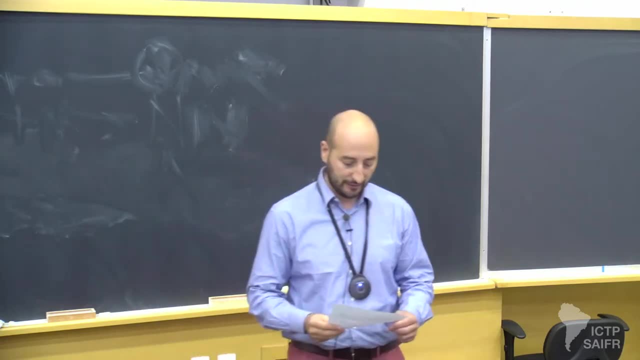 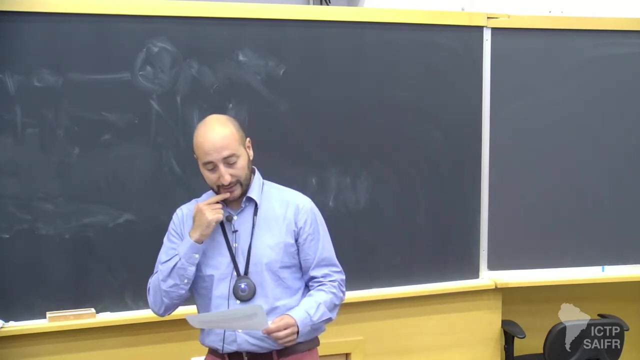 They are more the type of exercise that are useful for you to realise if you have understood what was said or not during the lecture and to familiarise with some concepts which are not necessarily familiar to you. This is the other difficulty I had. 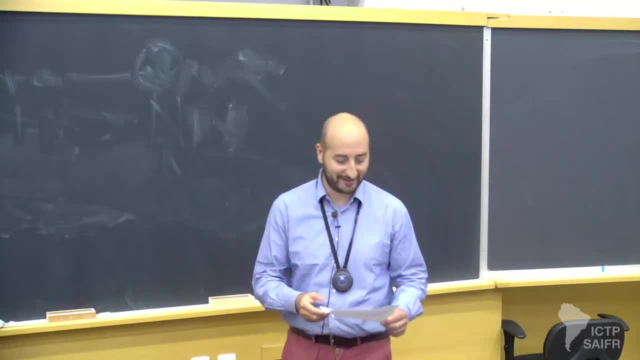 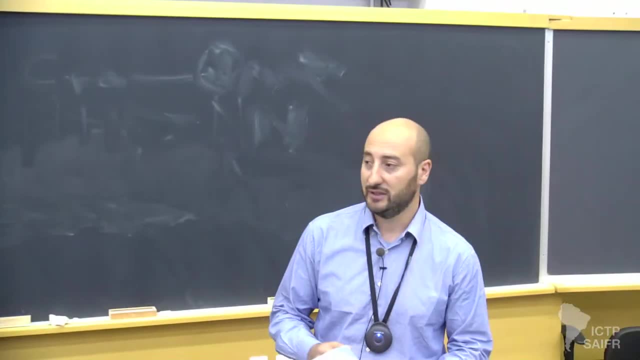 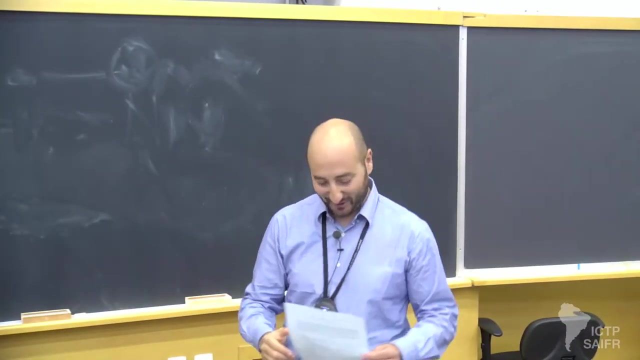 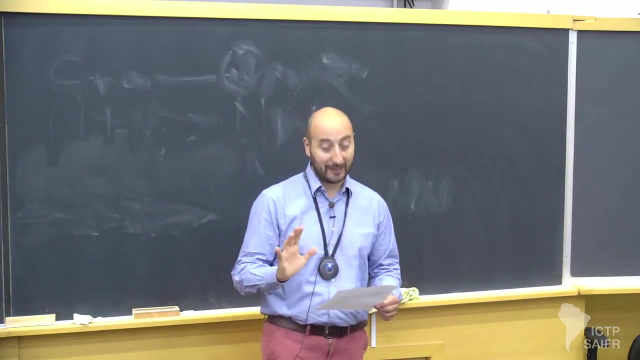 So you come from very different places all over the continent and probably have different backgrounds, So- and I think there is also somebody from outside this continent. Yes, so I'm not sure what you know, what you don't know. This is why the lecture will be probably mixed. 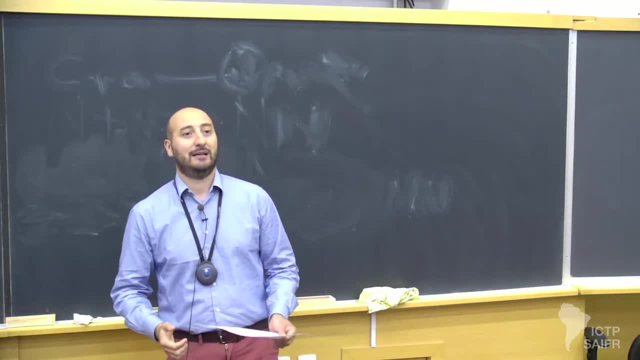 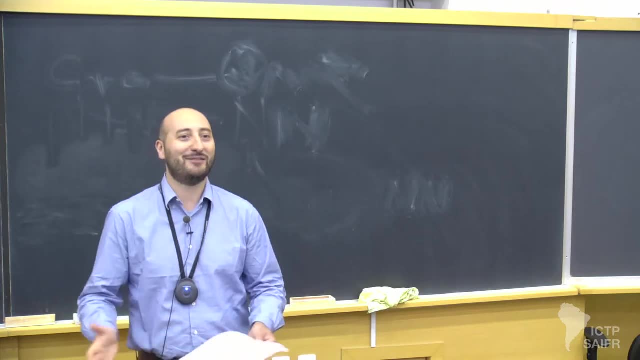 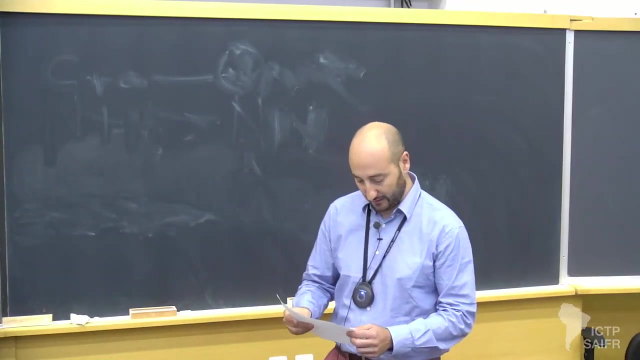 There will be some topics which are elementary and some topics which are maybe too advanced for some of you. I try to go for a compromise and so that everybody can profit a little bit from these lectures, And before starting let me sketch the plan of these lectures. 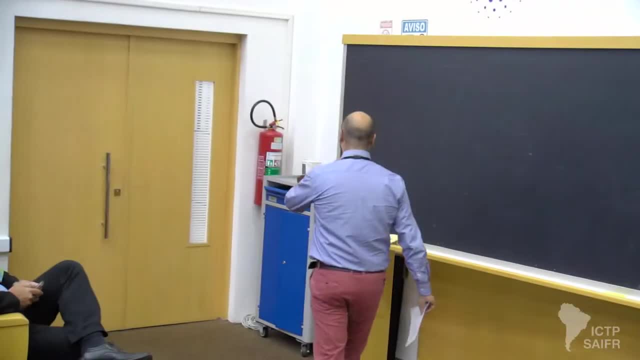 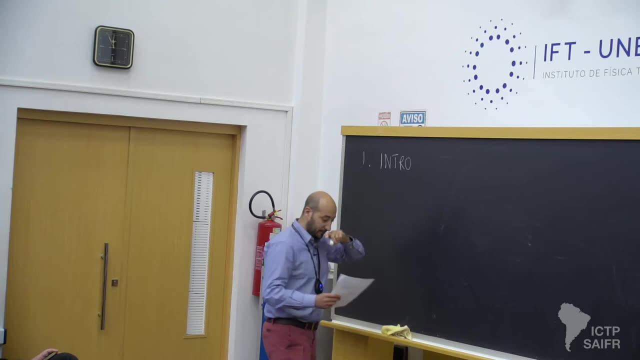 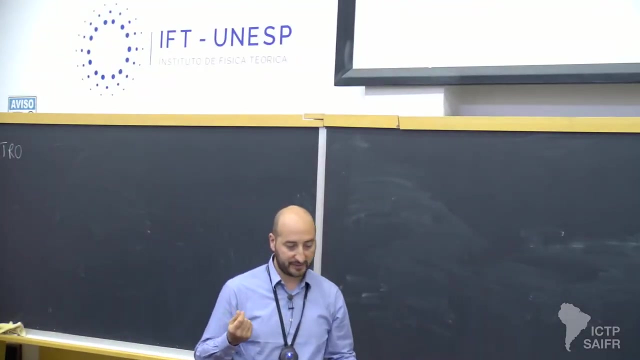 Maybe I start, I put the plan here. I will start today with some introduction. So this introduction is about units convention, that I will use, some generalities on the environments like the galaxy and the extra-galactic system, space, and I will give you a first sketch. 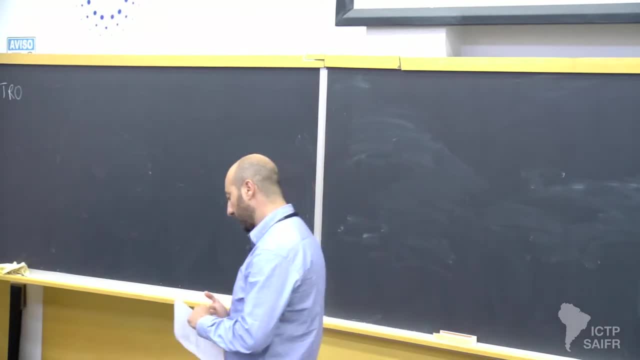 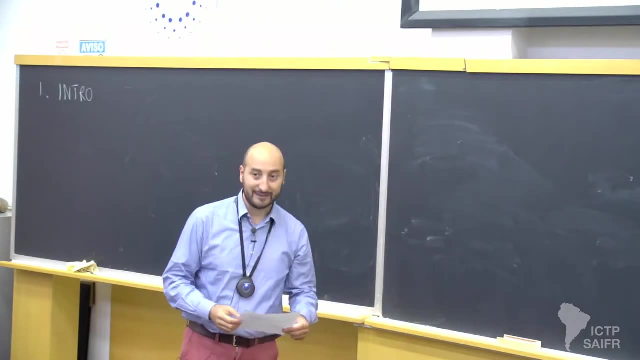 or a model of the kind of diffusive propagation Professor Blasi just mentioned before. This is not a realistic model, but it's probably what some of you have already seen, I don't know- in statistical mechanics or other courses, And then in two. 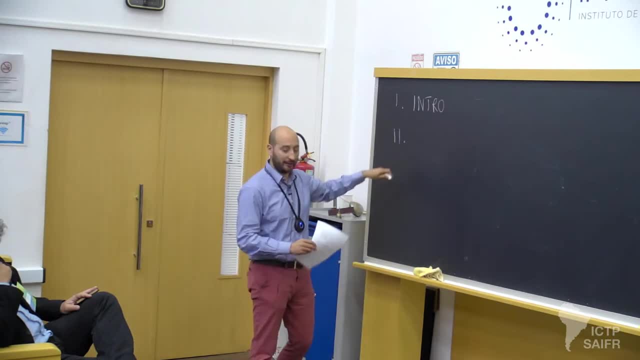 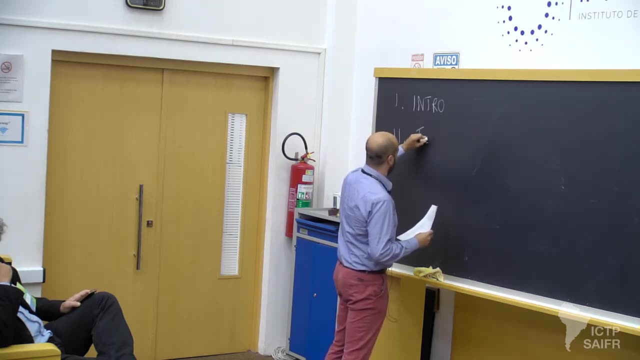 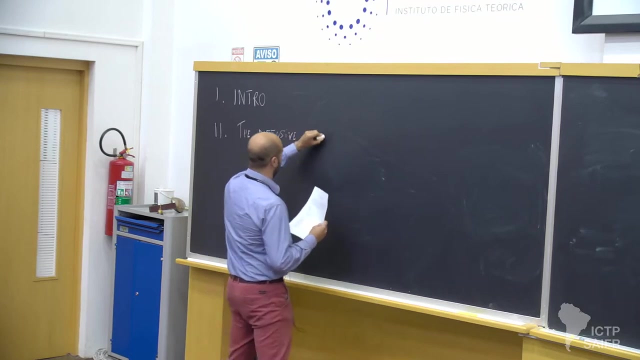 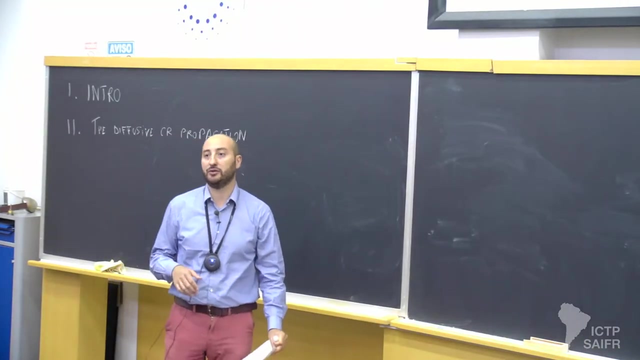 which probably we'll start covering at the end of today's lecture. I will move to the diffusive cosmic ray propagation, Okay, Propagation Again here in this stage I will go gradually. First recall a few reasons, I will give you the notion of the movement. 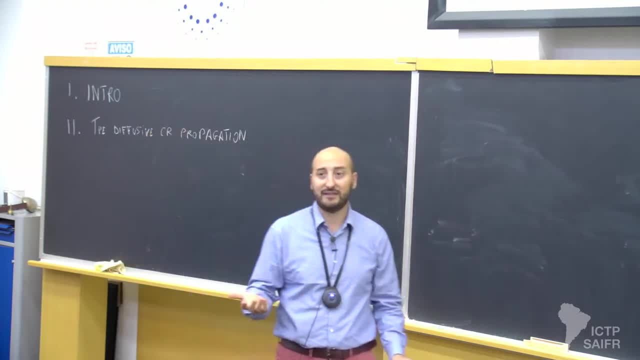 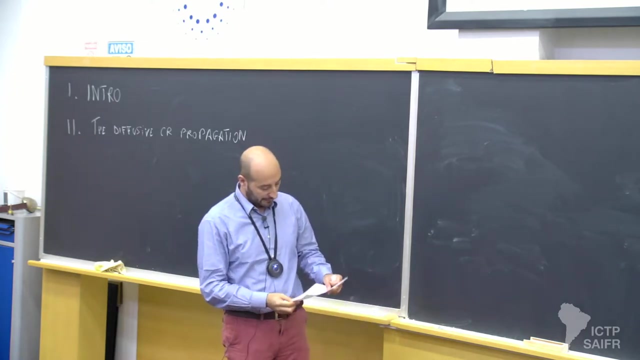 of a particle in a constant field, Then give a heuristic idea why you should expect then, once you add, some turbulence, some fluctuations in this field. charged particle, relativistic charged particles in particular, should move diffusively. Then I will give, I don't know if at the end of today or beginning. 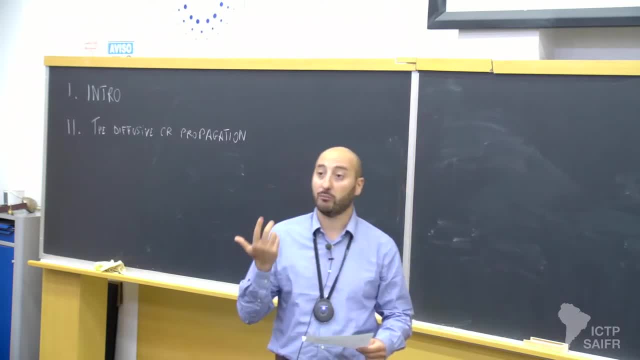 of tomorrow's lecture, a more formal description of that. Even if you cannot follow the details, that would be useful because you know it's something that you will find in books et cetera, So you can make the link to what you find in books. 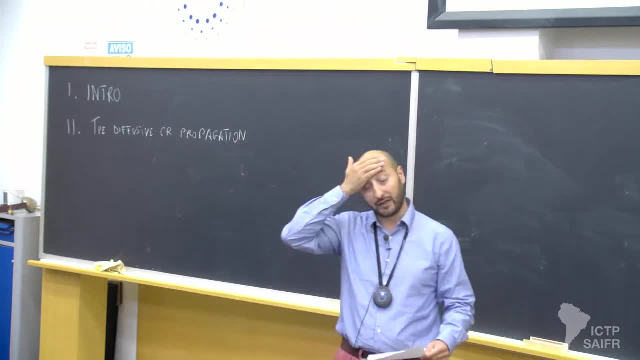 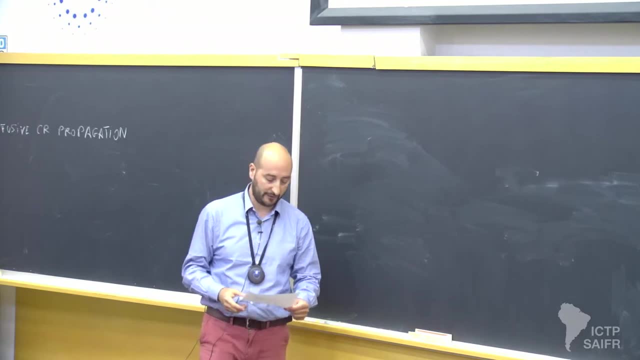 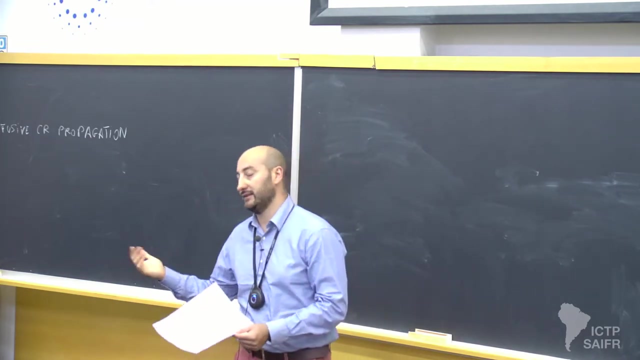 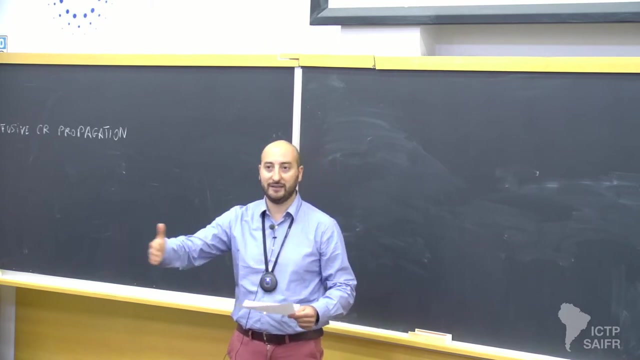 And explain later how this generalizes. when you add the further complication, the fact that scattering centers are moving actually in your frame, And then it's clear that this is not the whole story. as you heard from the previous lecture, Particles do not only evolve in configuration space. 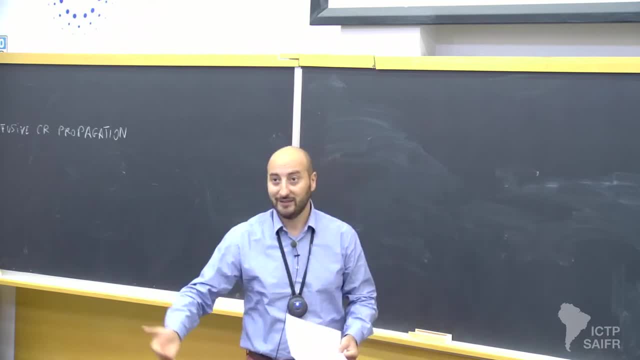 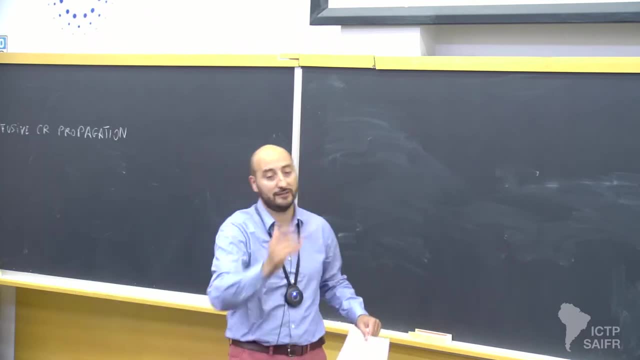 in the three-dimensional space, They also evolve in energy space. Okay, So there are energy loss processes which are very important for both diagnostic purposes and for knowing the energy spectra that were shown in the previous plots and figures. So I will move to the description. 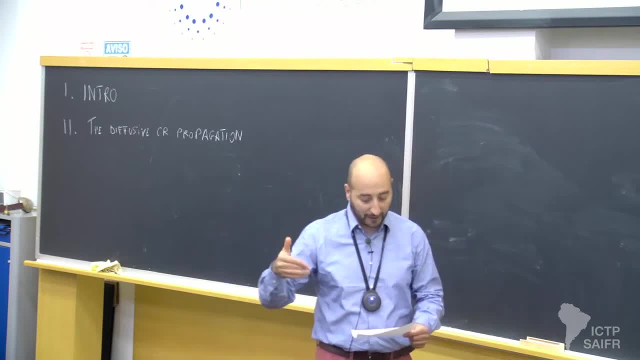 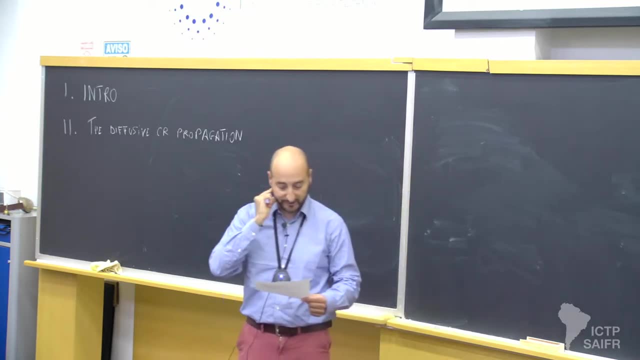 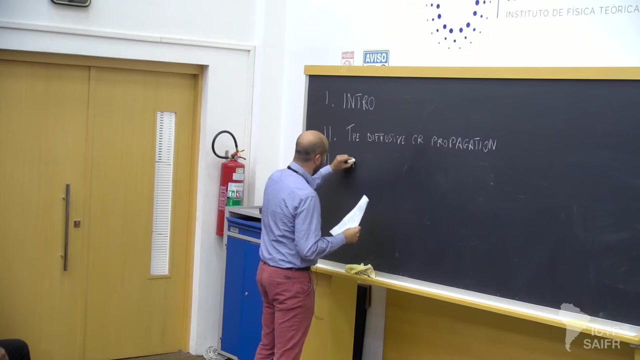 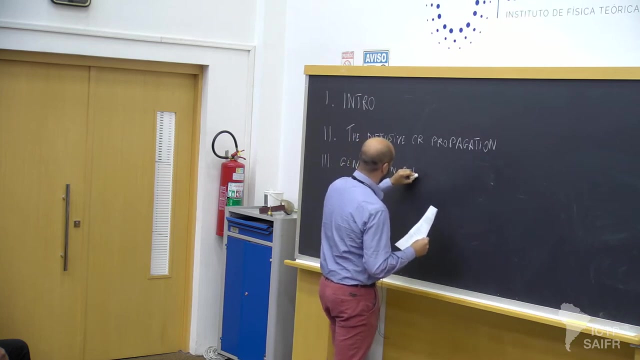 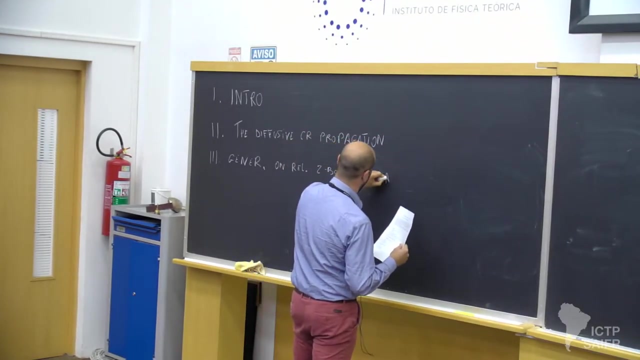 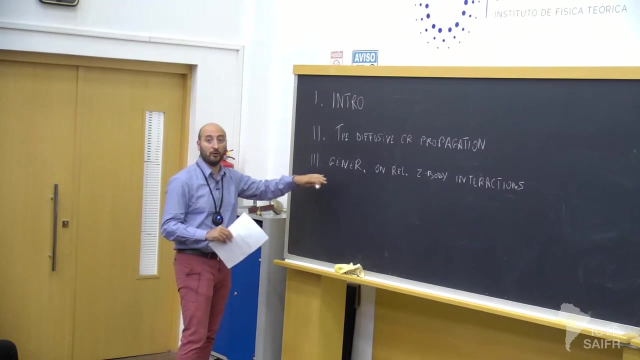 of the two-body particle-particle interactions which are responsible for the main energy loss, The main channels of energy losses. So I will give some generalities on relativistic two-body interactions. Probably most of you, if not all of you, know about that. 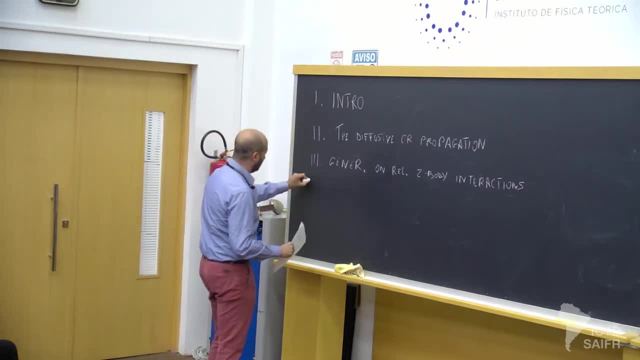 But just to set the stage And then describe a few very important processes. So synchrotron radiation, This was mentioned already today- Inverse Compton- So this is the inverse Compton. So this is the inverse Compton. So this is the inverse Compton. 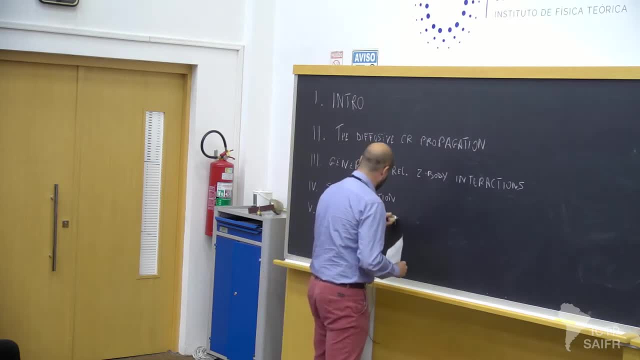 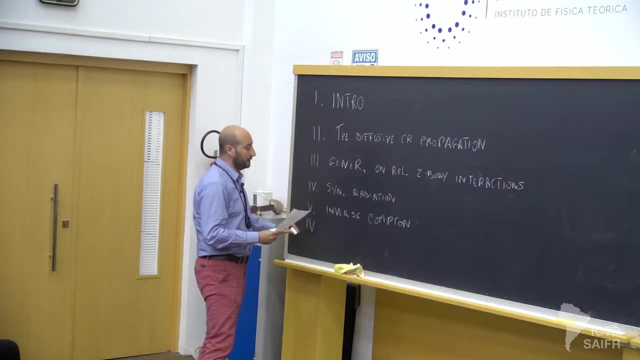 Okay, Then I will cover some liptonic interaction with matter very briefly, Because this is not the main subject of really high energy astrophysics. It's more intermediate energies that will be more of interest, for example for X-ray, X-ray astrophysics. 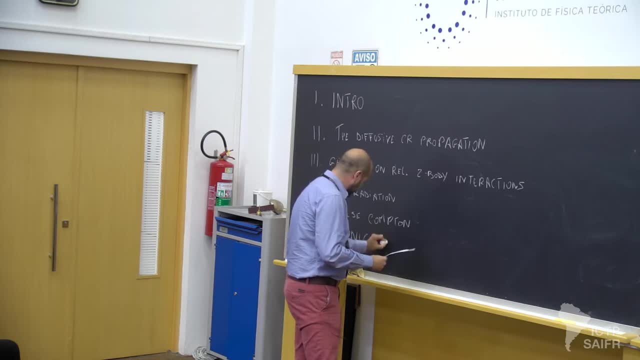 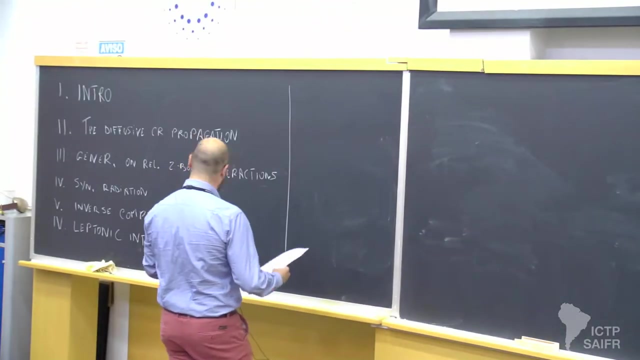 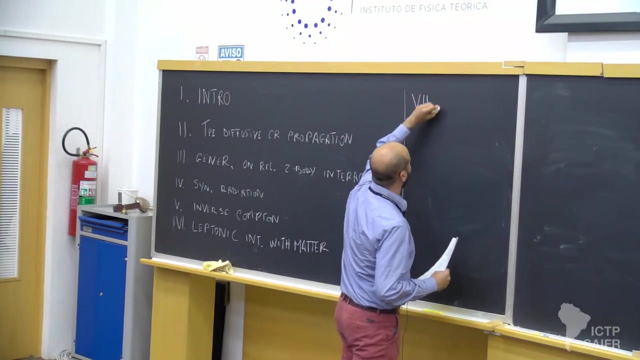 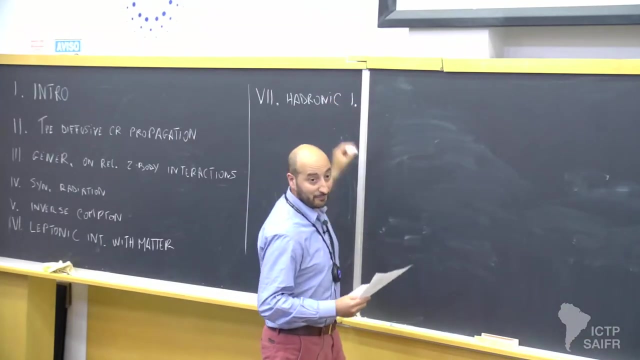 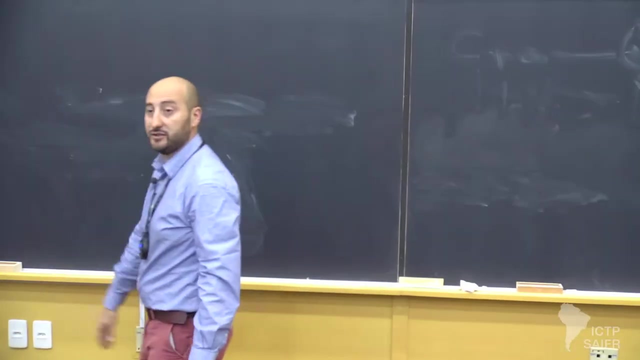 So I will just go briefly with that. Then there is a sorry, what did I do? I put the high on the wrong side. Then adrenic interactions. This is a big chapter because it also includes all the processes you have been that were sketched just before. 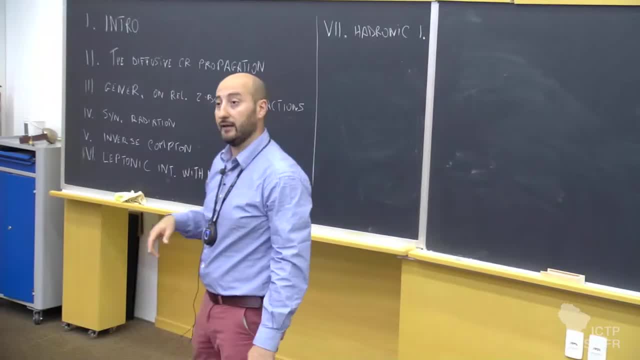 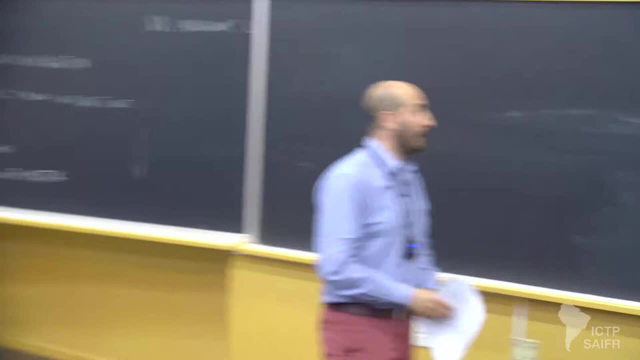 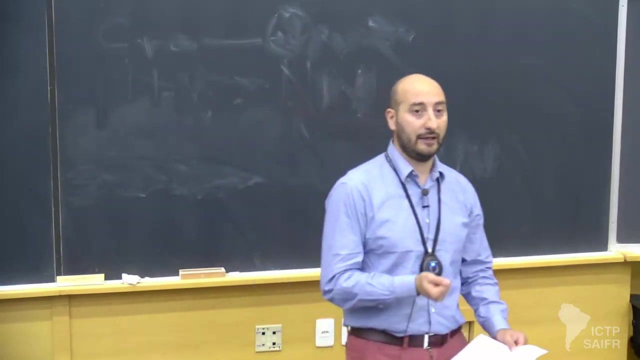 So the processes of energy losses concerning ultra-energy cosmic rays, all these adiabatic beta-Hitler photopion productions and the GZK-related effect, Inelastic proton-proton collisions, And then I will spend some time. 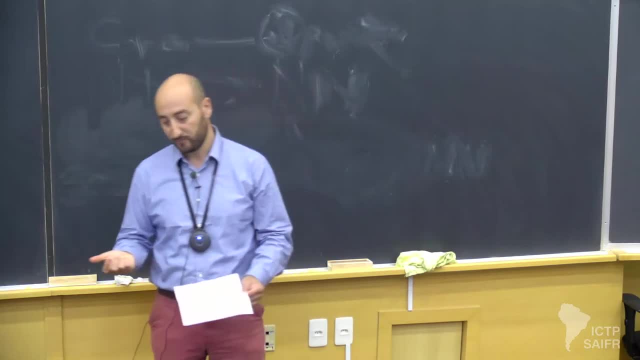 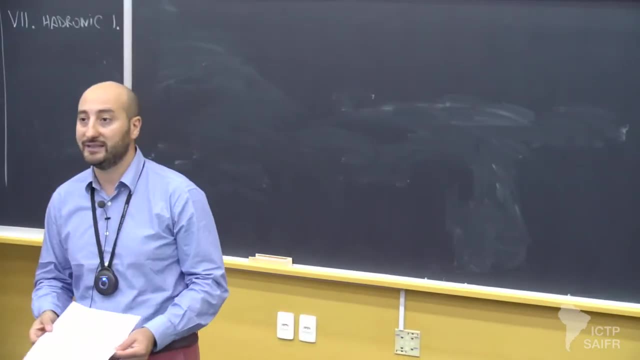 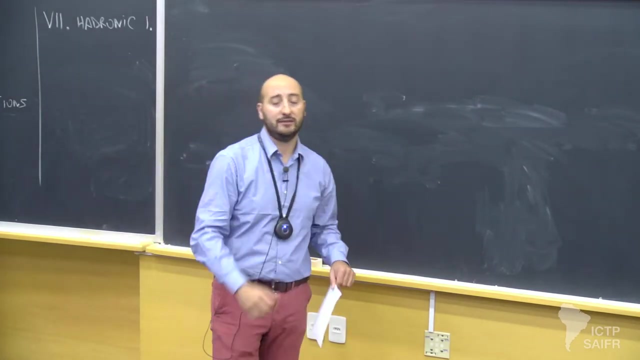 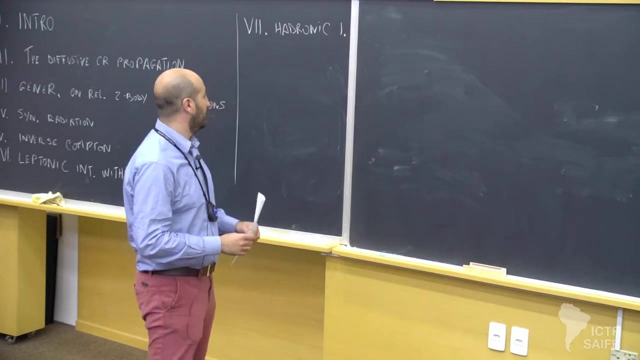 showing you some basic information on the neutrino spectra coming from pion production and the photon spectra coming from pi-zero decay. So basically, this sets the stage for what you would need for other lectures on the neutrino and the high energy gamma ray of adrenic origin. 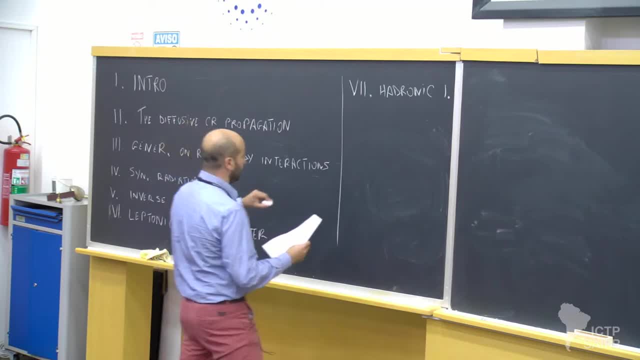 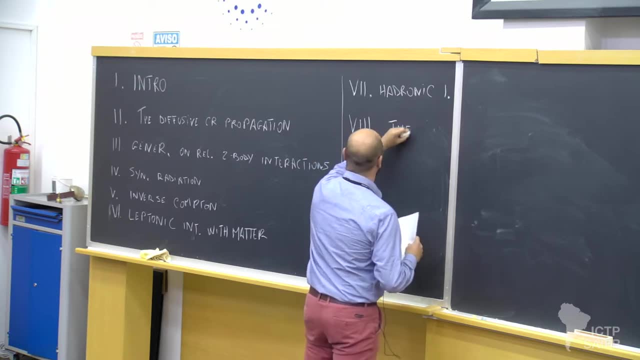 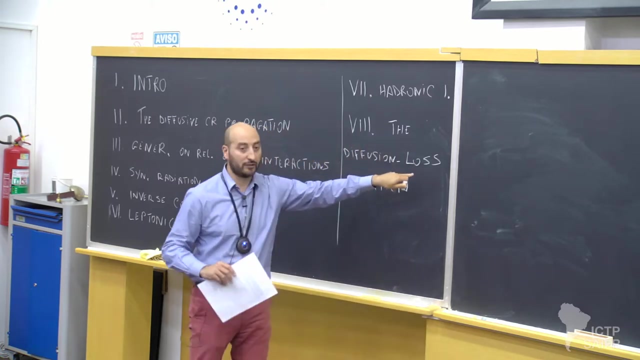 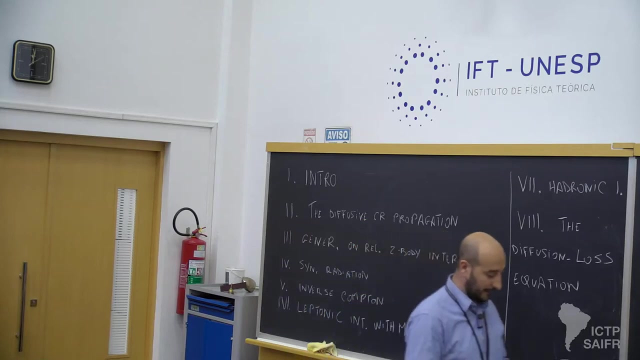 And then we will come back, like in a circle, we will come back. We will come back with the diffusion loss equation, where now we have integrated the loss term on the top of the diffusing term that are treated today and tomorrow And we will see some basic analytical solution to this equation for specific cases, one of 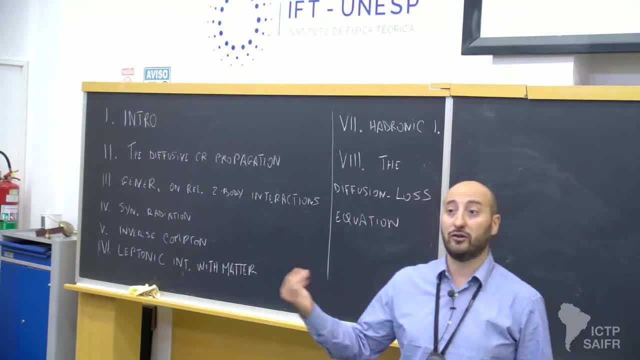 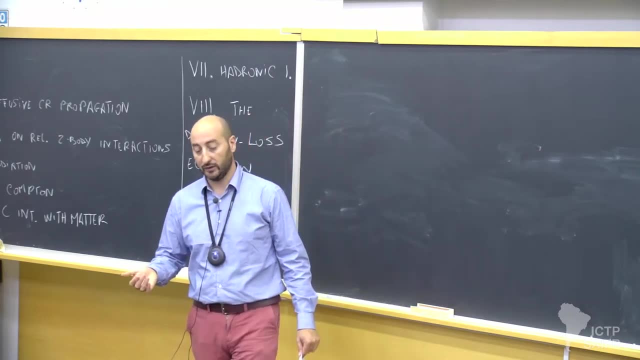 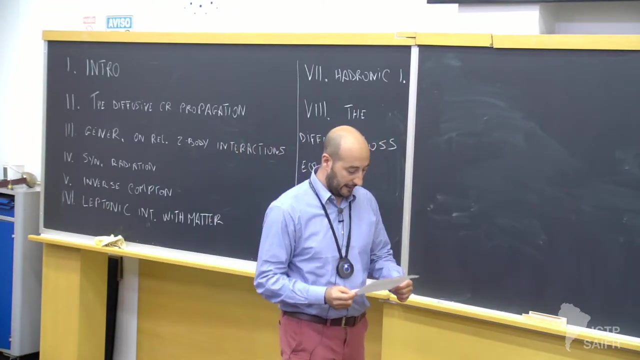 which will be the secondary over primary ratio mentioned before, which is used for the diagnostics on the parameters of diffusive propagation of cosmic rays in the galaxy. I will give you also a simplified model, a proxy for what changes, for instance if 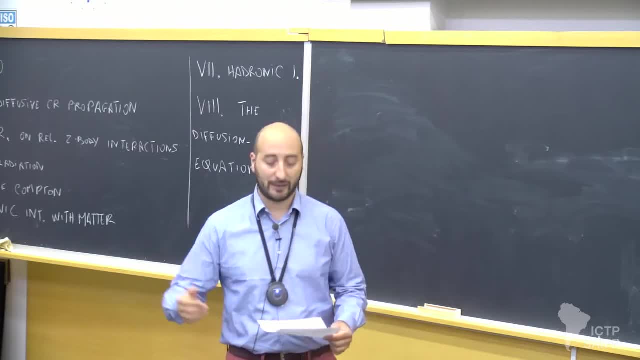 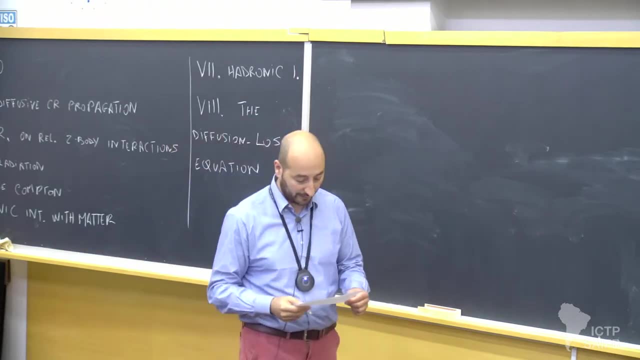 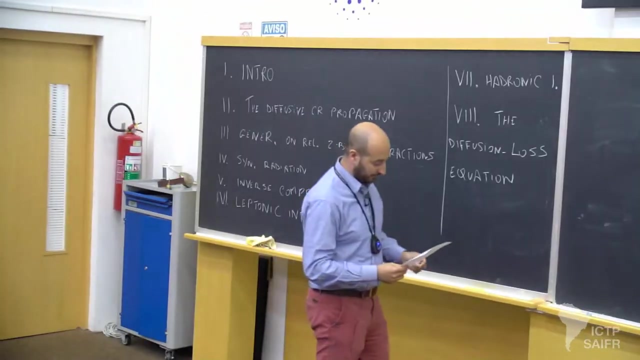 you want to look for For dark matter through antiprotons, although I won't enter into that too much because this will be the topic of some lectures next week. But the idea is that we go back and put together all the pieces of the puzzle, okay, 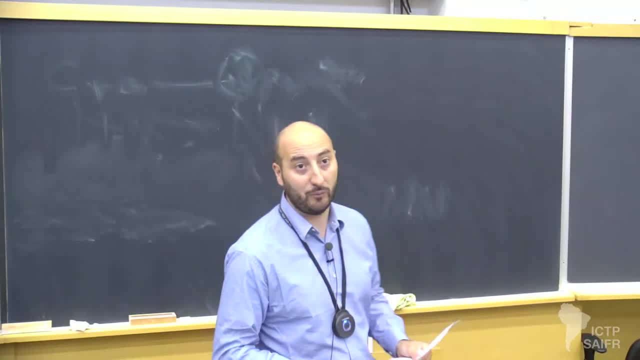 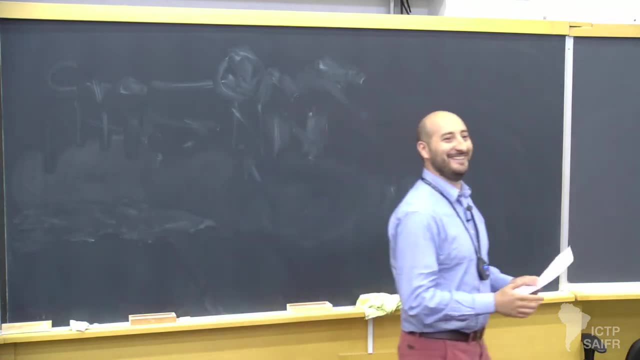 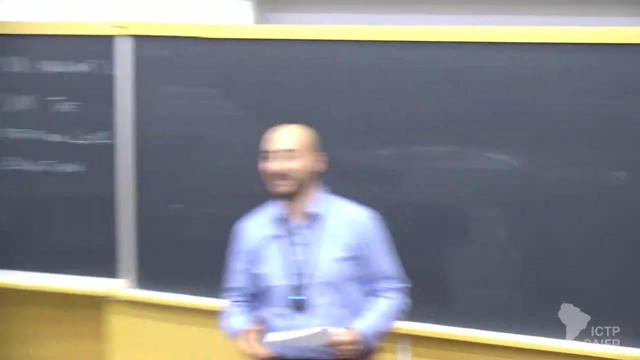 Now something about units. How many of you are familiar with natural units? Have heard about them at least. Okay, More or less everybody, or almost everybody, has heard about them. Maybe not familiar in use In astroparticle physics. it's a strange situation. 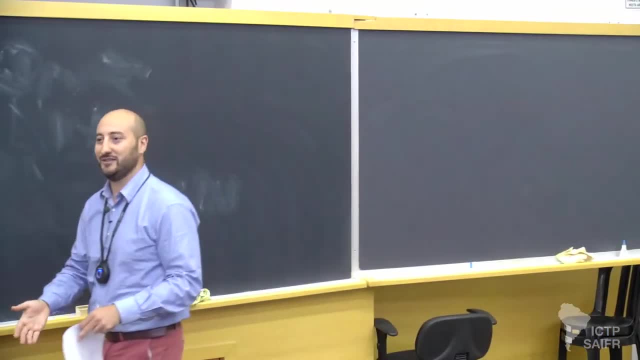 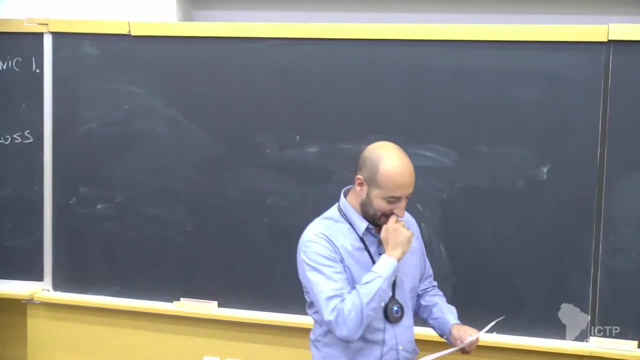 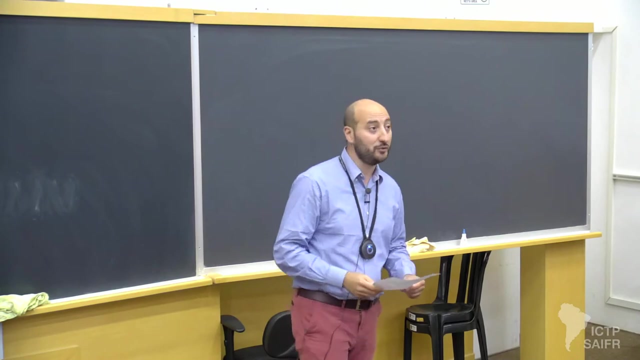 So in astroparticle physics we share some convention with particle physicists and other conventions with astrophysicists. So let's be clear on what we do, because otherwise you are shocked after a few lines of what I write. So we tend to use natural units. 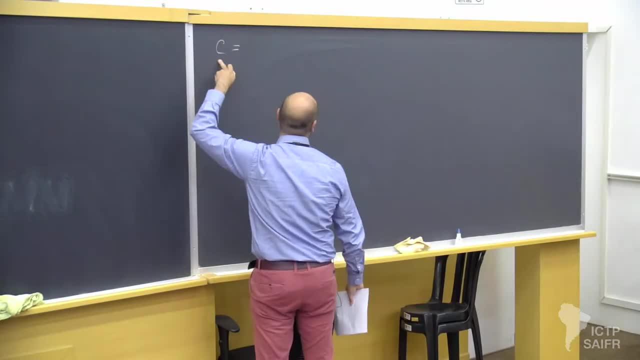 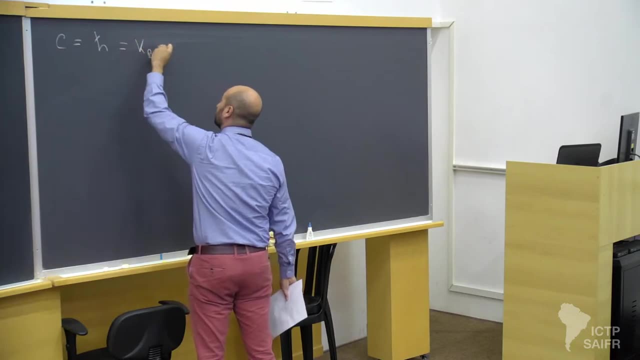 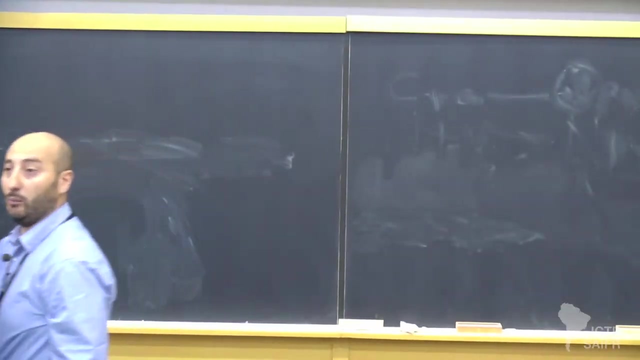 Natural units system basically means that C speed of light, h-bar reduced, Planck constant and the Boltzmann constant, these are set to one. okay, It means that we measure energy, mass, momenta, inverse length, inverse time, temperature. 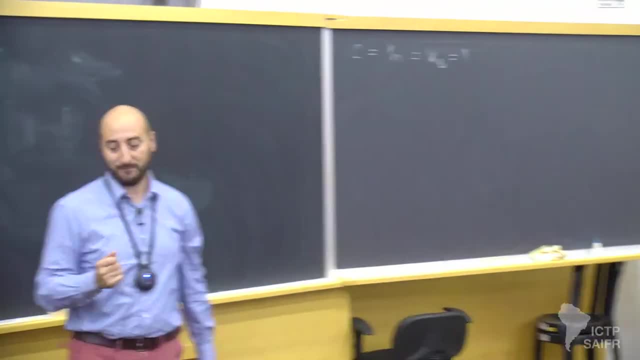 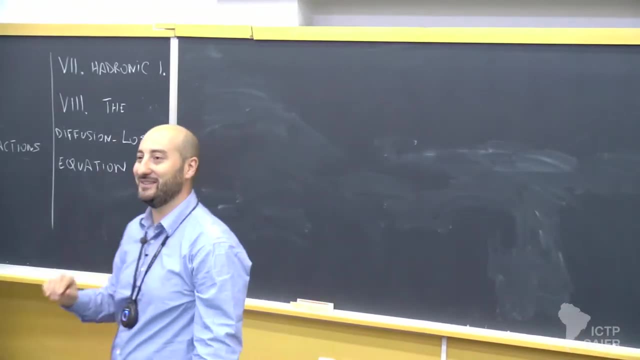 all are energies, okay, The units are energies, Okay. So what kind of units? Typically electron volts, and there is the subtlety: Electron volts and multiples like G, V et cetera, are unit, the units preferred just. 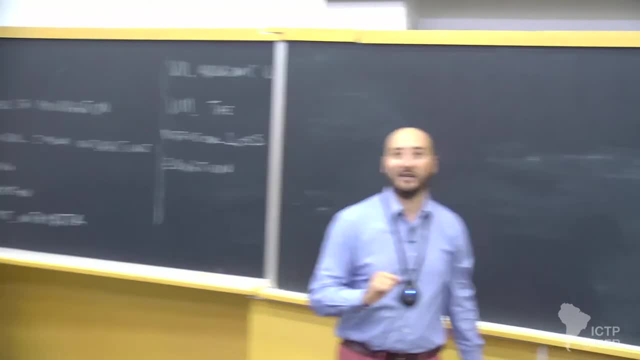 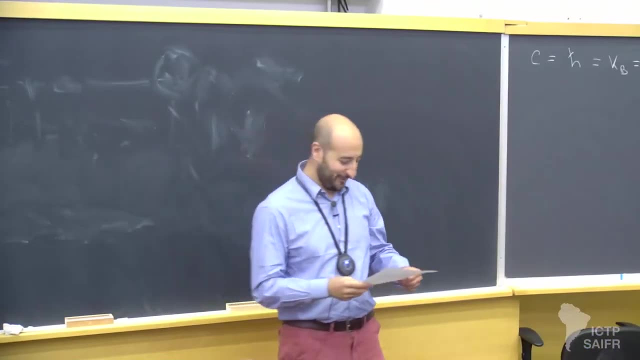 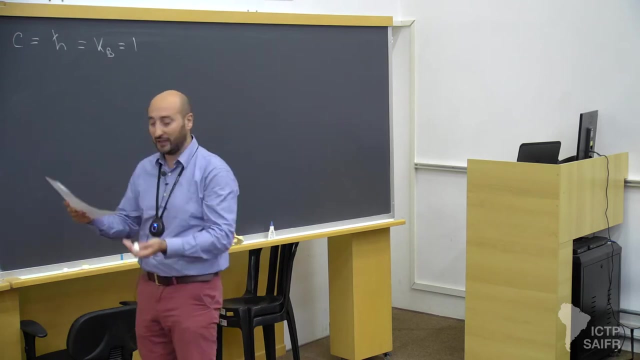 like in particle physics. However, when referring to astrophysical objects, macroscopic scales, the typical unit becomes the Herc. okay, So in order for you not to be too much confused, I wrote down a little table, for quick reference, of these correspondences. 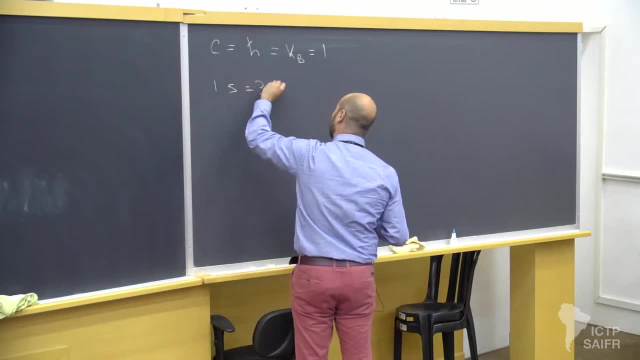 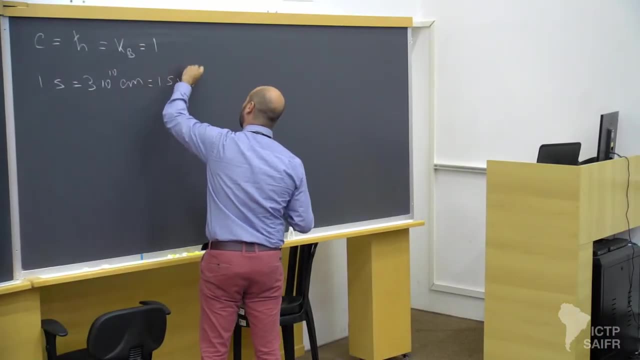 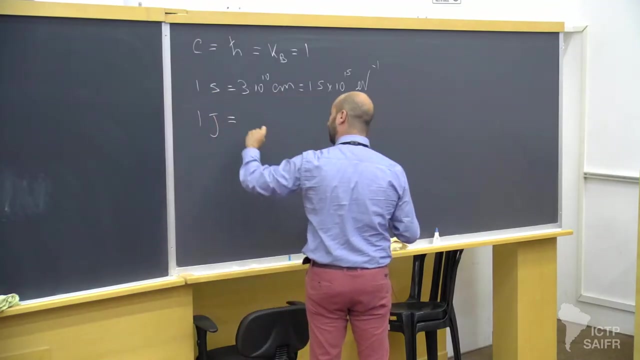 So one second is three times 10 to the 10 centimeters And this is 1.5 times 10 to 15 electron volts to the minus one. One joule is 10 to the 7 hertz And this is 6.25.. 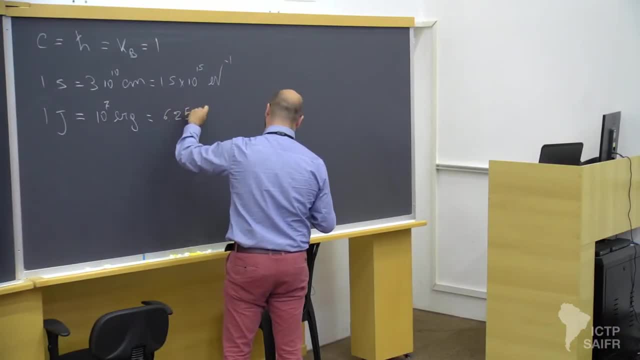 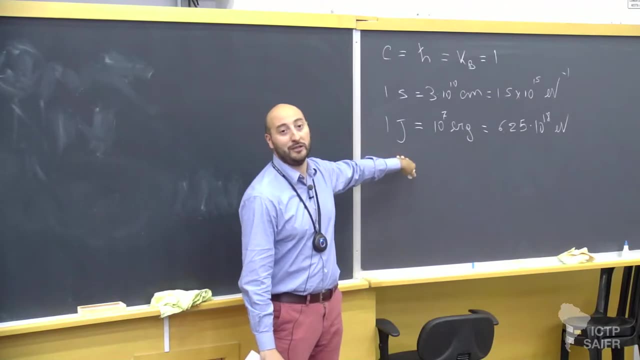 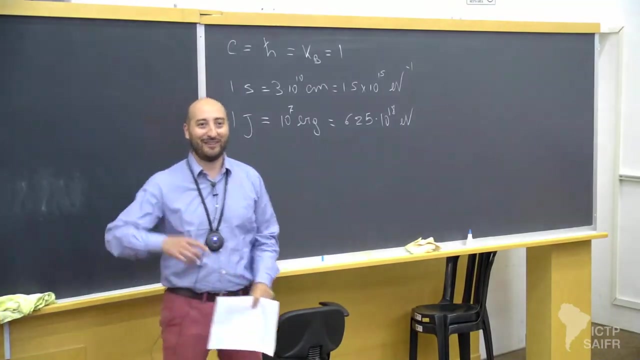 Okay, Okay, So this is 6.25 times 10 to the 18 electron volt. By the way, for your curiosity, a macroscopic unit that you find in basic physics is roughly the energy of an ultra-energy cosmic ray. So you can think of the ultra-energy cosmic rays close to this GZK cutoff as bringing. 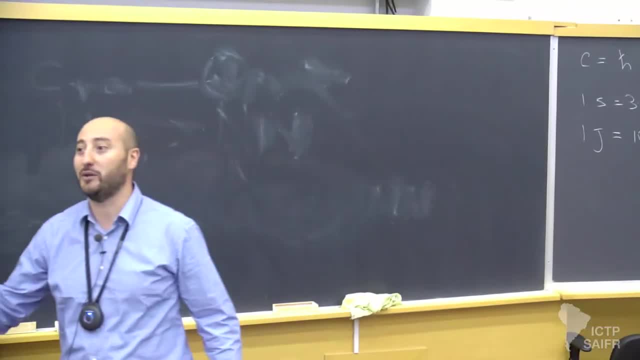 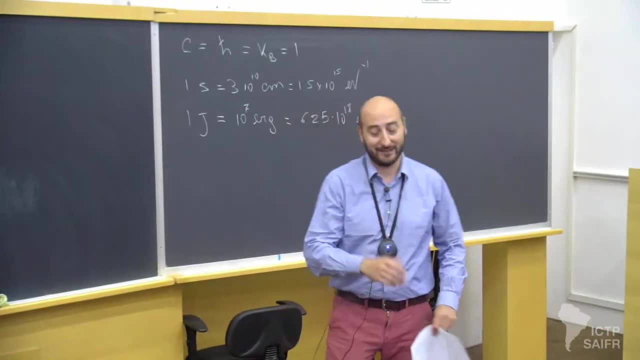 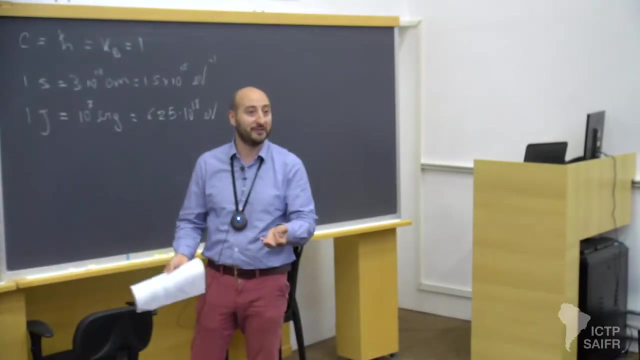 in one particle typical energy of a macroscopic object which contains all other Avogadro particles. It's amazing, Okay, Okay, The other units of distance that we use very often, for obvious reason, is the parsec. I hope you know what a parsec is. 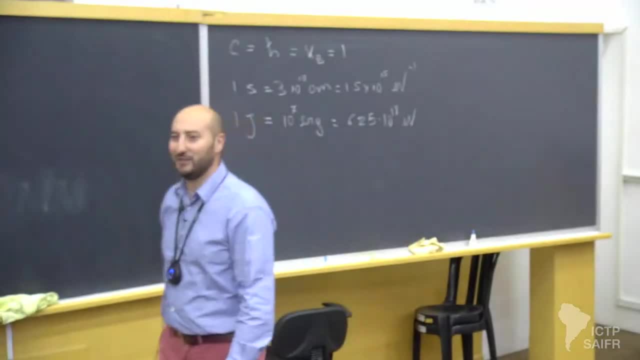 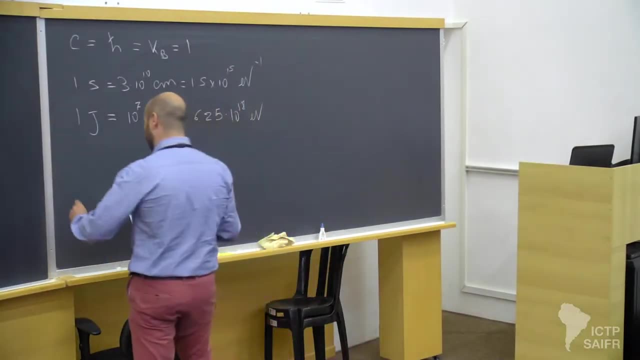 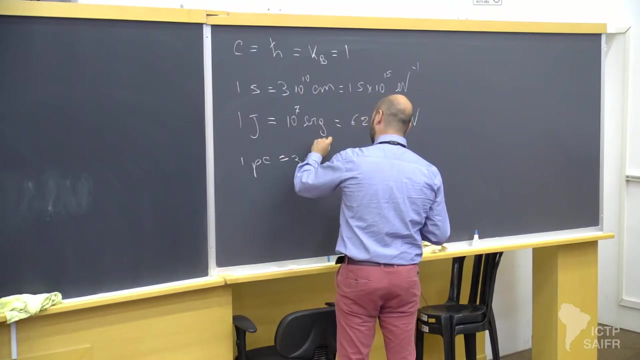 One operational definition is 3.24,, if I'm not wrong, light years, But this is clearly an astrometric-related notion. But one parsec is 3 times 10 to the 10 centimeters. Okay, So this is 10 to the 18 centimeters. 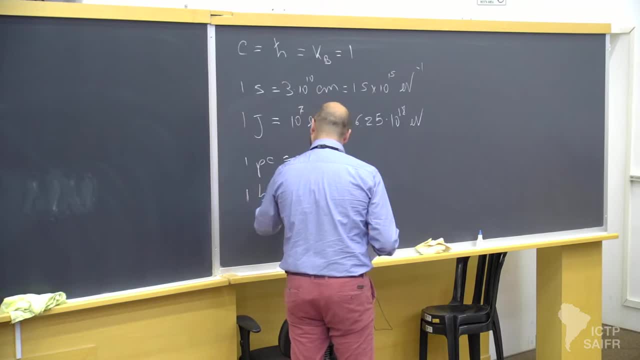 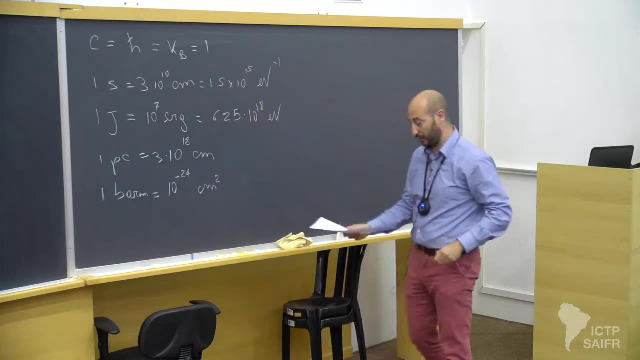 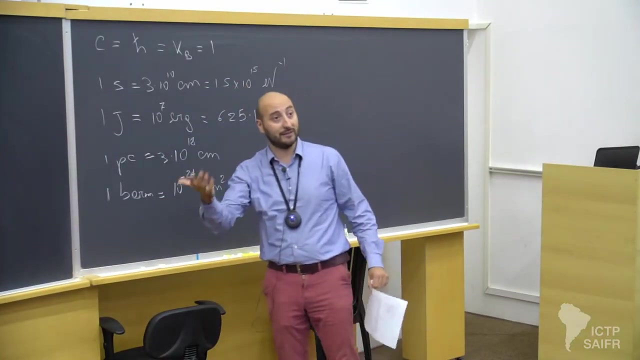 And another unit that we use is the barn for cross-section, which is 10 to the minus 24 centimeters square. This is shared with particle physics, of course, And then for magnetic fields, the Gauss is the typical unit used for astrophysical purposes. 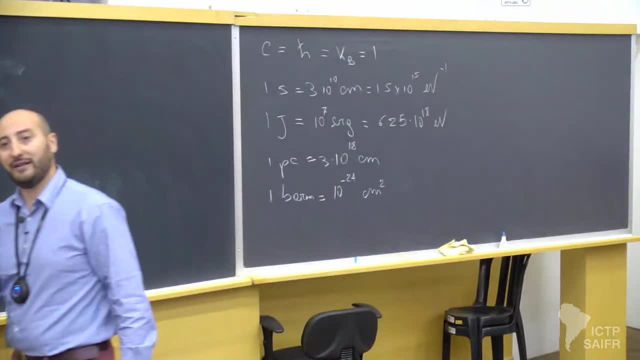 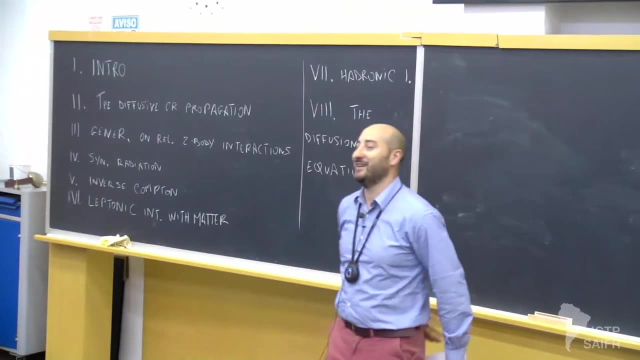 By the way, do you have any idea What's the typical unit? Do you know What's the typical field strength of the magnetic field of the Earth If you take a compass? what's the kind of magnetic field strength that is underlying? 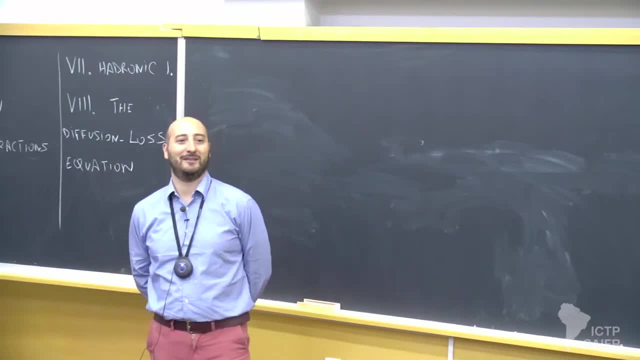 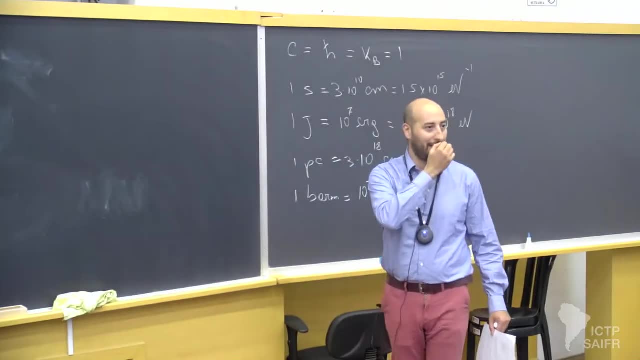 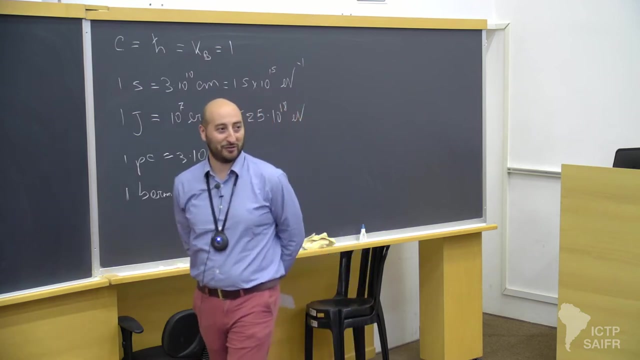 this phenomenon? Have you ever Sorry? Yeah, something like that. So the right scale is a fraction of 500? What did you say Micron? No, it's much bigger than that. It's 500 milliGauss maybe. 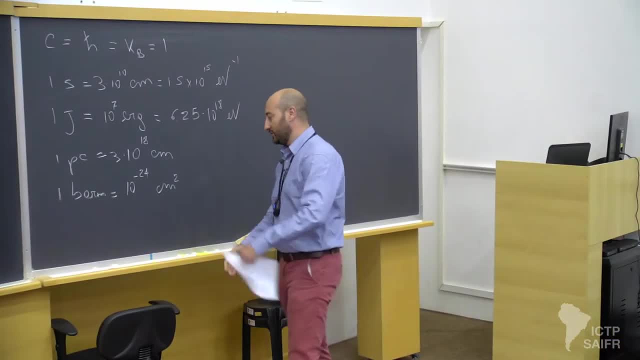 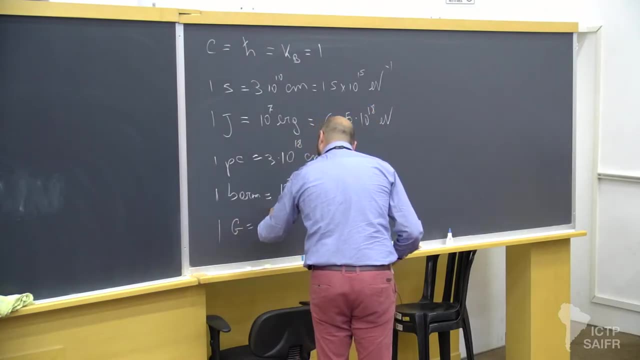 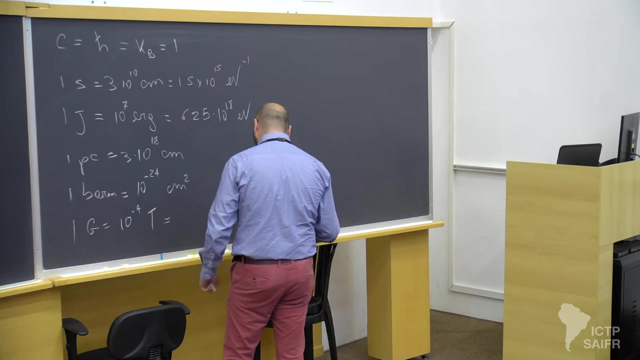 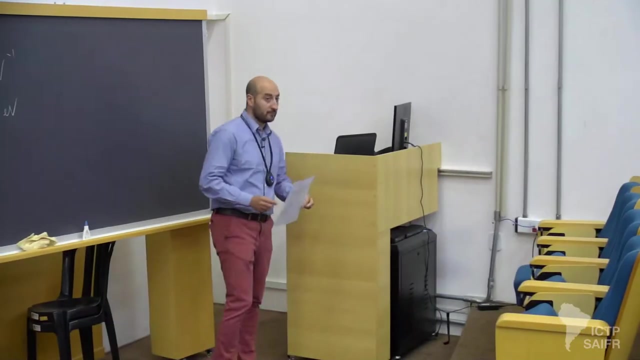 So it's roughly a Gauss, the right scale okay. So, and the Gauss okay is 10 to the minus 4 Tesla, which is the international system unit for the field, And this is roughly 0.07 electron volt square okay. 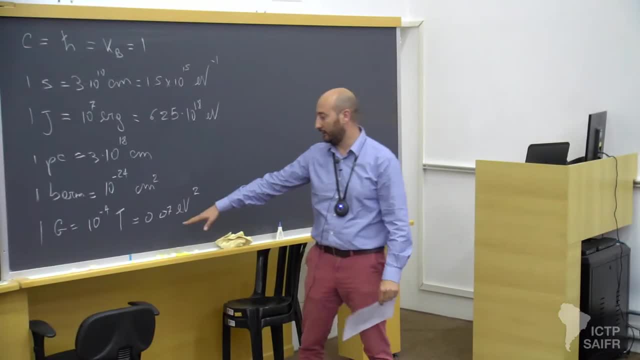 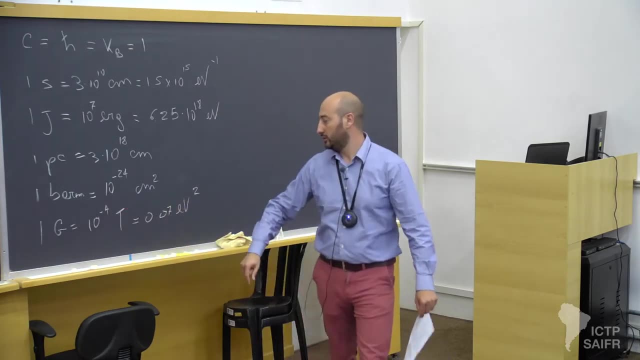 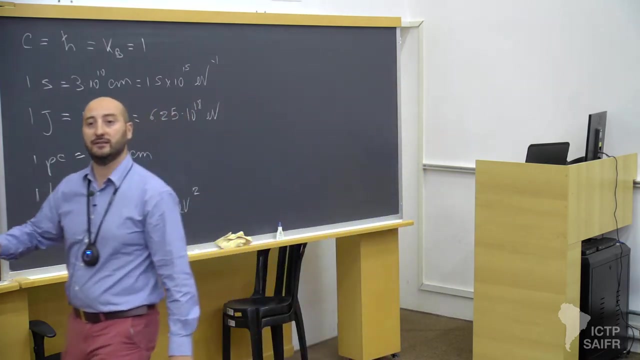 Why it's electron volt square. One simple reason Why- Because you can get this- is that a magnetic field square is an energy density. okay, So the square of this is electron volt to the fourth power and the electron volt to the fourth power is an energy density, because an energy density is an electron volt over. 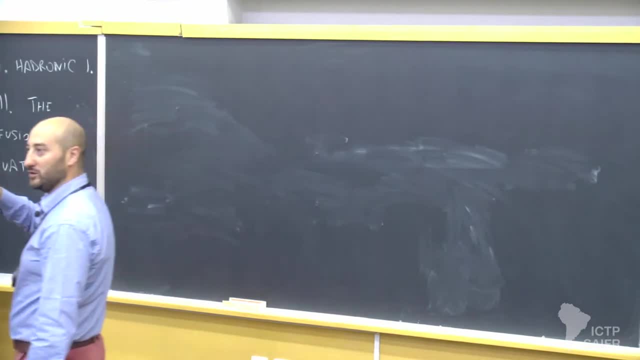 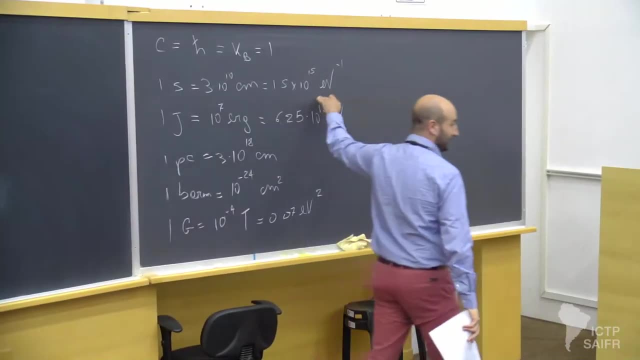 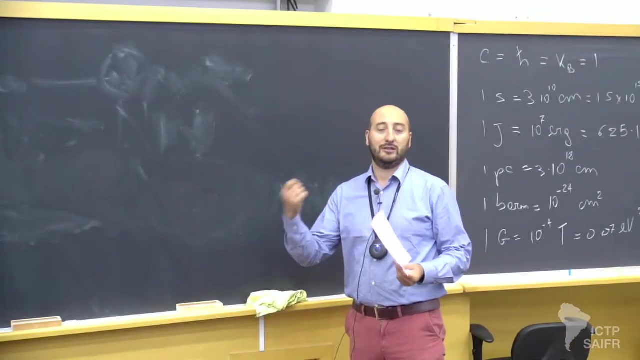 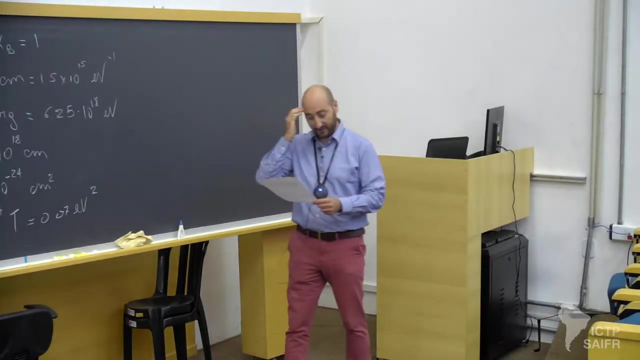 volume. but the volume is length to the minus third power, and the length to the minus third power from here is electron volt cube. Okay, This is just a practical use to go quickly into some numerical conversions. So first things this afternoon, when you have some time, is to do some exercises to if 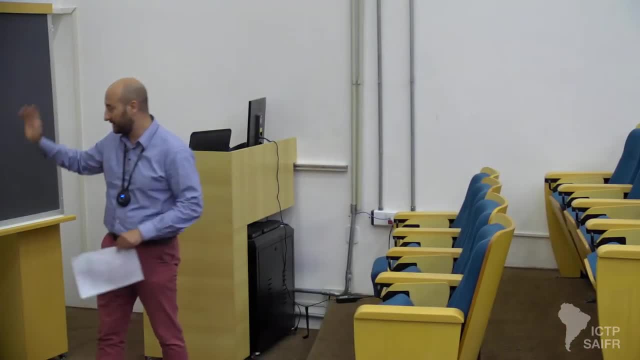 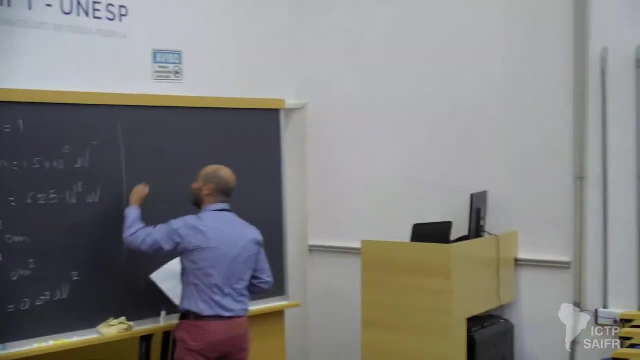 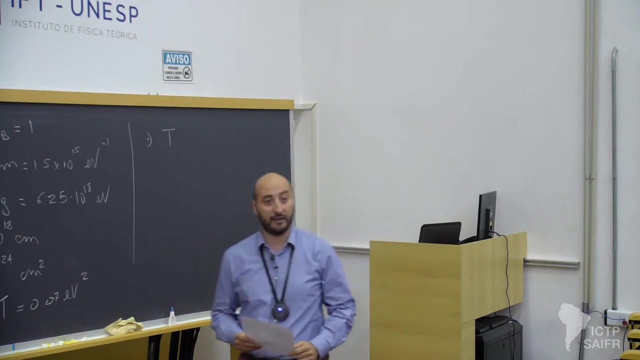 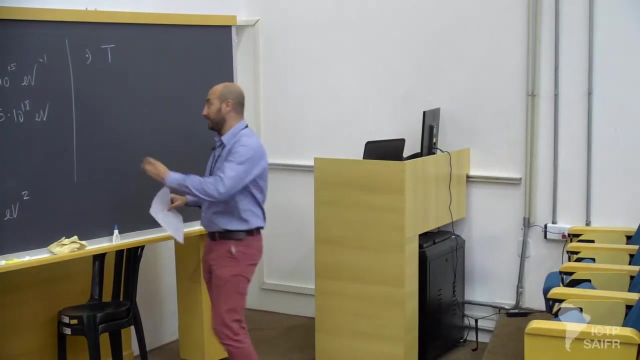 you are not familiar with this. if you are familiar with natural units, you can skip it, but I suggest you to do this kind of exercise. So the first thing is Okay, Okay, Okay. So Temperature: Compute your body temperature in electron volt, assuming you're still alive, then mobile. 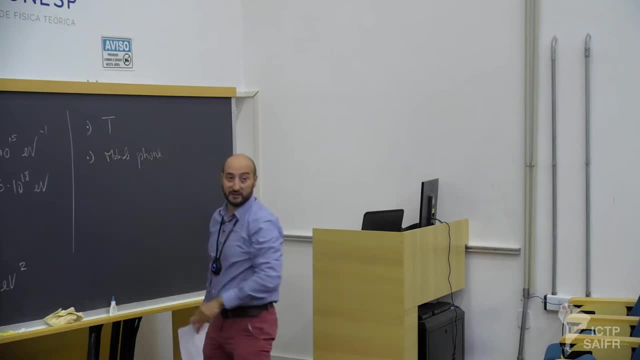 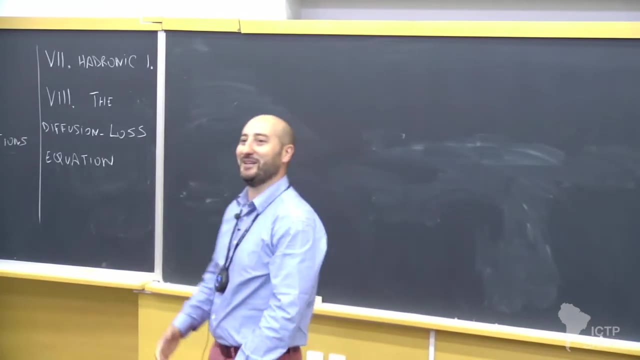 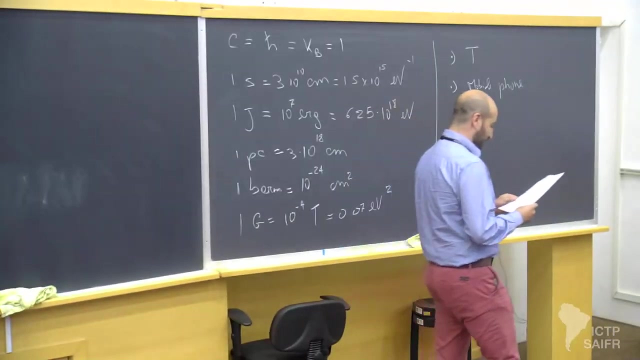 phone compute the frequency of your mobile phone in electron volts. if you know, I hope, what's your mobile phone frequency. Otherwise you can look it up. Okay, your height and weight in natural units. You don't have to tell me the results. 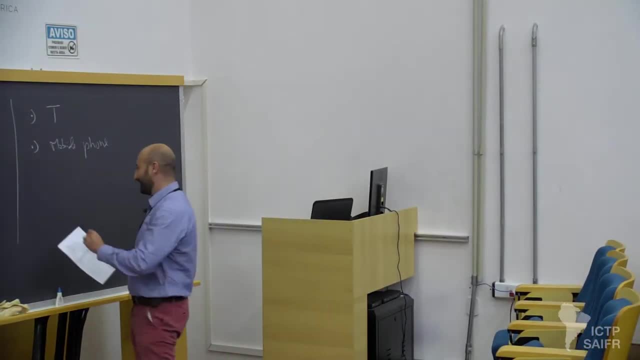 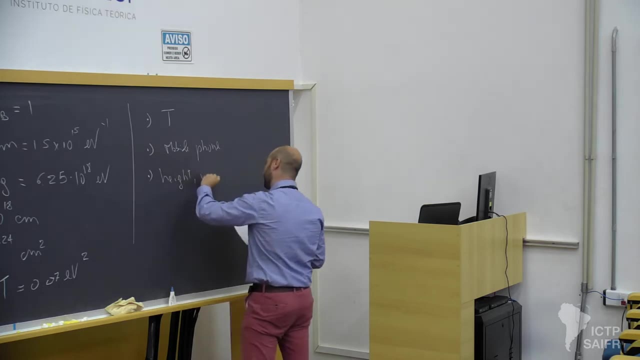 You can keep them yourself And also, okay. so actually you can compute height, weight and age. This is in electron volts. This will be in electron volts to minus one and electron volts to minus one, And then your density in electron volts. 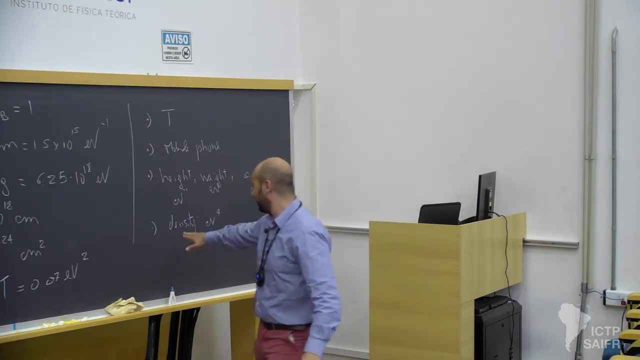 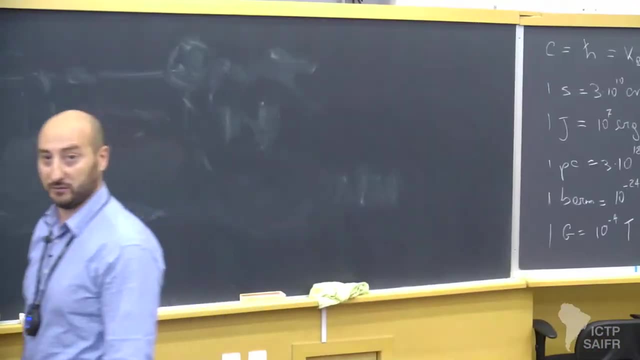 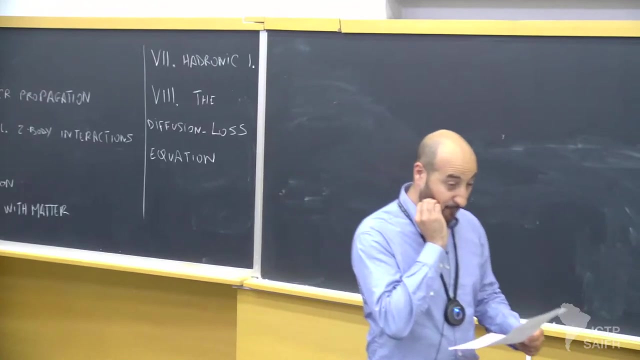 to the fourth. Again, this is within 10%. I hope you know roughly what's a human body density. If not, jump into the sea on a swimming pool and you will get an estimate. And then I told you that there is a. 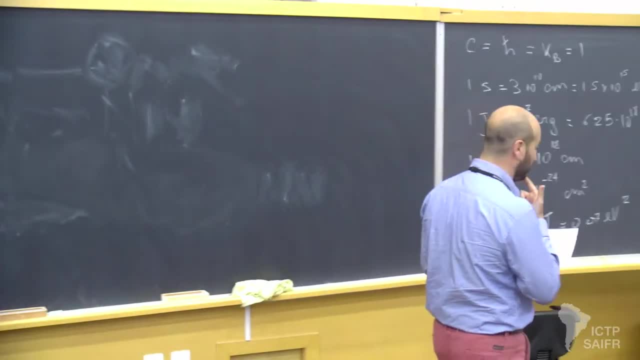 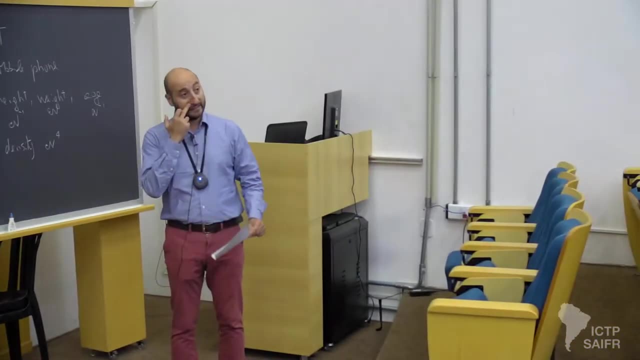 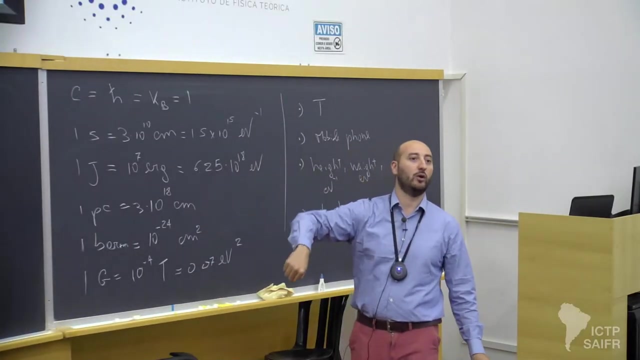 hybrid sort of convention. The convention that is used for electromagnetic units. in most of what I'm saying- if not all, hopefully all- is the Gaussian electromagnetic convention, which means that the four pi's enter into the Maxwell equation, not in Coulomb's law. 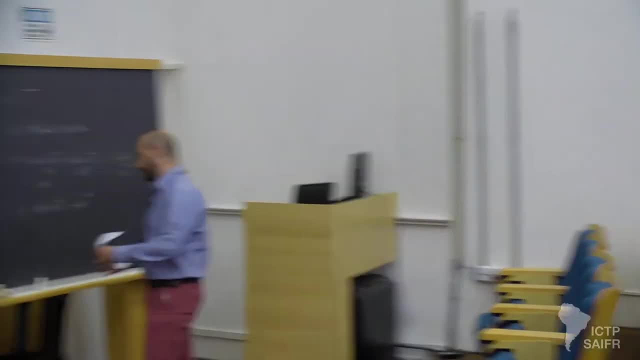 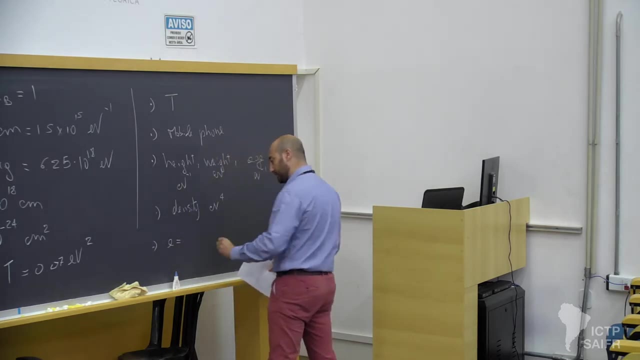 and Biot-Savart's law. And then the electric charge of the positron, which is the square root of alpha, is the square root of one over 137, roughly at low energy, And this is 0.85.. So that you have. 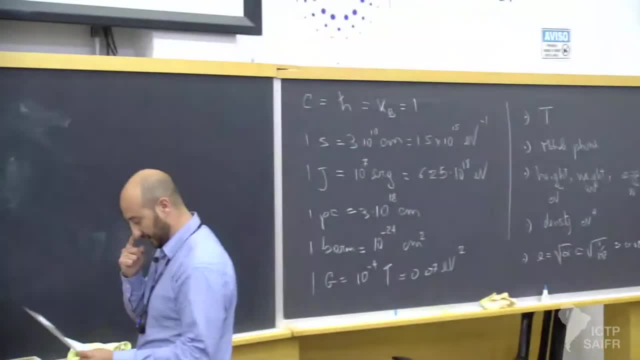 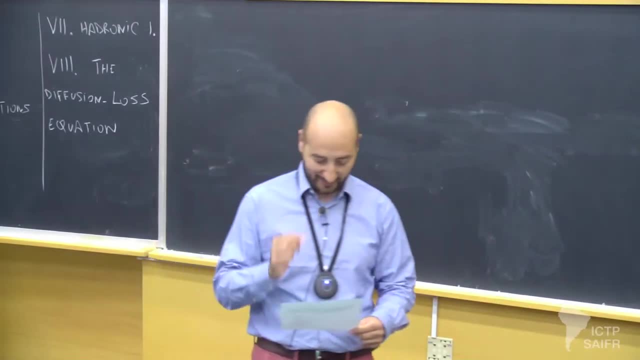 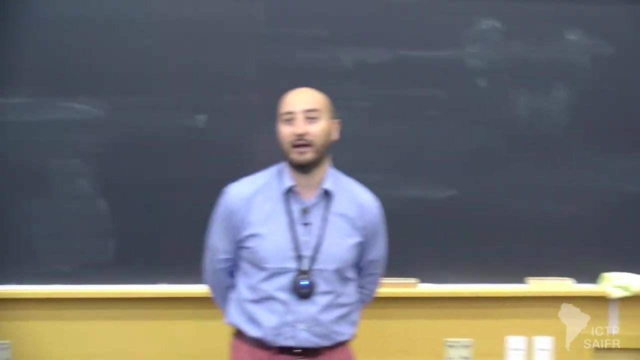 a quick table for numerical conversion in what I'm saying. So this has nothing to do with the subject of the lecture. It's just to set the stage of some basic numerics. Now, how many of you have more particle physics background than an astrophysics? 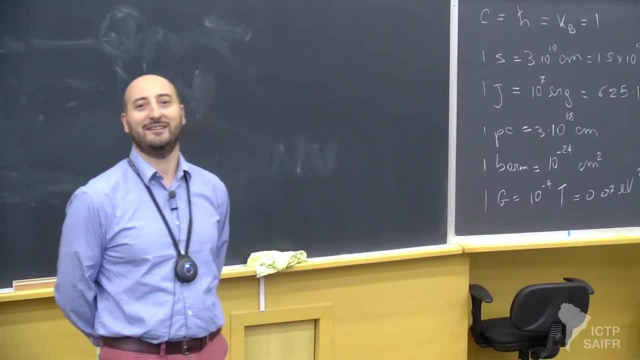 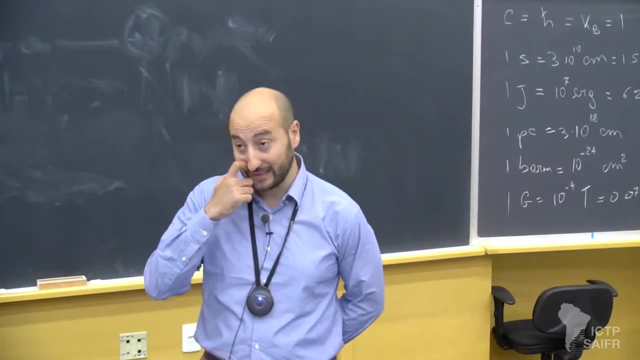 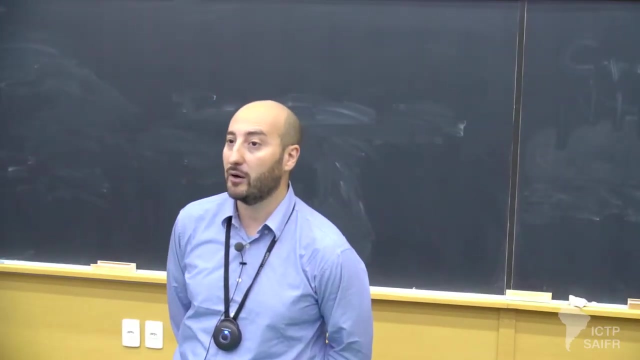 background or just to have a statistical. okay. so it's a minority, I would say. But for those of you who are not familiar with these systems, let me sketch a few of the differences When we talk about galactic environment or extragalactic environment. these 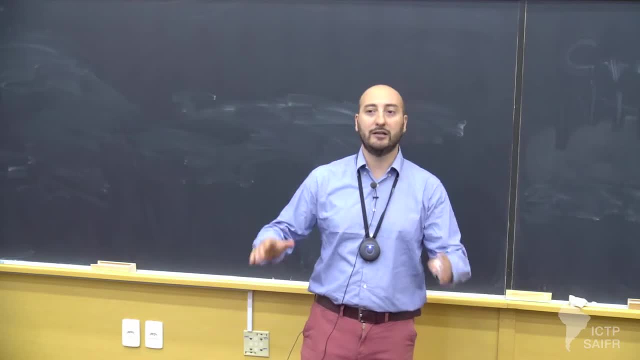 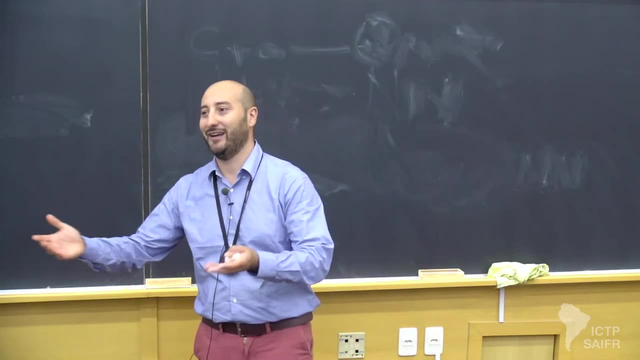 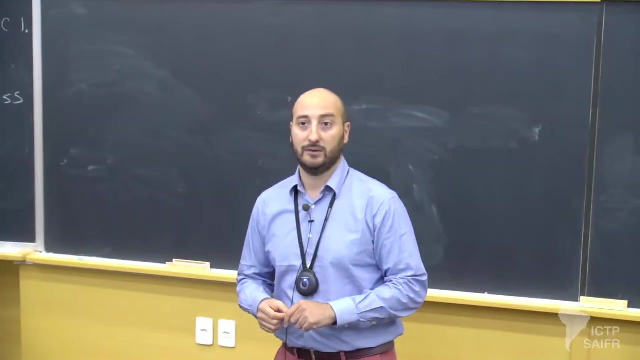 are very, very different from laboratory environments, including the kind of conditions that you may find in the beamline of a collider or so. A first difference is that the density of matter is very, very low. You have very few particles per centimeter cube in the galaxy. 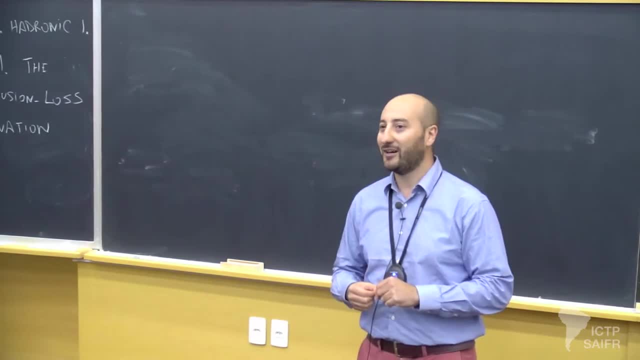 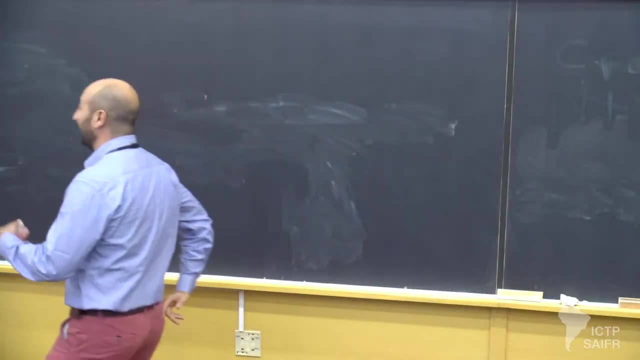 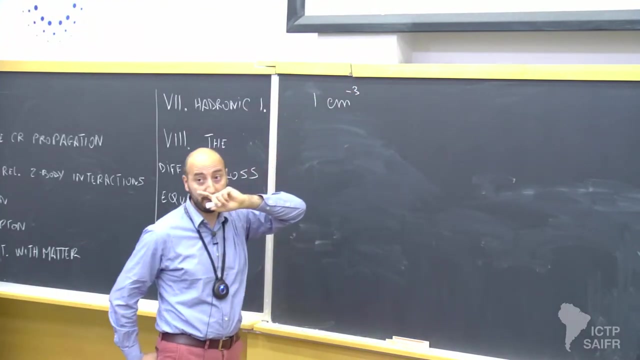 and in the extragalactic space. So it's hard for human mind to conceive how empty these objects are. To give you some idea, the typical densities that you find in the galaxy are of the order of one particle per centimeter Cube, or even. 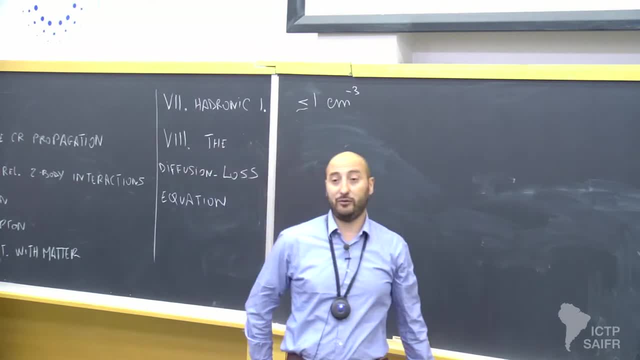 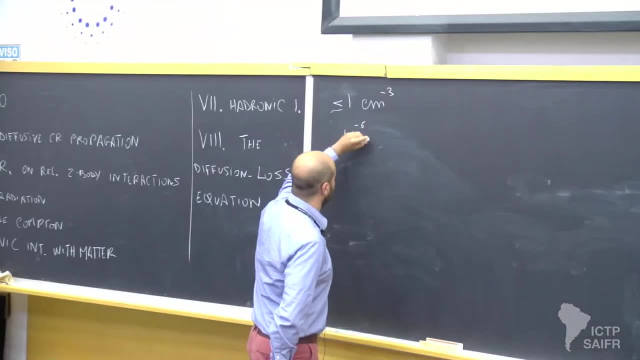 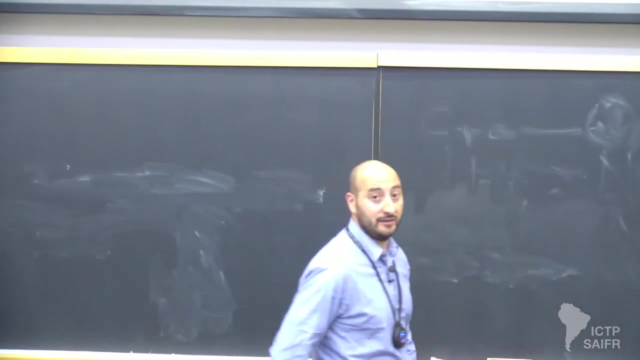 below that, And if you go to the extragalactic space, these drops by something like six orders of magnitude or so. So these are extremely verified objects. okay, Compared to, say, these kind of conditions where you have an Avogadro number of particles per centimeter. 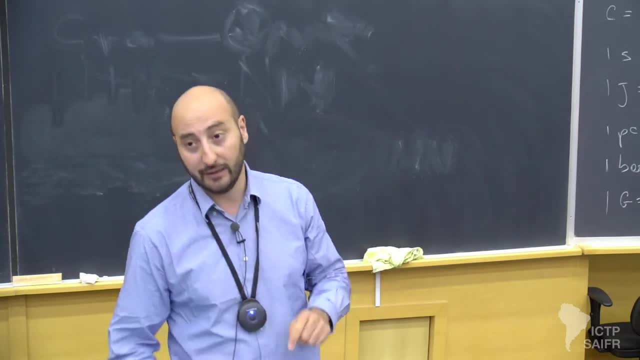 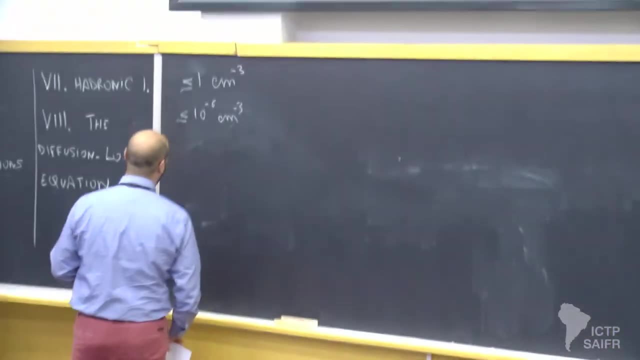 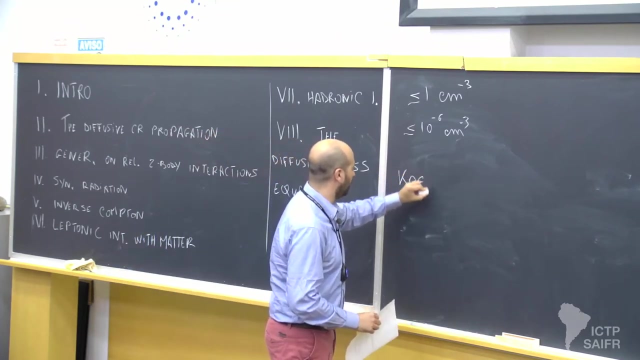 cube of that scale. The second difference concerns distance scales. The distance scales we deal with are very, very large, So a typical distance scale in the galaxy is of the order of a few kiloparsec. The distance from the Earth to the galactic center is about. 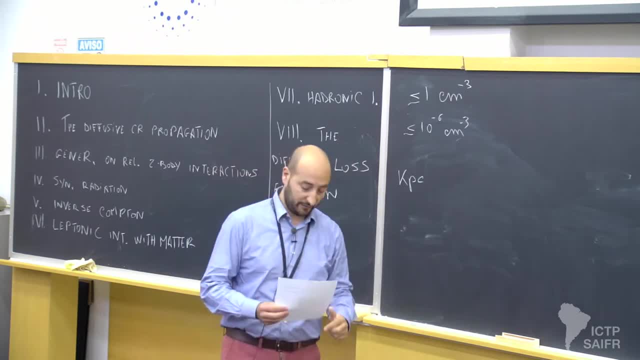 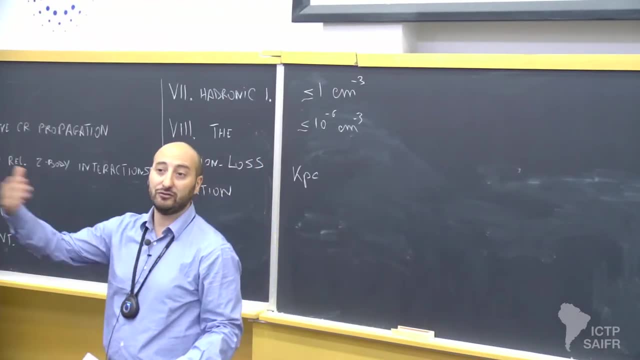 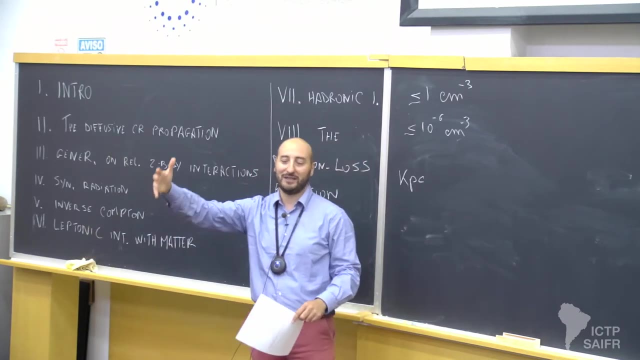 eight kiloparsec. You can have an idea in meters or centimeters by this conversion. Typical distances to extragalactic objects are hundreds of megaparsecs, So the nearest galaxy is roughly Andromeda. so big galaxy, spiral galaxy, is roughly one. 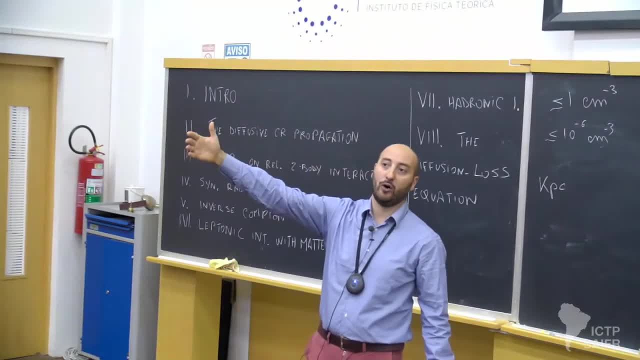 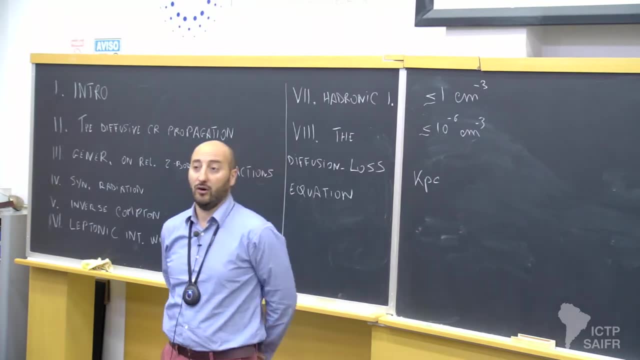 megaparsec away, And typical objects which are maybe invoked to accelerate ultra-energy cosmic rays are typically located at hundreds of, or at least several tenths of, megaparsec, Hundreds of megaparsec if you are below the GZK cutoff. 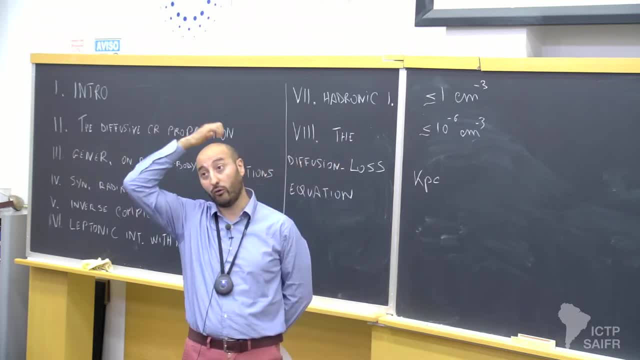 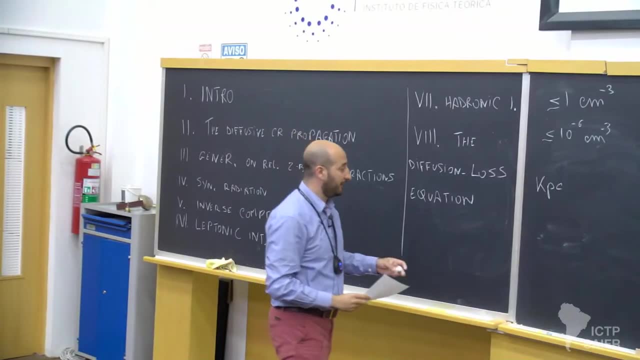 and can go up to gigaparsec or more, for instance for the putative origin of the neutrino flux. So we are talking about very, very large scales. So from kiloparsec for the galaxy to gigaparsec from the extragalactic sky. 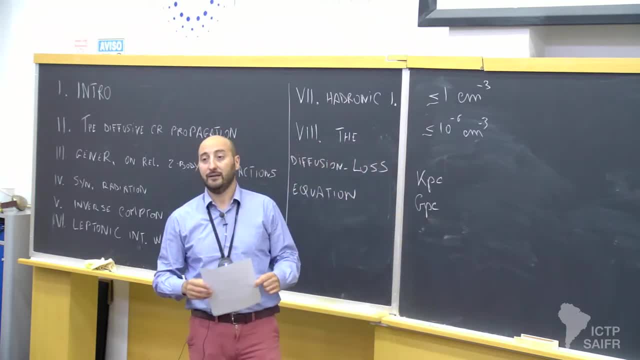 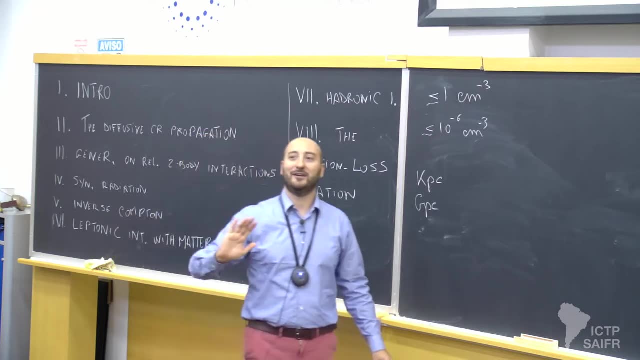 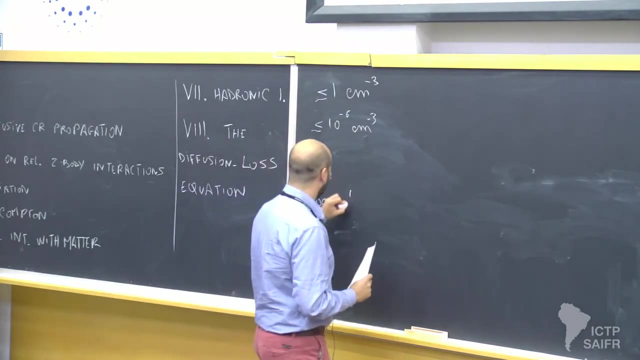 typically, instead of using distances for the extragalactic sky, people tend to use the redshift. Has anybody heard about this concept before the redshift? I see everybody, So it's fine For a quick conversion at low redshifts. 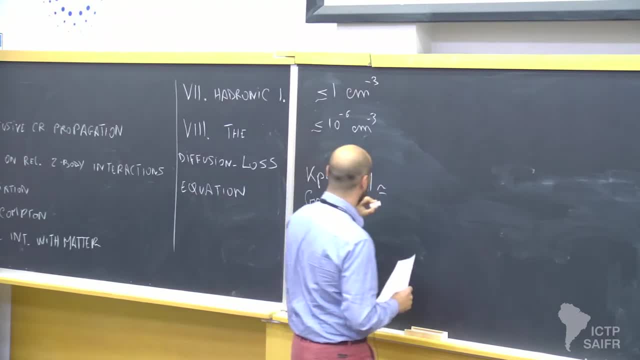 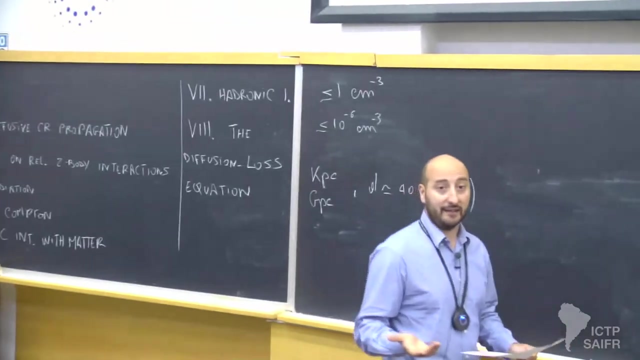 the distance to an object which is extragalactic is roughly 40 megaparsec times the redshift in units of 0.01.. And then there are timescales. These systems evolve over very, very long timescales. You heard in the previous: 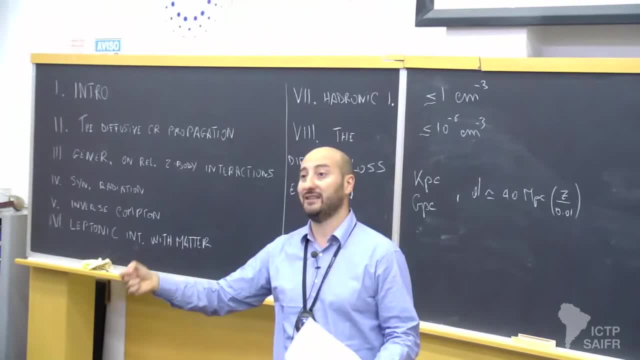 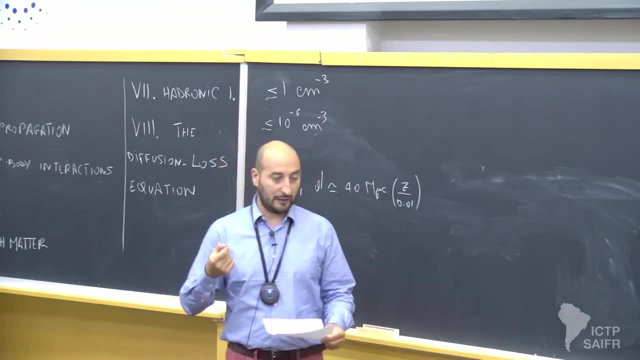 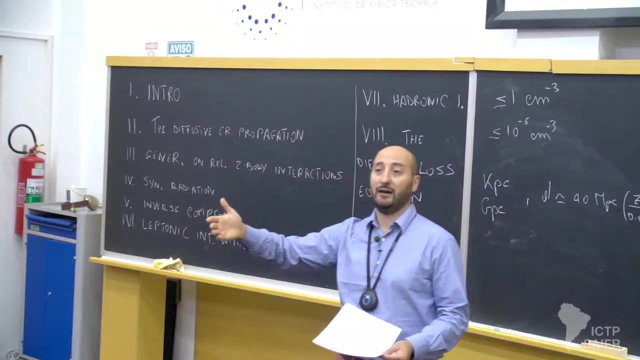 lecture that the typical residence time of cosmic rays in the galaxies are of the order of tens of millions years, maybe 100 million years or so. For comparison, the orbit of the sun in the Milky Way has a comparable length. It's roughly 200 million years. 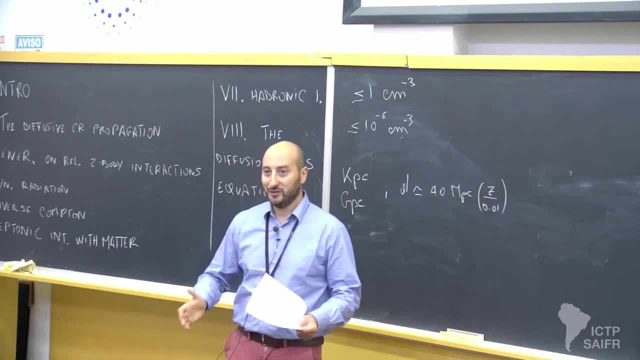 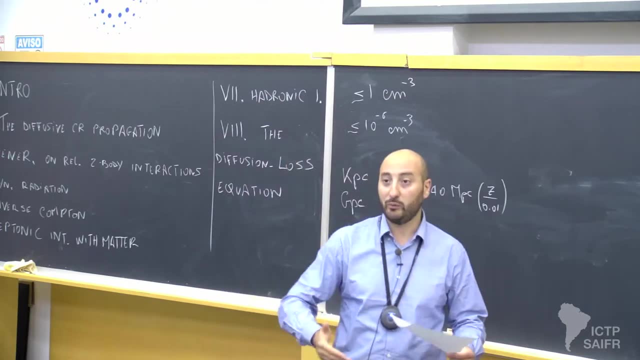 And the age of the universe is 14 giga years, So we are talking about very, very long timescales. This will come back very useful at the end of this lecture Because we will make some heuristic argument why you can neglect some terms, with respect. 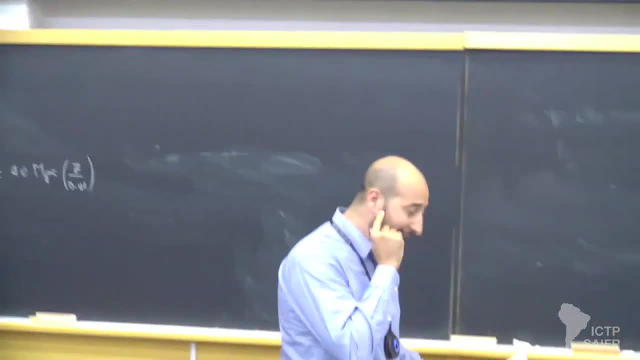 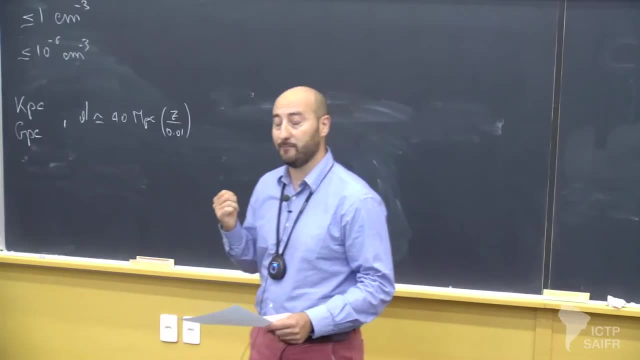 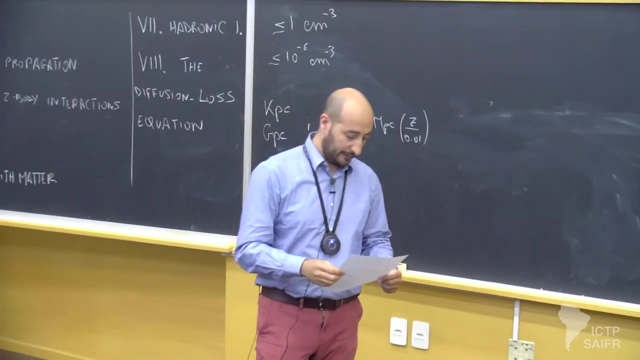 to others, et cetera, et cetera. Another important notion is that the galactic and also actually the extragalactic media are magnetized. OK, So there is a magnetic field pervading the galactic environment. How we get to that conclusion has 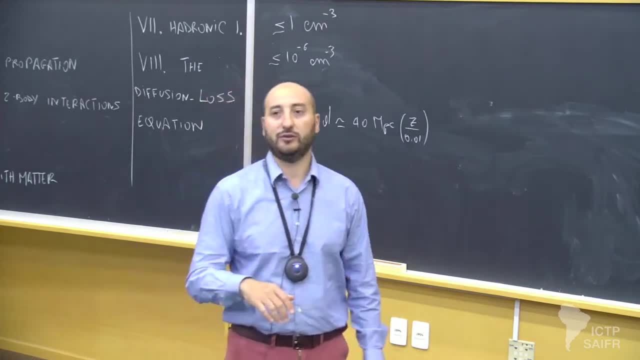 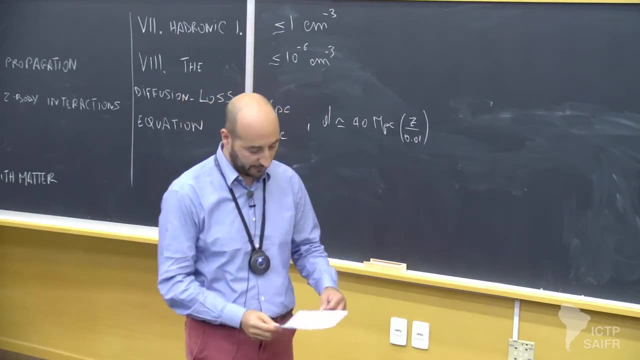 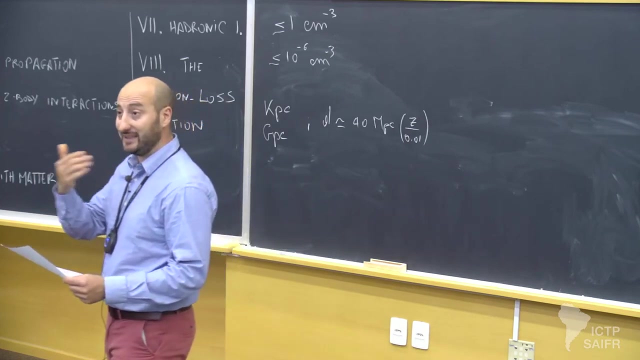 to do with observation through lots of different tools, From faraday rotation to Zeeman splitting, to synchrotron emission and so on and so forth. That's not important for the remaining of these lectures, But there is a typical magnetic field strength. 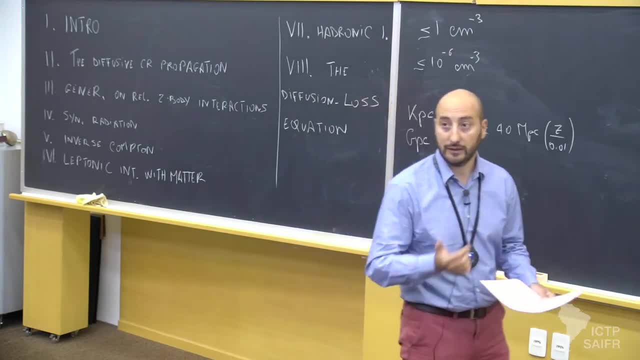 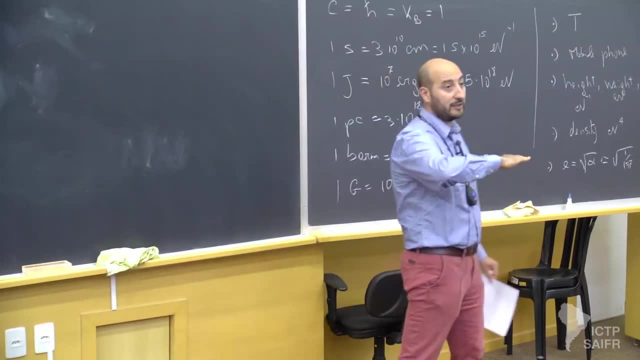 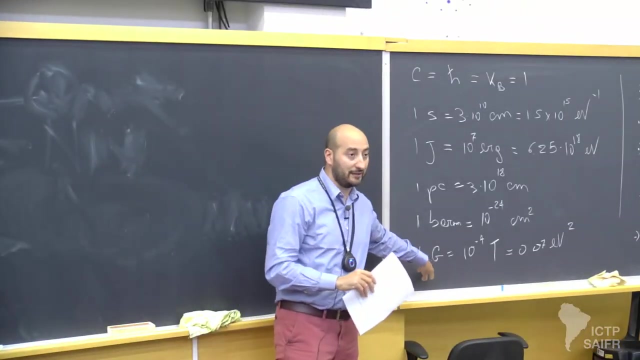 which is of the order of few microgauss in the galaxy. In particular, there is a regular field more or less in the plane of the galaxy, related probably to the spiral arc. But you see that the strength of the galactic field is roughly one millionth of the strength. 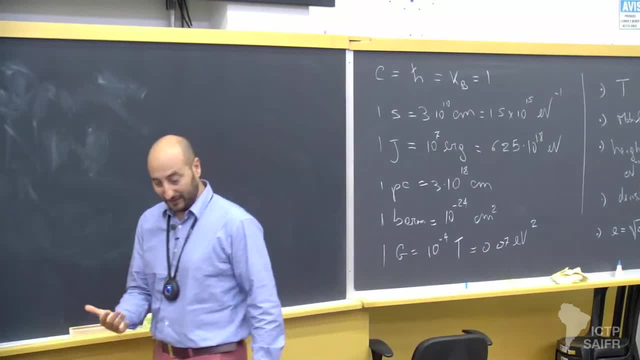 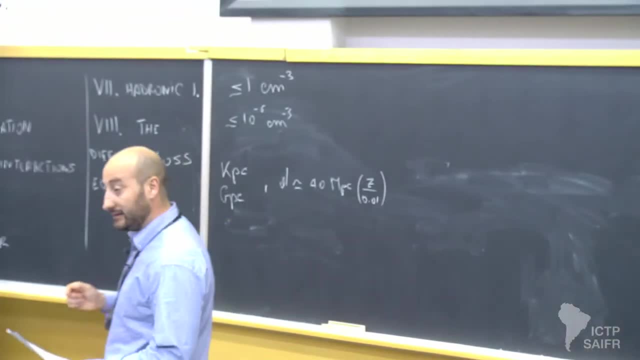 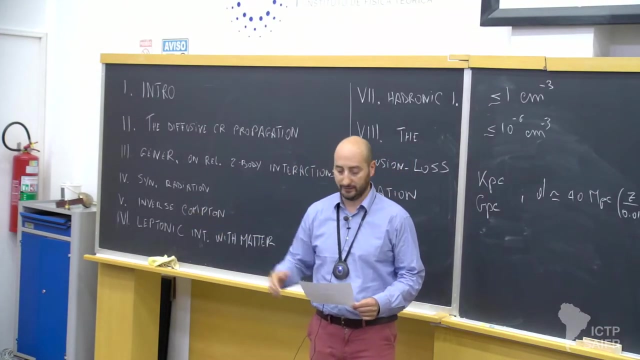 of the terrestrial field. So we are talking about relatively quite small fields from a laboratory point of view. And then another important notion that was briefly sketched in one picture that Pasquale showed is that the radio sky presents some sort of smoothness or some thickness. okay, 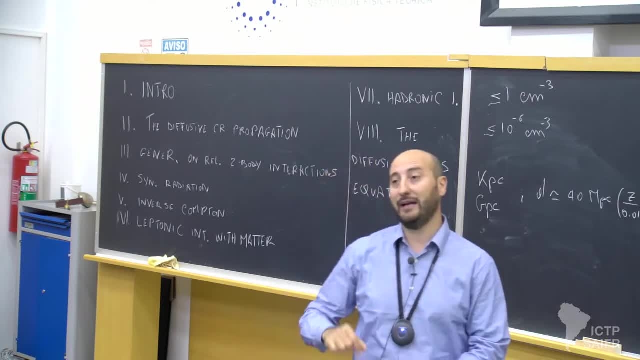 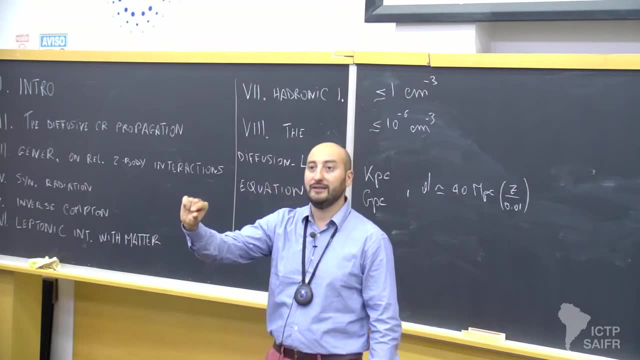 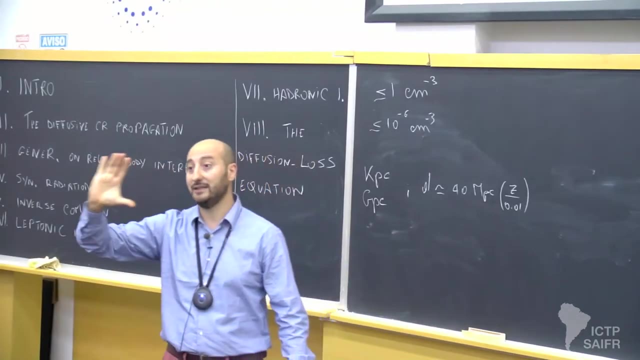 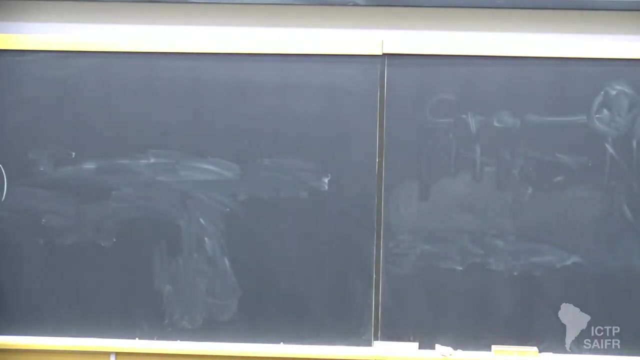 So this has to do with the fact that, despite the fact that the galactic plane, in terms of gas and stars is relatively thin, is something like 100 parsec thick, the magnetized part of the galaxy is relatively thicker, So you can think of the galaxy like Alpha Horus. 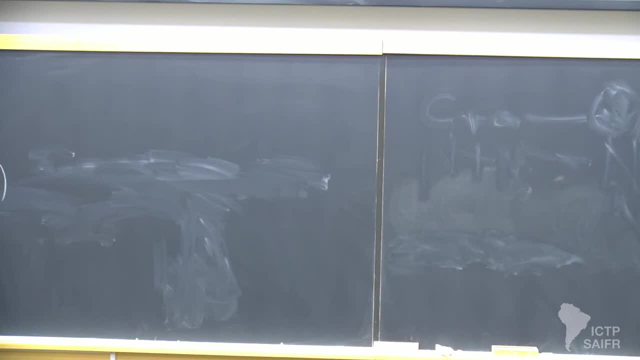 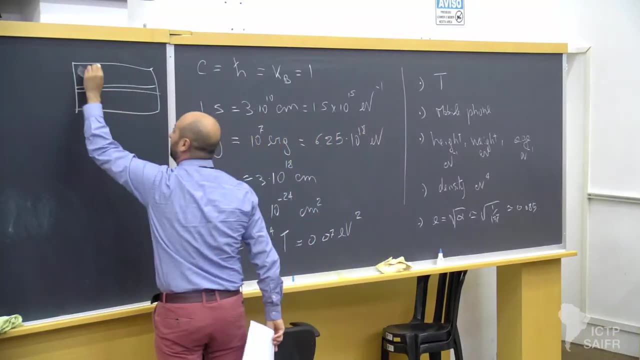 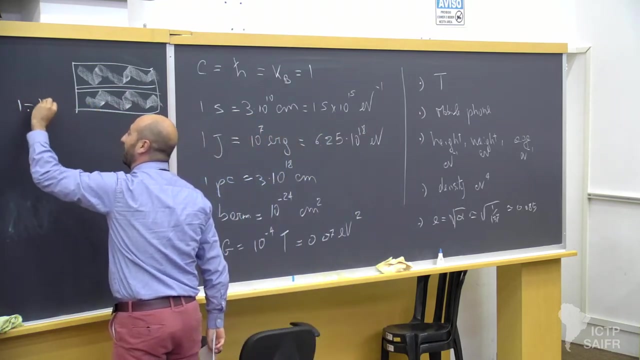 From the side, there is a thin plane That's the Dulce de Leche, And then there is a magnetized area which is much thicker. okay, So this is maybe from 1 to- I don't know- 10 kiloparsec. 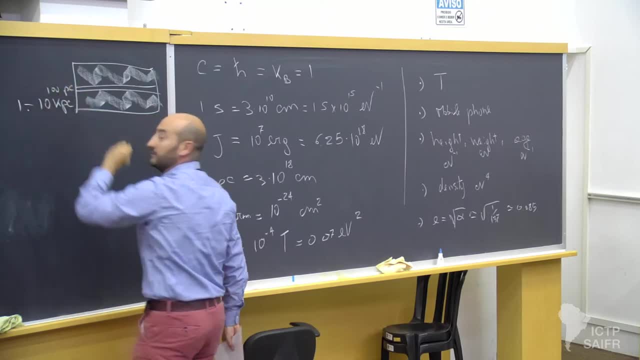 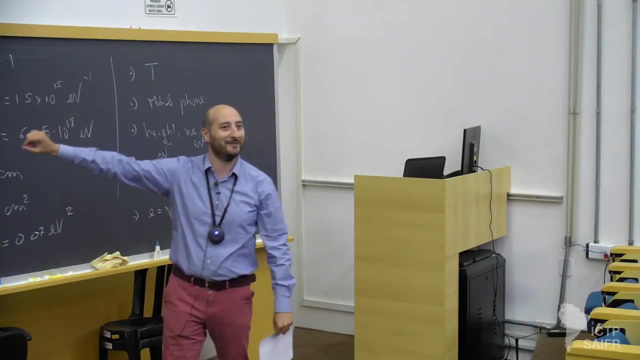 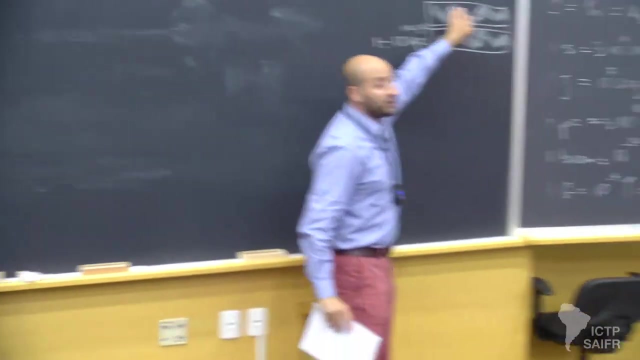 And this is of the order maybe of 100 parsec. okay, So it's a relatively poor cake because there is very little Dulce de Leche and there is very little of the other. But anyway, that's an idea And that's the region where cosmic rays, basically, are propagating. 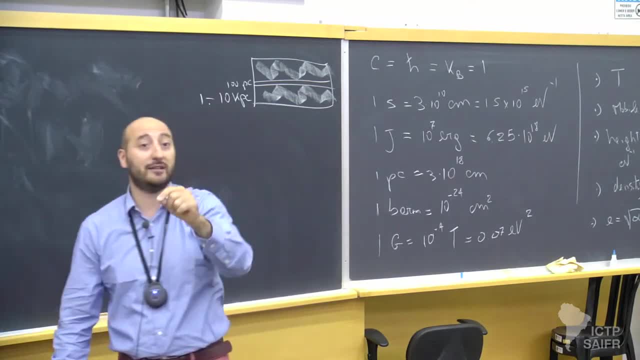 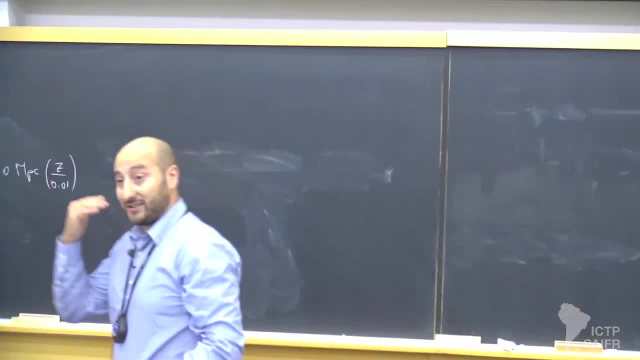 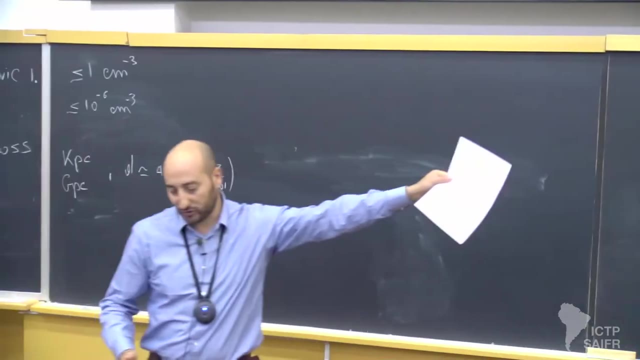 It's much broader than the region containing the putative sources of these cosmic rays, which are stars and all the like. Also, the extragalactic sky is very likely magnetized. Okay, this is still, of course. this is also the description. of the magnetic field of the galaxies. It's an open subject of research in detail. But for the extragalactic sky we don't really know what's the strength and the structure of the fields. However, there is indirect evidence that the extragalactic sky is magnetized. 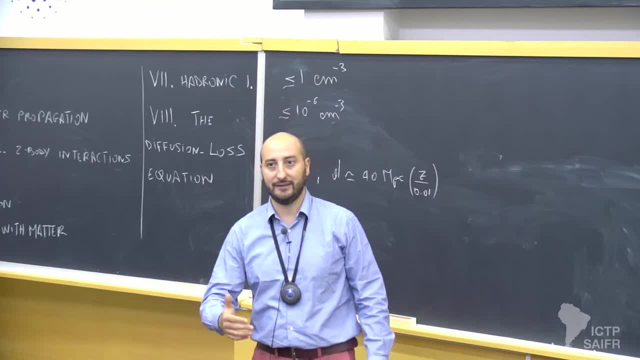 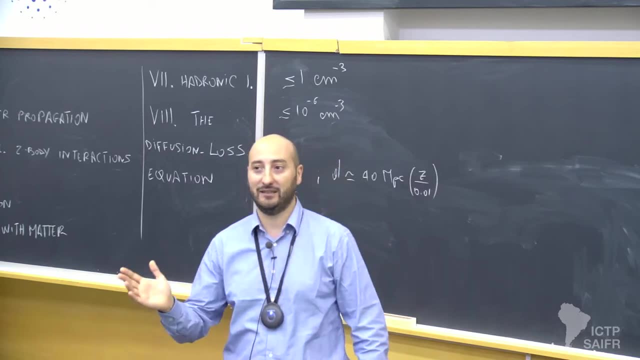 We don't know what's the strength of the magnetic field that is trading the extragalactic sky. Lower limits are around maybe 10 to the minus 19, 18 Gauss, And upper limits are at level of 10 to the minus 9 Gauss. 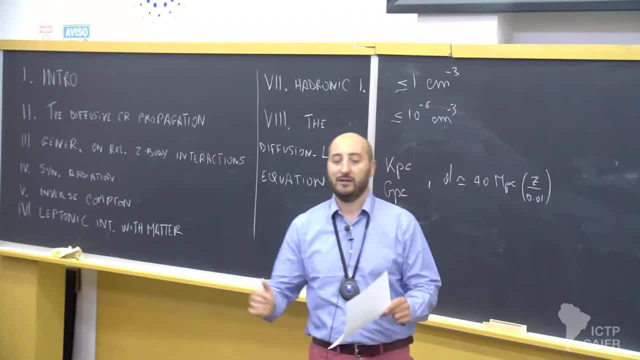 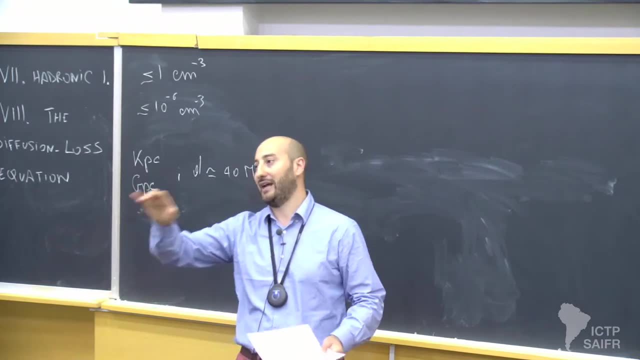 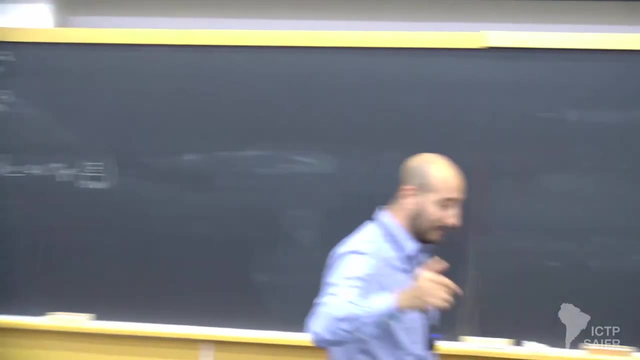 nano Gauss. So somehow in between these two there is a sort of structure which we imagine, probably tracing the filaments connecting galaxies one to another. If you have seen any cosmological simulation you have an idea of what I'm talking about. But probably there are fields also entering the cosmic voids. 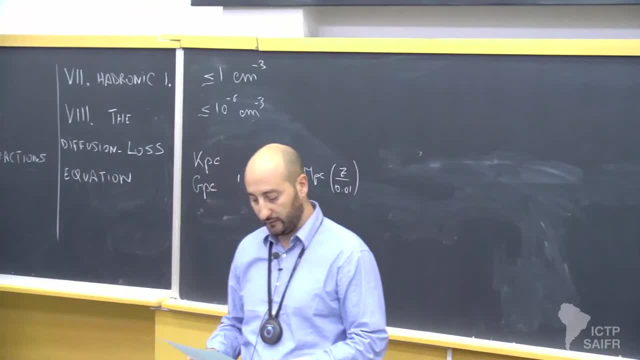 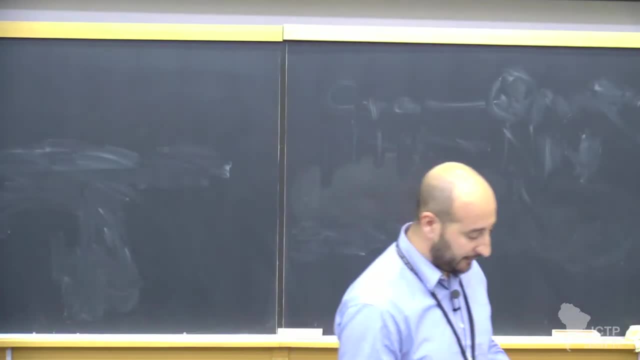 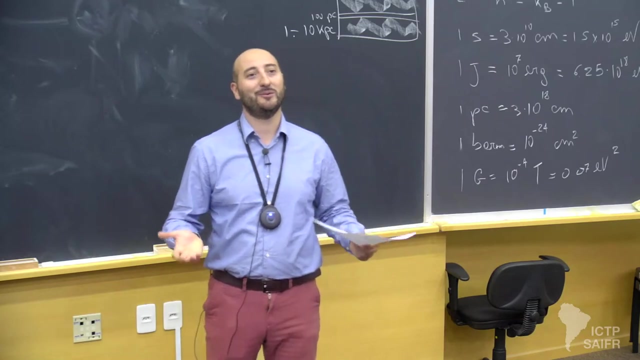 although very, very, very small. This is about magnetic fields, and that's all we need. There is also light. This is not surprising, although we all know that the universe is mostly dark. If you look at the sky, you see light. 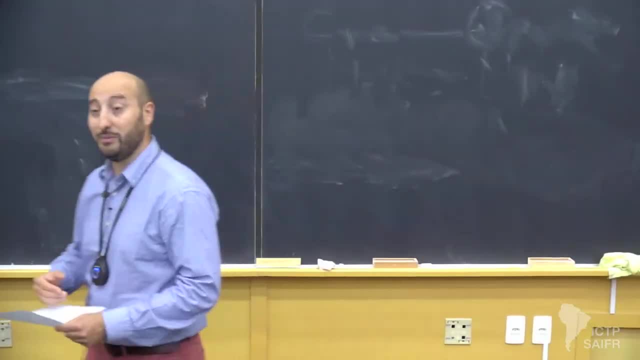 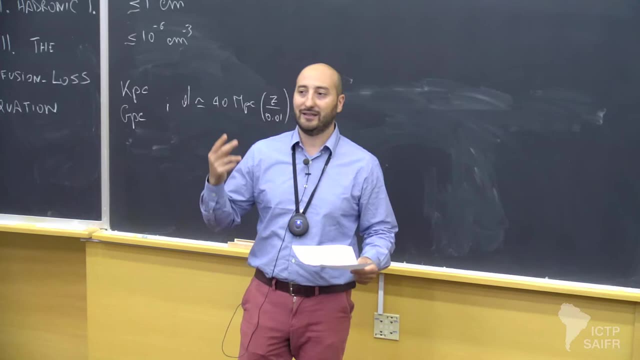 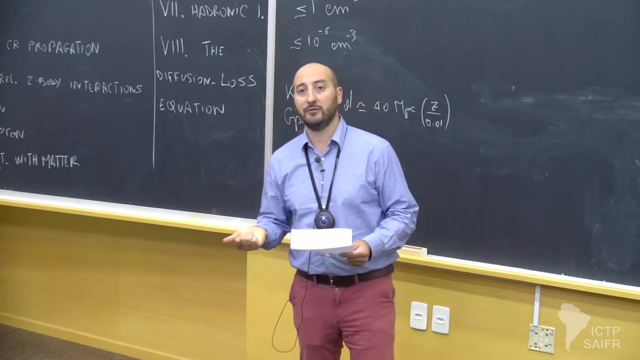 And these lights contribute to the background that the cosmic rays will feel, In particular in the extragalactic sky. there are two backgrounds of light, which means photons That we have to take care of. One is the cosmic microwave background. You have heard about it, I hope. 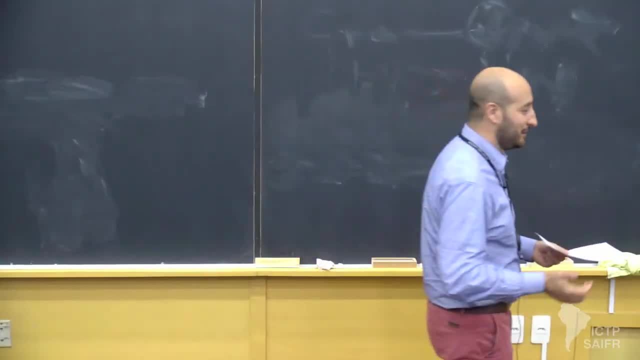 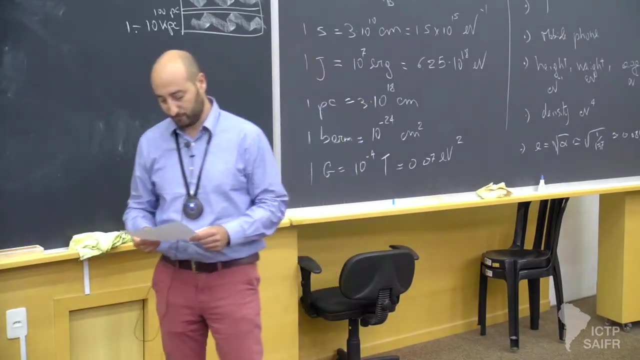 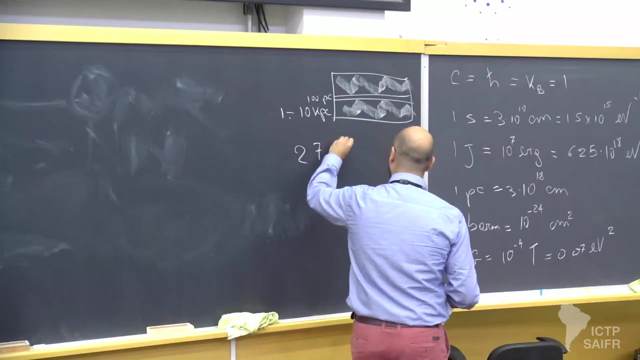 This is the thermal radiation. It's a blackbody radiation, almost isotropic, that pervades the whole sky. corresponds to a blackbody with a temperature of roughly 2.7 Kelvin, okay, And the energy density today is roughly 0.3 Kelvin. 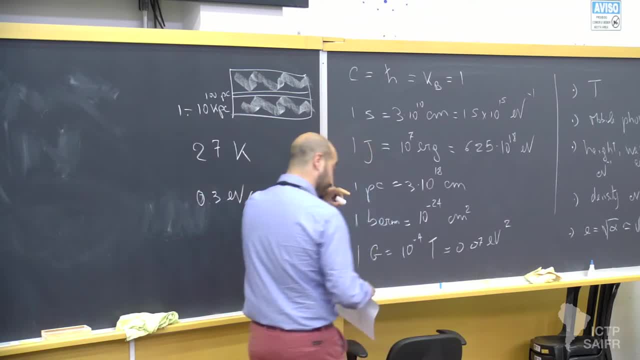 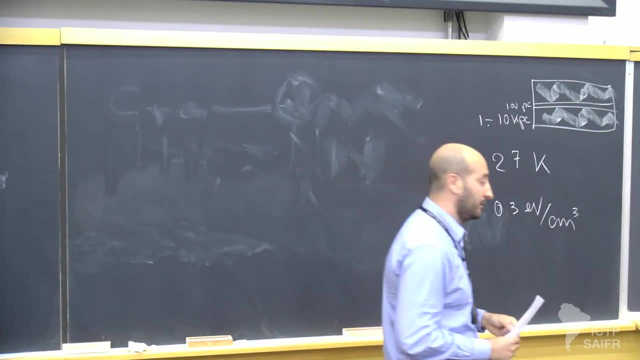 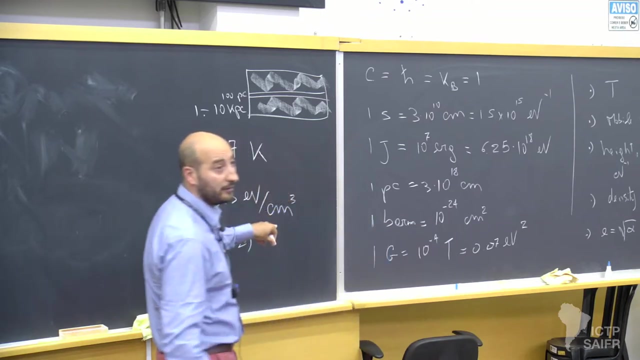 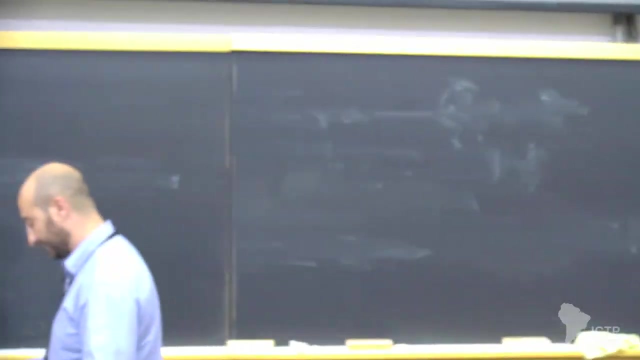 Electron volt centimeter cube Roughly a little bit below This. energy density scales quickly with redshift okay. So earlier in the universe this is 1 plus z to the fourth power higher And the number of photons is growing with the cube of 1 plus z. 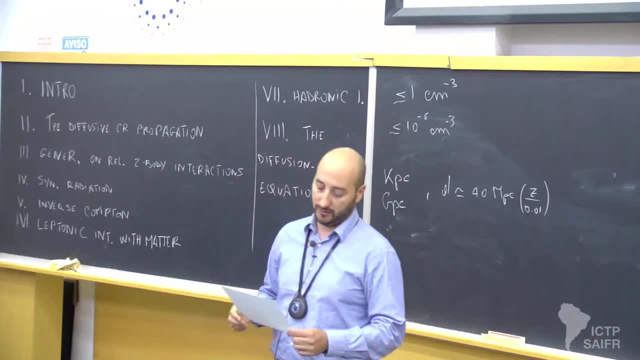 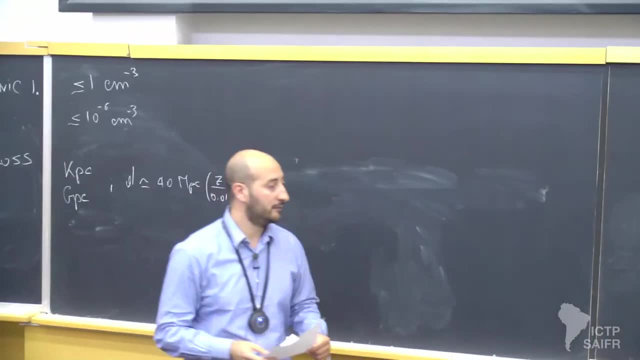 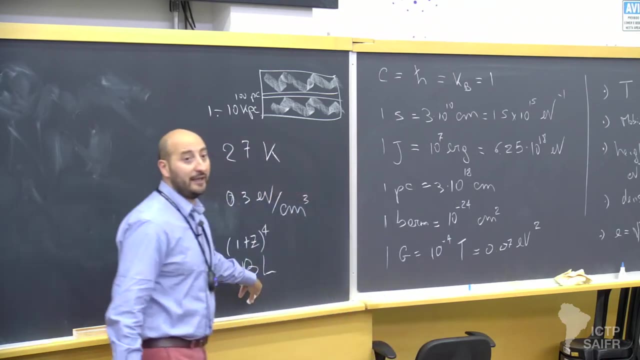 And there is another background which is of importance for cosmology: Cosmic rays propagating over the extragalactic sky, which is the so-called EBL, EBL, extragalactic background light, which is not surprising there, because there are stars and galaxies all over the sky. 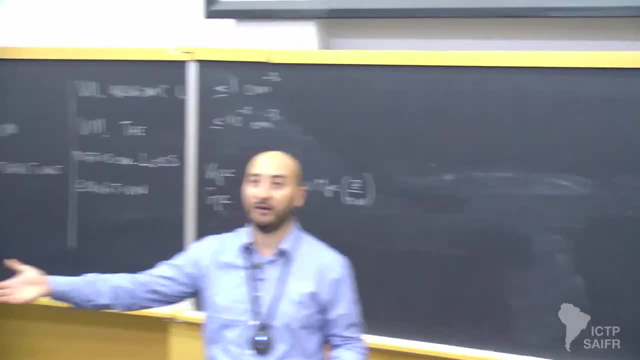 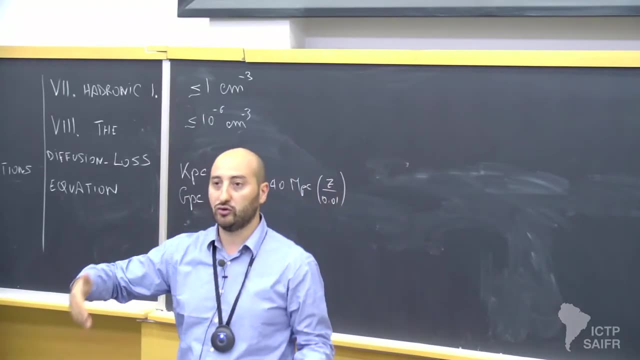 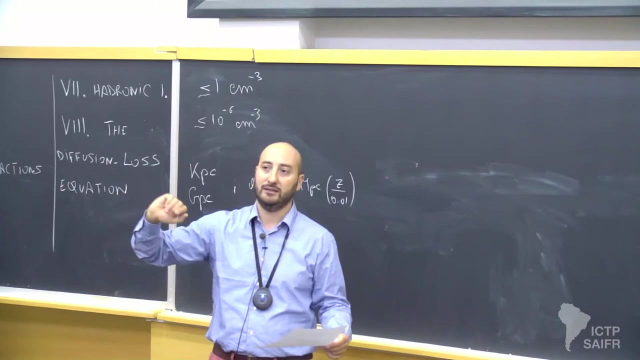 They emit light, in particular optical ultraviolet light, and this light contributes to a diffuse background filling the whole universe. Actually, there is also an important infrared background association. It's associated to the EBL, which comes mostly from reprocessed light into the infrared band. 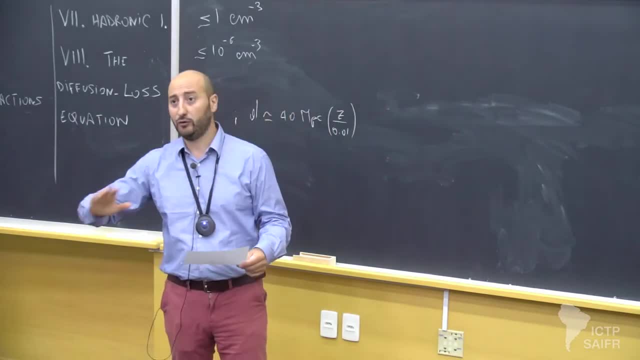 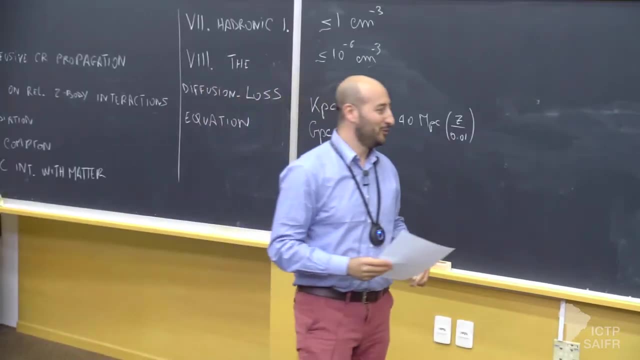 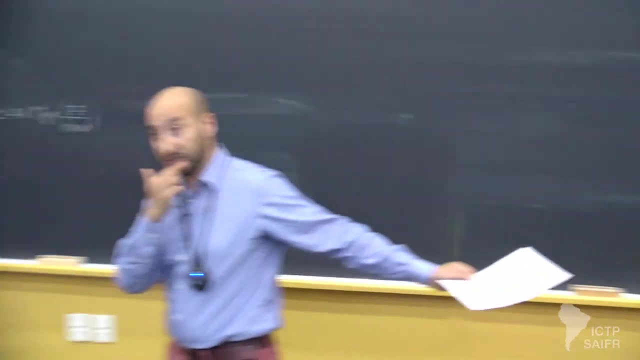 through scattering with dust. okay, If you do cosmology you know that dust is a very important object, But for us it's only contributing to populating a lot this part into the infrared And roughly. actually this is much less abundant than the CMB. okay, 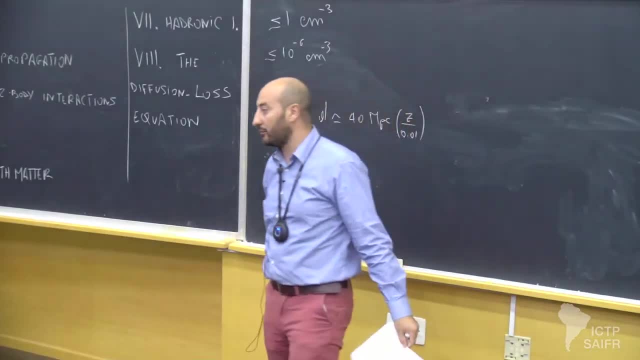 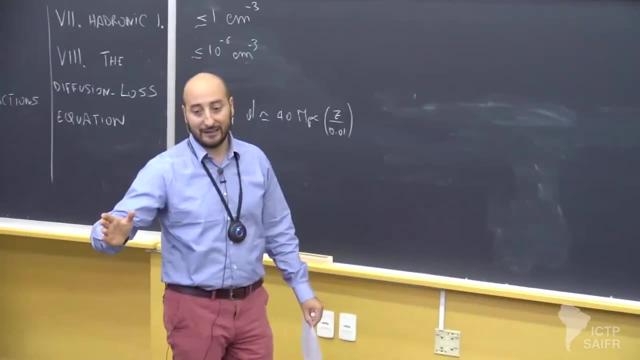 The energy density in the EBL is, I think, a couple of order of magnitude below the CMB. However, since these are optical photons, ultraviolet photons and so on, there are some processes which are characterized by threshold, So they need targets of higher energy. 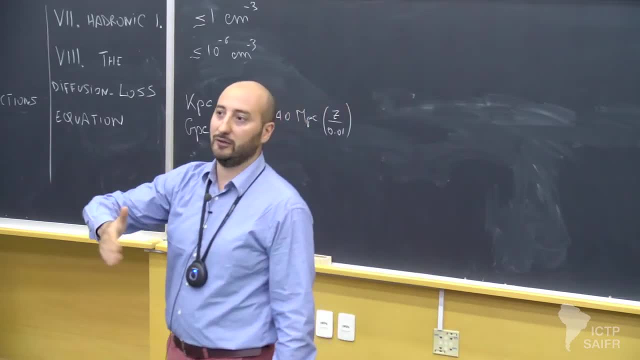 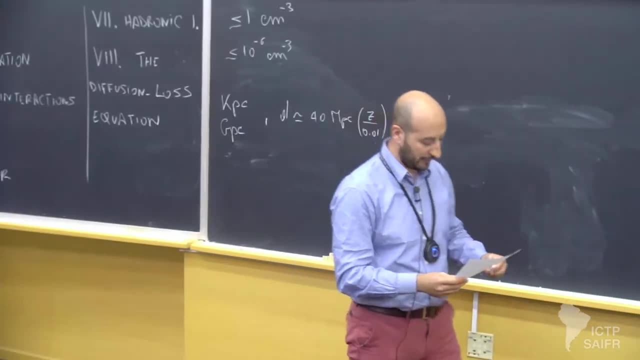 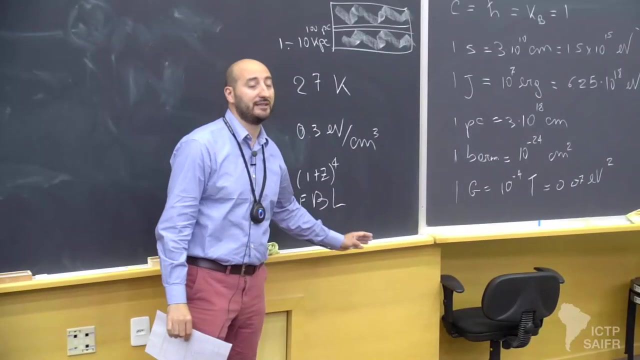 and they can be operational earlier on in the propagation of cosmic rays. So we will see what I refer to in, probably toward the end, third or fourth lecture or so. And then, okay, there is a similar contribution from stars and dust in our own galaxy. okay, 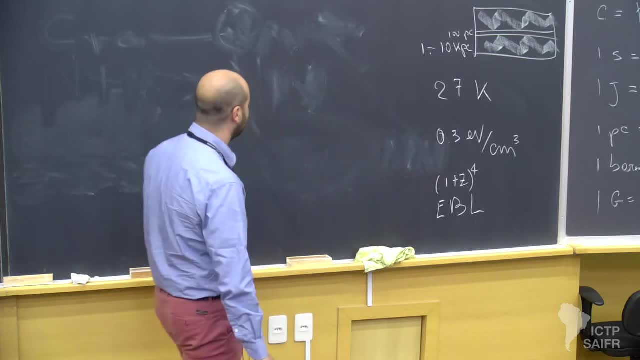 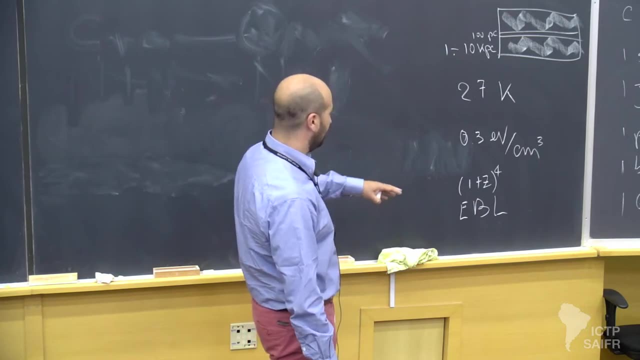 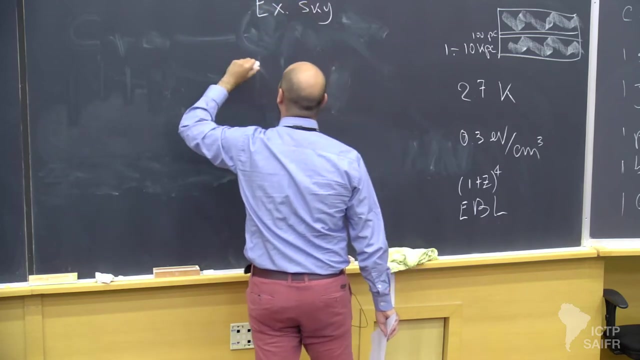 So besides the CMB, which is everywhere, including our own galaxy, there is starlight and there is infrared light In our galaxy. that's not true anymore. So in the extragalactic sky you have a sort of hierarchy. So the energy density U in the CMB is not true anymore. The energy density in the CMB is much larger than the energy density in the EBL In our galaxy. that's not true. So the energy density in the CMB is actually lesser or equal than the energy density in starlight. 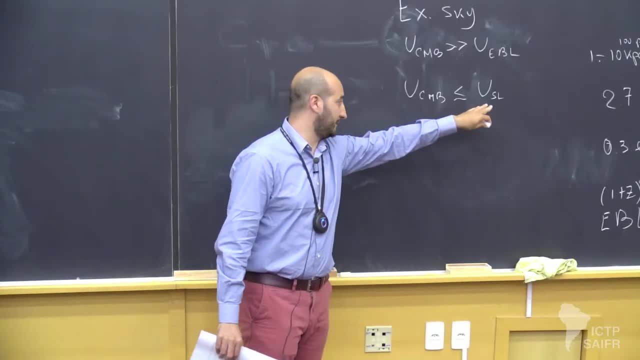 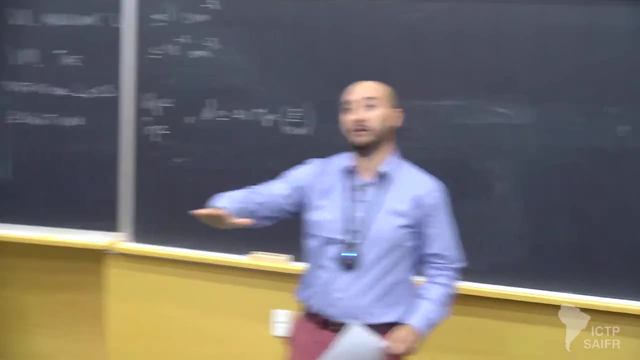 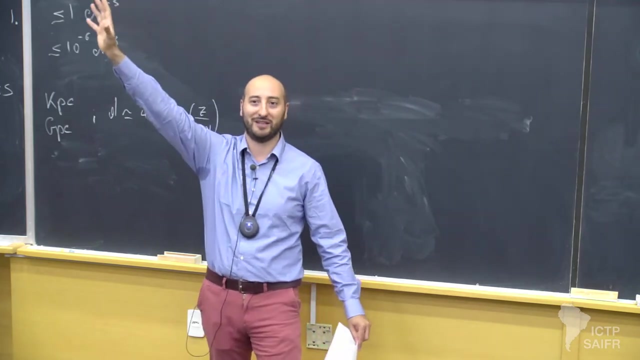 And another important difference is that the energy density in starlight depends on your location in the galaxy. This you immediately realize, especially in the southern hemisphere. You look in the night sky. you see that there is a starlight, There is lots of stars toward the inner part of the galaxy. 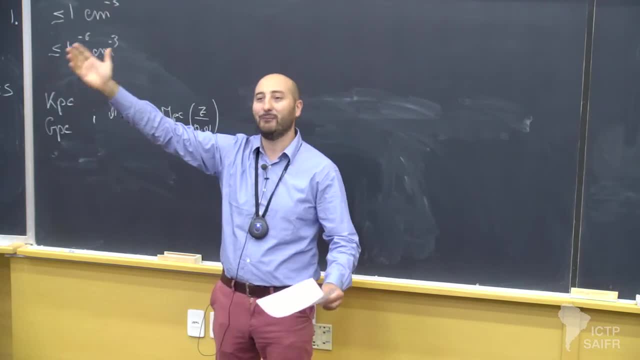 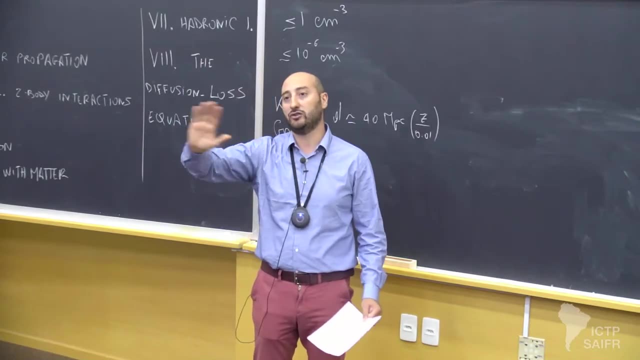 the Milky Way, the bulge, et cetera, And, okay, some of it you don't see because there are clouds and there is absorption, But clearly the night sky is not homogeneous. okay, So towards the inner galaxy, there are more stars. and there is more light, And this is probably locally around the sun. the amount of energy in the CMB and starlight are comparable. If you go toward the inner galaxy, there is a hierarchy of a factor of 10 or even 100 higher starlight. 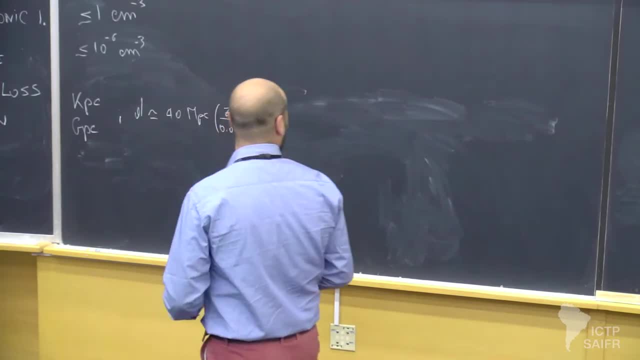 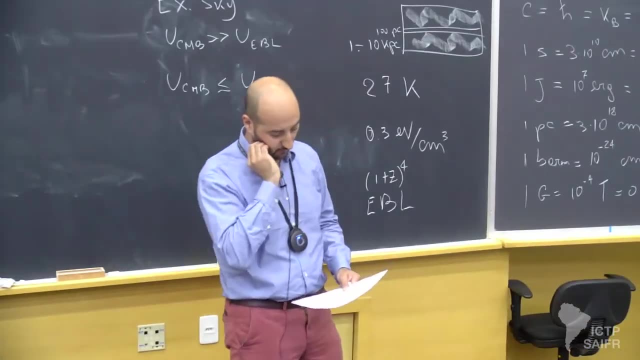 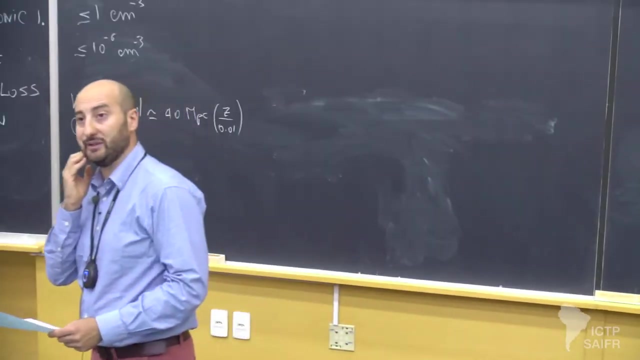 So so far, so good. I think this is the only notions I need you to keep in mind for quick estimates of some processes in the following, Let me reintroduce a few notions about random movements. Probably you know about them, But it's a little bit complicated. 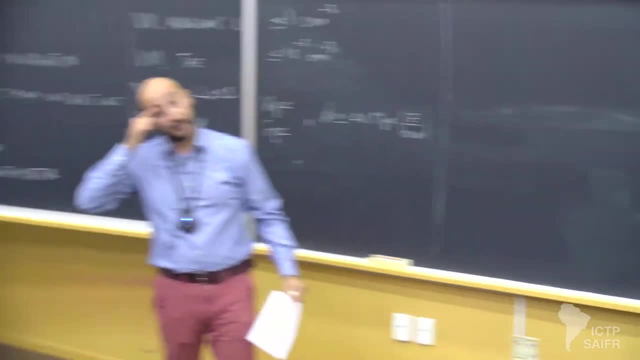 So let me introduce a few notions about random movements. Probably you know about them, But it's a little bit complicated. So let me introduce a few notions about random movements. It's good to set some stage If you have a medium which a finer density of a target. 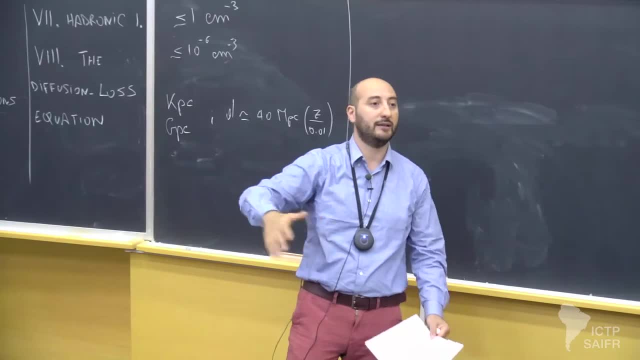 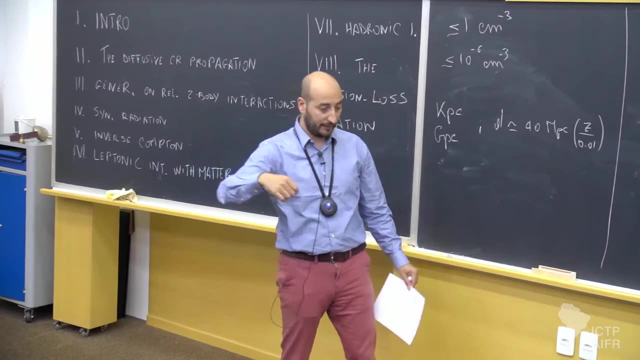 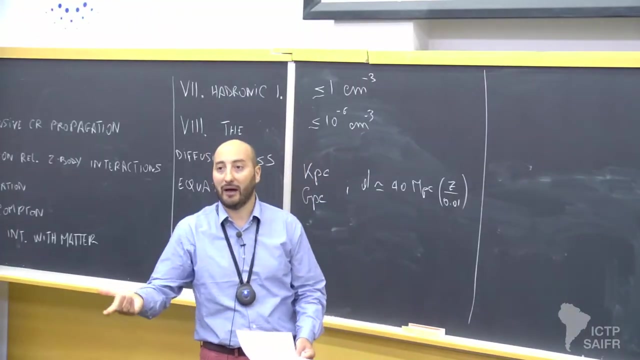 and there is a process. for instance, think of a photon propagating in a material. okay, The type of propagation that this photon will experience is essentially described as a random motion. okay, There is a characteristic length, which we call the mean free path. 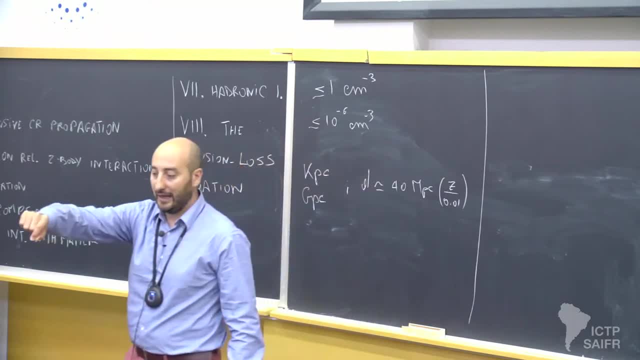 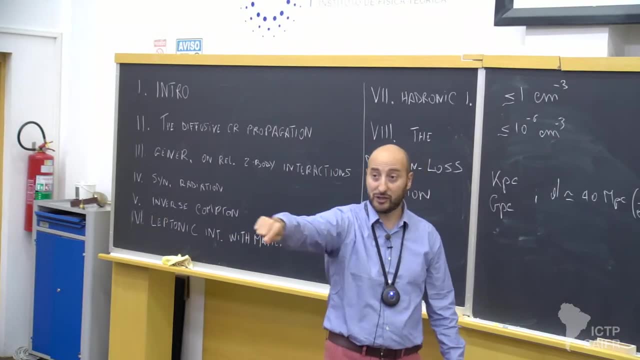 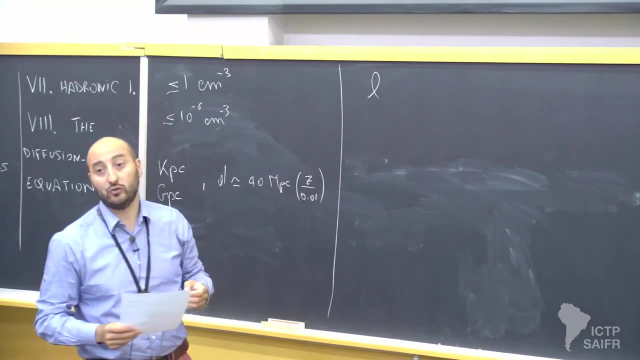 over which the photon moves straight, And then every night it moves Now, and then this will bounce against some target, an atom, for instance, of your medium, and change its direction. okay, So the characteristic length, the mean free path, L, has to do. 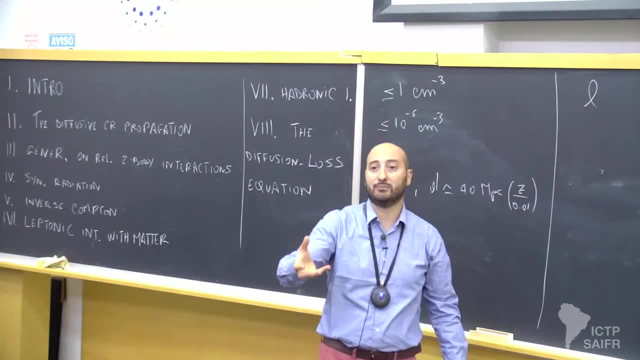 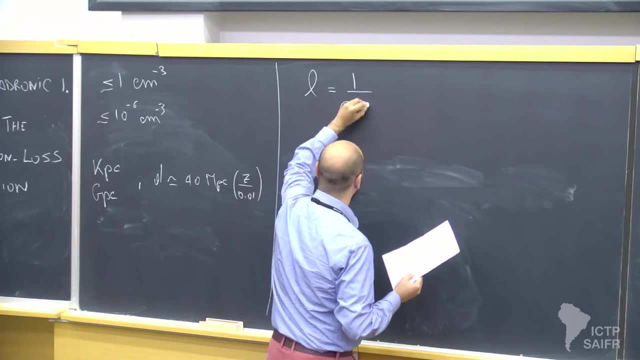 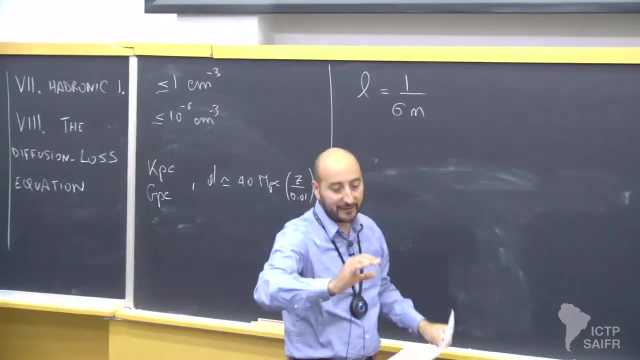 with the density of your medium and with some intrinsic properties, which is the cross-section. In particular, this length is 1 over the cross-section times the density of your medium. okay, So you can think of it as the effective cross-section that the target presents. 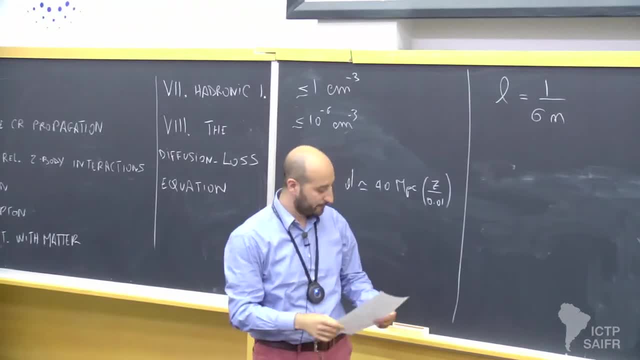 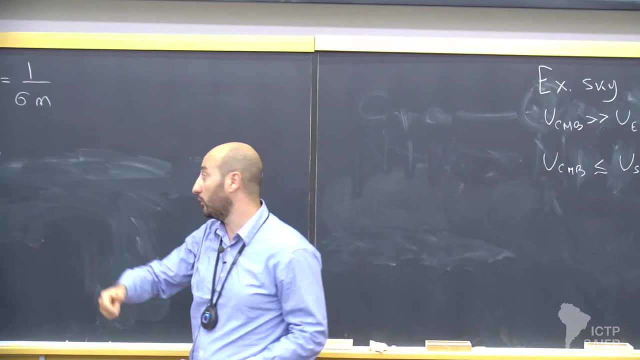 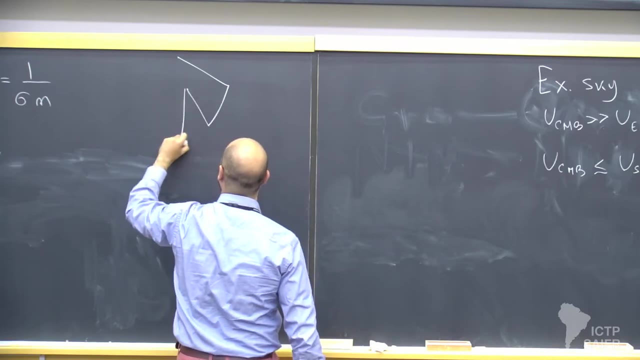 to your photon or other particle in its propagation, And then there is a rate of interaction, of course. So there is a typical time scale over which your photon, let's see, will go on straight and then move, changing direction. okay, 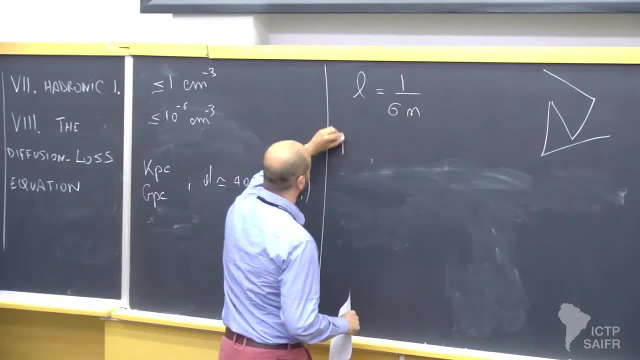 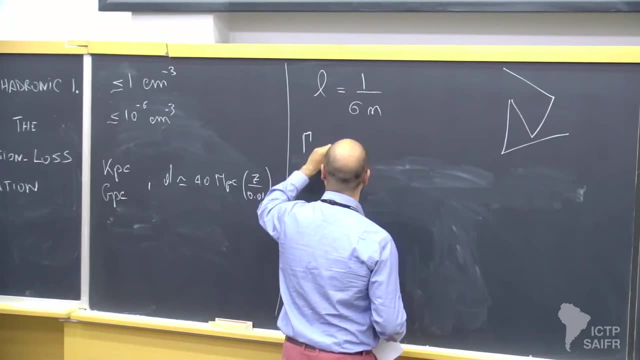 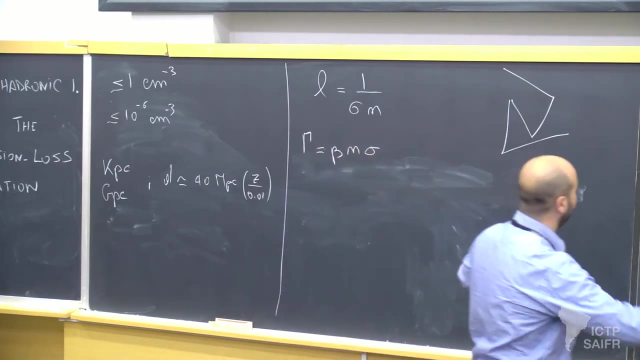 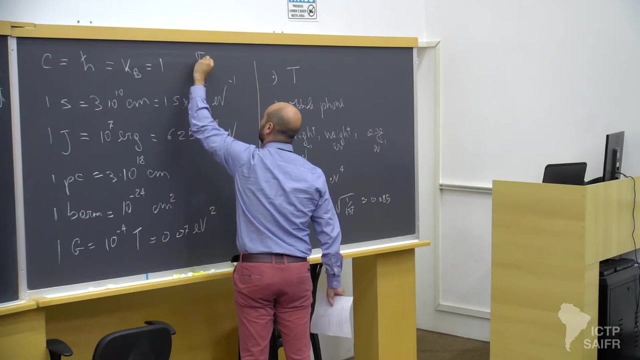 And this rate let's denote with gamma. this rate is nothing but the velocity of your particle, which I will denote: beta times, the density times the cross-section. Remember that if I put c equal 1, v over c, which is typically denoted. 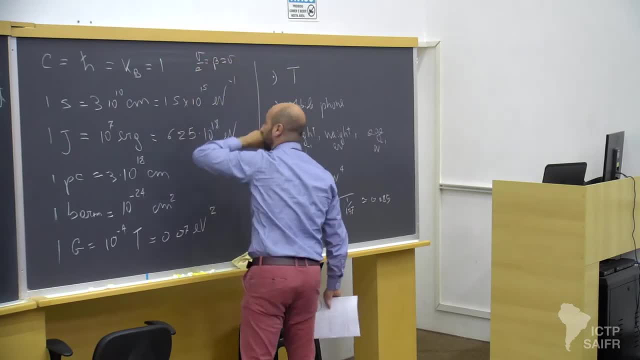 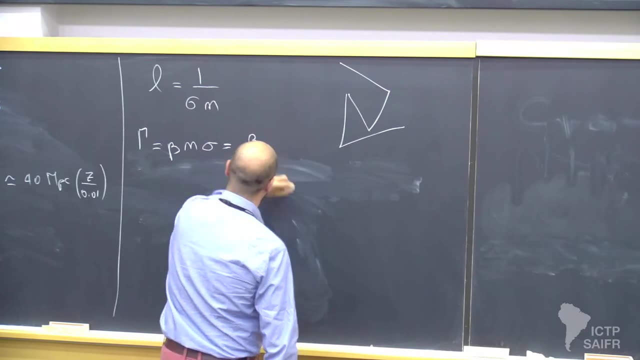 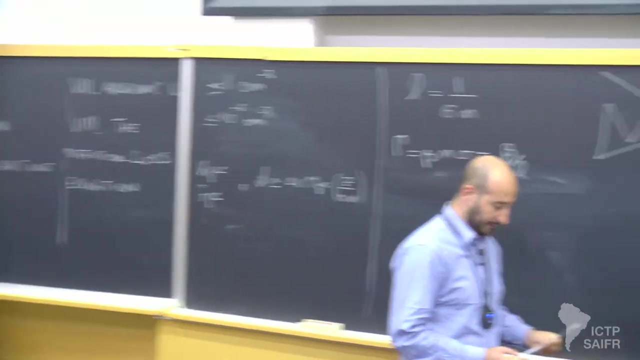 as beta is also equal to v, And you immediately see that this is nothing but beta over a. Okay, So this is the inverse time after which your particle will have interacted. Nothing so complicated, And there is also a notion of optical depth. 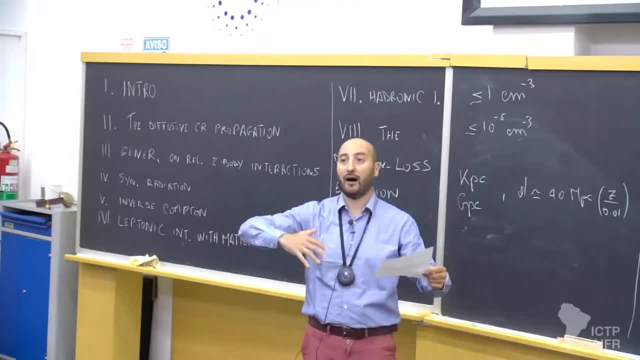 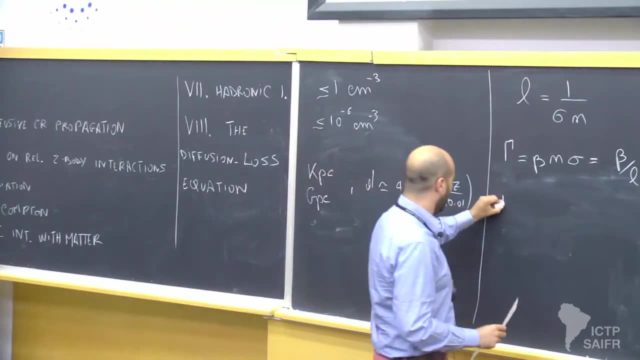 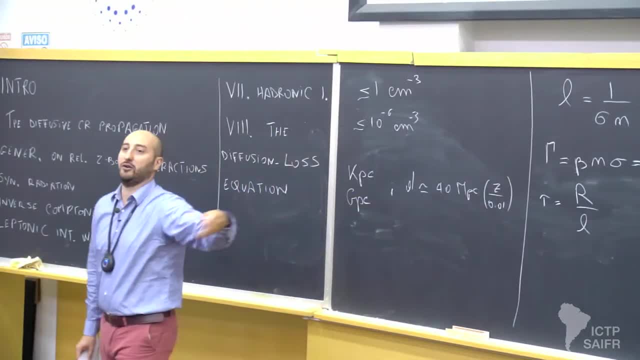 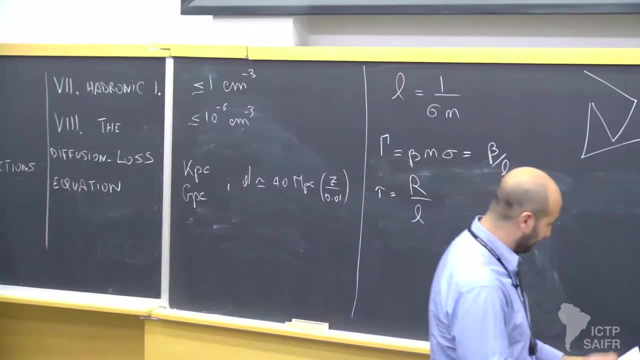 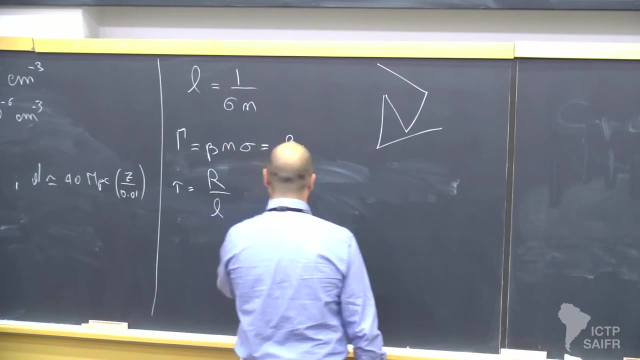 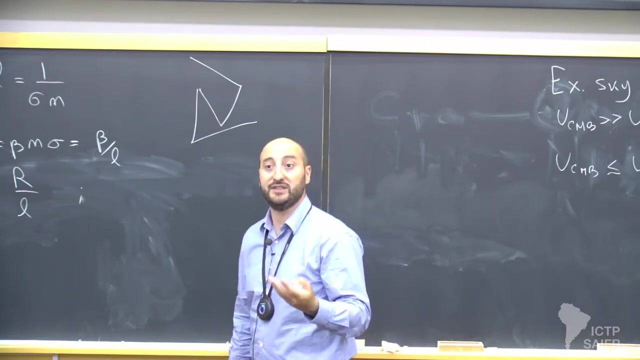 and this has to do with how many times your photon will interact in your region before escaping. okay, So we can quickly estimate what this value is. If we have the typical distance, the average distance that your photon will travel is easily seen to be zero. okay. 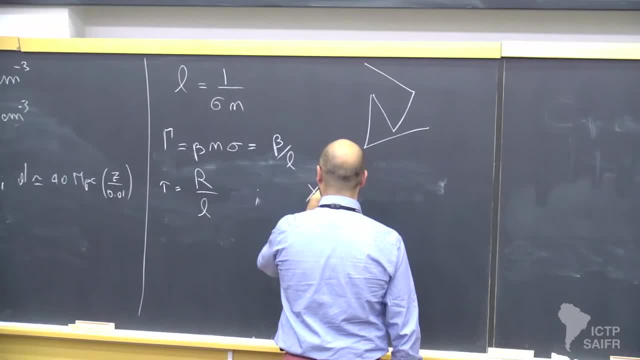 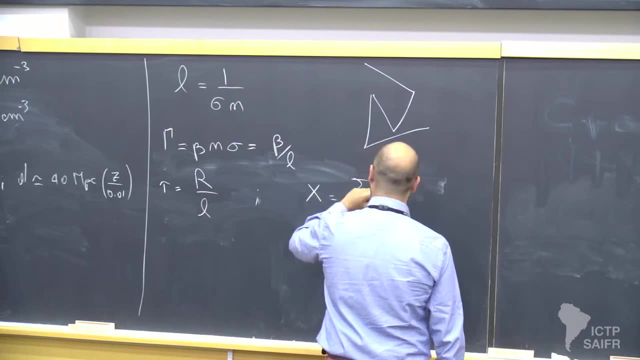 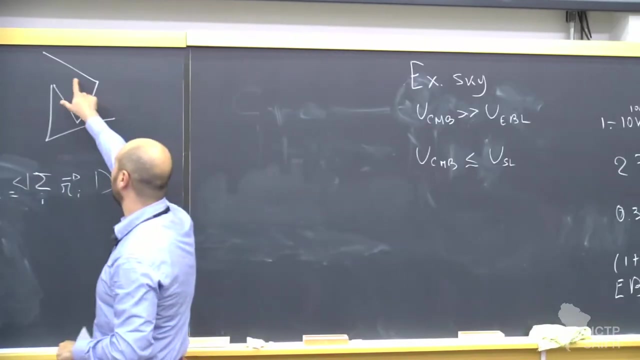 So the distance that your photon is traveling is basically the average. So it's the sum of all these vectors, The average of this thing. But you see that if I assume that the directions are random, well, basically what I'm summing over, 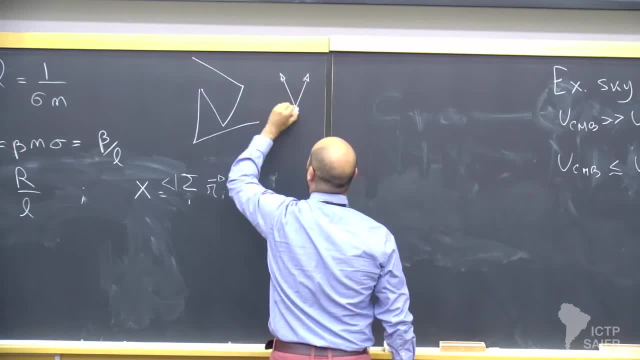 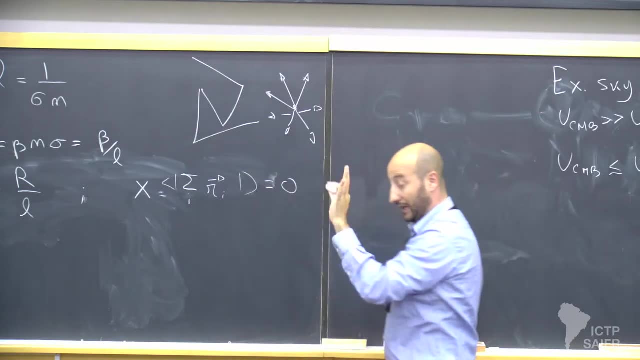 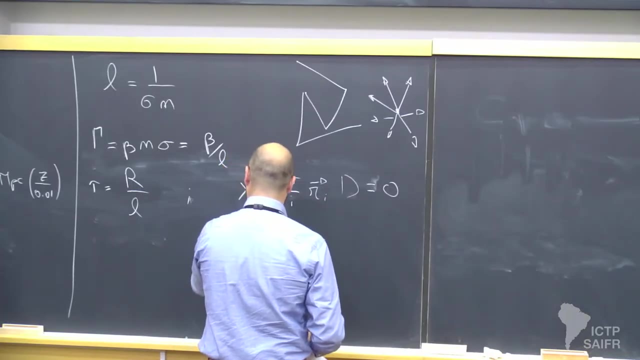 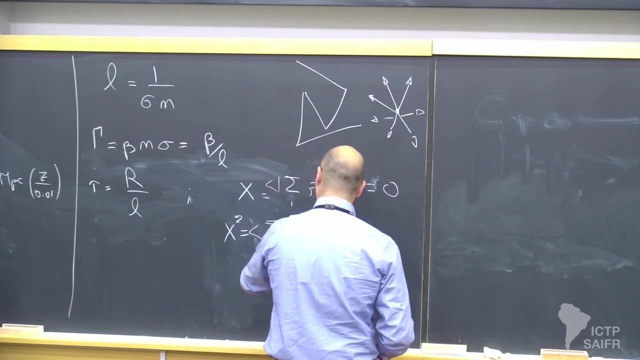 is something which is randomly directing. okay, On average these are randomly directed, so this is zero. So, on average, This is not true for the variance This is. I hope you are more or less familiar with these notions, but if not, 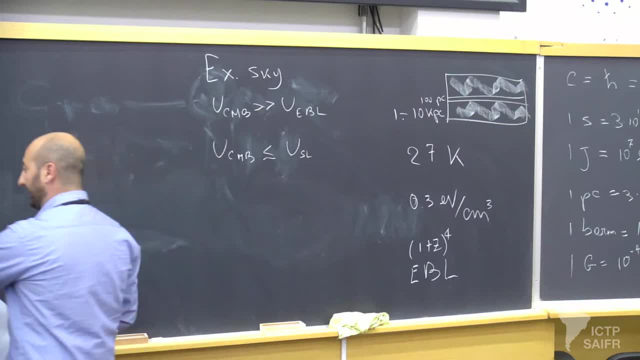 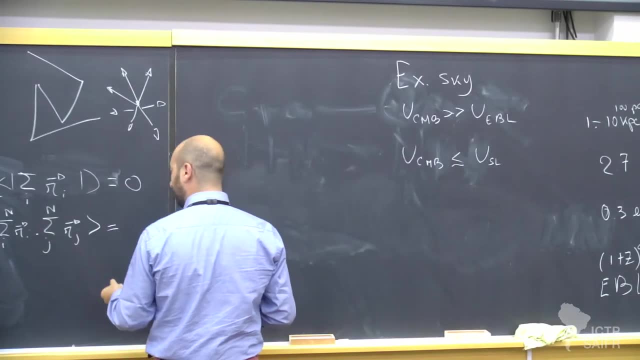 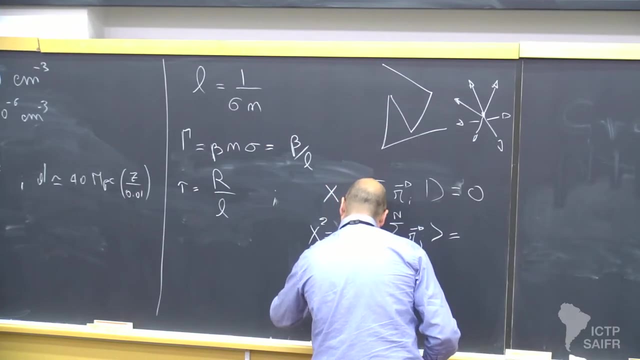 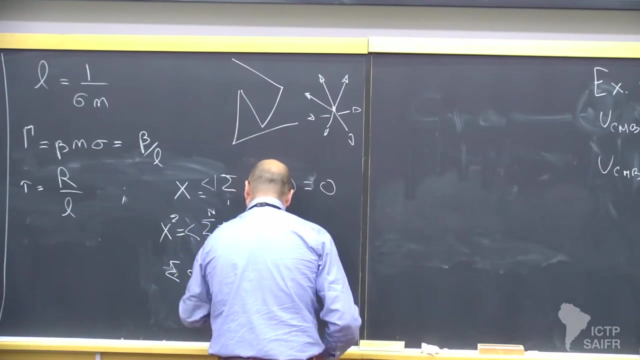 that's a good time to introduce them. If I sum this so, after n steps, the variance will be given and I can split this sum into a sum of r? i square plus something which is l square times. basically, i j of the cosinus of these two angles. 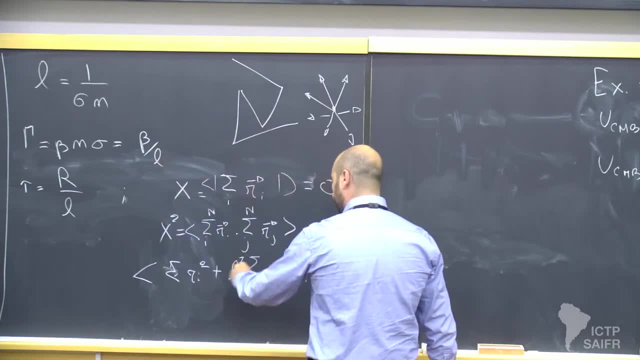 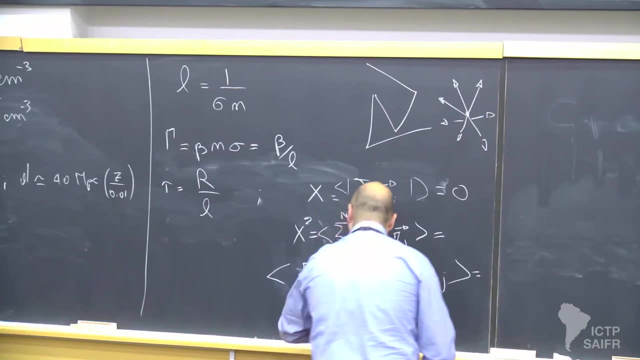 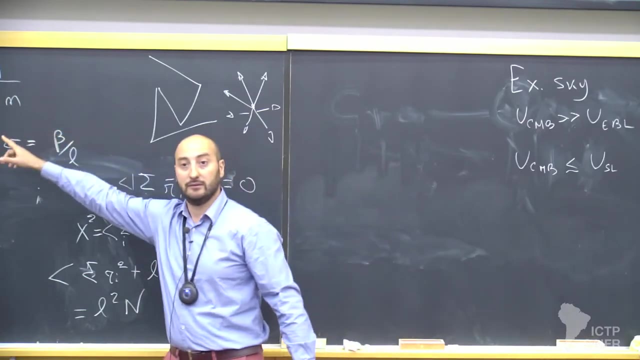 And since this is random, well yeah, So this goes to zero for the same argument as before, but the first term remains, and this is l square times n. Okay, Because now I'm summing over n terms, each one as a typical length of l. 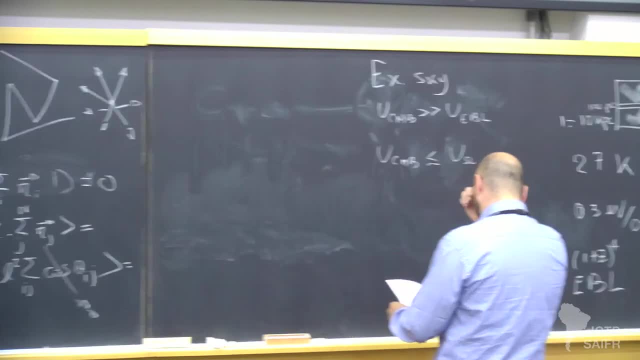 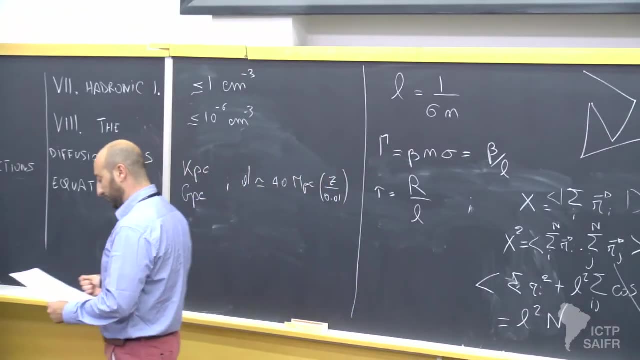 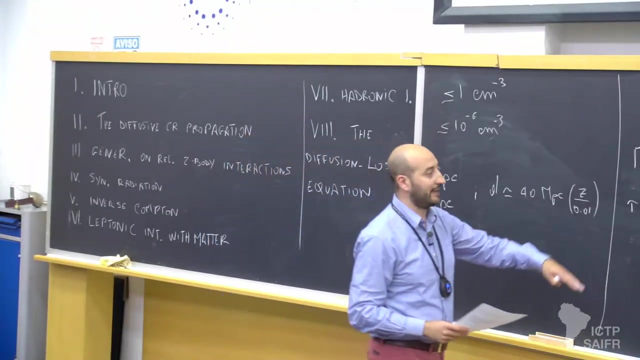 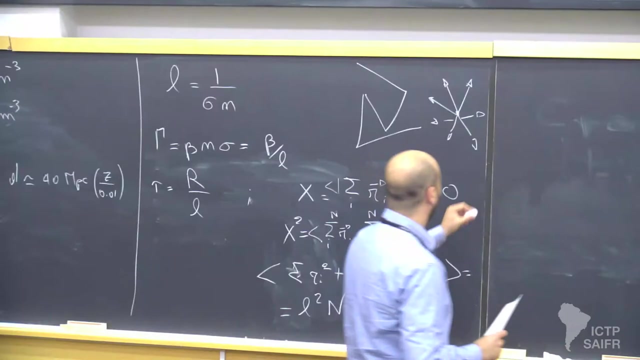 and so this gives me l square times n. So, for instance, you can ask yourself what's the typical time a photon or a generic particle requires to escape my region of optical depth, tau, or of size r. Okay, So you impose that your x square. 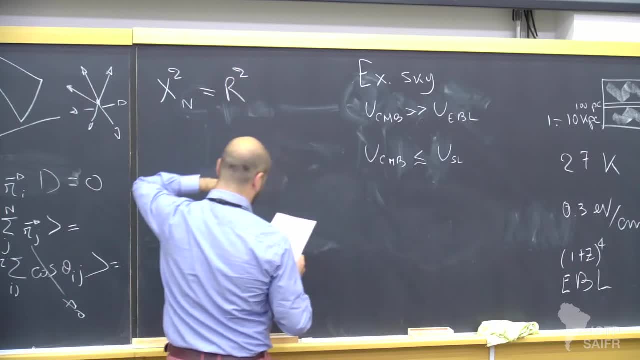 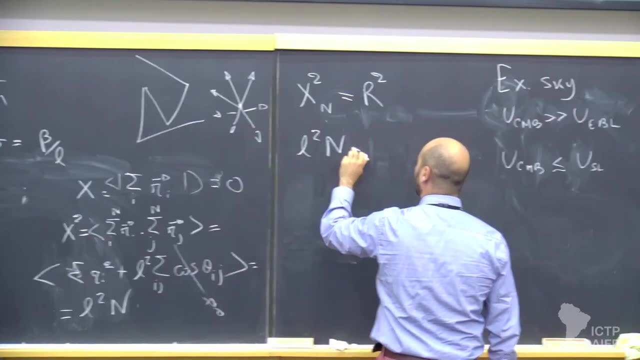 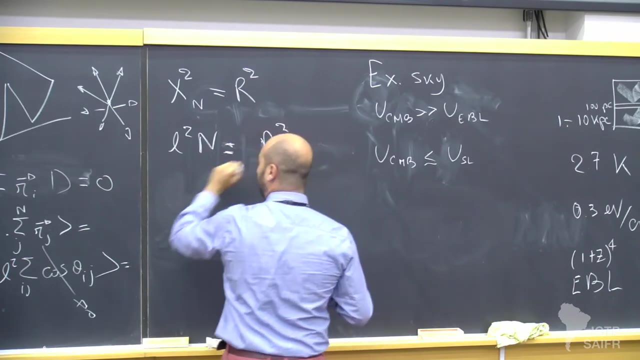 as a function of n, is equal to r square, and this will turn out to be true when l square, n is equal to tau- sorry, to r square, which means that n will be equal to r square, r square, which is tau square. 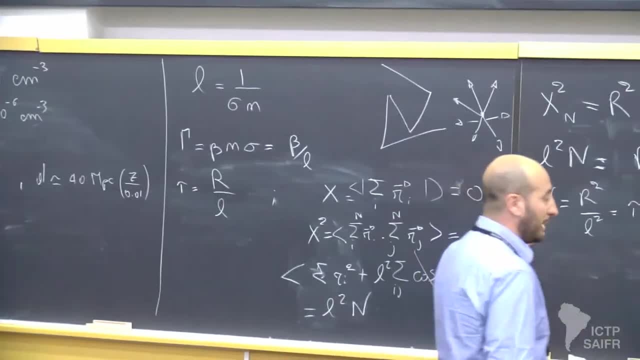 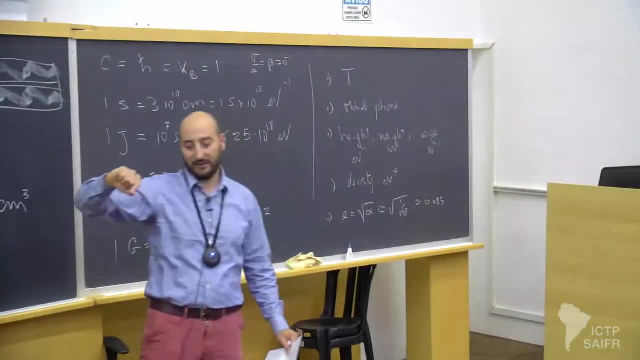 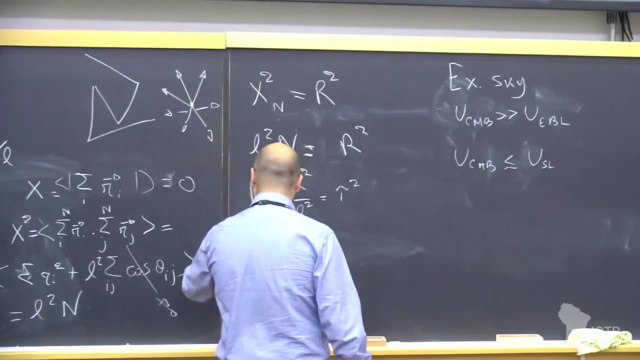 and tau square is equal to r square, n. In general, you can generalize this to any time, so there is a correspondence between n, the number of steps of your trip, and the time elapsed and, in general, the time to escape, for instance. 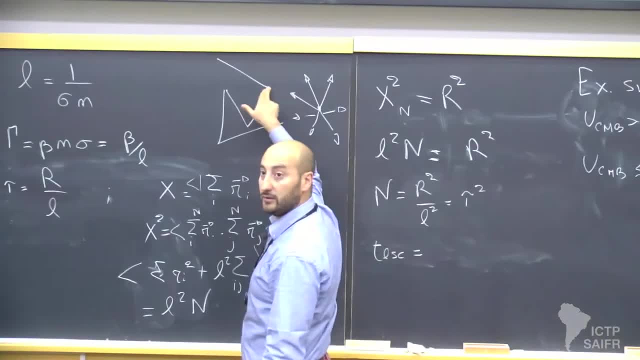 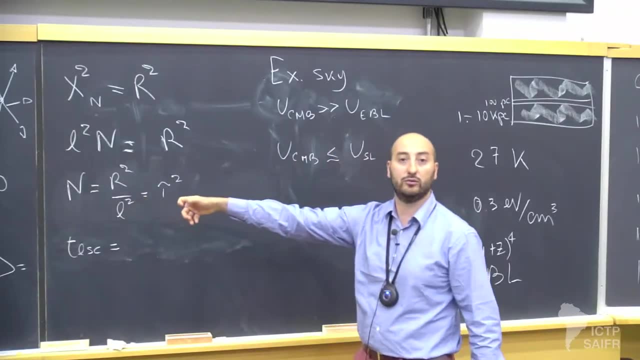 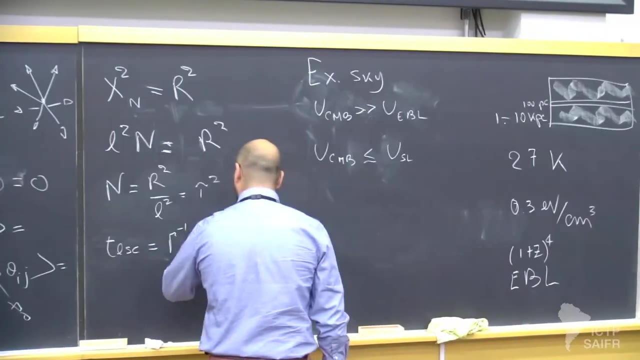 will be given by what? By the typical time it takes for a particle to do one segment, which is the inverse of these, by definition, the number of segments that you need to go before you escape, right. so this will be given by gamma to the minus 1 times n. this is n is tau squared, so it's R. 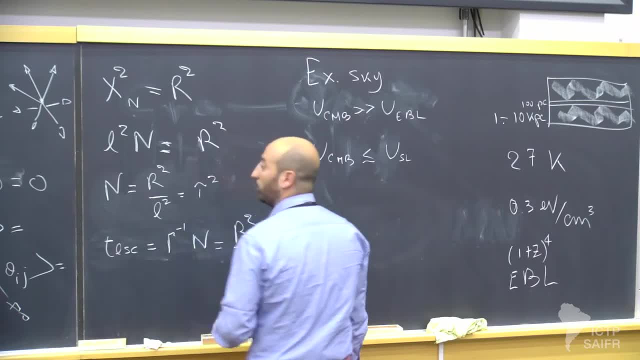 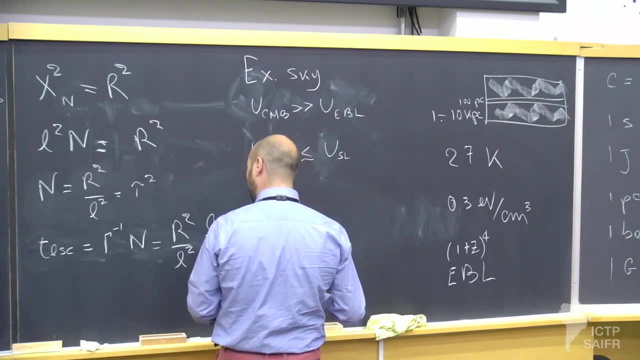 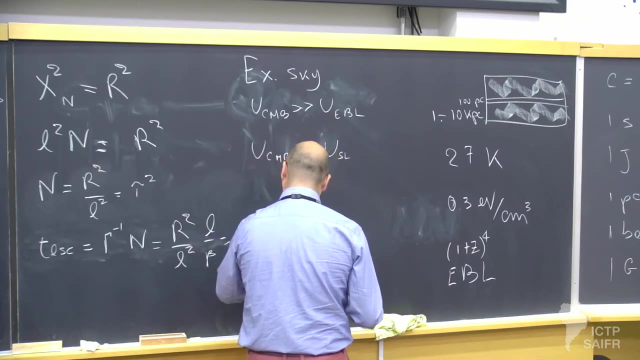 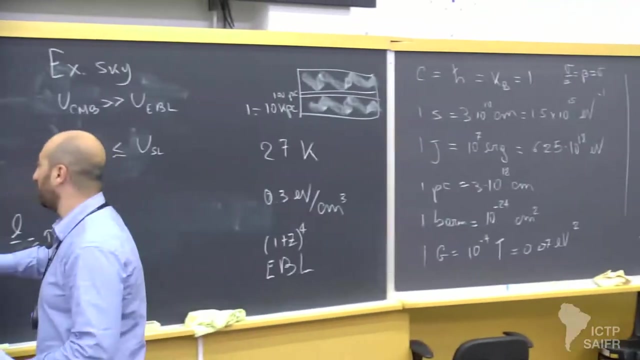 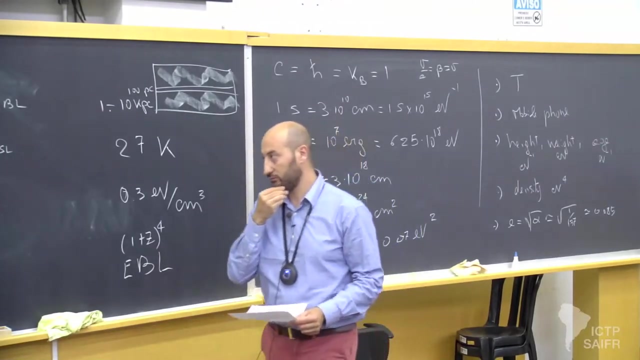 square L. square 1 over gamma is L times beta. okay, so this gives you tau times R divided by beta. okay, the kind of propagation that we have here is a discrete version of what we call a diffusive motion. okay, so you can think of it like this: time scale 1 over gamma to be the your unit. 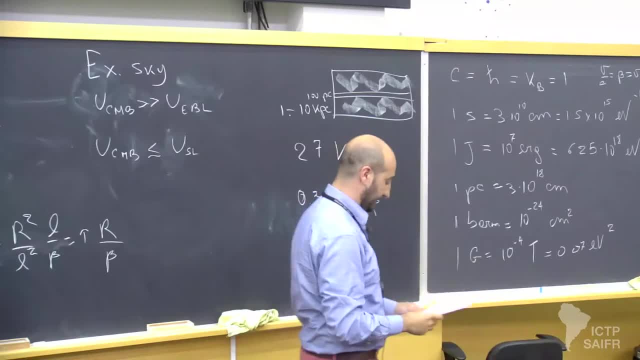 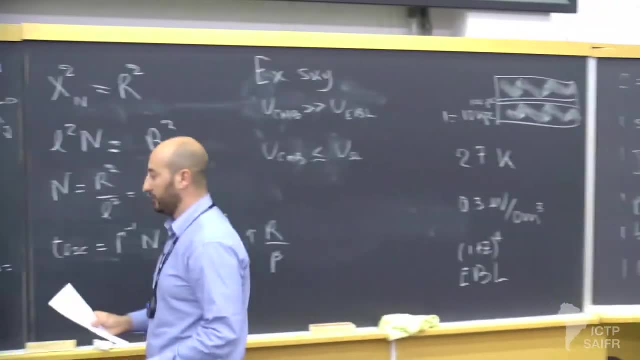 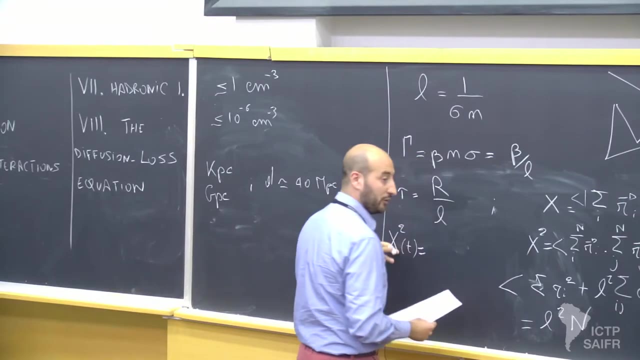 of time, but it can be generalized to a, to an arbitrary time and, in general, consistent with this expression. you will have a typical variance as a function of time, which is nothing, but it's the same formula just written for a generic time and not a function of time. 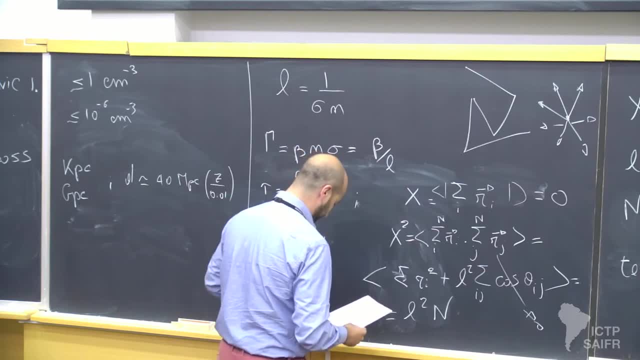 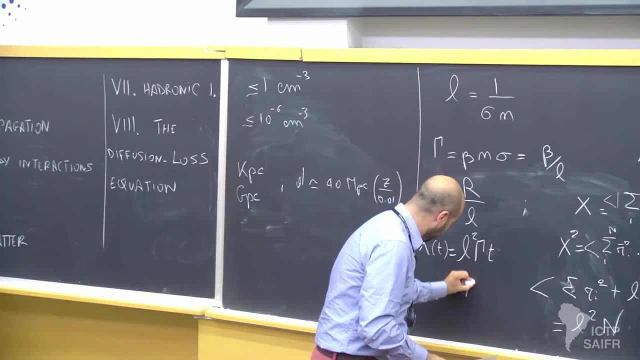 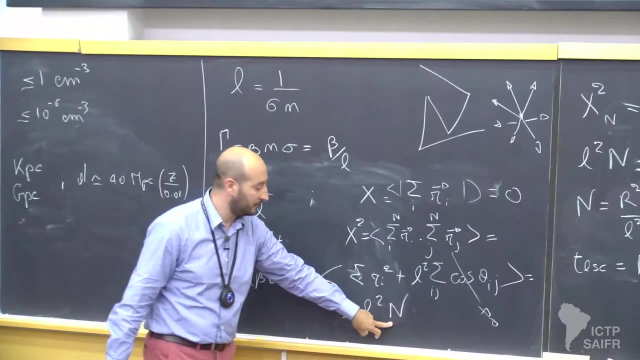 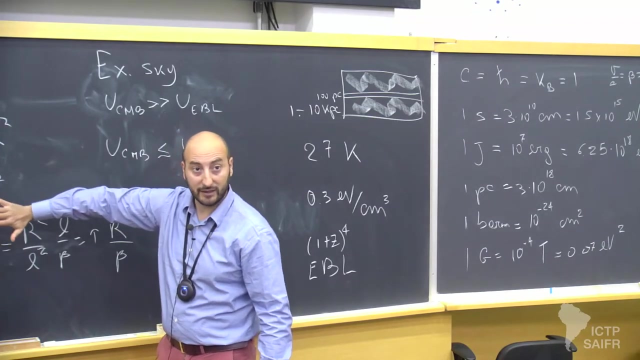 for the escape time, gamma t, which is also equal to L, beta t. t is nothing. now I'm replacing the n coming from here with from here t times, gamma, nothing but that. so this is the escape time. if I replace with this generically for any other t. 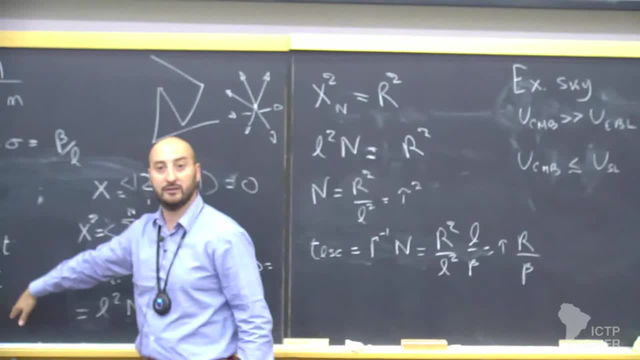 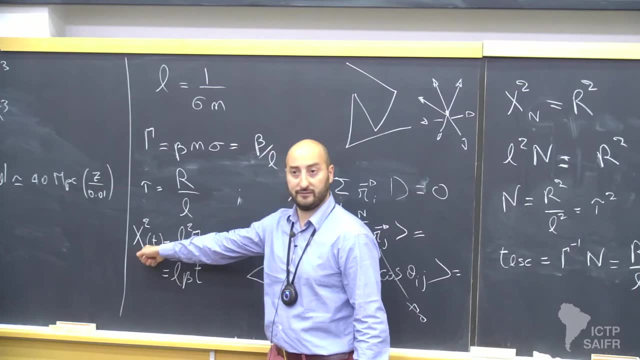 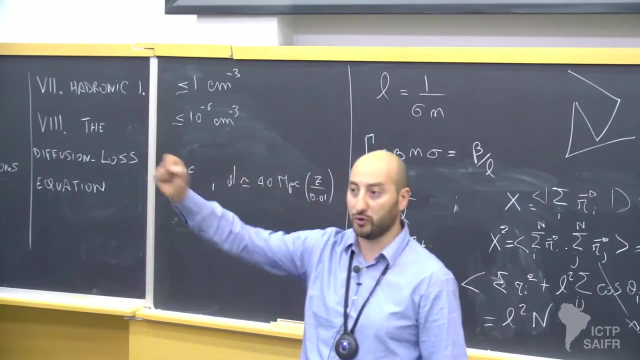 lower than the escape time. this will give me this expression. ok, the only thing that you should retain from this is that the variants of the distance that your particle has traveled is linear in time. okay, this is very different from a ballistic motion, where the distance is proportional to time. x. 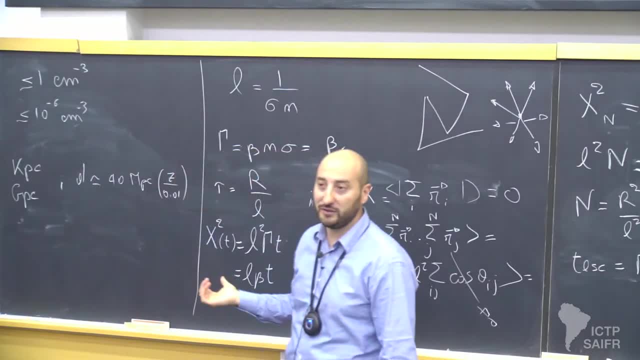 equals V times t in a diffusive motion. in a natural response we could take distance for a number of times per second and the distance equal to the term at equal to time last. before we make this expression okay, the linear expression is: is very different from ballistic motion, where the distance is proportional to time. x equals d times t in a diffusive motion. 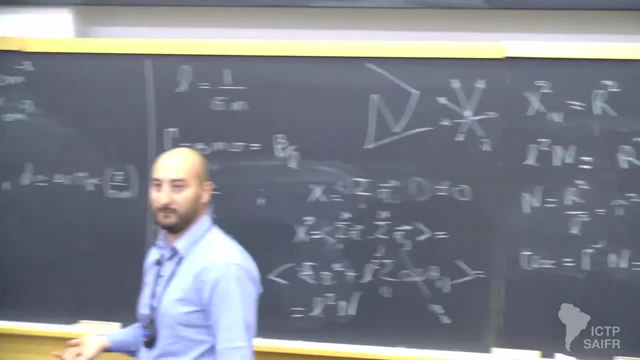 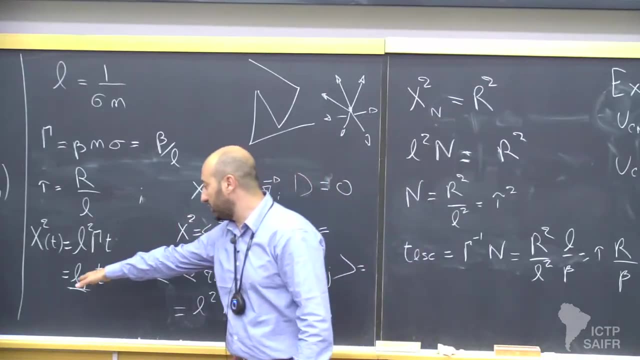 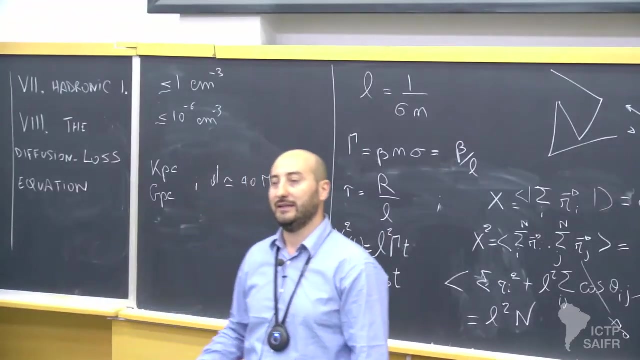 motion. the square of the distance is linear in time. This proportionality constant here, which is dimensionally the mean free path, times the velocity. this is related to the diffusion coefficient. It's actually the diffusion coefficient, apart for a numerical constant, that 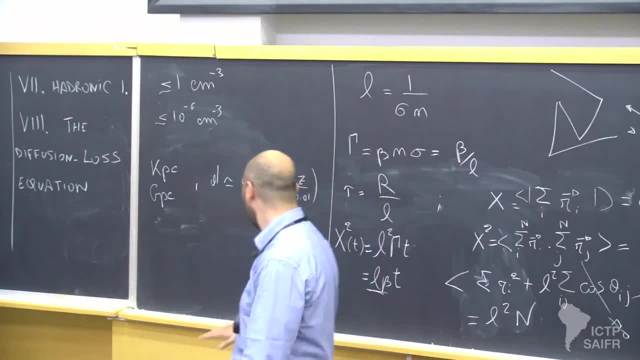 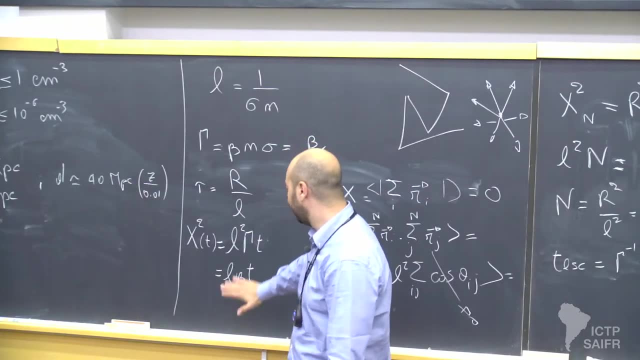 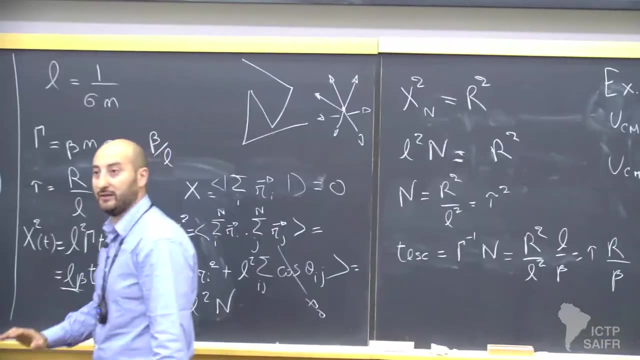 depends also on the dimensionality of the space over which you are. We will see a more exact version and correspondence to the cosmic ray movement later on, But for the moment, keep in mind this picture, OK, If you are diffusing back home after a long night. 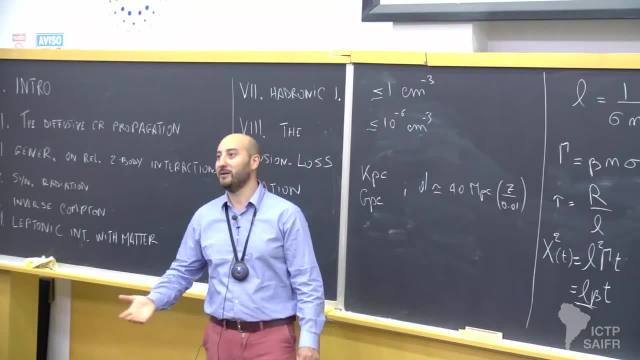 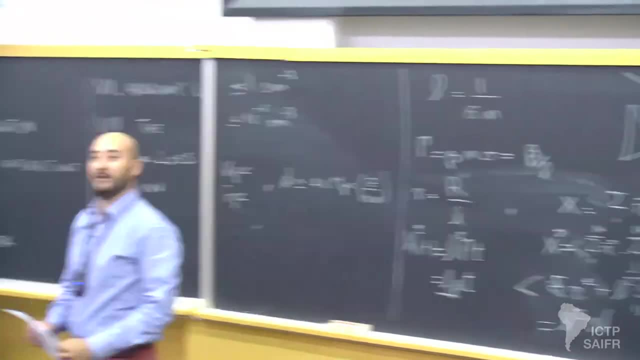 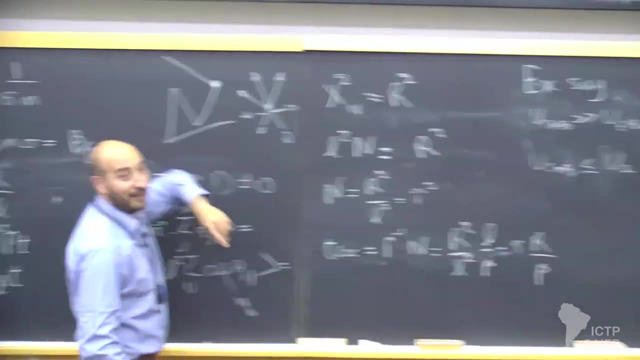 you have been drinking a lot. Well, now, probably you call an Uber and that's it. But if you walk back home, that's the kind of movement that you will experience. OK, And probably you can think of it like: these are traffic lights. 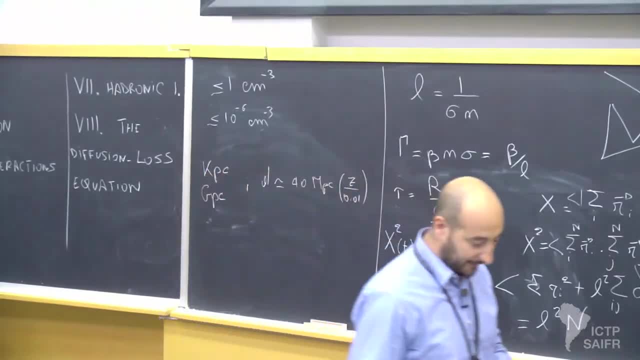 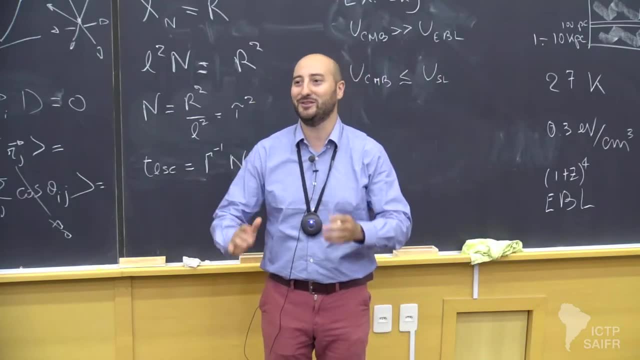 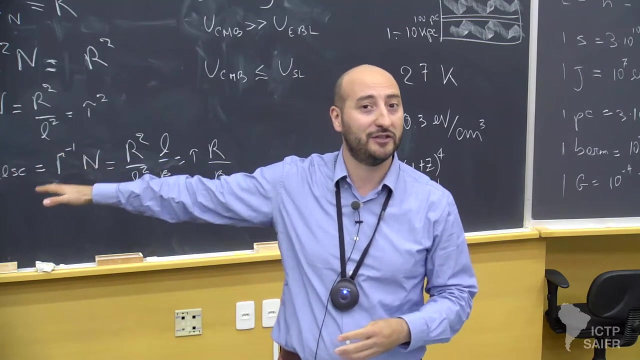 or poles Or Or buildings. Very good, So any problem till now. I hope most of you are familiar with these notions, But if not, it was a good moment to introduce them because we will find these features in a more realistic treatment of the way cosmic rays propagate. 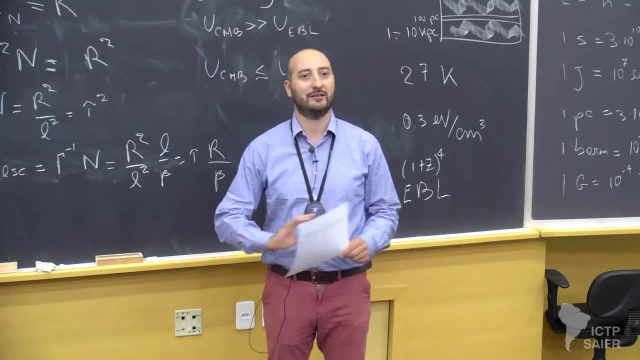 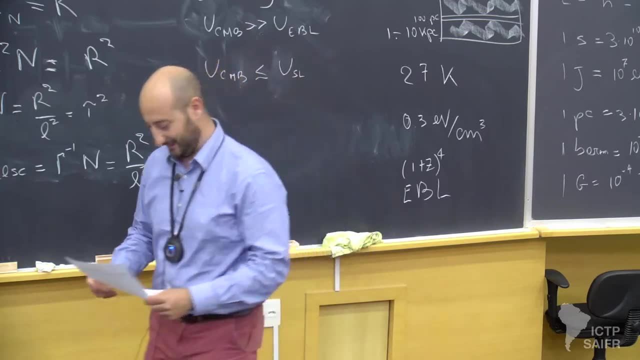 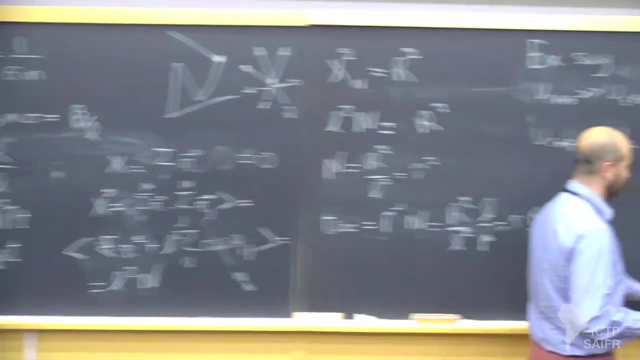 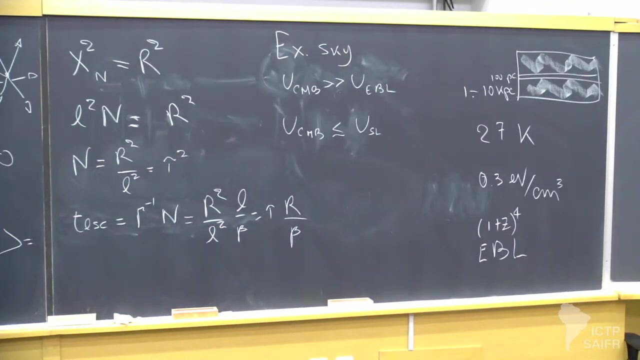 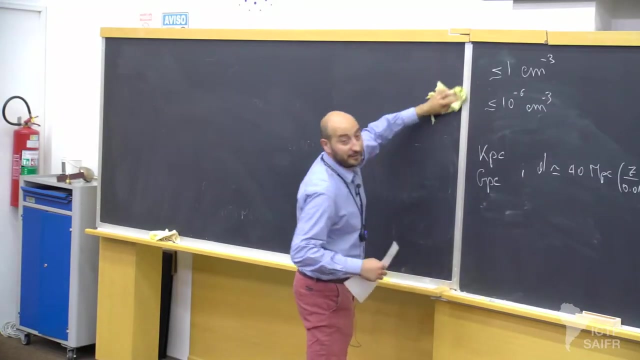 Are there quick questions on things like that that are completely above your head? OK, I don't see any lost people, So I will erase something. For sure I can erase the sketch of the lectures. So imagine you have a tree, You have a charged particle and a constant magnetic field. 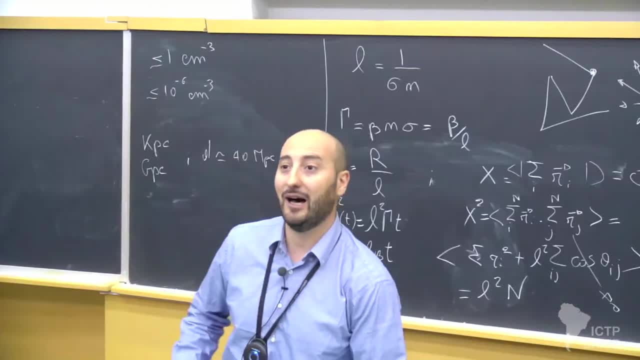 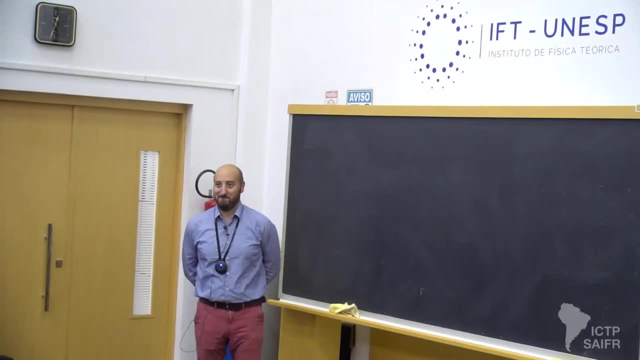 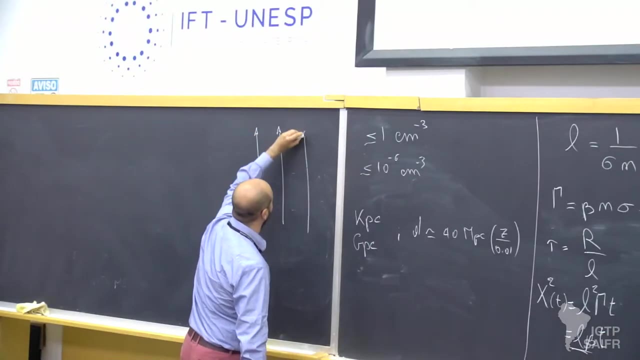 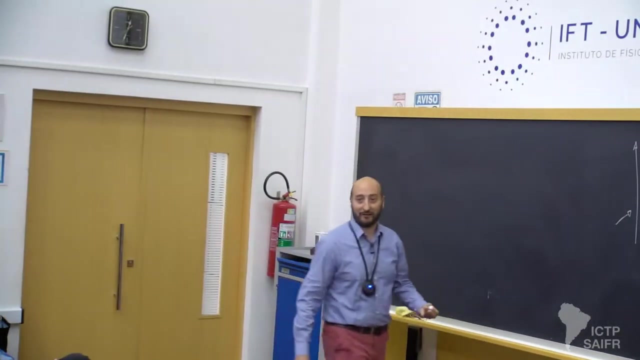 I throw this particle into the magnetic field. How this particle moves. What's the trajectory of this particle? I have a constant field And I throw a particle into it. What will happen? OK, it's spiraling. OK, So you have seen that right. 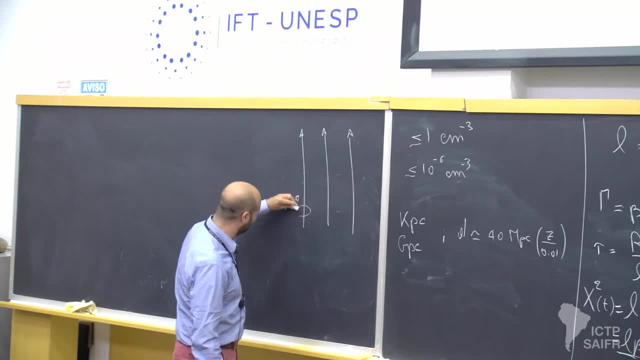 So if I throw it perpendicular to the field, this will just move on a circle. If I throw it with a component which is parallel to the field, this will evolve on a spiral. OK, So this is still valid in a relativistic context. 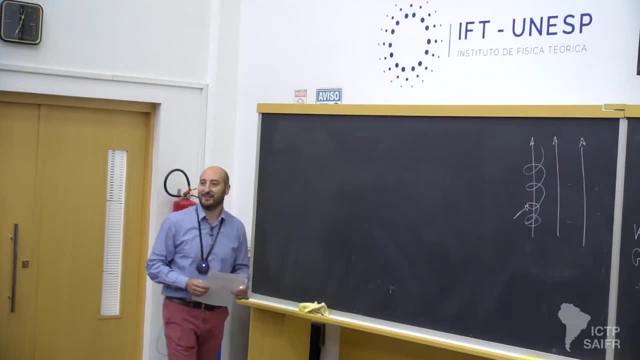 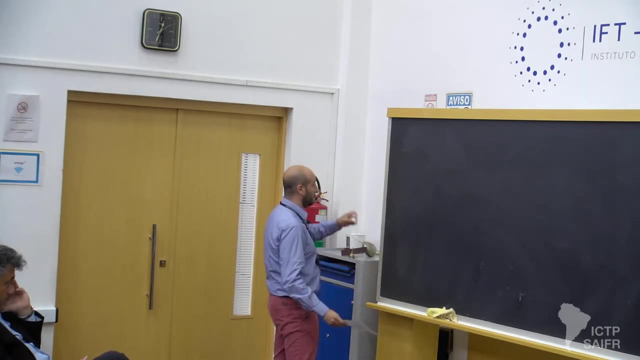 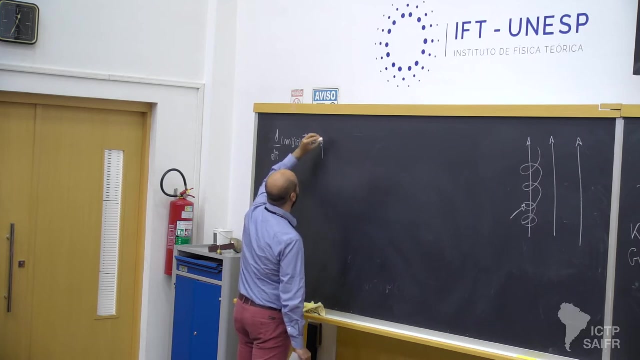 Probably you have seen these in classical mechanics and electromagnetism, But this is still valid in a relativistic context. The only difference is that the equation of motion gets some gamma factor in it, So mass times gamma is going to be equal. qv cross b0. 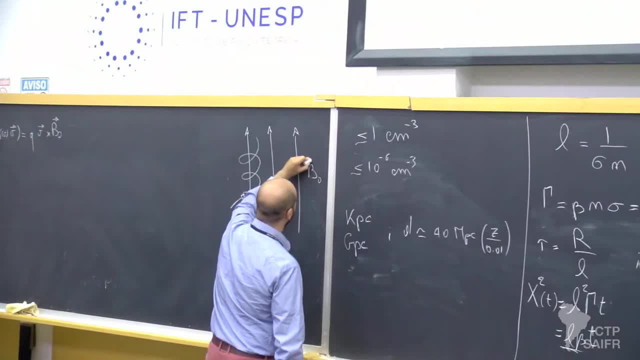 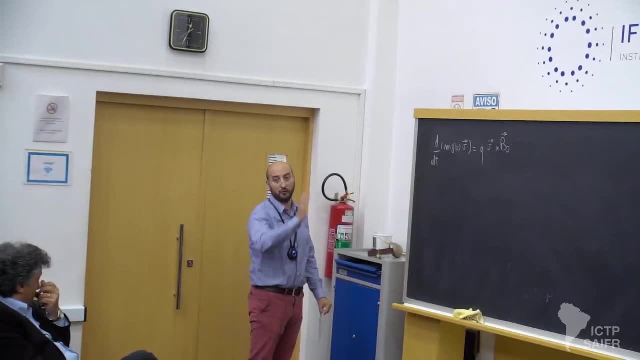 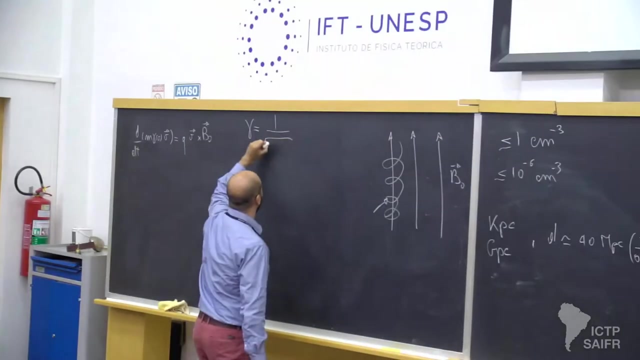 b0 is my field, This homogeneous field, and OK, whose direction in the field? This is my field. OK, This direction in the following will assume to be the z direction, by the way. So the gamma here is the usual 1 over square root of 1. 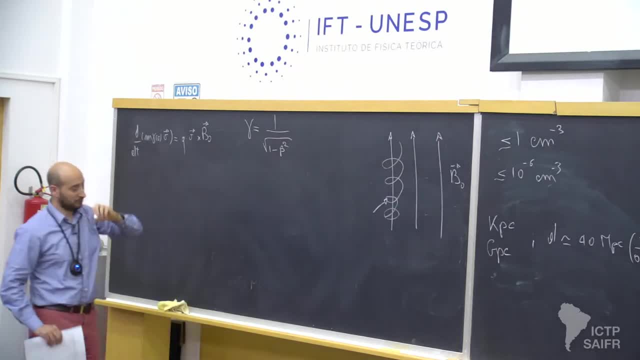 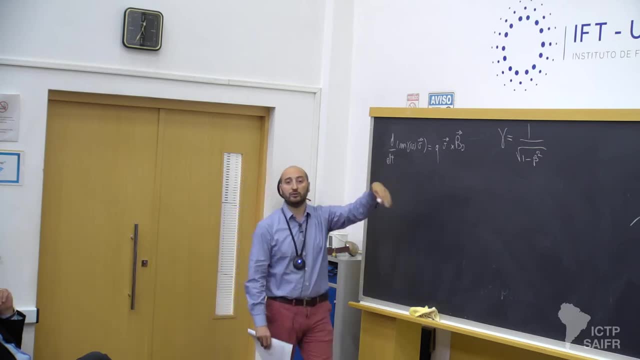 minus beta square. OK, And actually, since the acceleration is orthogonal to the velocity, it means that the modulus of velocity is preserved. This is exactly like in non-relativistic physics, So I can bring this out. If you are not convinced, OK there. 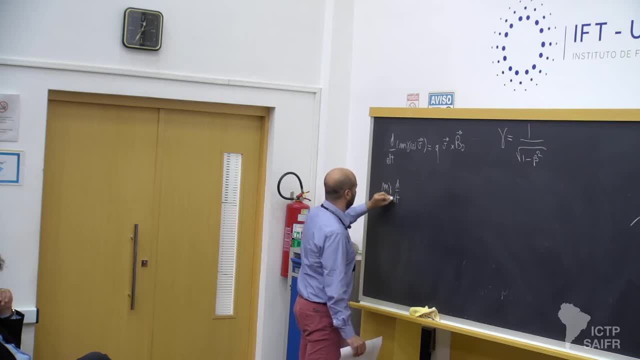 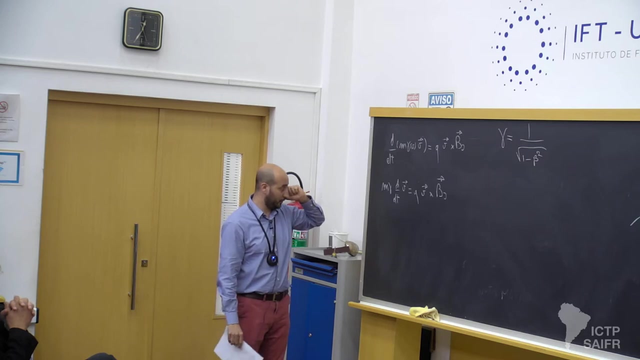 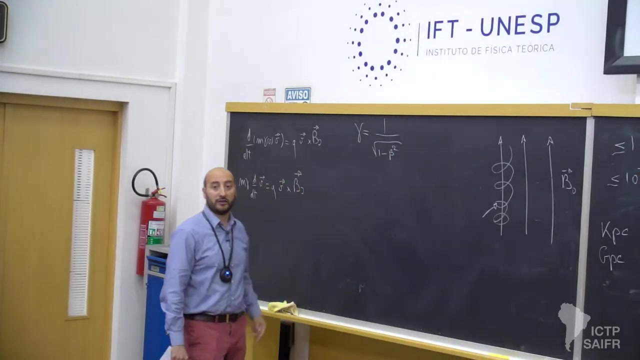 is a little exercise proposed that can prove this to you. OK, And immediately from this you can take the projection of this on the axis of the magnetic field, the projection along z direction. This will be 0, because this vector is orthogonal to both the velocity. 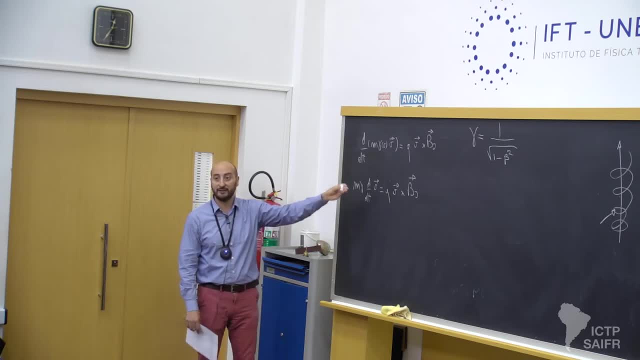 and the magnetic field. So if I take the projection on z, this is 0.. The right-hand side is 0, which means that the derivative of vz is 0.. vz is a constant, So vz is constant, which also means that pz is constant. 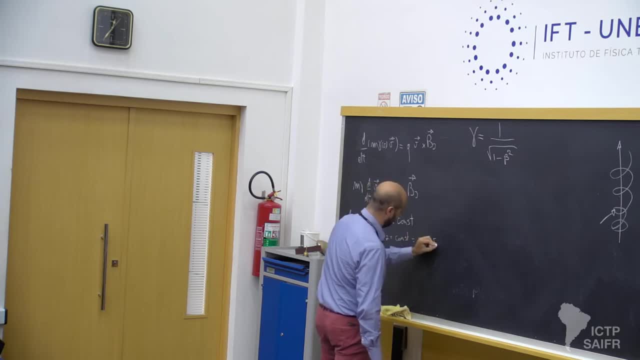 This is nothing but m gamma vz. OK, OK, So m gamma vz, And also the pz over p, which is called mu or pitch angle, is also a constant. To be more correct, this is the cosinus of the pitch angle. 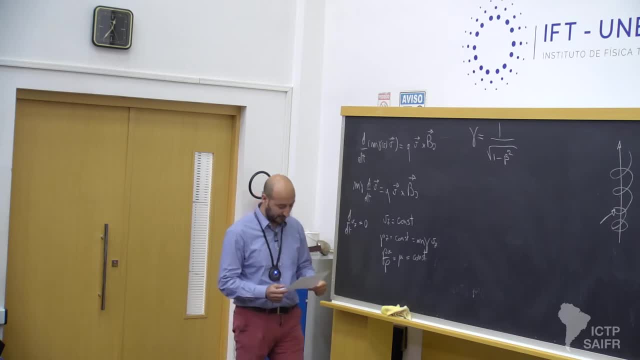 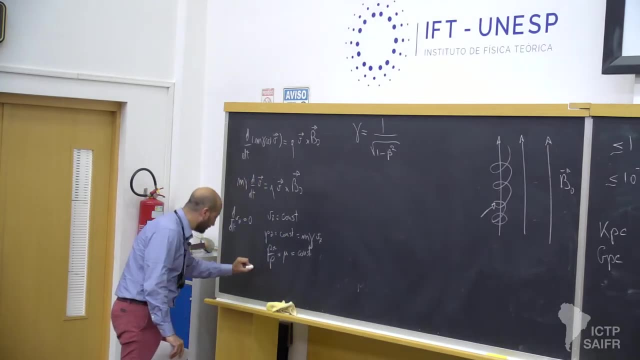 But yeah, that's also constant. OK, We will use this in the following. Of course the momentum by this condition also the momentum p orthogonal, which is the square. So this is the square root of p square, minus the z component. 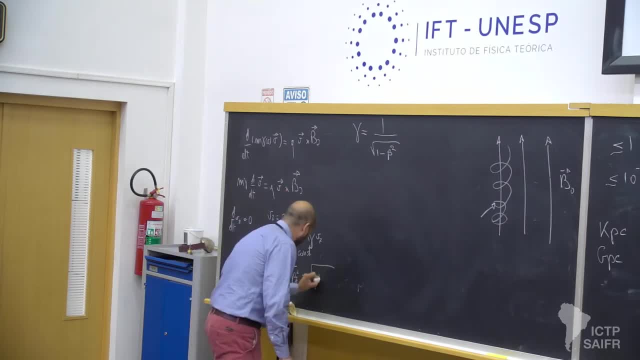 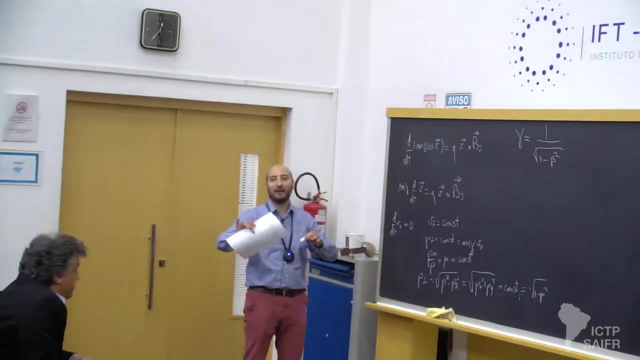 square. If you wish. this is the square root of px square plus py square. This is also a constant And this is equal to square root of 1 minus mu square. You will see this type of 1 minus mu square, et cetera. 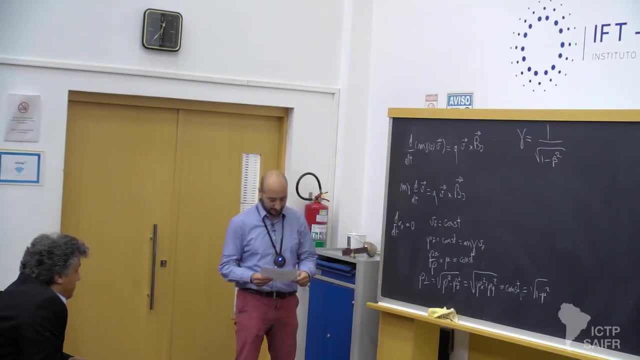 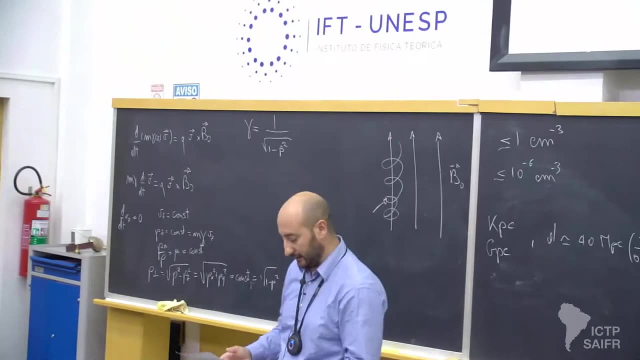 appearing again and again. This is nothing but a geometric projection factor. OK, And that's it, Thank you. And as you described in words, the motion is quite trivial. So the motion in the z direction. we have the equation of motion here. 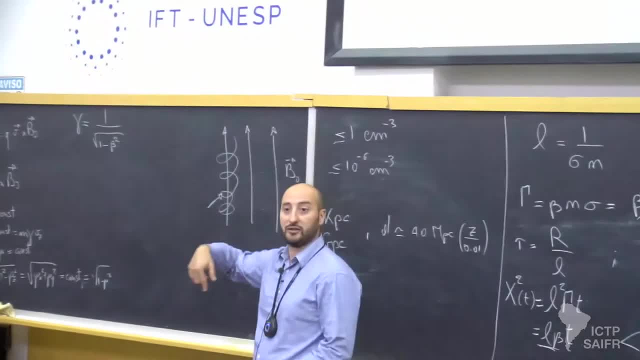 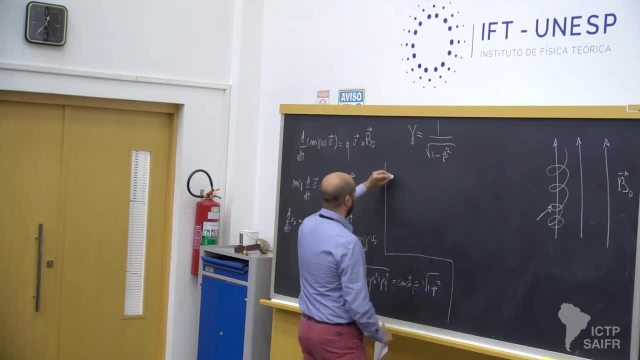 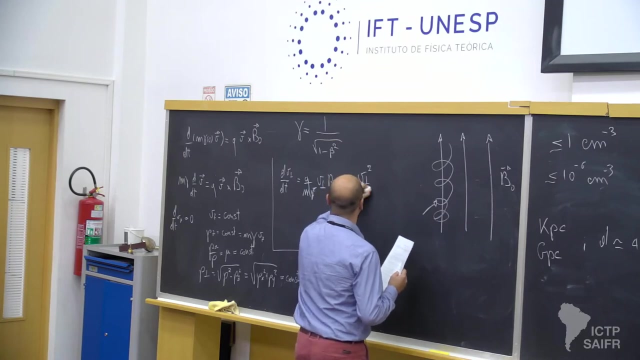 It's just constant velocity And the motion in the xy direction is a circular motion. So we have that dv gamma. This is the orthogonal projection. So xy is q over m gamma. sorry, v orthogonal b0.. And this is also equal to v orthogonal square over r. 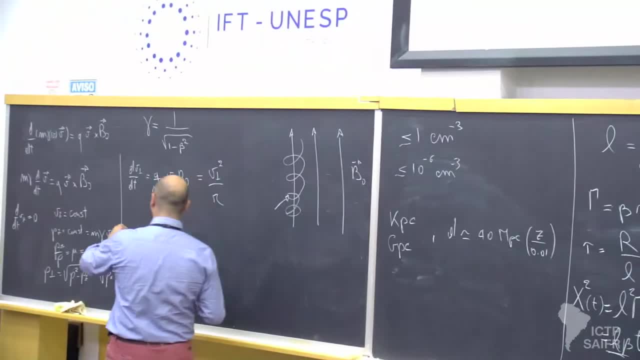 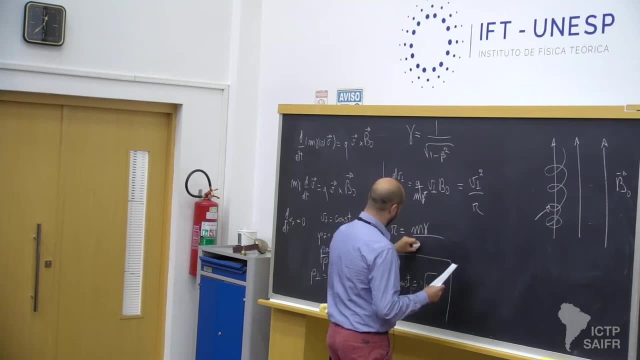 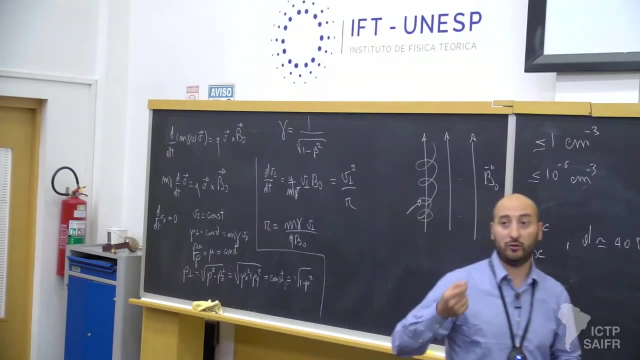 This is a centripetal acceleration. So from this we derive the r, which is m gamma over q, b0 times v, orthogonal. This is exactly the same expression, The expression that you have derived for the so-called gyroradius of a particle spiraling. 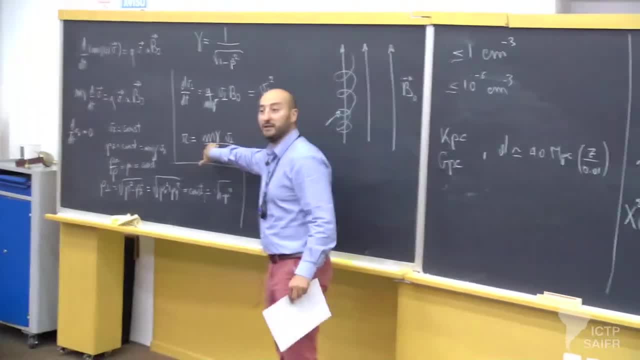 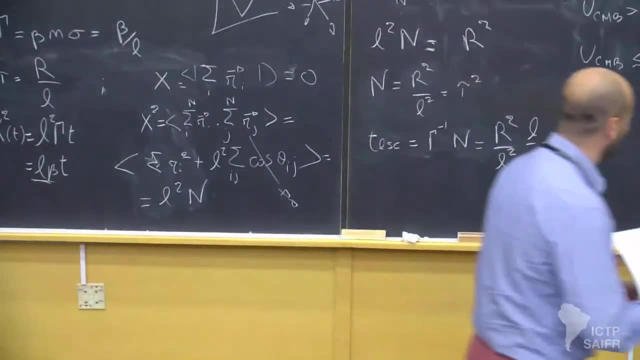 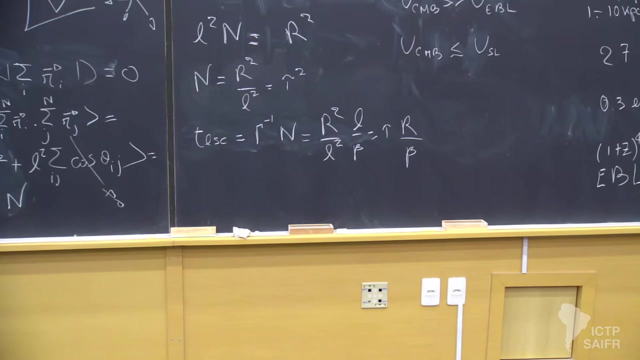 in a magnetic field, apart for this factor gamma that appears in the relativistic context. OK, So since these are important quantities, I will put them here. Why they are important? Because they will set some scales which are extremely useful for our problem. 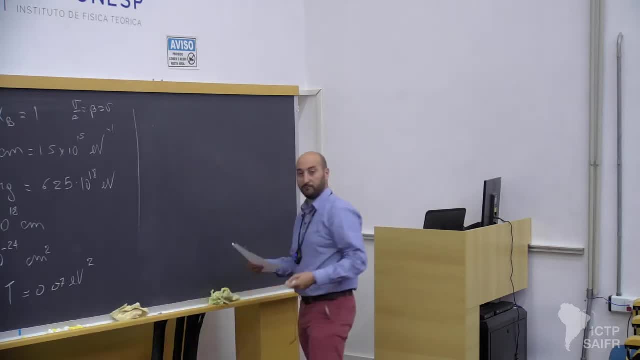 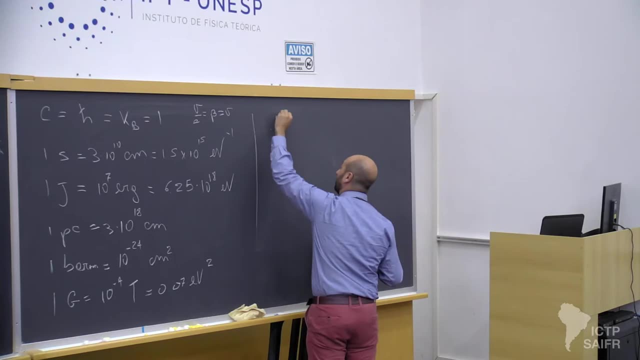 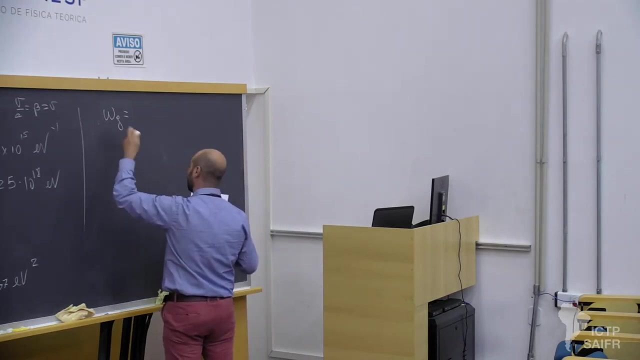 OK, Thank you. So you are familiar, I hope, with the non-relativistic counterpart of this problem, And this problem is described by the inverse of the period of rotation, omega g gyration. That's what the suffix stands for, which is q, b0 over m. 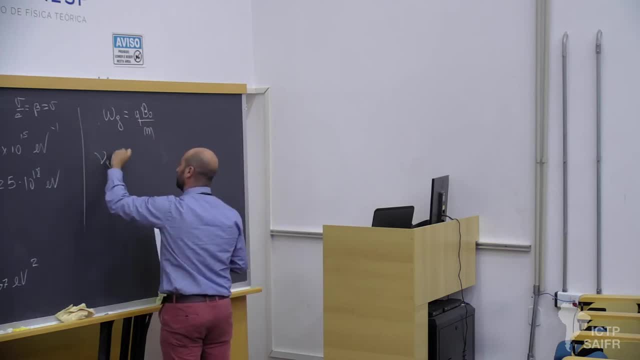 Associated to this there is a frequency, nu g, which is- oh, this is omega g over 2 pi. And this frequency for your reference- OK, of course, this is q b0 over 2 pi m And this frequency in useful units. 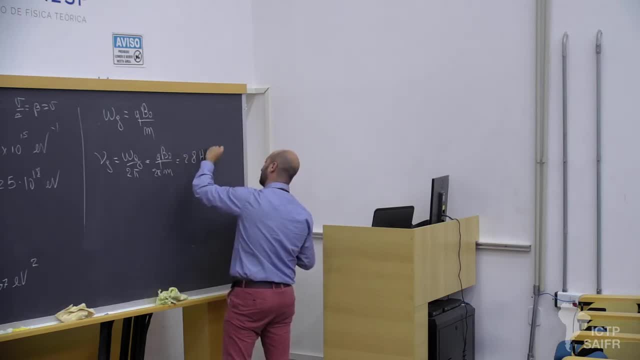 is going to be 2.8 hertz times, the. if I write the charge of your particle as z times e times, z times m, e, over m And the field And the field And the field In micro Gauss, OK, 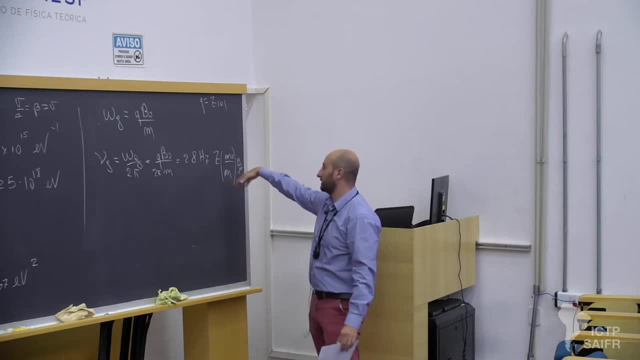 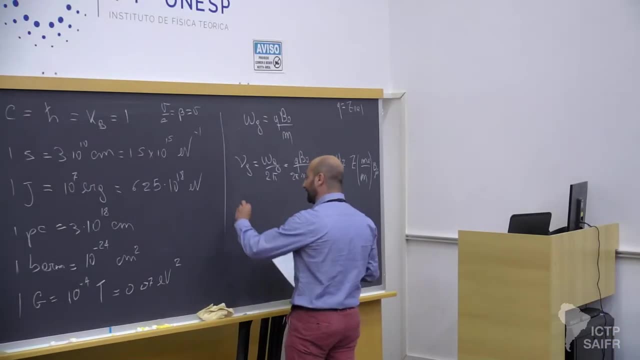 So you see that this is quite low frequency for a particle, which is say the mass of the electron and in a field of micro Gauss strength. And then there is the gyro radius, which is just v, orthogonal over omega g. OK, And the only difference that you have in the relativistic case. 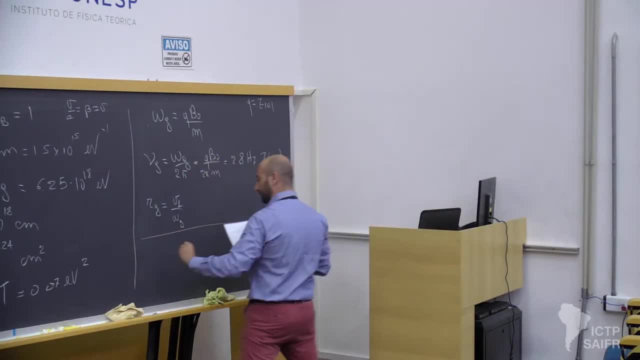 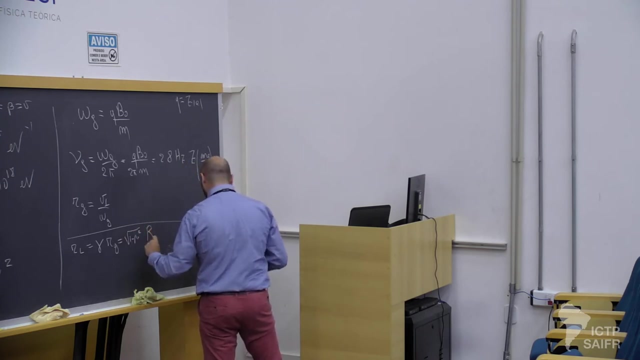 is that now r r l is going to be gamma times r g. And another way to rewrite this is square root of 1 minus mu square times rigidity in over b0.. Rigidity is momentum over charge. OK, And this is 10 to the minus 6, 1 minus mu square. 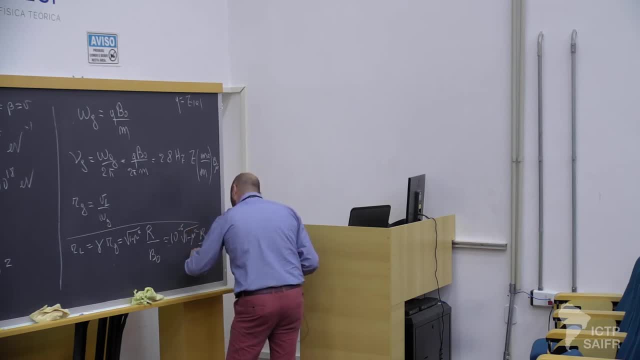 OK, So this is r in gigavolts, 1 over b0.. So this is b0 in micro Gauss parsec. This is exactly the comment Pasquale was doing before. So you see that this is a very, very, very small scale. 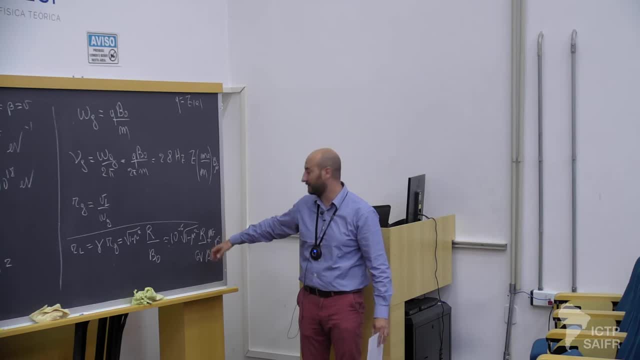 for particles which are gigavolt or even teravolt, et cetera. So basically, compared to the astrophysical scales- the kiloparsec, The megaparsec, et cetera- this is a very small scale. 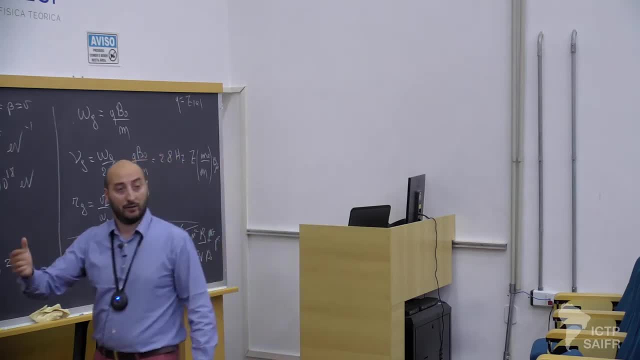 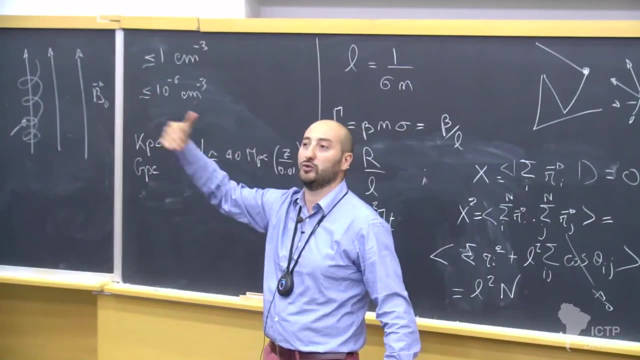 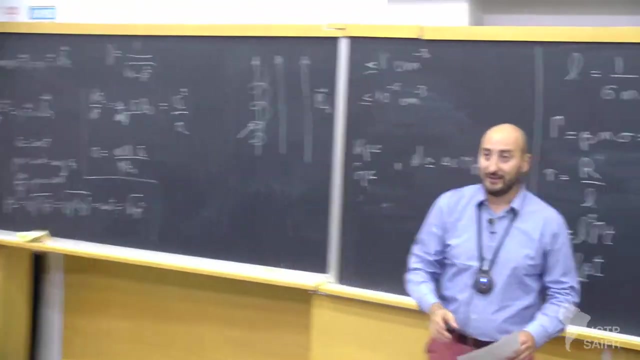 So your particle is gyrating on a scale which is much, much shorter than the typical scale, over which, say, the distance from a typical source to us. OK, So you can think of the particle making many, many orbits. OK, Now, is this always true? One of the exercises that I suggest you to make is to compute at which rigidity or, if you wish, at which energy this starts to be a bad approximation. OK, In particular, which energy? a proton or an iron nucleus will have a gyro radius which is comparable to typical kiloparsec? 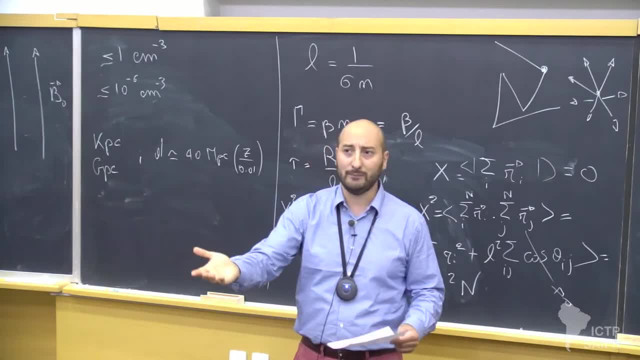 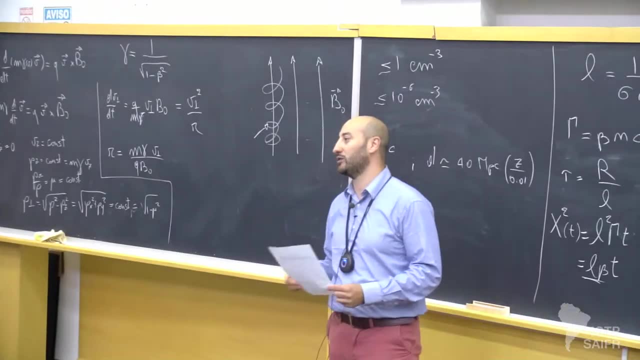 distances in the galaxy. OK, And this is quite important, because one picture that Pasquale was not showing to you is the arrival direction of ultra energy, cosmic rays, And I can tell you that it looks quasi, quasi Isotropic. OK, 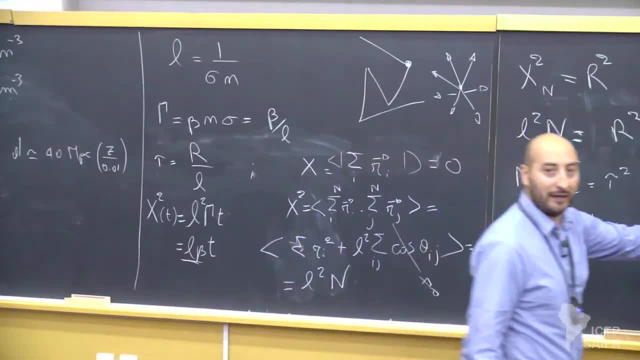 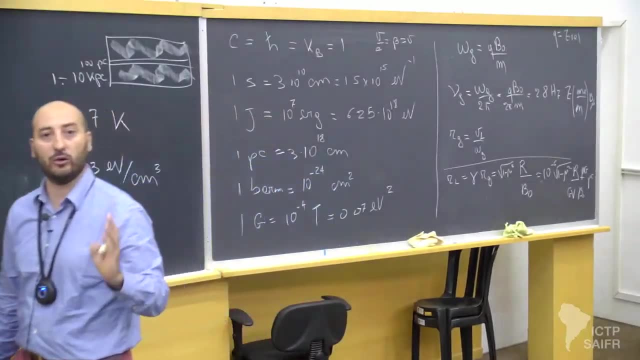 So I invite you to think what this calculation implies once I tell you the scaling and the fact that at 10 to 19 electron volt the sky looks almost isotropic. And you should tell me what you learn about the origin of ultra energy, cosmic rays- from these two. 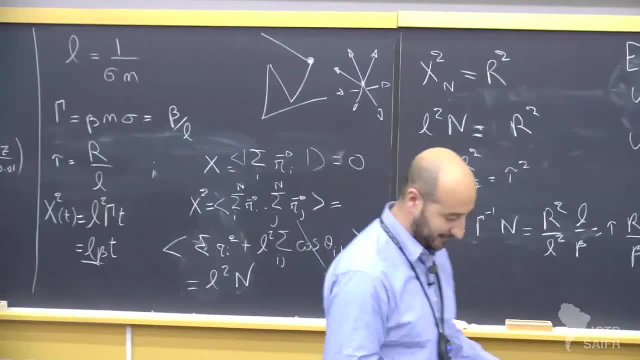 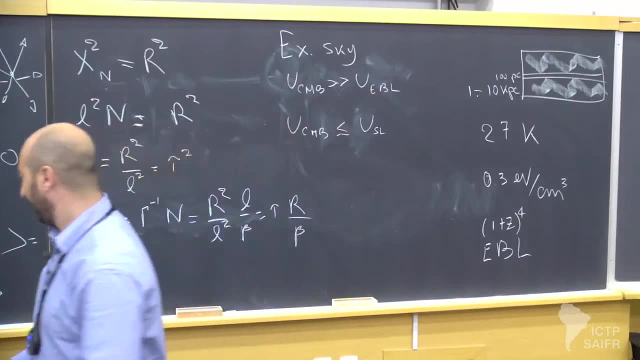 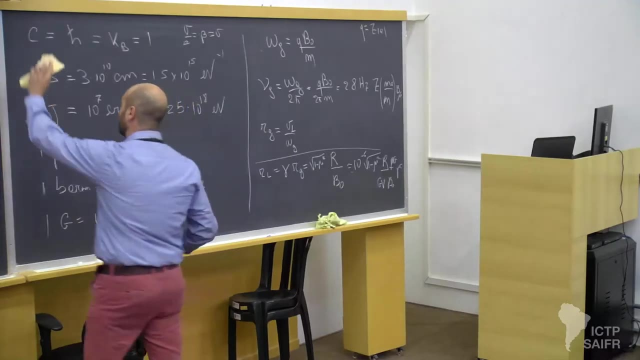 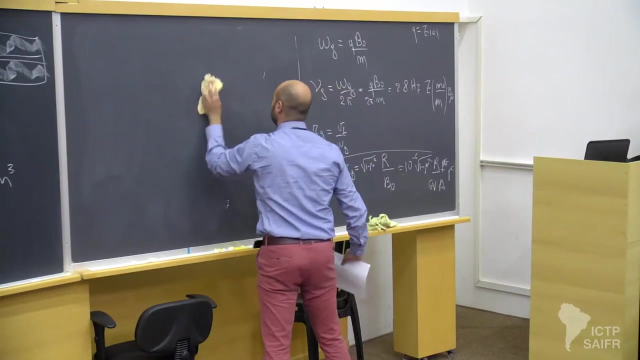 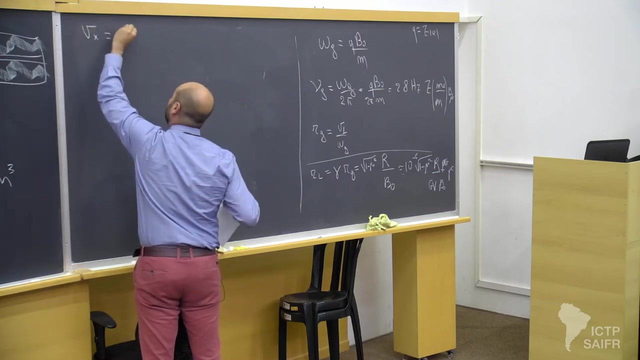 observations. OK, So this is the one exercise I propose. So, after this quite elementary, I think, calculation, we are ready to write down the equation of motion for our particle. We have integrated our problem And the result is vx. is v, gamma, cosine, omega t? 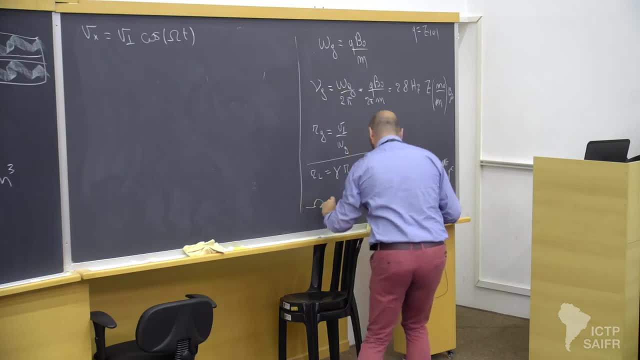 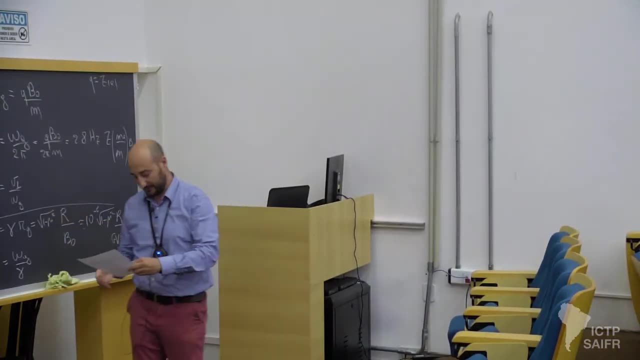 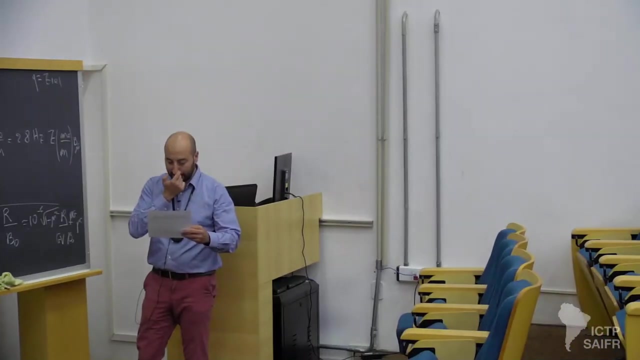 Omega is nothing but omega j. OK, So we have a g over gamma which replaces your gyro frequency in the relativistic concept, And if you do the calculation in numbers, this will turn out to be of the order of, basically, a fraction of a radian per second for a GV particles which 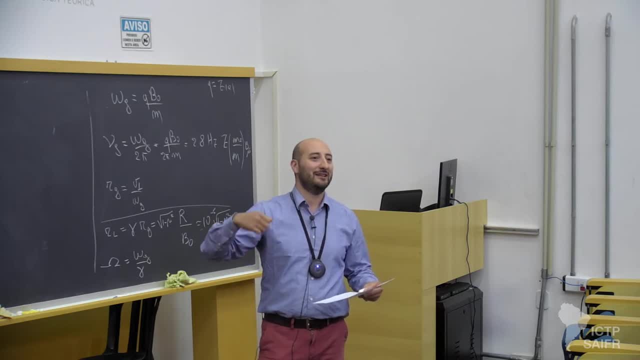 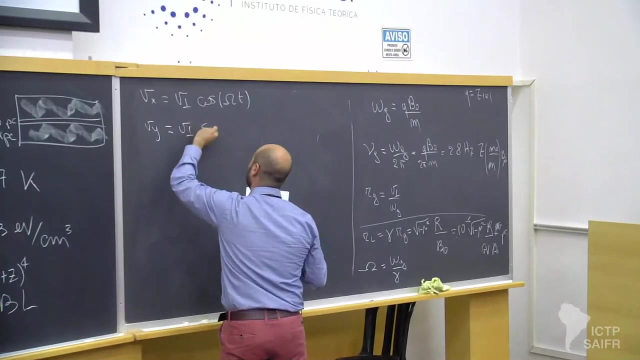 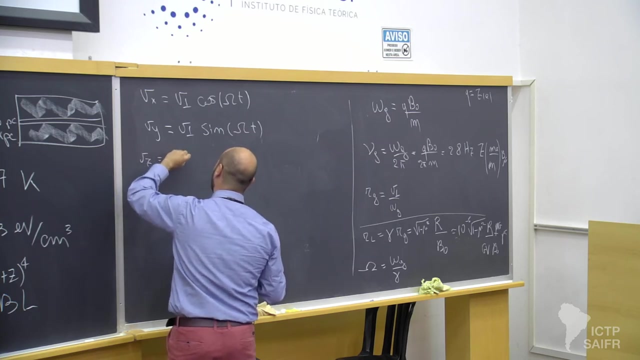 means that your frequency is ridiculously high. Yeah, Your time scale is ridiculously short compared to the time scales of propagation. OK, So vx will be v orthogonal sinus, omega t And vz is just a constant which we can also write v times mu. 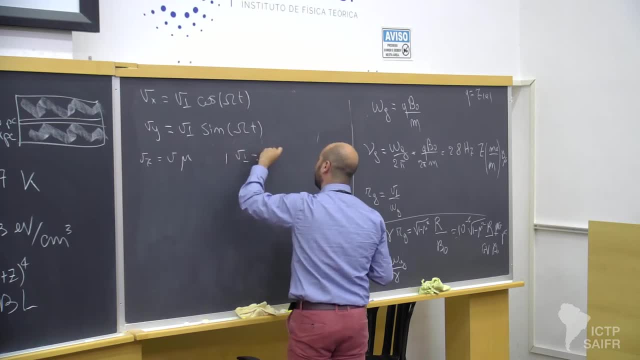 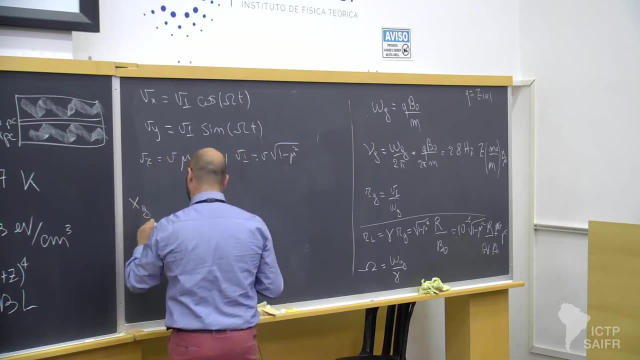 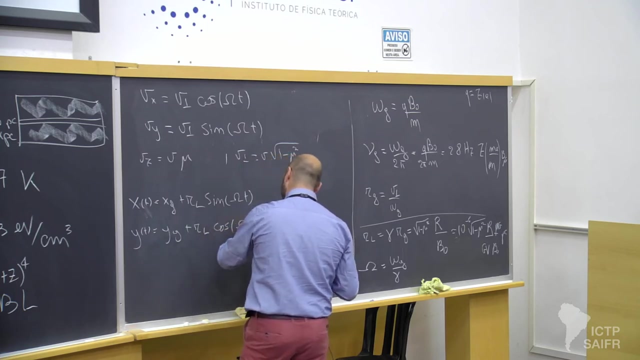 while v orthogonal, is v times 1 minus mu squared. OK, So far, so good. The coordinate, sorry. x of t will be xg, the initial position, plus RL sinus omega t. y of t will be yg plus RL cosine omega t. 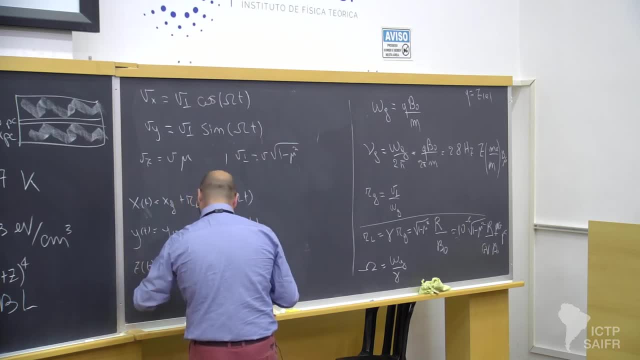 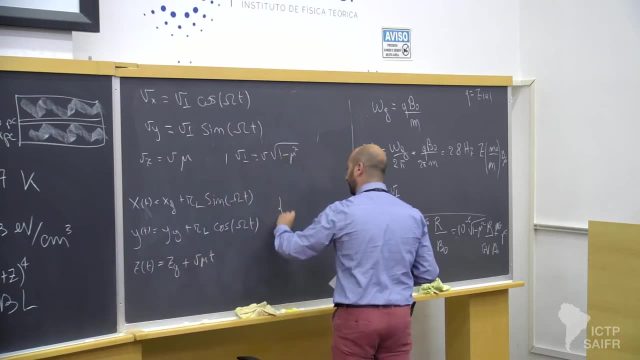 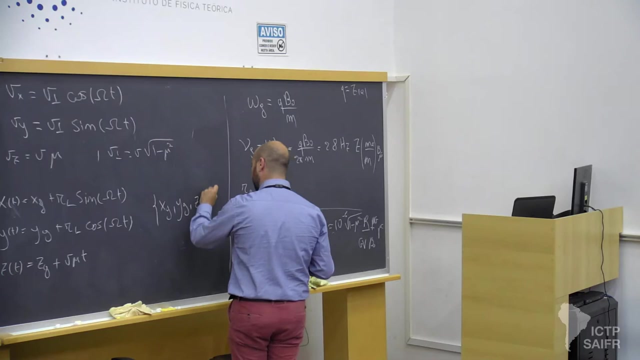 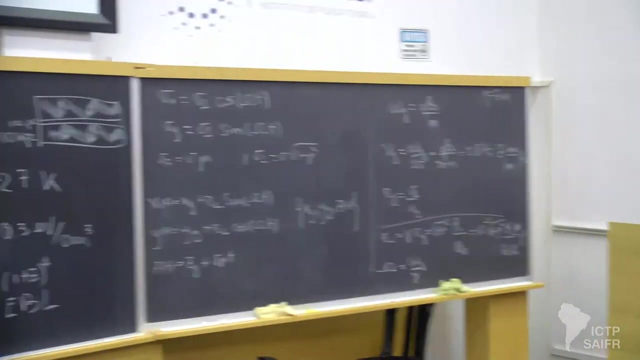 And z of t will obviously be zg plus v, mu, t. This point xgy, Yeah, Yeah, Yeah, Yeah, Yeah, Yeah, y g, z of t. This is called the guiding center of your particle. So what does it mean on this plot? 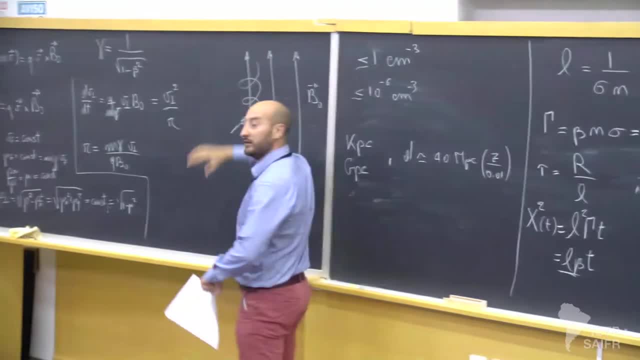 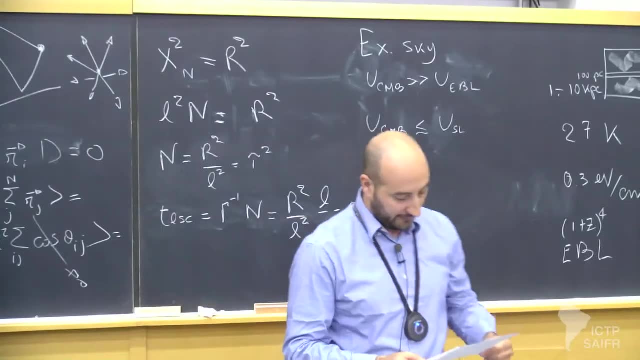 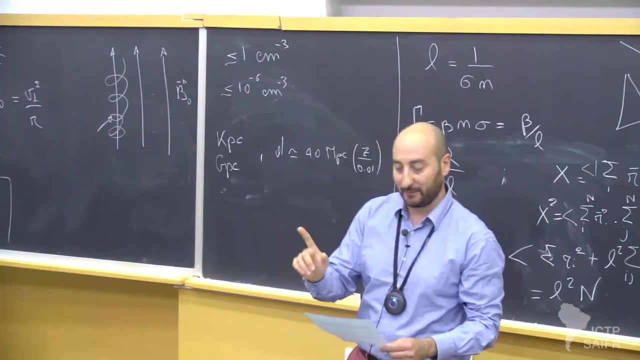 It's a point which is moving uniformly along this direction, So it's the center of this circle at any time. Very good, This was the easy part. Now, and probably you have seen this before- the interesting aspect happens, if I now. 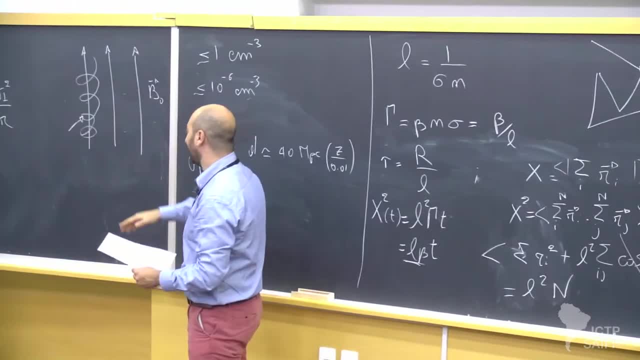 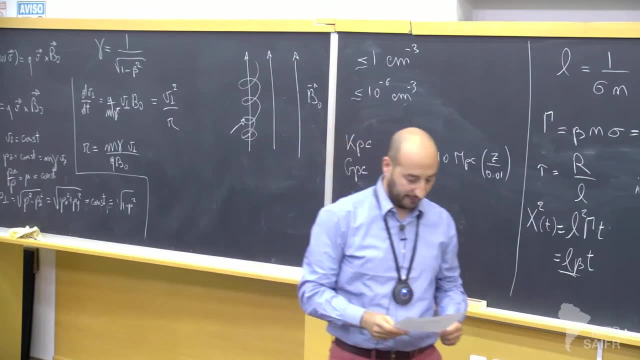 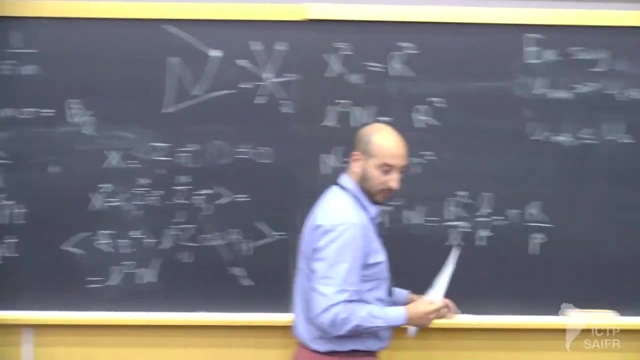 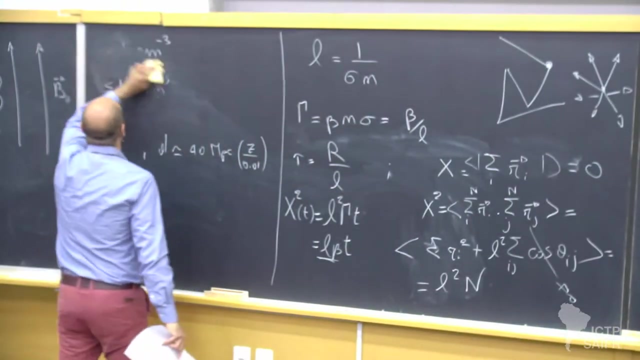 yeah, perturb this configuration and I will start adding a little sinusoidal perturbation on the top of this homogeneous field. I will choose this perturbation and I can erase probably this central part of the blackboard. I will choose this as orthogonal to my big field so that the 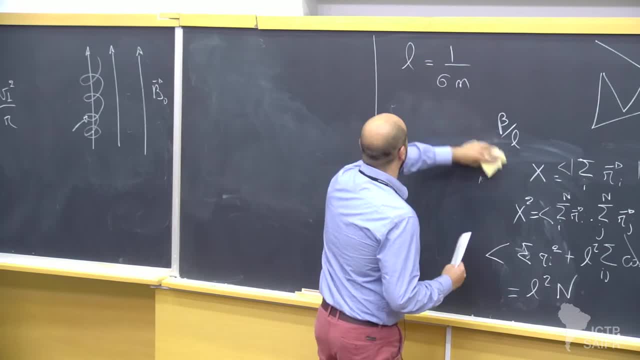 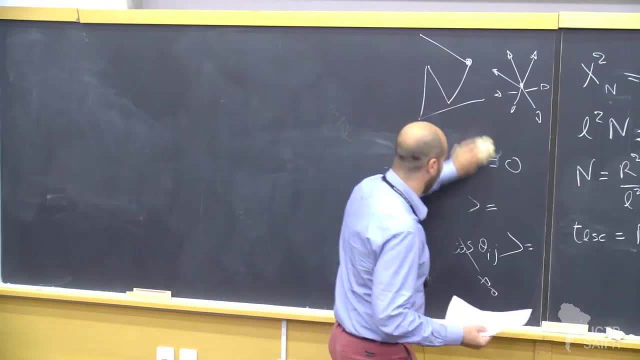 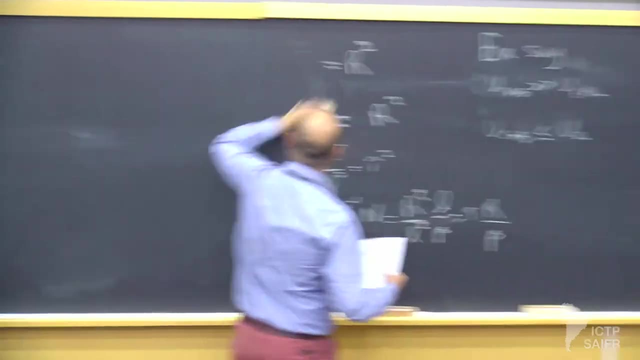 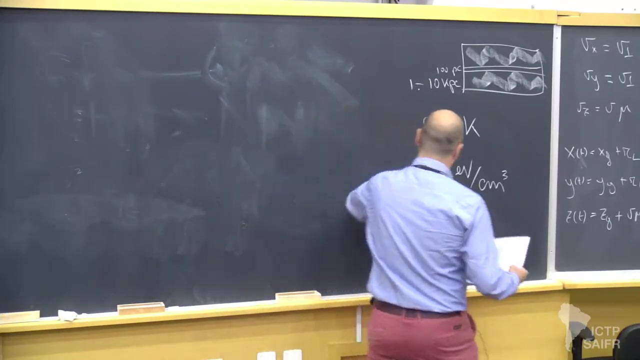 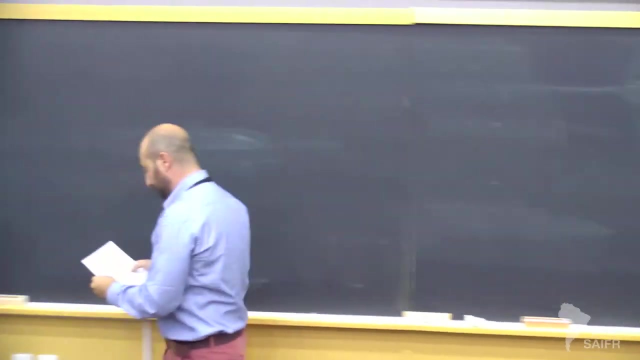 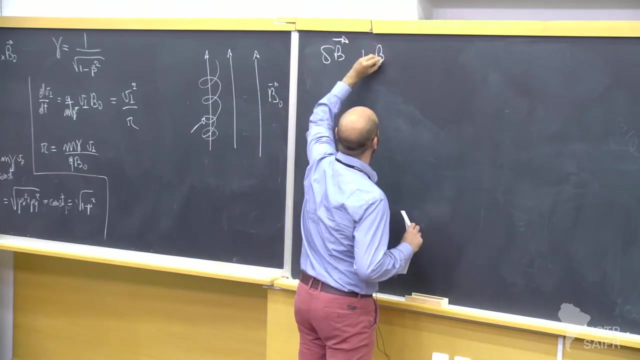 x-y movement is not altered and the only thing that is altered is the movement along Z. This will turn my problem into an effectively one-dimensional problem. So this is a simplification which is very useful to grasp the physics Very good. So I add a delta B orthogonal to my B zero, so that you can imagine now. 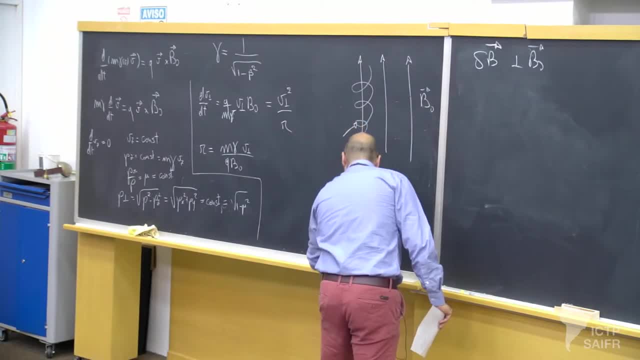 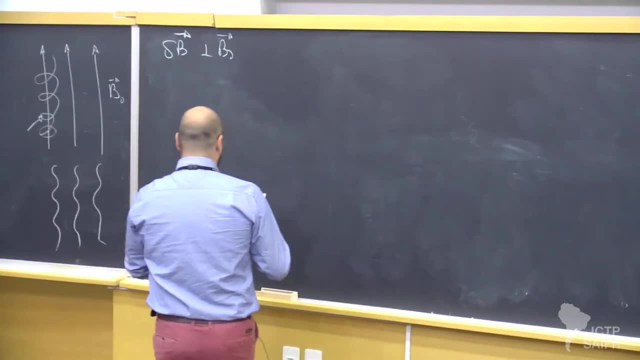 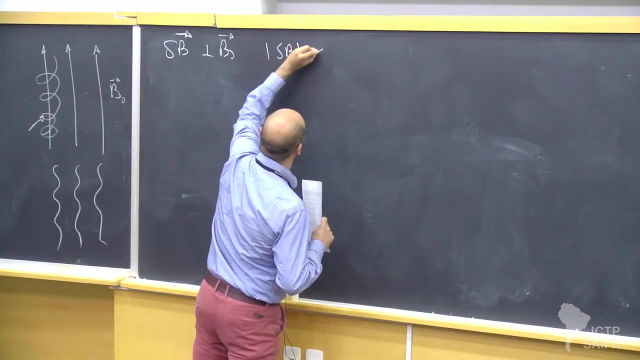 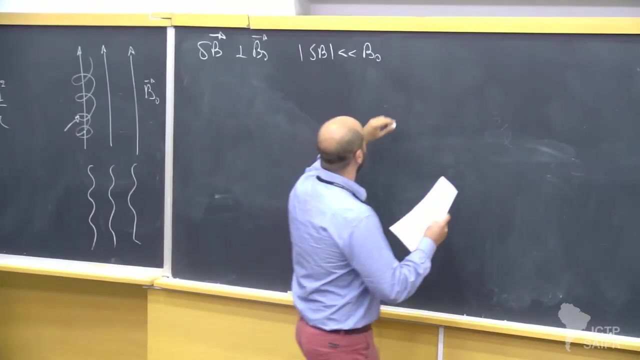 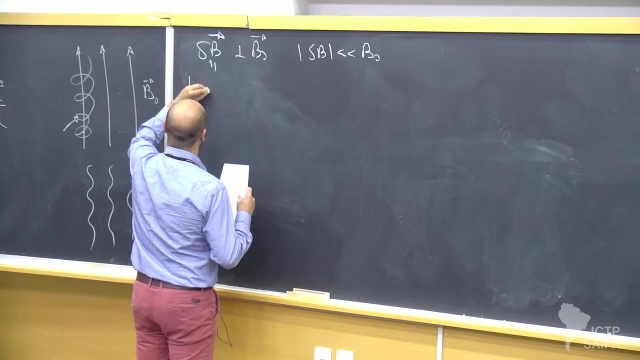 the field as being like that: Okay, Okay, Okay. And the x-y, this delta B in modulus is much smaller than B. Very good, And then for fixing the notation, this is the coordinates. This is what I choose. The components of this field are going to be cosinus minus kz, plus some random. 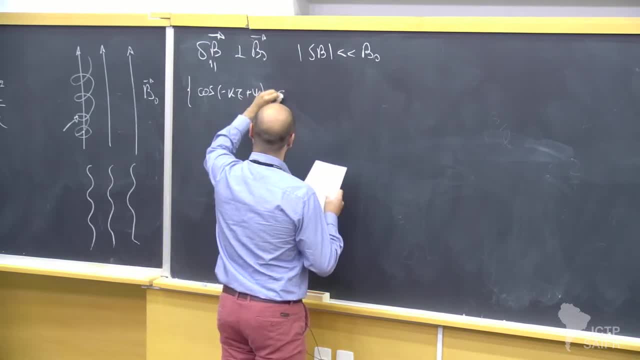 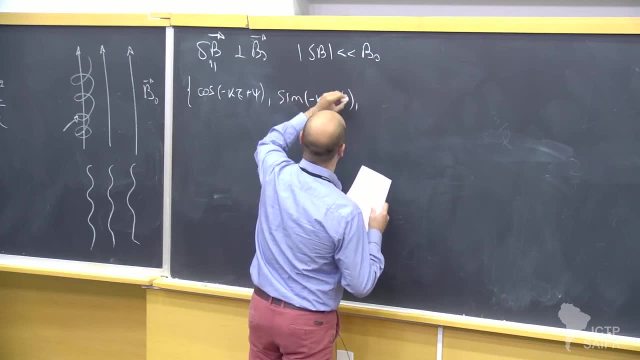 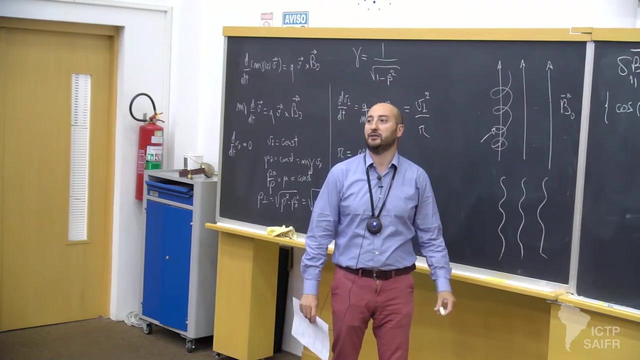 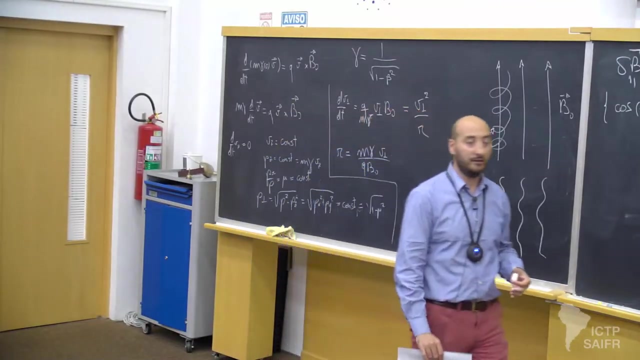 phase: psi Sinus minus kz, plus psi zero. Okay, Know that I chose a static field. This is not a propagating perturbation. Okay, You see no time here, Just the space direction. Okay, We will drop this approximation. 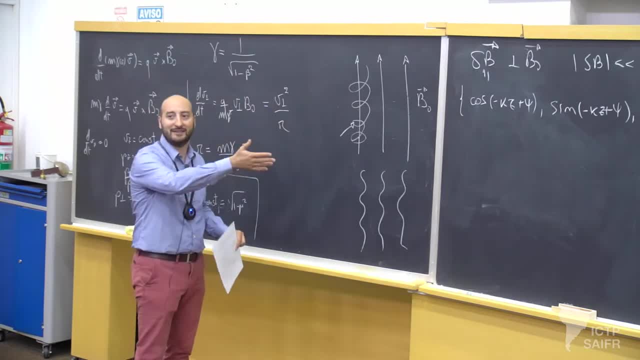 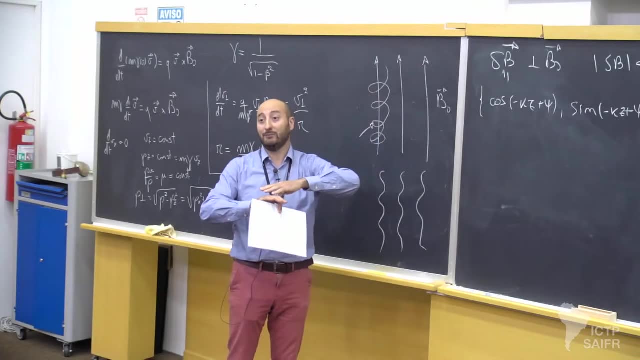 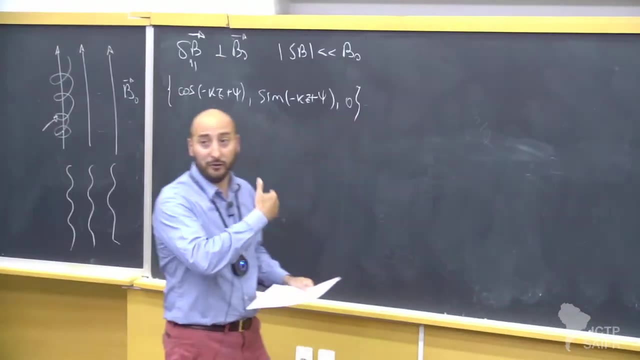 One good of a realistic argument for why this is not so bad to describe the zero potato. zeroth order is that you can think of the cosmic ray like moving much, much faster than the velocity of this perturbation. okay, So by using the equation of motion, 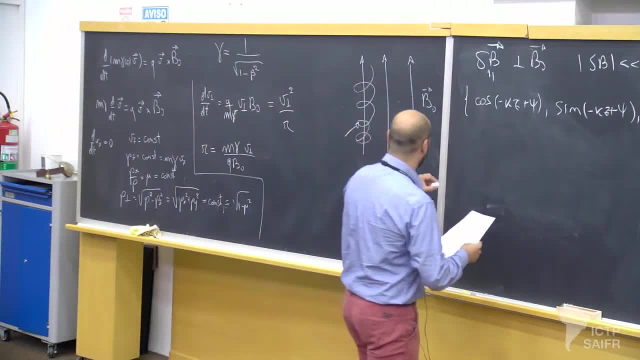 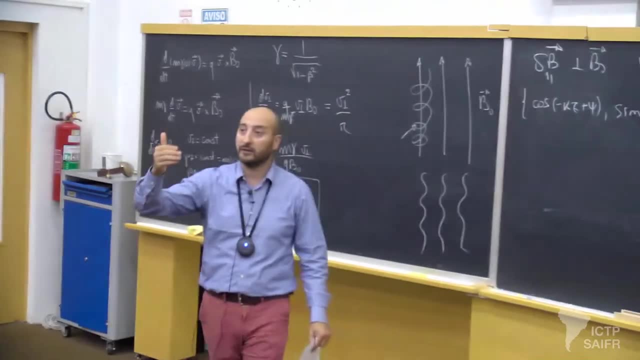 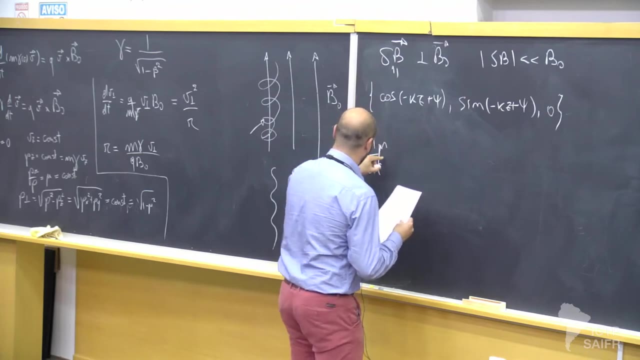 that we wrote. you will end up with describing the only coordinate which we assume has changed, which is the z component. okay, because of this condition, which means that d? mu over dt mu is the ratio of pz over p, so it's equivalent to vz. 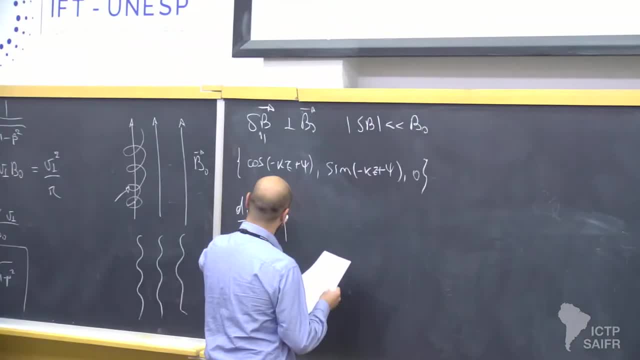 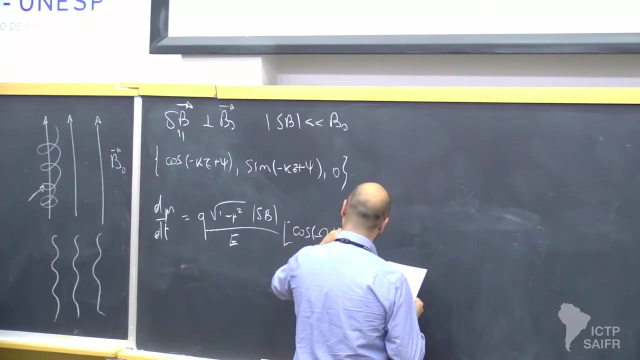 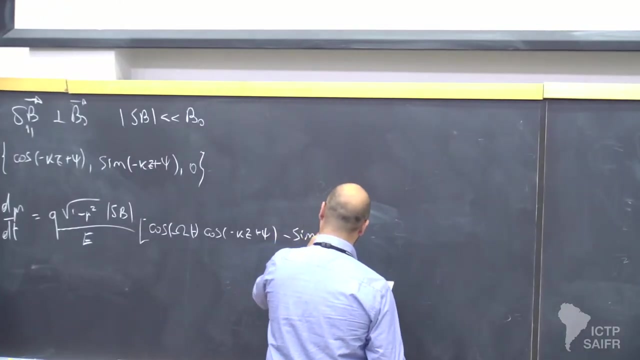 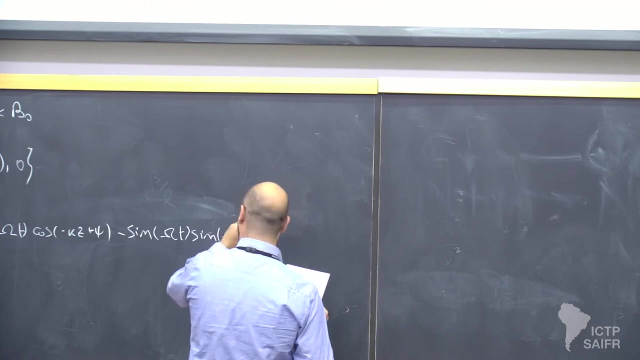 the third component of velocity is going to be q square root 1 minus mu square delta b over energy times: cosinus, omega t. cosinus minus kz plus psi, minus sinus. omega t sinus minus kz plus psi. And now I define some shorthand notation. 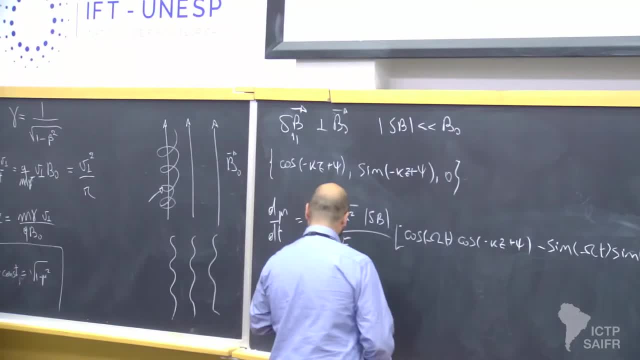 so let's call this capital C, for instance, and these will be these. I can use the trigonometric identity to rewrite as a single cosine cosine. I will call it cosine of w times, t plus psi, and this w. however. 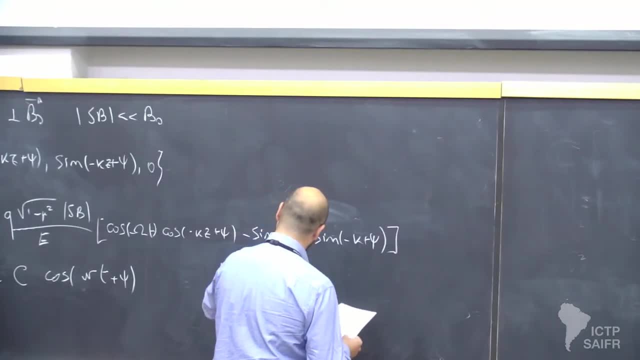 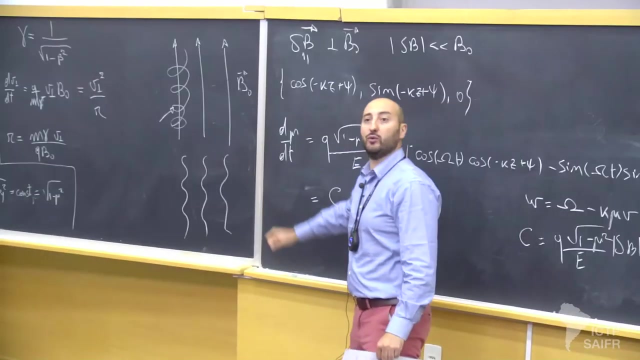 is going to be omega minus k, mu, v And c is q square root of 1 minus mu, square over energy times, delta b modulus. Now, what happens if I take the average of this quantity? The average over what? Well, the average over the random phases of these waves. 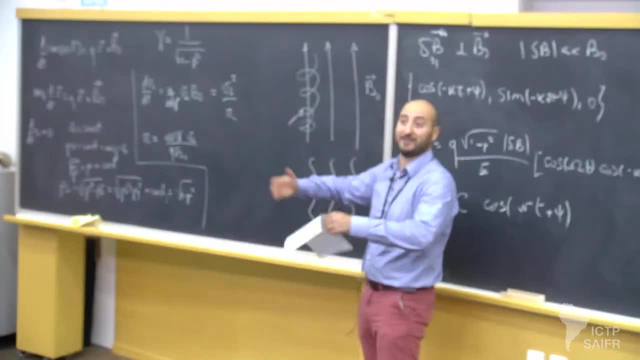 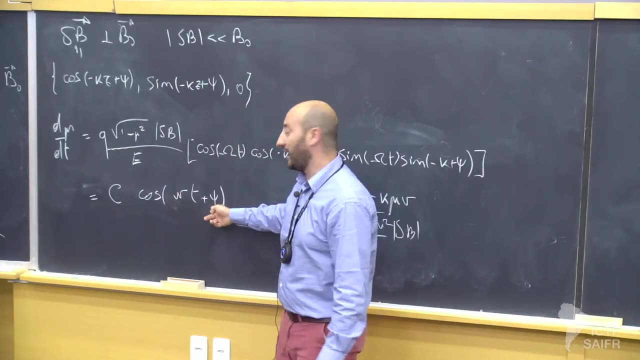 because there won't be a single perturbation. for instance, there will be an ensemble of perturbations. if I take a random phase approximation and you average these over psi, you get zero. Okay, There will be another approximation. that will be done. 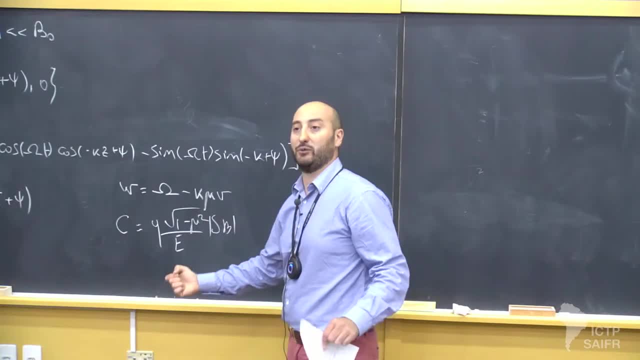 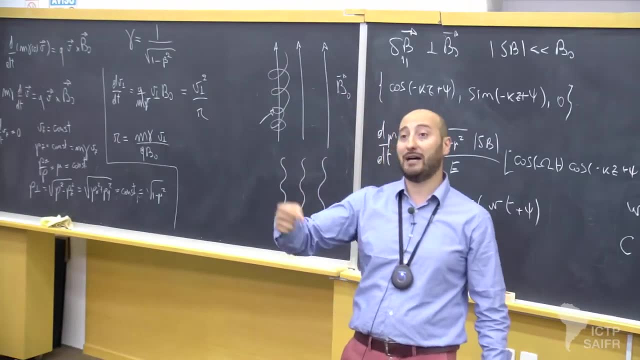 in the following, which is a long timescale approximation. Namely, we are only interested in the evolution of this particle over timescales which are much, much more complex, much, much larger than the gyro period. Okay, Why, I told you. 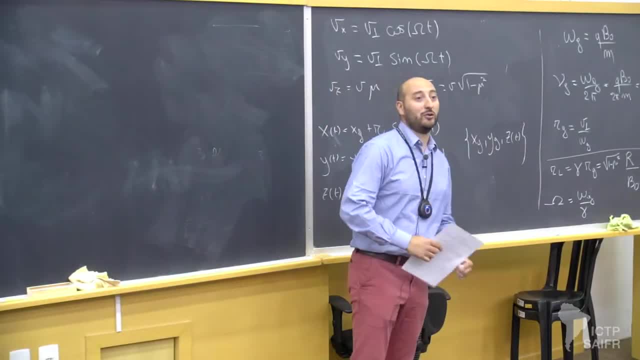 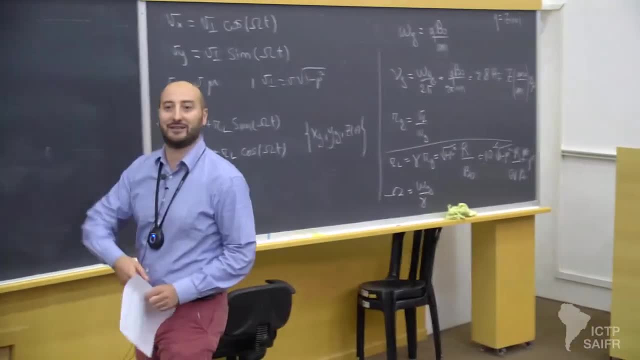 these are ridiculously small scales. Okay, We're talking about seconds or things like that, or 10 to the minus 6 parsecs, and we are interested to evolution over 10 million years and maybe kiloparsec. So basically, we don't care about the. 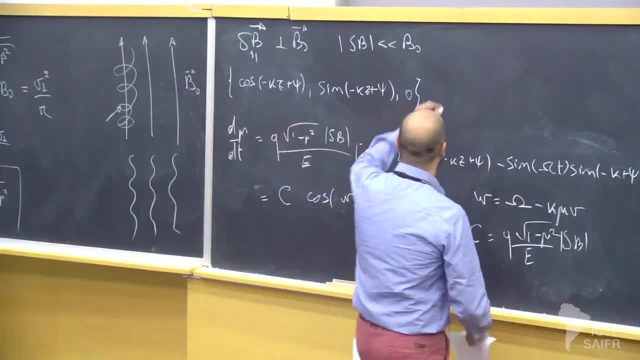 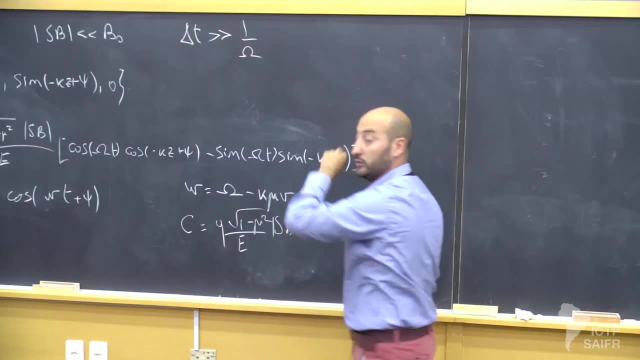 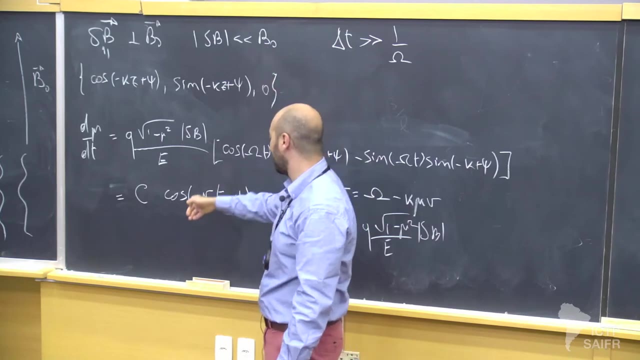 short timescale movement, which is equivalent to say that we care about typical timescales which are much, much larger than 1, over this omega that I was mentioning before And, of course, if you average these over timescales which are much, much larger than. 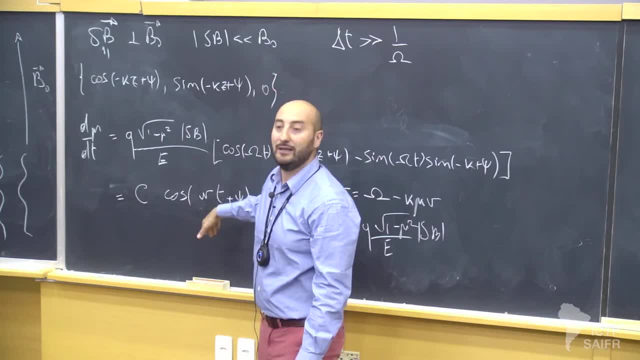 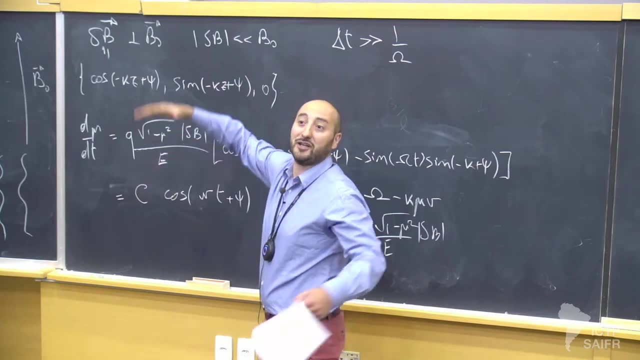 1 over w, or so you get 0.. Okay, Because this is a bounded function between minus 1 and 1, and you divided this over a large timescale, so you get something which is bounded by 1 over a large timescale. 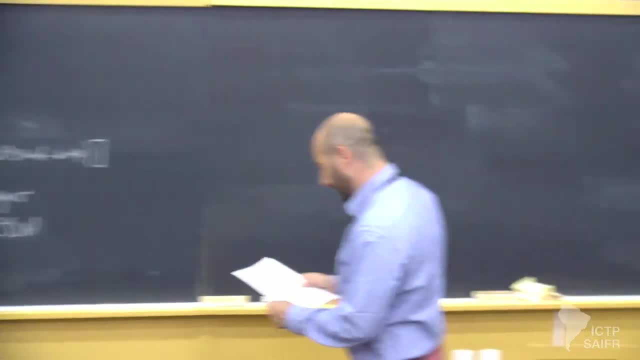 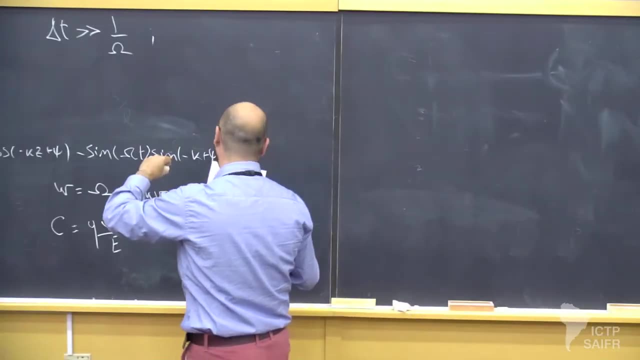 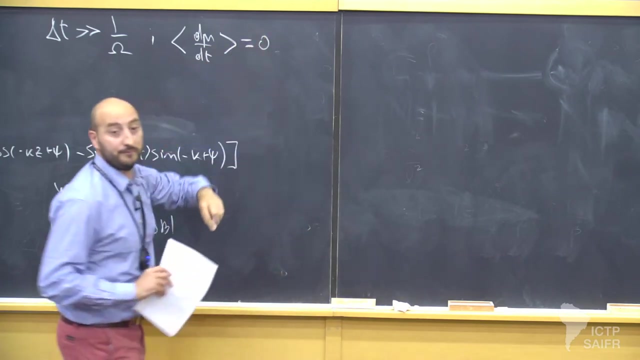 and that's basically 0.. Okay, So, on average, we say, keeping in mind this ensemble average of this sort that I explained to you, on average, d, mu over dt is equal to 0.. And you see now the similarity to the. 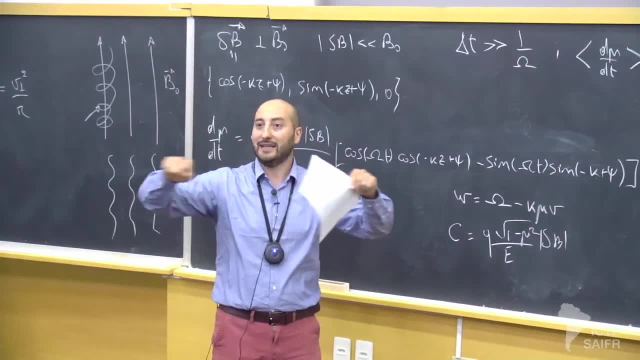 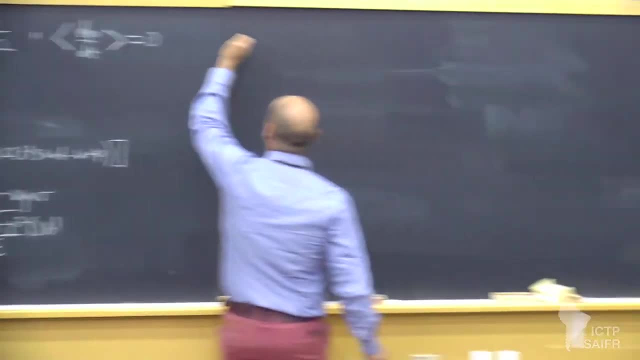 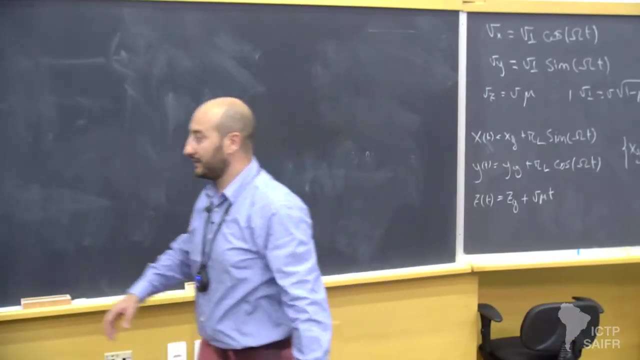 drunken path that I described before. Even there, the average displacement was going to be 0.. Okay, This is not true anymore. if you compute, however, the delta mu square as a function of time, So I take this, I multiply it by dt. 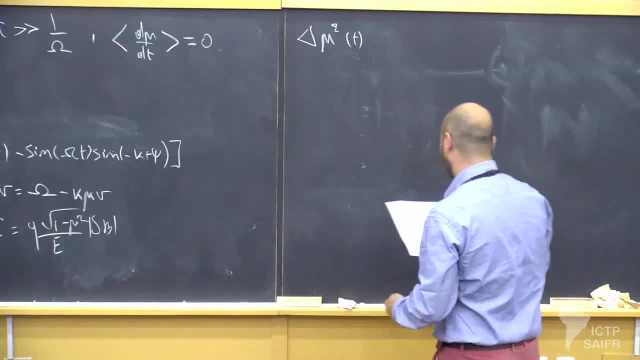 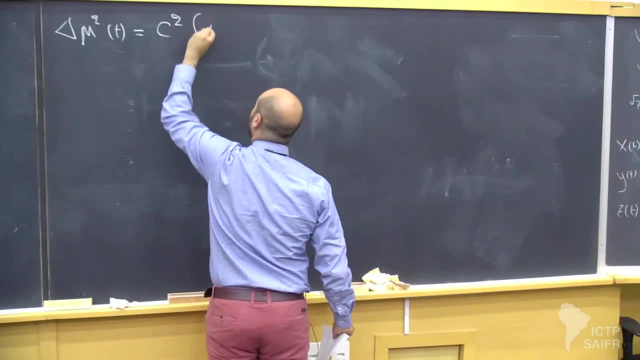 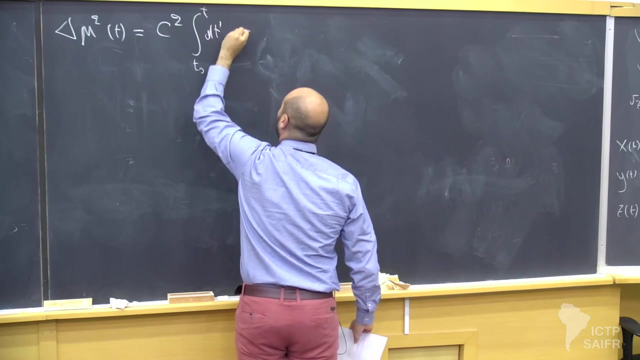 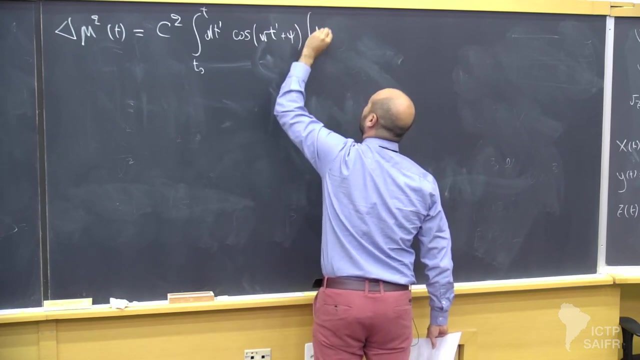 and I integrate over a finite amount of time. What do I get? I get something which is c squared integral dt from some arbitrary t0, sorry dt prime to t of what Cosinus w t prime plus psi. integral dt d prime d seconds, sorry. 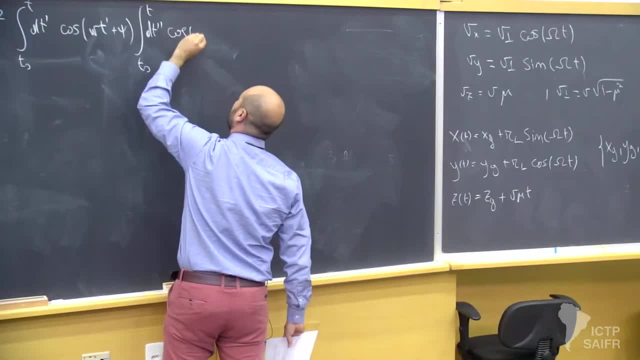 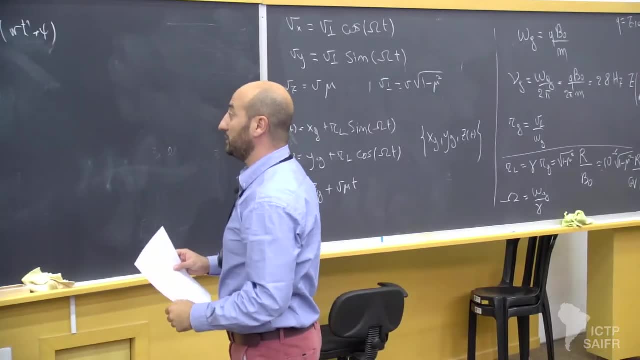 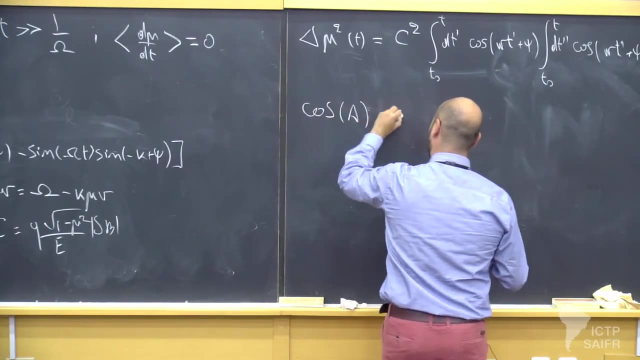 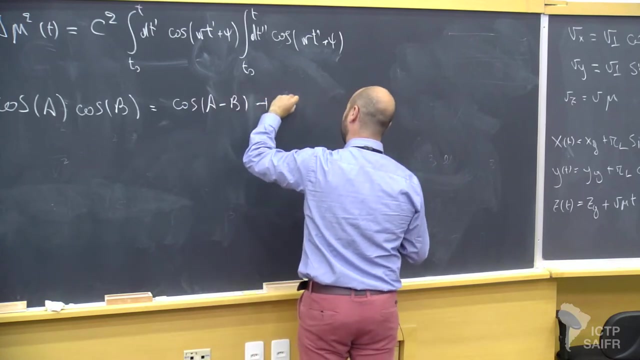 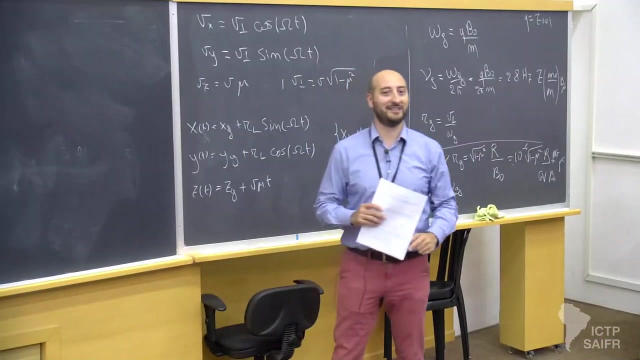 t0, t of cosinus, w, t seconds plus psi. And then I use a very advanced piece of math. Don't be shocked. You have seen this a long time ago, I think. Okay, So basically I rewrite this product as the cosinus. 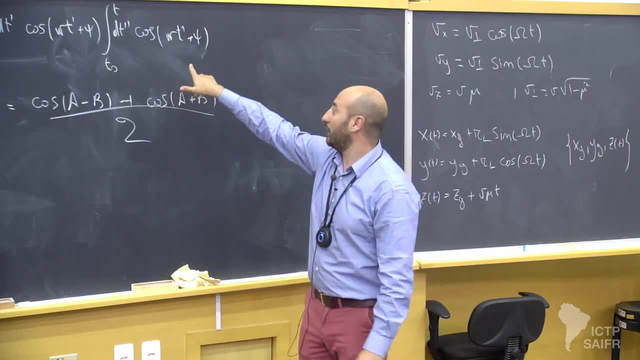 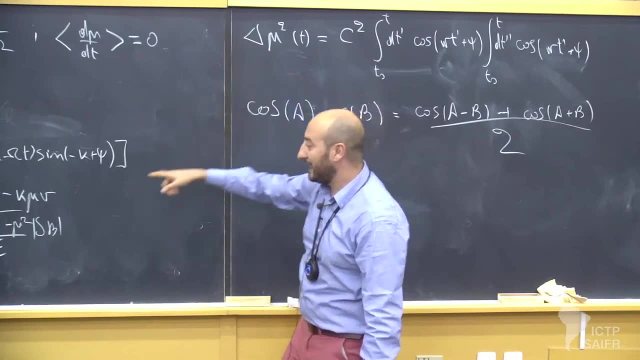 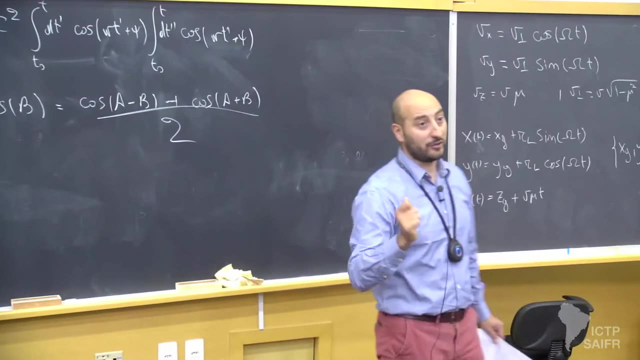 of a sum plus the cosinus of a difference. Now you see that once I have the sum and I take the average of this guy, this behaves exactly the same way as this. So this piece on average goes away. However, the piece containing 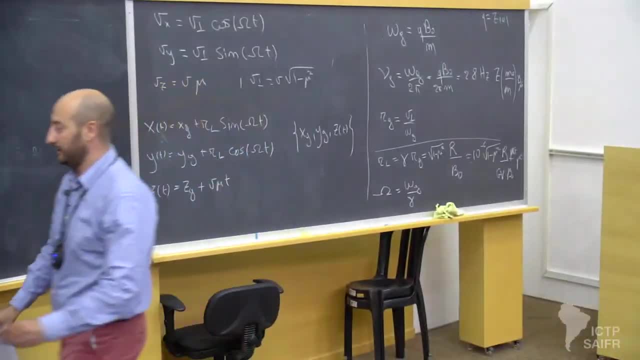 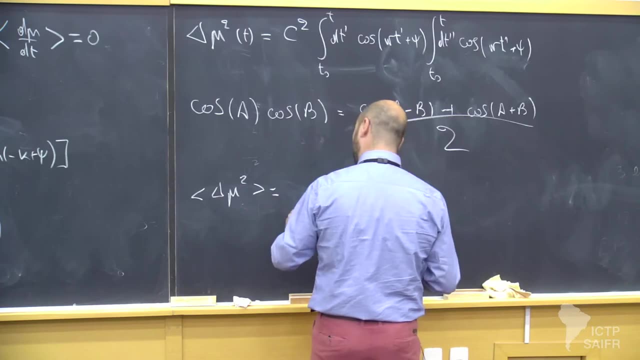 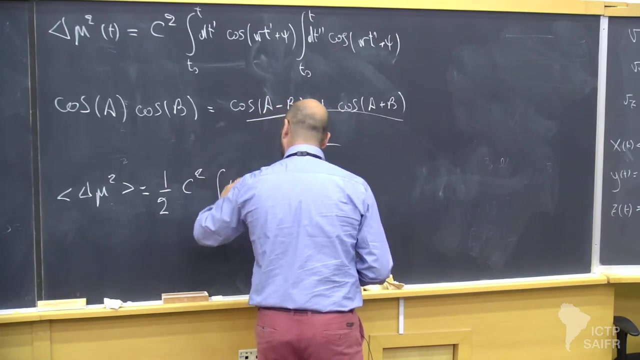 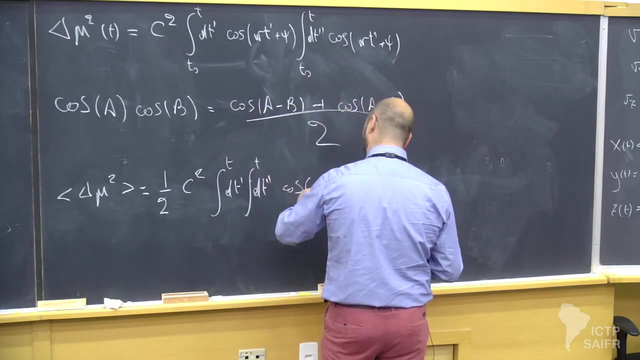 the difference does not go away. Okay, Why? We will rewrite it like delta mu squared. Okay, This will be one half of c squared, and then you have this double integral: dt prime, dt second, up to t, cosinus of w, t prime minus. 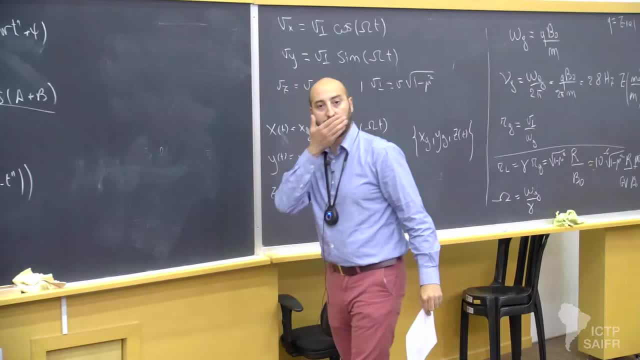 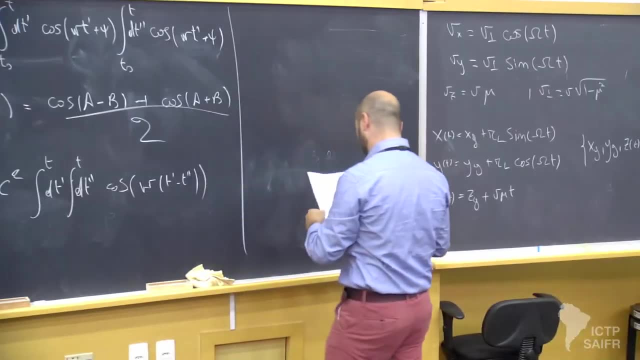 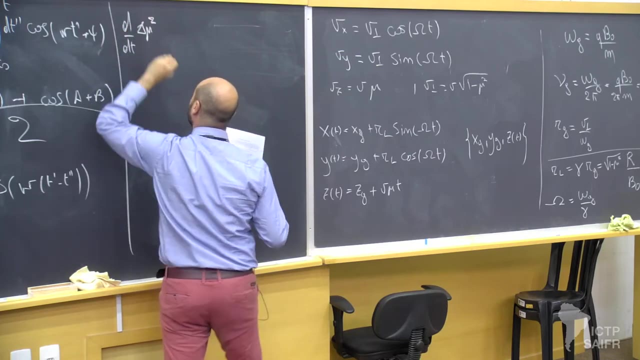 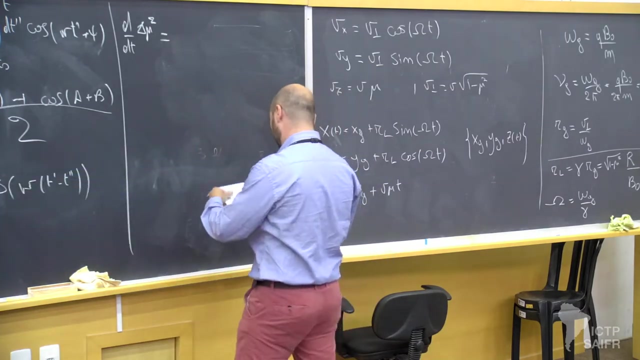 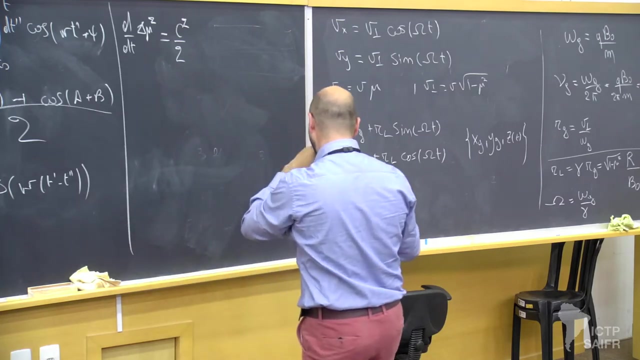 t second. So far, so good. This implies that the derivative over time of delta mu squared- this comes from the definition of a function through an integral. okay, is going to be c squared half, and then you have two pieces. In principle, you have the piece. 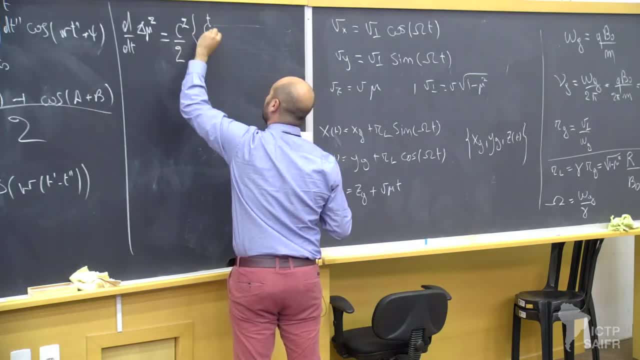 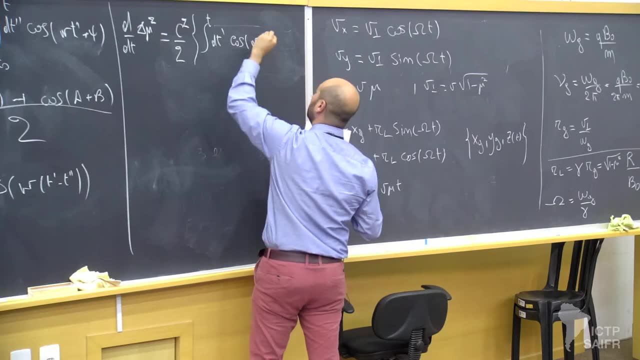 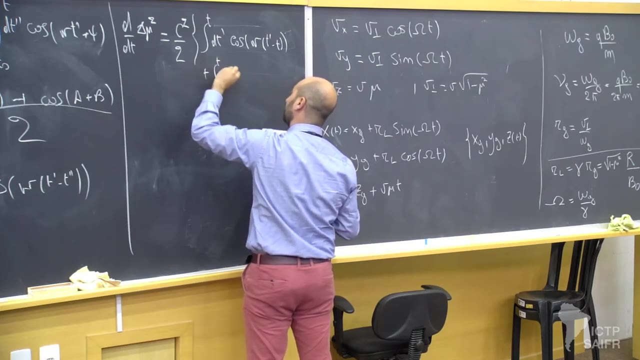 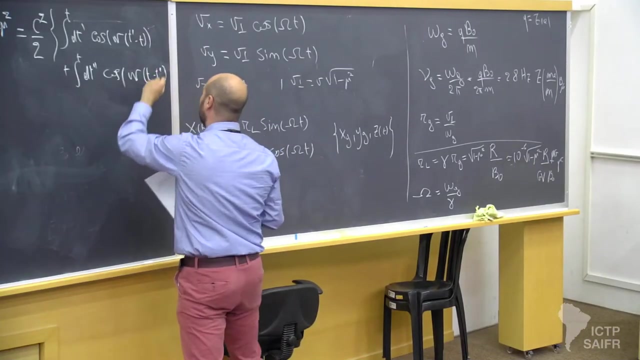 which goes as integral over t dt, prime of cosinus w t prime minus t. and another piece which is integral over t dt, second cosinus w t minus t second. Okay, Now, these are exactly the opposite of each other. I can rewrite this as an integral minus t. 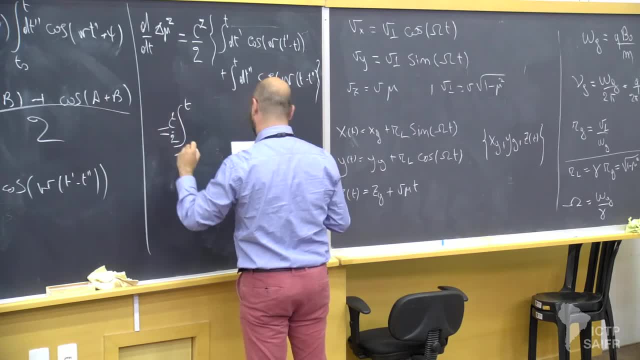 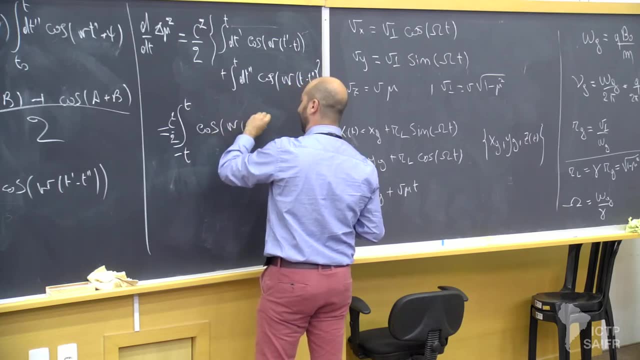 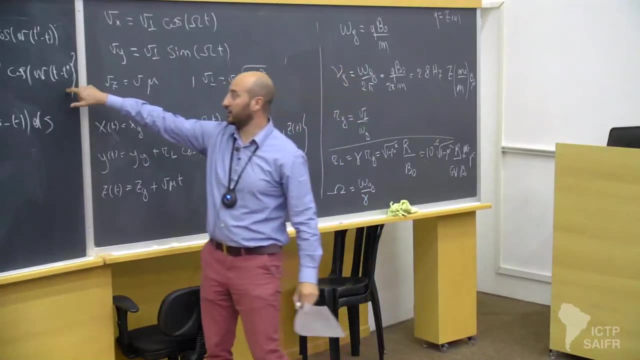 t c square alpha of cosinus. let's call it something like w s minus t prime, sorry, minus t d s, because you see that the argument here is just the opposite of the other. I can change a variable and that's what comes out. and now comes. 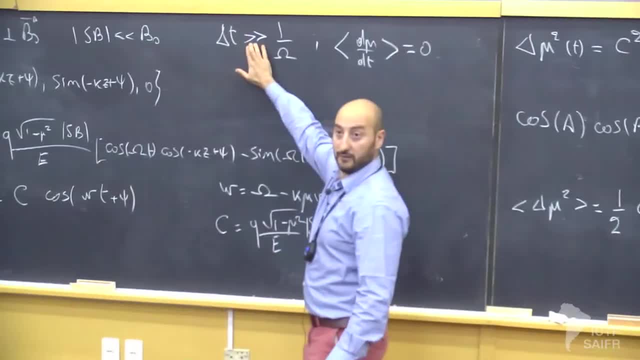 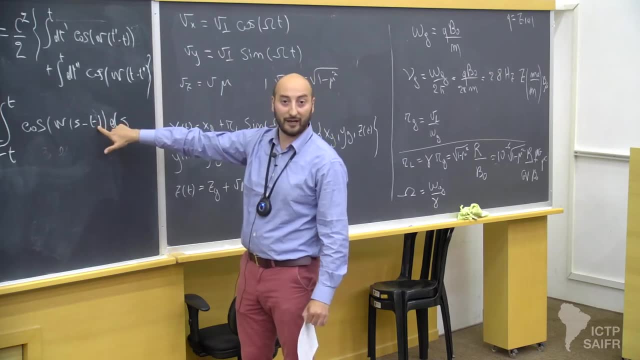 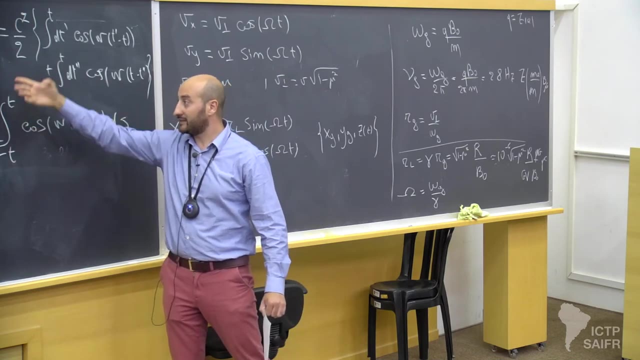 in again this approximation. so this is a little bit tricky because you see that the t argument, the time variable, enters here and then there's also in the extreme of integration. however, I know that whatever time I'm looking at is very, very long with respect to the typical time scale. 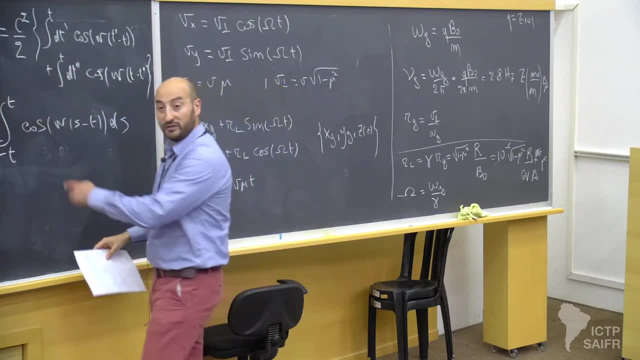 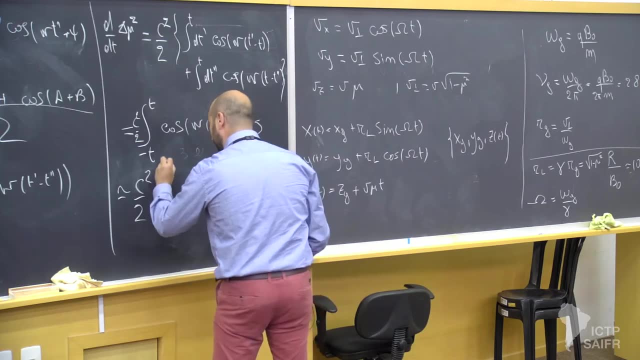 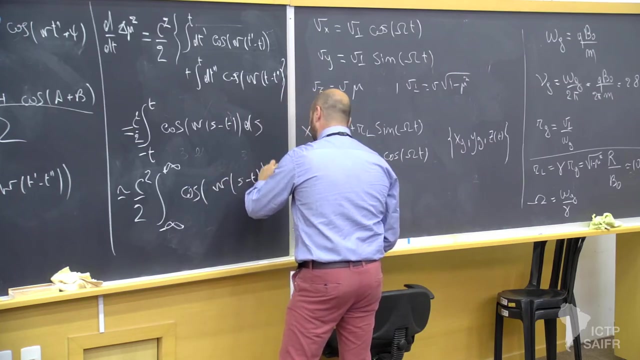 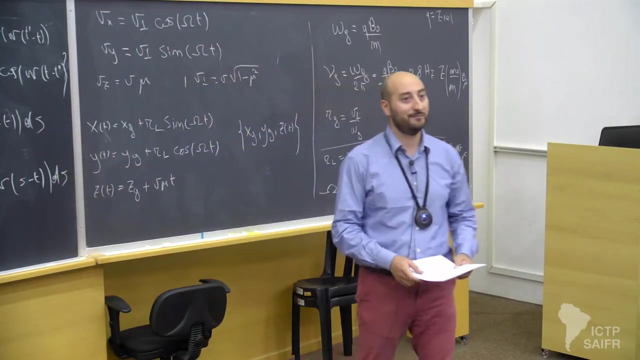 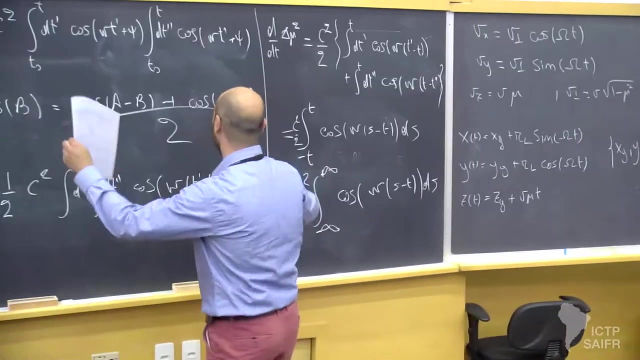 of your one over omega. okay, so I approximate this to c, square, alpha, integral minus infinity to plus infinity of this function, d, s. and here is the magic trick, because now I can rewrite this in terms of the exponential representation. what can I erase? I can erase probably this part. 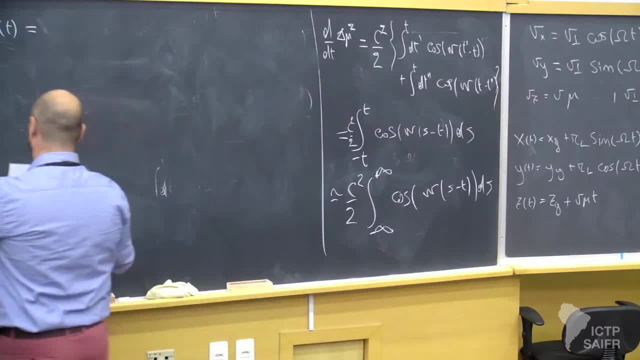 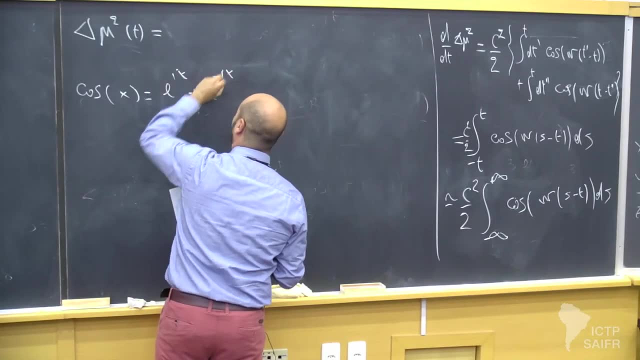 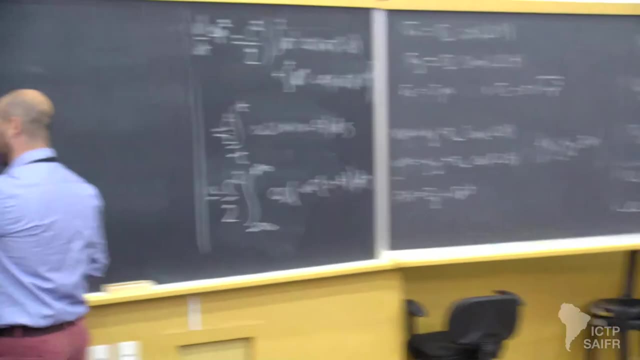 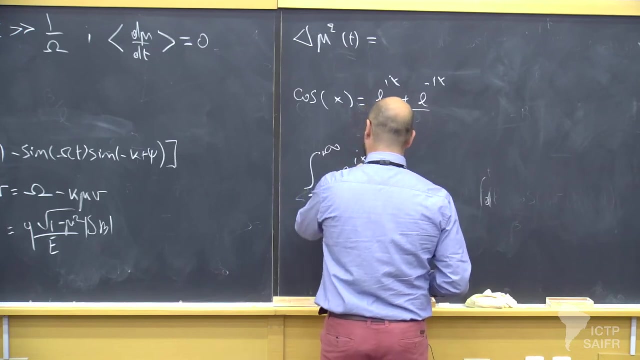 another very advanced piece of mat is that the cosinus of x is e i x plus e minus i x divided by 2, and then I have the integral minus infinity plus infinity of something that behaves like x, i, x, d x- sorry, x say y times d x. 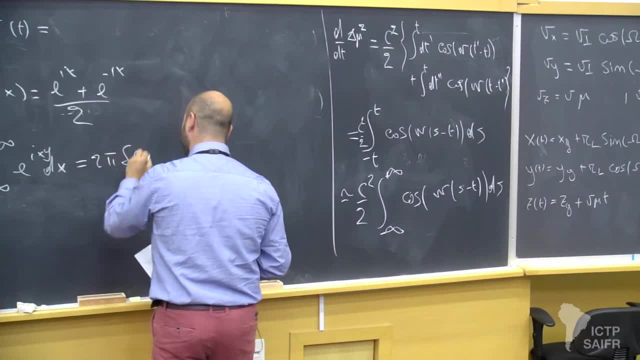 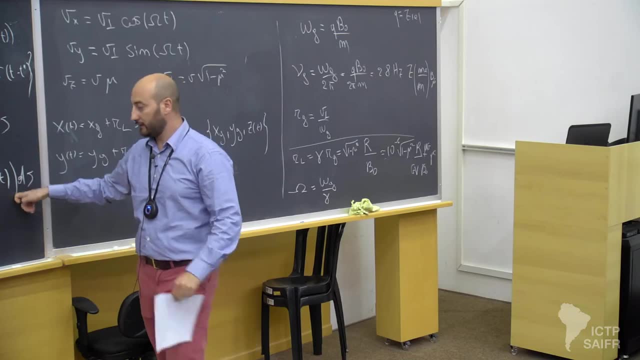 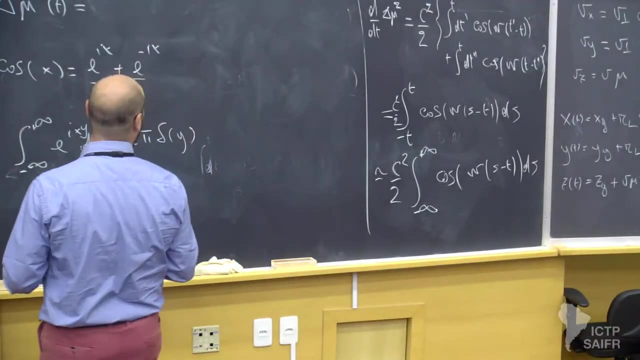 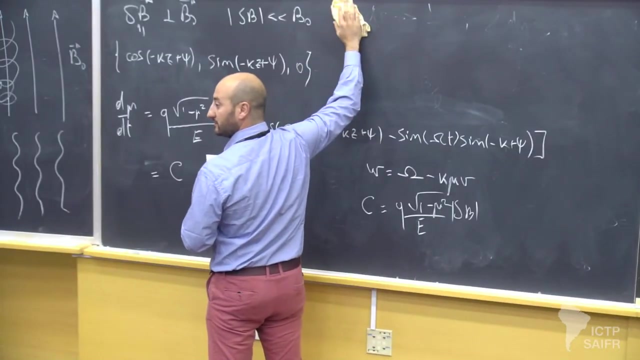 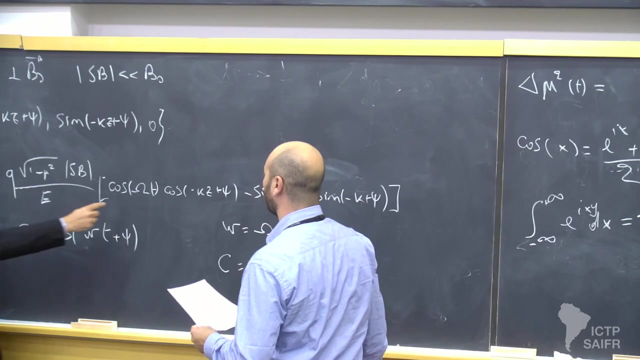 and this is 2x to the 1 x, And this is 2 pi delta y, which means that if I replace this here, I get an important result that deserves to be put. probably Yes, Yes, of course, Of course. 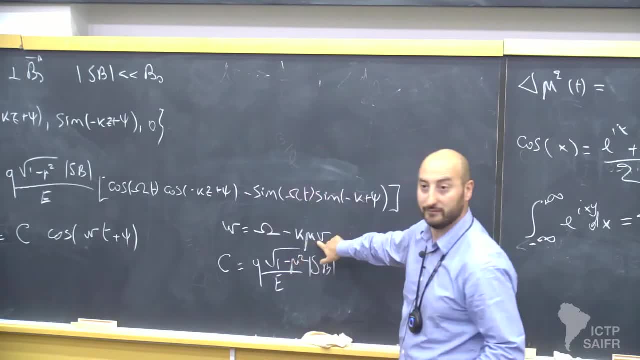 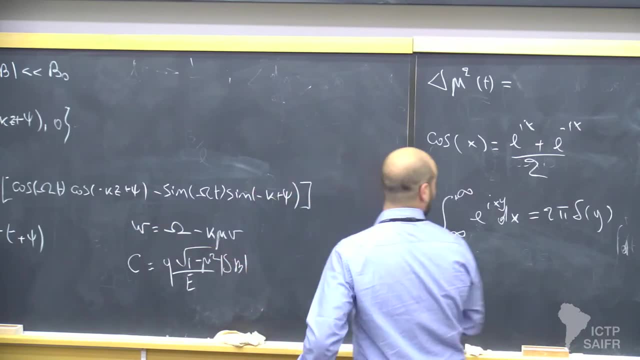 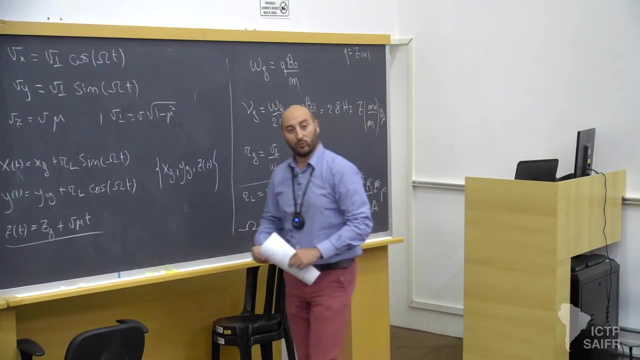 Exactly. Yeah, This is simply sorry here. Okay, So here I'm replacing the z with this expression here that you see comes from here, Okay, So what I'm doing here is a little bit delicate, in the sense that I'm assuming that, as a result, 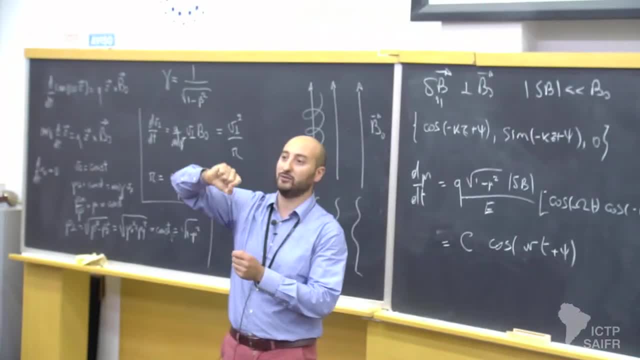 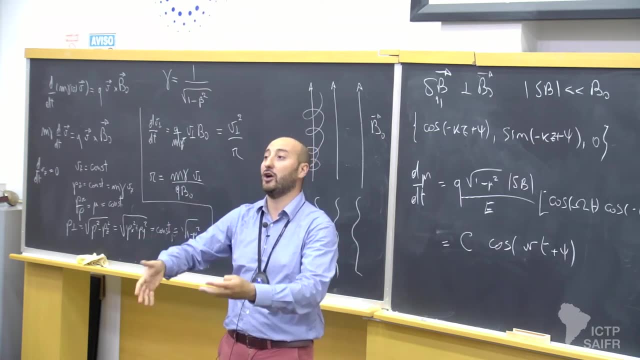 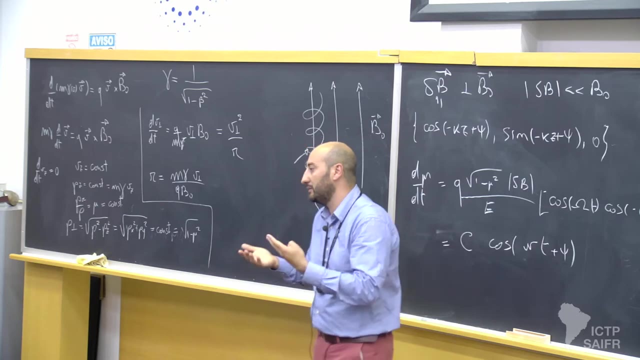 of this perturbation affecting this movement, the how to say that I can apply this perturbation on the top of the unperturbed trajectory that I had computed before. Okay, So this is intrinsically a perturbative approach, Which is justified as long 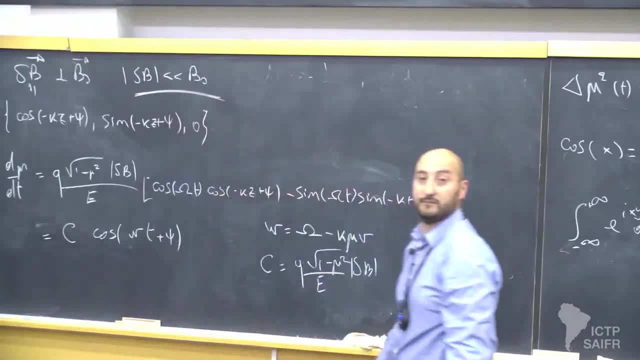 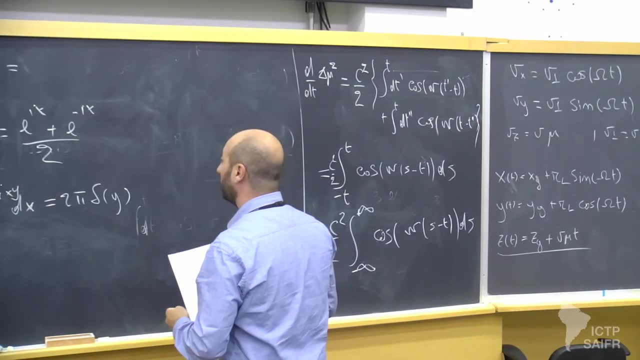 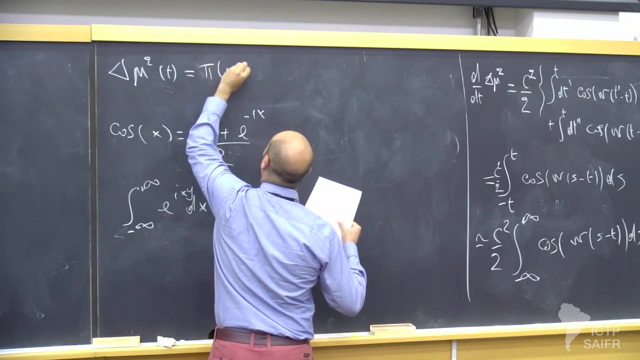 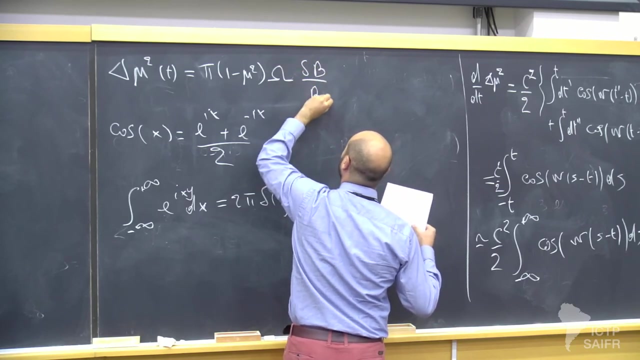 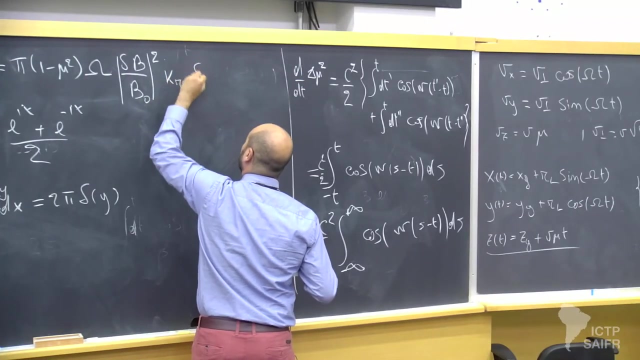 Exactly This comes from this. Okay, And as a result of all this mess, we end up with an expression: pi 1 minus mu squared, omega delta b over b0 squared, And then 19.. And then we introduce this resonant momentum: 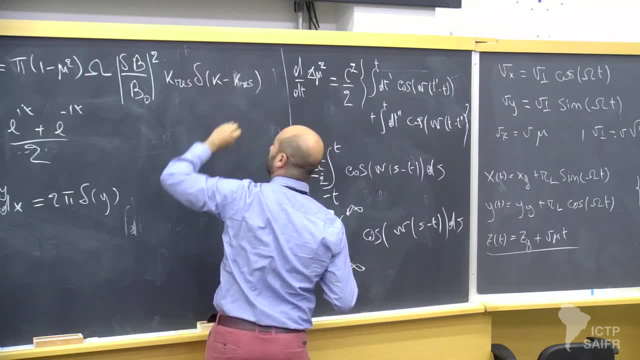 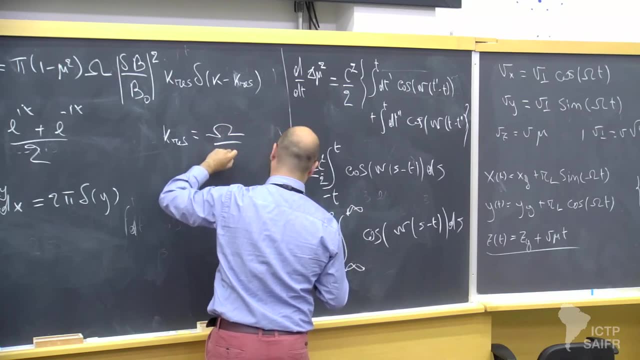 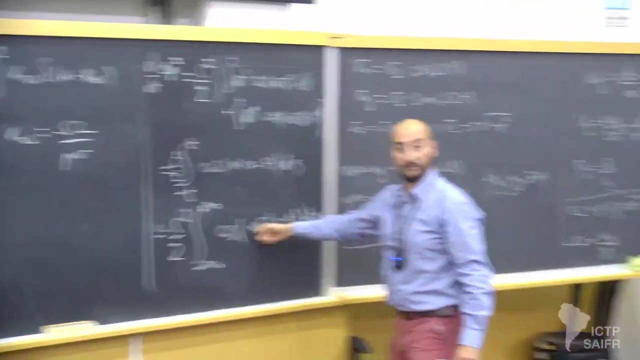 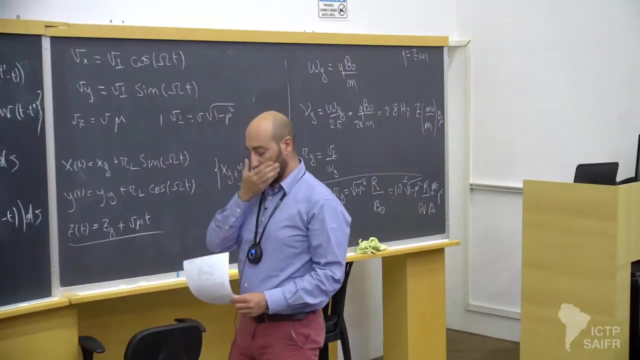 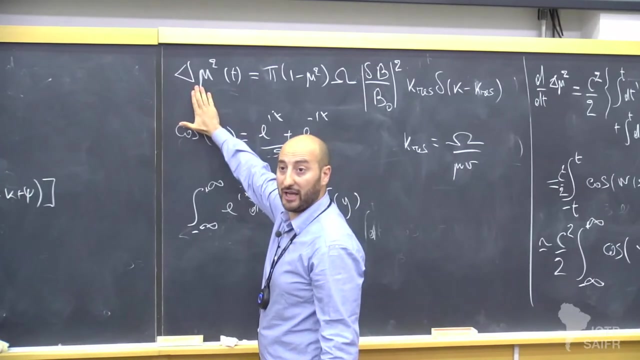 This comes from the properties of the delta, Where k res is just omega over mu times v. Okay, So this comes from this, plus this identity. So what have we discovered? Basically, we have discovered that the variance of the pitch angle over time is not vanishing. 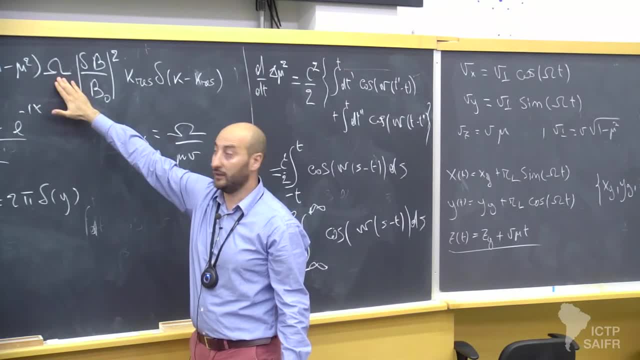 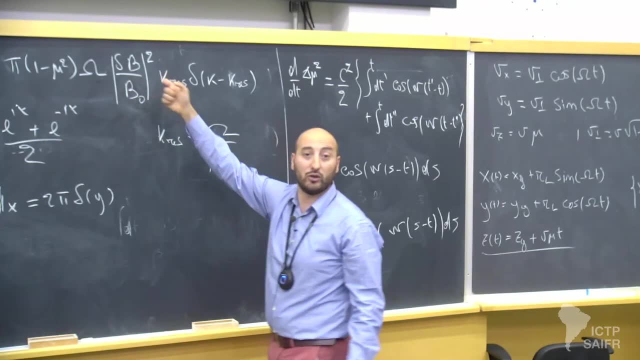 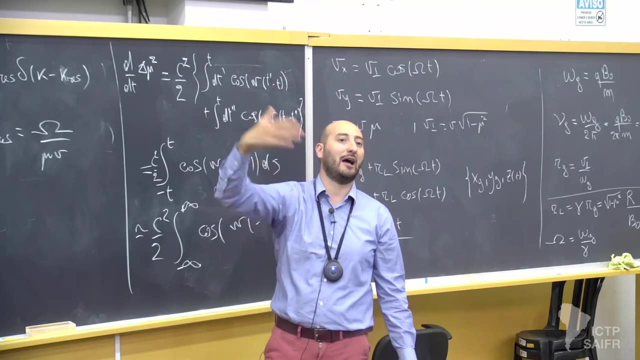 It's proportional to the relativistic gyro frequency times. what? What is this piece? This piece is the amount of energy in the perturbation with respect to the baseline field. Okay, The more perturbed, the larger this variance. Okay. And then there is this resonant piece. 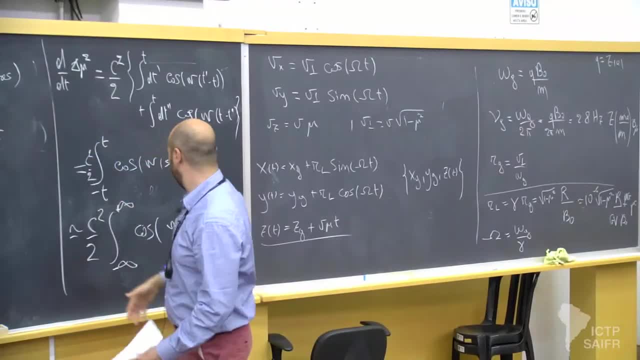 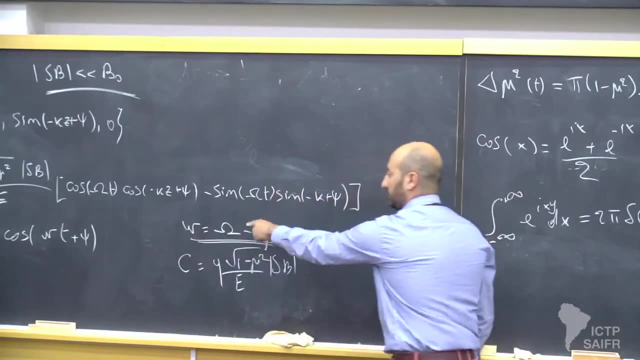 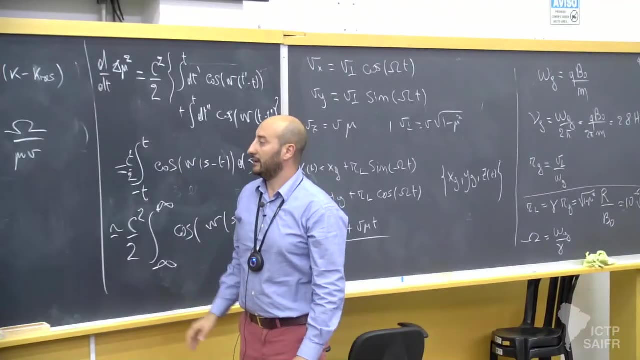 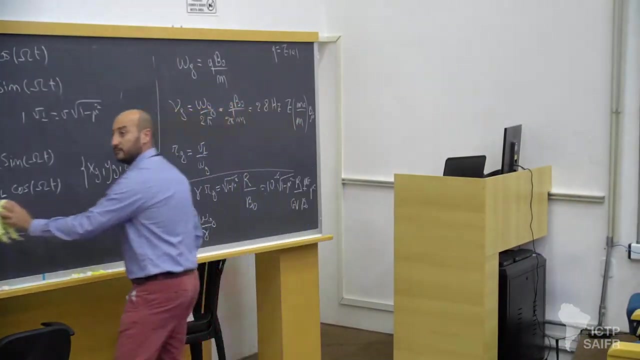 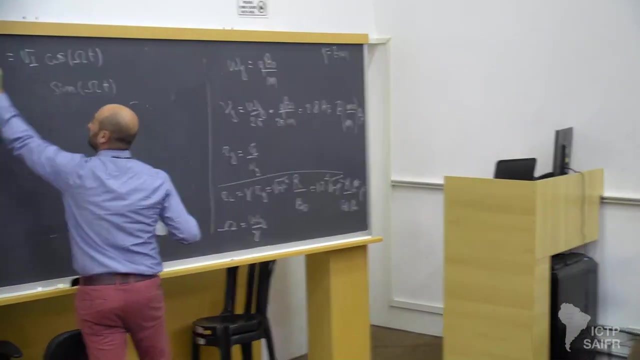 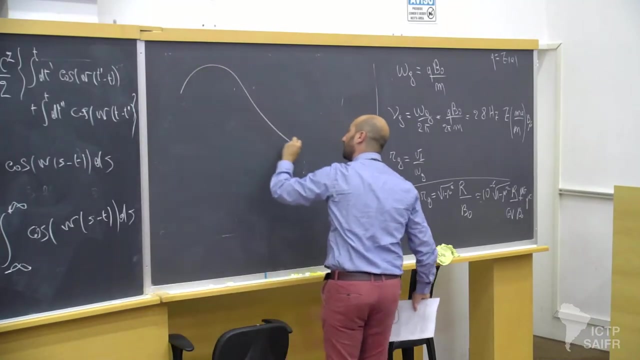 Okay, This resonant piece basically depends on this argument: this thing to vanish. And what does it mean physically? The best way I can show you what it means physically is to draw a picture. Okay, What it means is that if you have a particle, imagine that you have a very long wavelength. 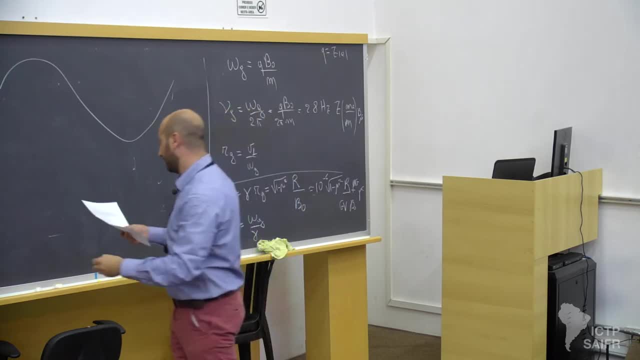 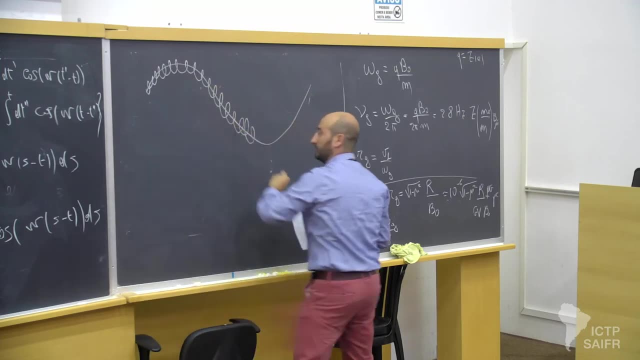 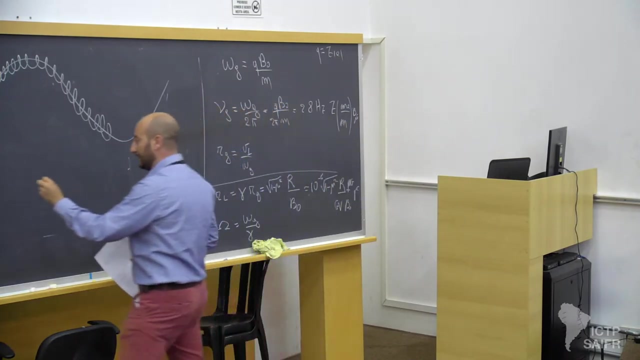 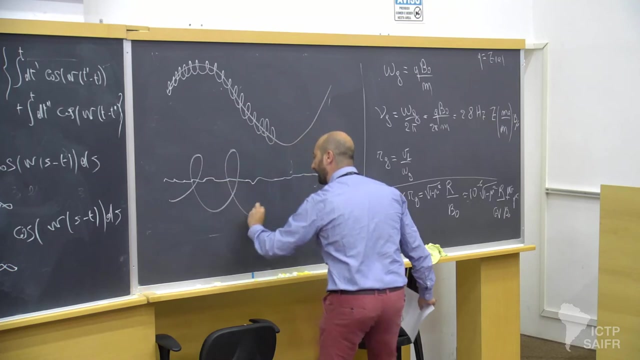 perturbation with respect to your gyrating particle, your particle will just surf this wave without any effect. Basically, Okay, Okay. So if you have a very long wavelength perturbation with respect to your gyrating motion, what your particle will see is some sort of little noise, but your particle keeps gyrating because 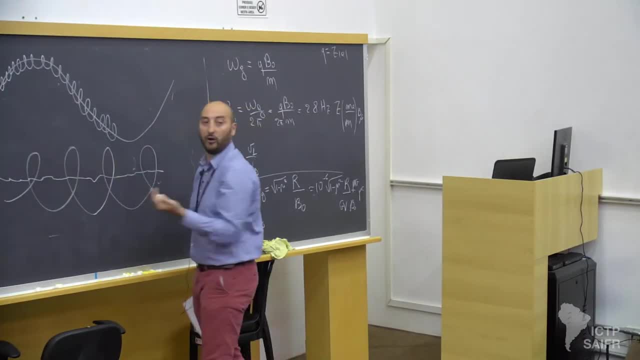 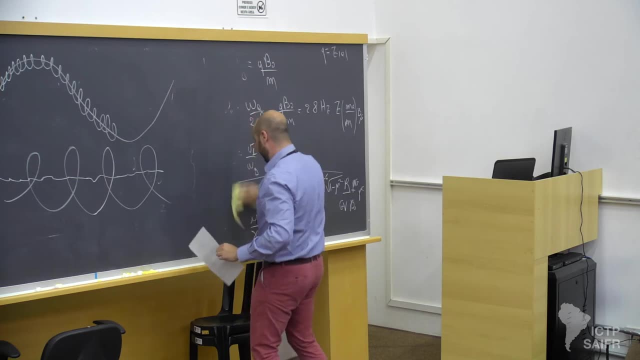 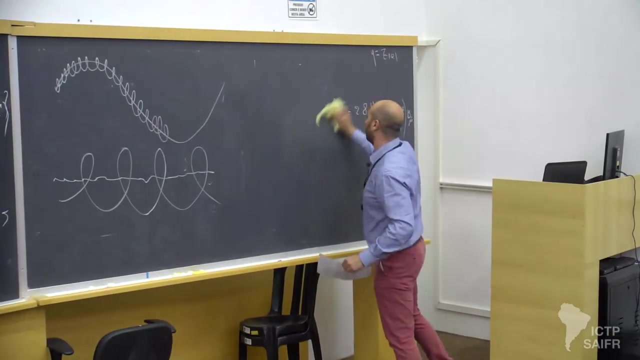 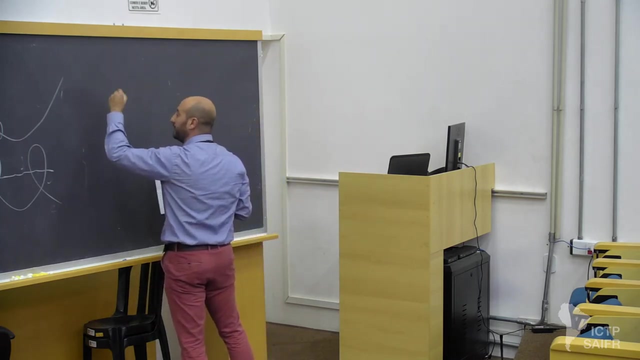 it's averaging out this noise over a single orbit already. However, if your particle has the right Larmor radius compared to the wavelength of your particle, Of your perturbation, then it can move away. It can undergo an efficient, an efficient. let me draw a line like that: 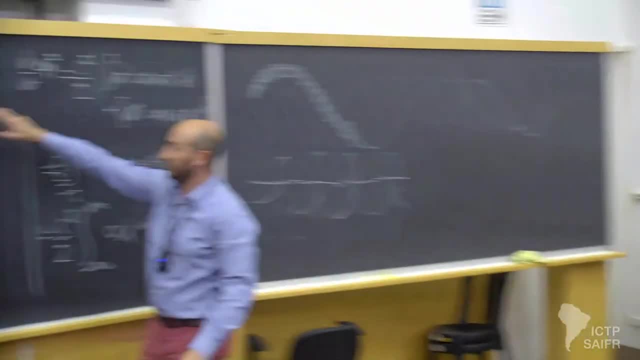 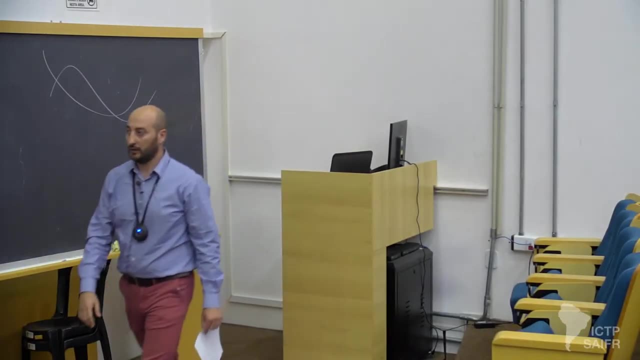 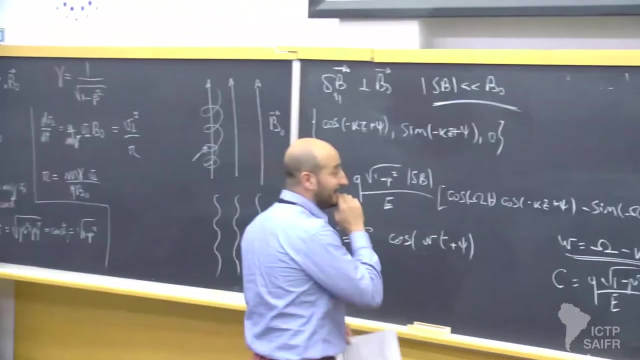 In this case, which is this resonant case, your particle can diffuse along your Z direction. Okay, And so there will be a finite amount of this. Okay, Now, an even more simple way to describe this phenomenon is to look at the fact that 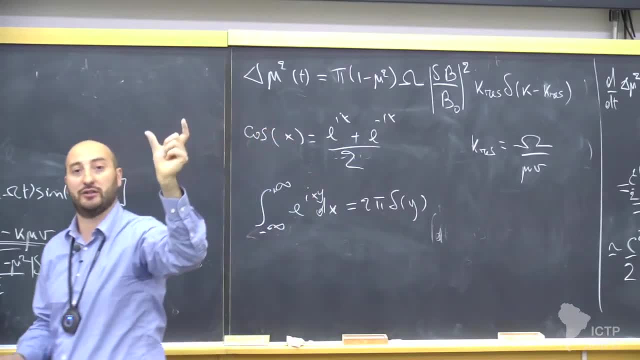 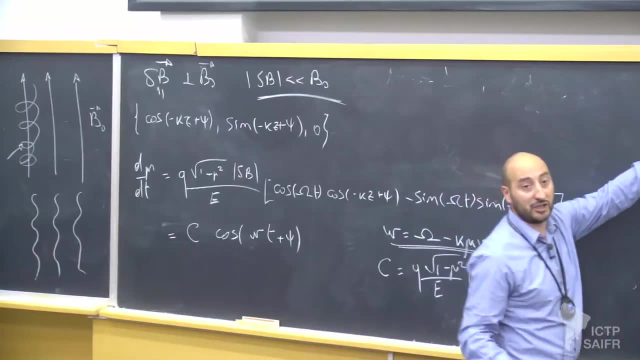 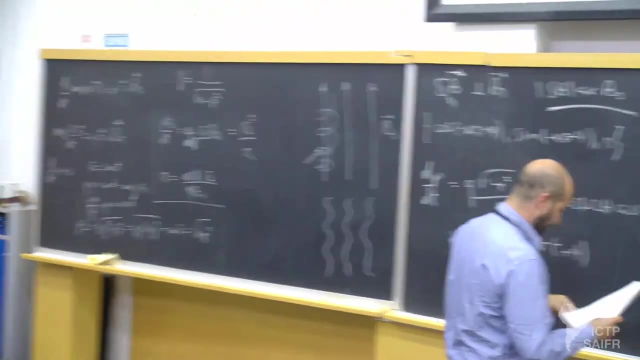 this one minus mu square is nothing but this projection effect on the orthogonal direction with respect to the field. So instead of writing the diffusive, the variance of the pitch angle, we could write directly the variance of the angle and define the analogous quantity, a sort of diffusion coefficient. 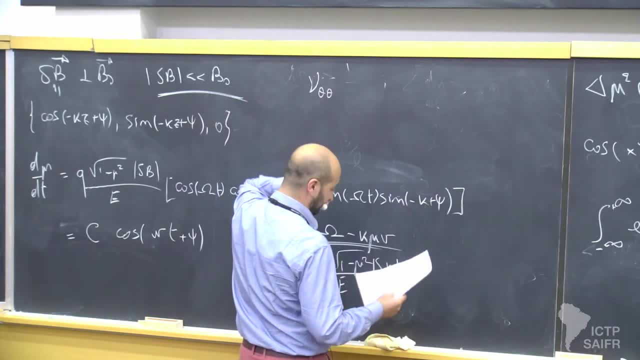 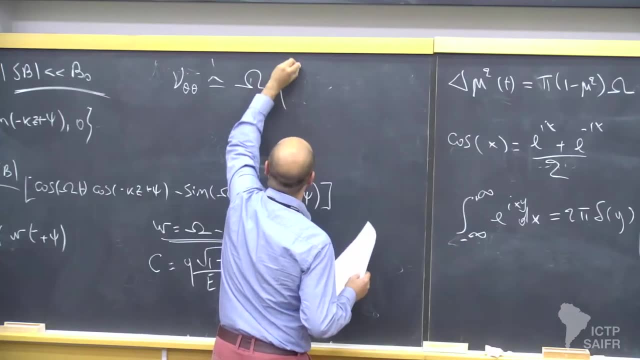 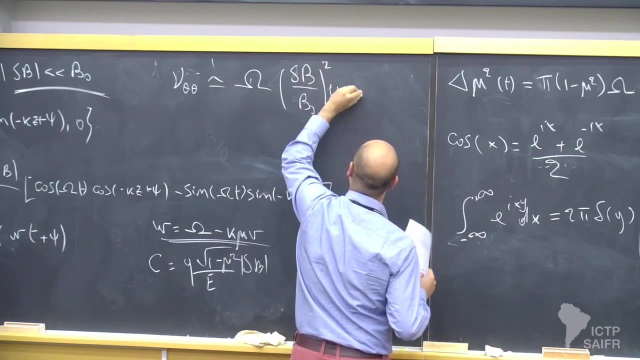 but for the angle directly, So we can write this as theta instead of the cosine of theta And as argued in the notes, I won't repeat all the steps here. this will be of the order of omega delta B over B, zero square, evaluated at this resonant condition. 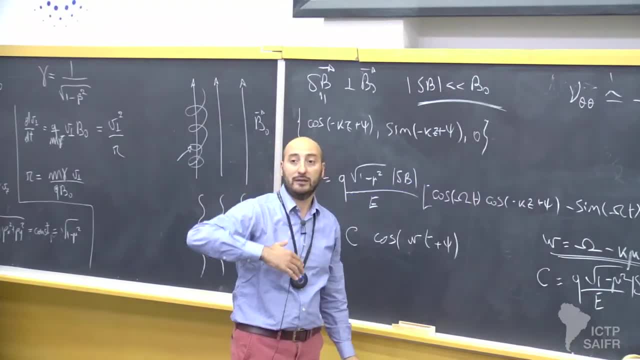 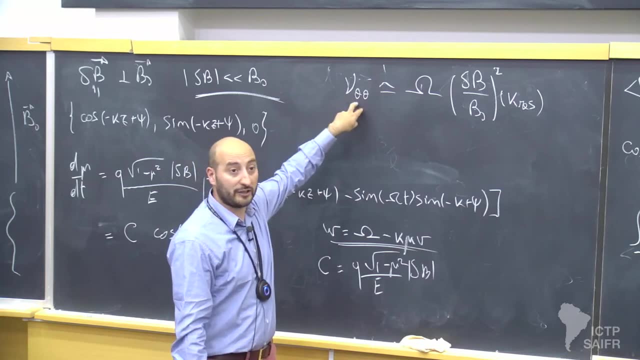 And this is now valid more in general, If you have an ensemble, a power spectrum, for instance, of perturbation in the field, basically the diffusion In angular spectrum, it's the diffusion of the angle And this is now valid in the angular spectrum. 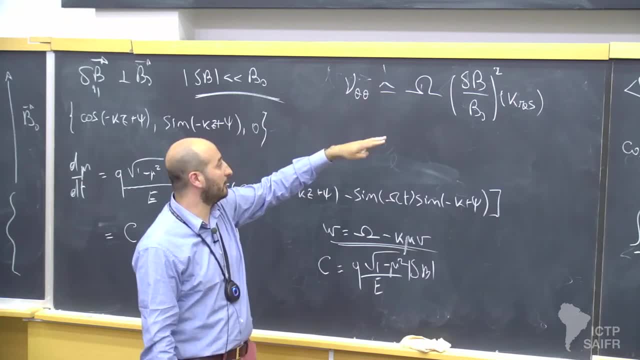 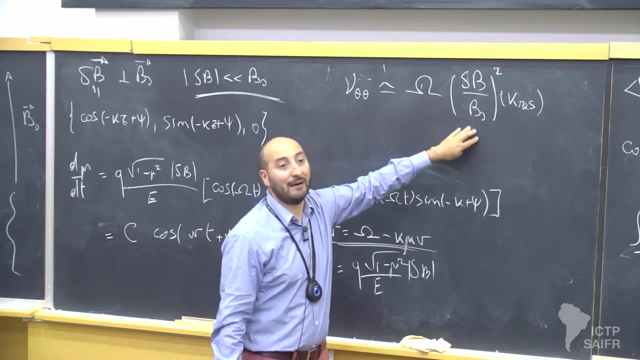 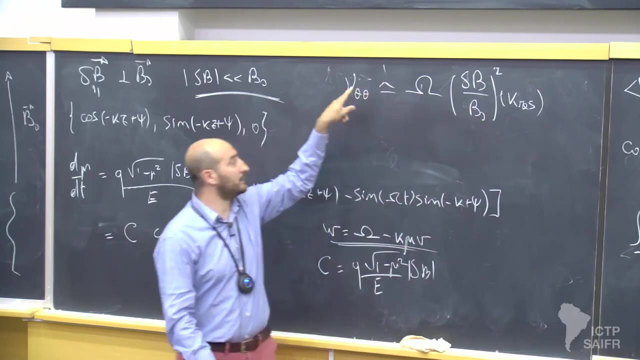 So this is now valid in the angular spectrum. So the diffusion of the angular spectrum in the space is nothing but a multiple, actually sub-multiple, of your fundamental frequency times, the amount of power that your fluctuation has at that wavelength, resonating with the field, with the cosmic ray. 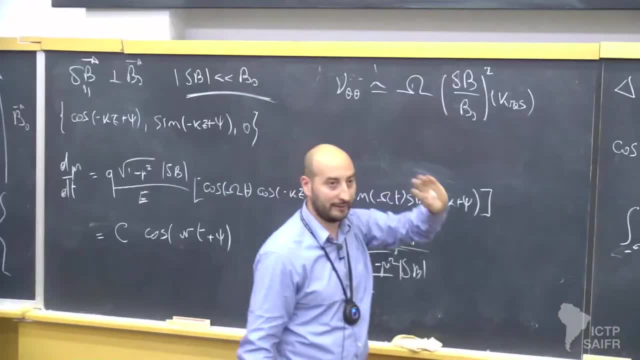 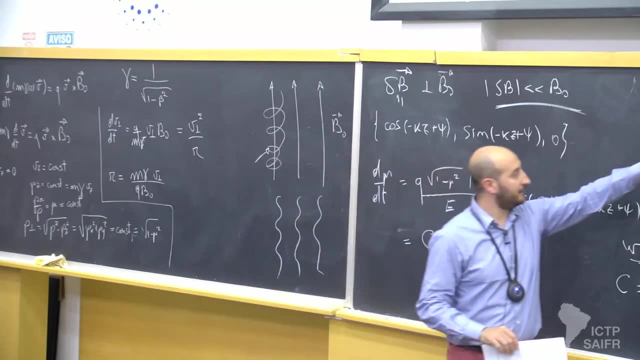 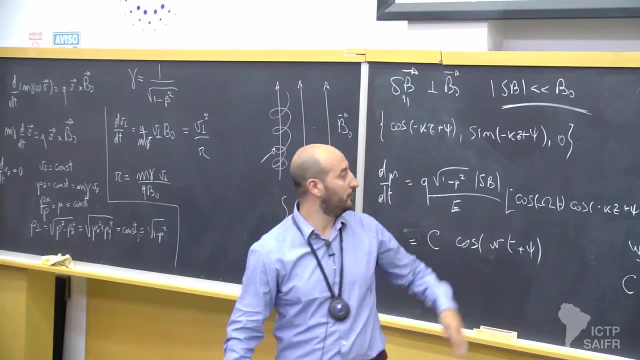 Okay, There are some numerical factors here, of order, one that I won't bother you with. So what that? What does it mean here? It means that basically, the angle of your cosmic ray will change over a time scale which is one over nu. okay. 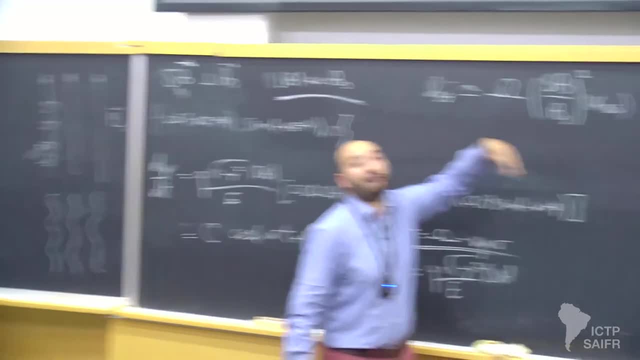 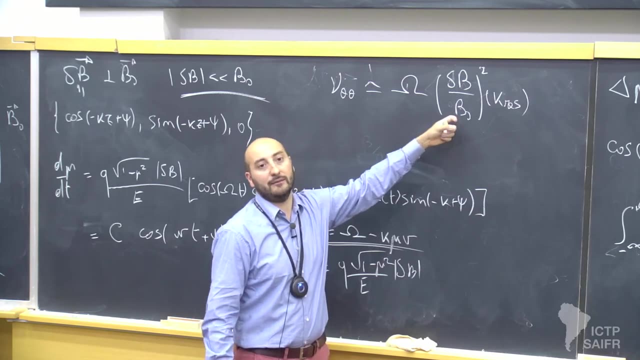 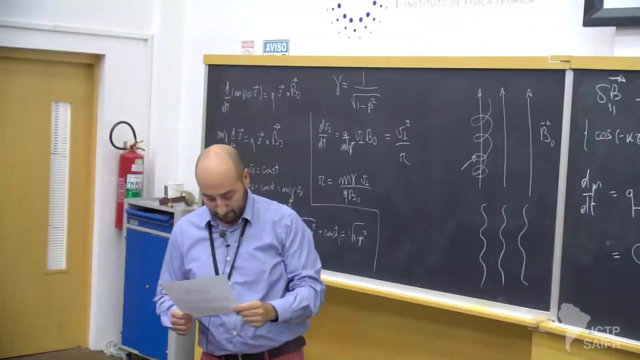 And this time scale is just a factor. a few say larger than the typical orbiting time of your cosmic ray, The factor being much and much closer to unity, the more perturbation there is at that scale. Okay, So this is a very simplified picture of what's going on. 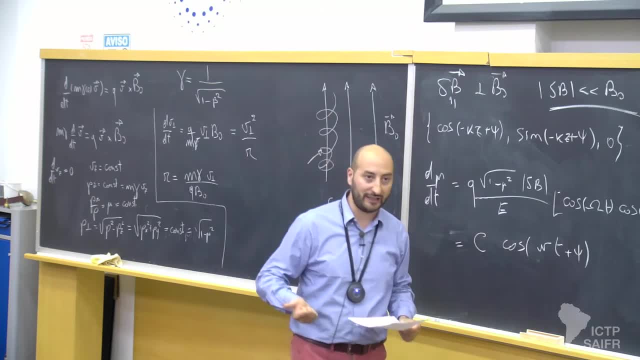 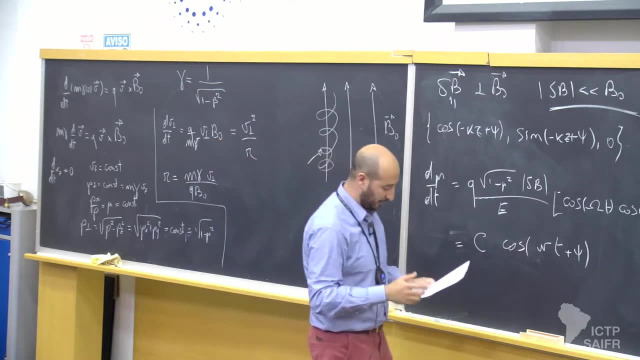 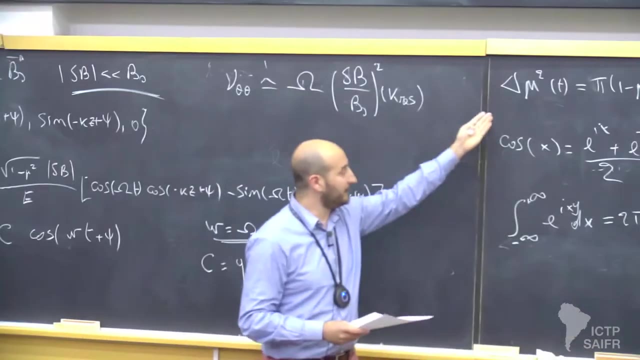 For instance, the propagation is not really exactly resonant. This is just the sort of dominant effect, unless there are special conditions kicking in, But it illustrates that the movement of the cosmic ray is diffusive, with this variance which depends on the amount of perturbation with respect to your baseline frequency. 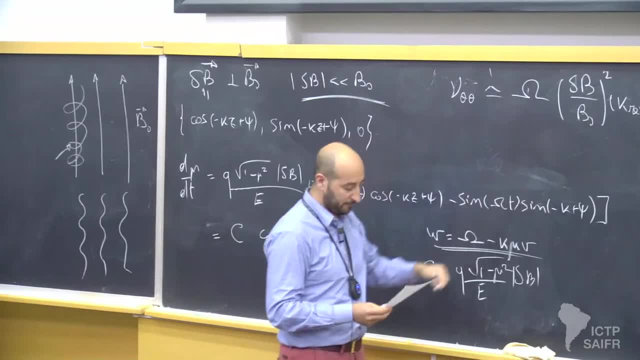 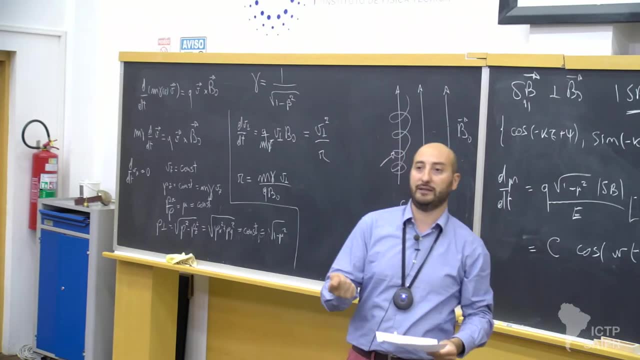 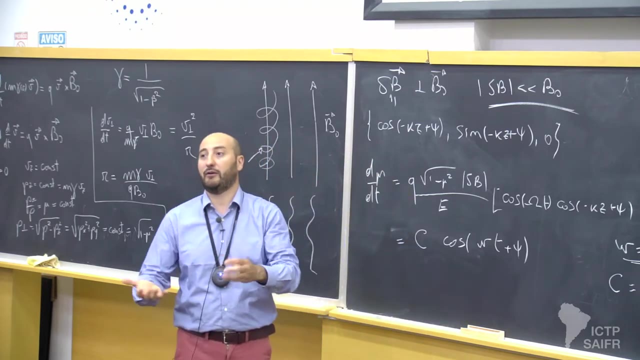 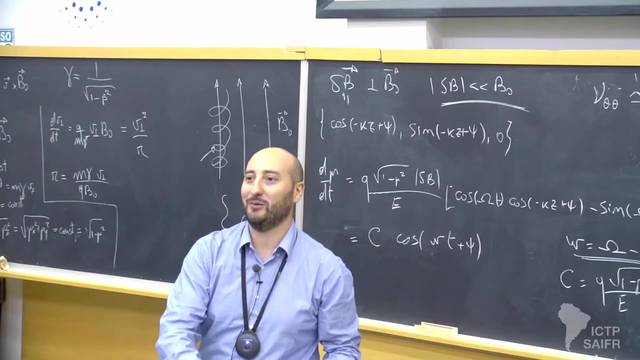 Okay, Okay. So it's a very different type of diffusive movement with respect to what you are probably used to. For instance, if I open a bottle of perfume and I let some time elapse, you will start smelling the perfume that I was opening. 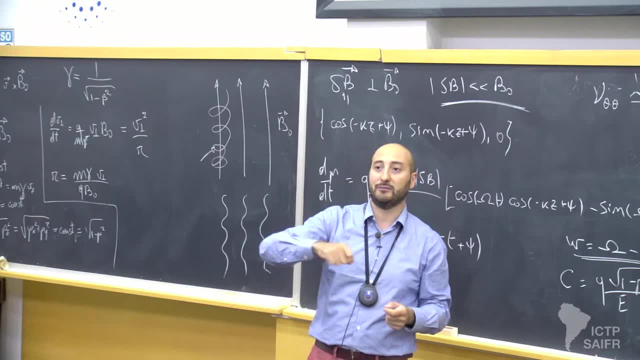 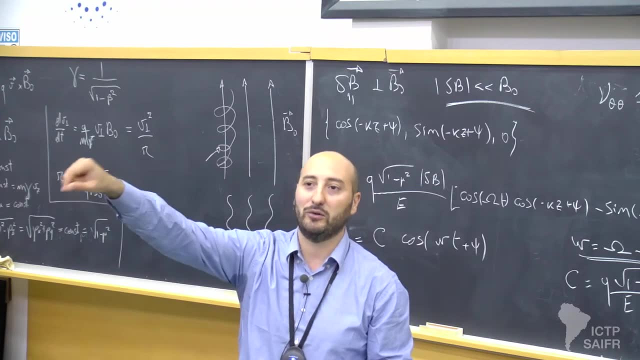 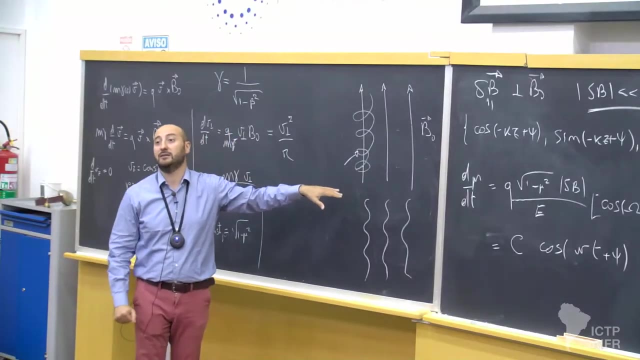 This kind of diffusion is a collisional diffusion. It comes from the slow time, the finite time The molecules will take, bouncing against other atoms and molecules in the air, to get to your nose. This is a diffusion against what? Against perturbation in the field? 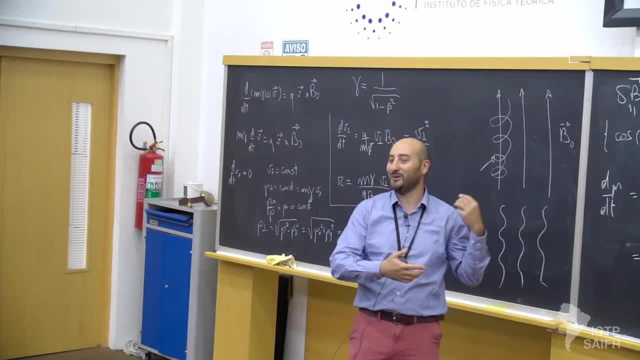 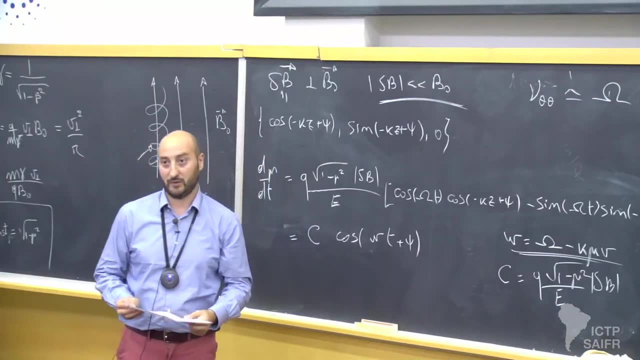 It's not hitting any particle, Okay, Although you could call this quasi-particle in some context. So it's called collisionless diffusion. Okay, And this is the basic motion that charged particle experience in the magnetic field. Okay, And this is the basic motion that charged particle experience in the magnetic field. 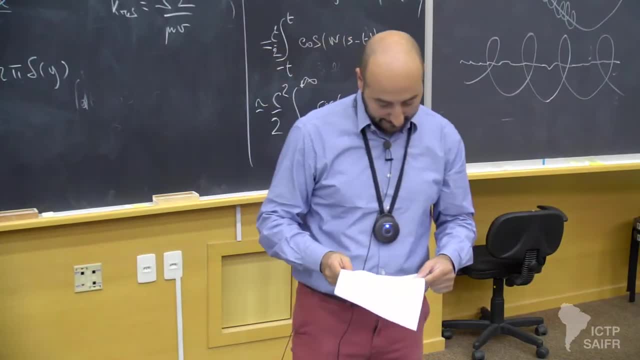 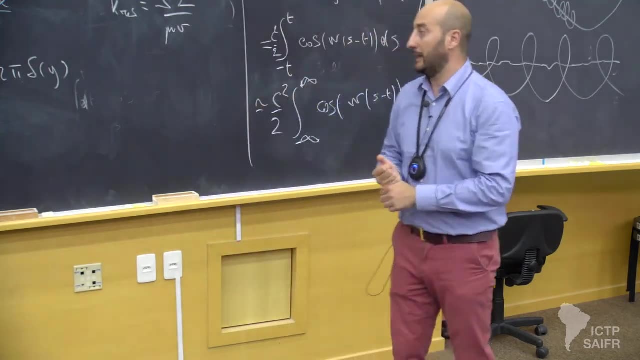 And this is the basic motion that charged particle experience in the magnetic field. Okay, And this is the basic motion that charged particle experience in the magnetic field, For instance in the galaxy, And, as Pasquale was mentioning before, actually there is empirical evidence which is known. 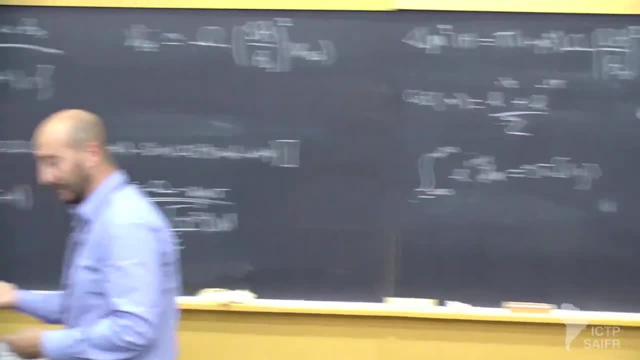 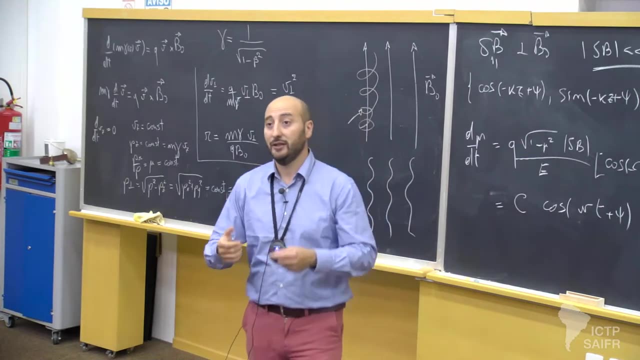 since very long time that this is the kind of stuff that happens in the galaxy coming from the observation of boron, beryllium, lithium or sub-iron abundances. you see that the typical timescales inferred for this element are very similar. 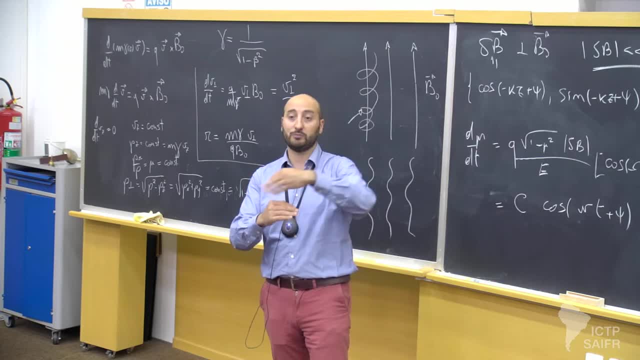 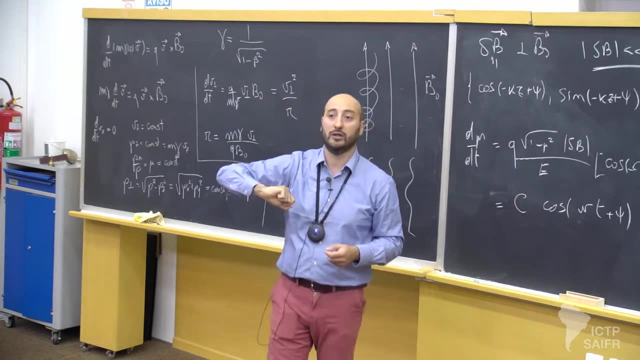 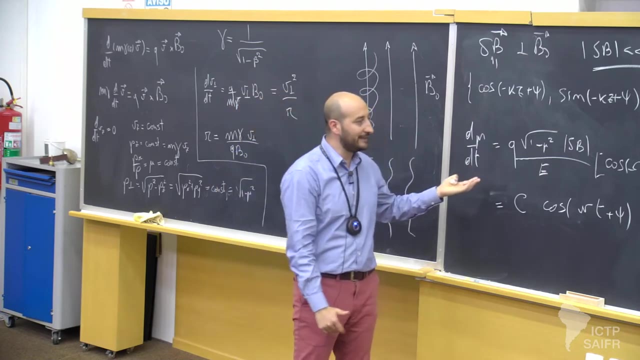 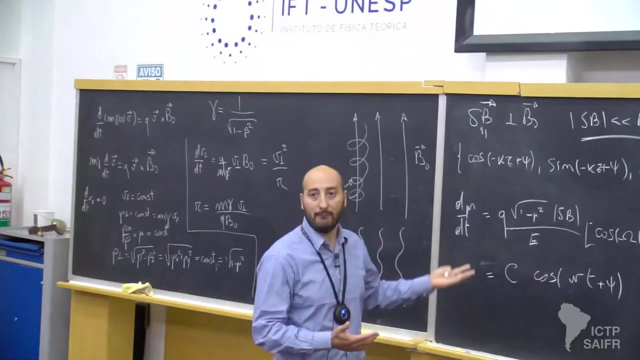 So it makes sense to model it in terms of a diffusive process and we see that quite elementary considerations tell you that actually you can get relatively easily a motion of this type for a charged particle, a relativistic charged particle moving through a perturbation. 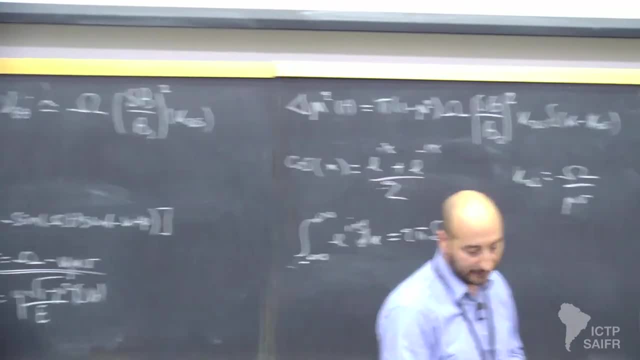 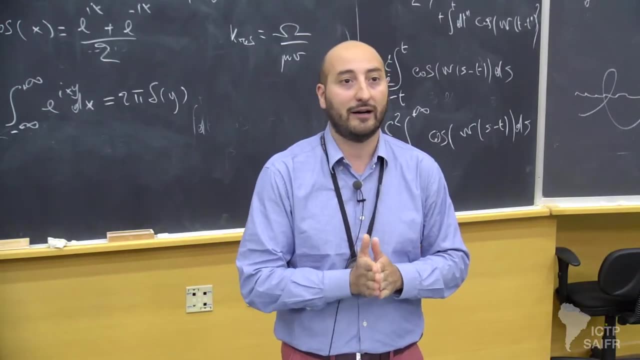 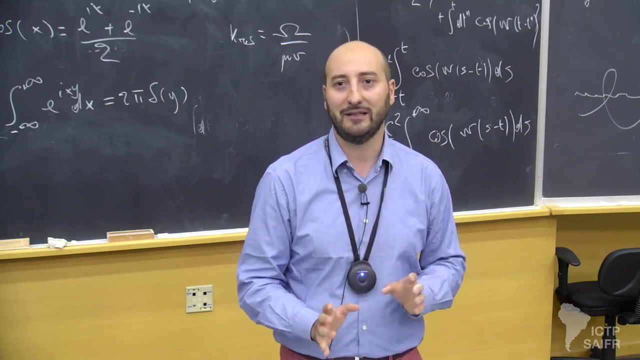 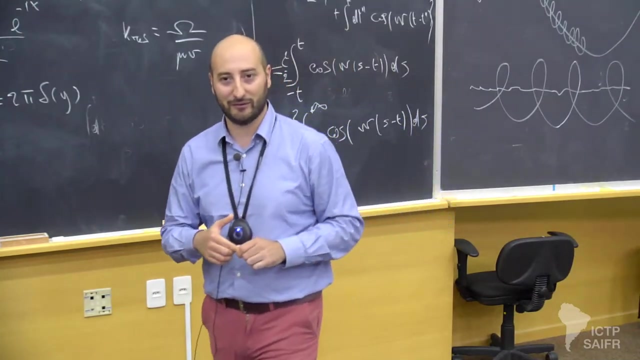 Okay, So I think I can stop here for the first lecture and I don't know if there are questions or doubts, but if you have some points which are not completely clear, but the whole picture is, I invite you to have a look at the notes and maybe come back to me after you have read. 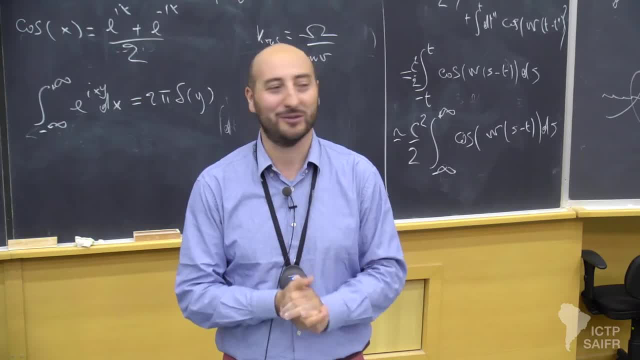 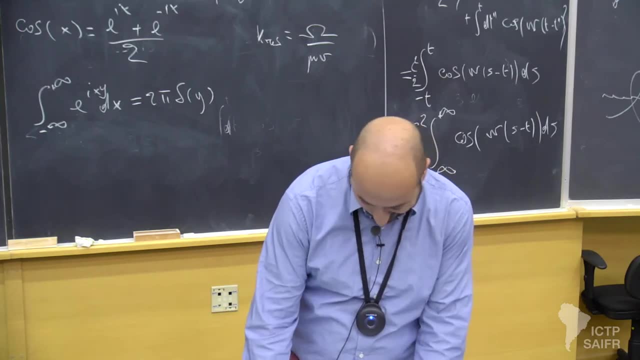 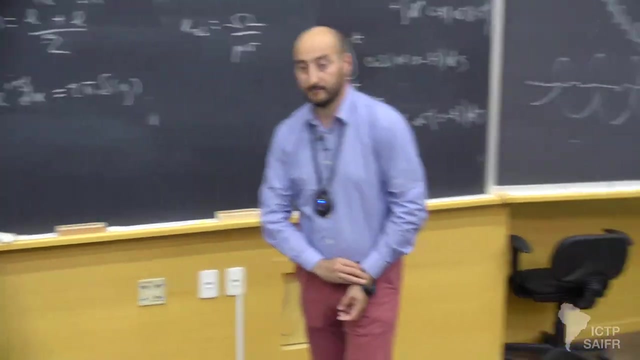 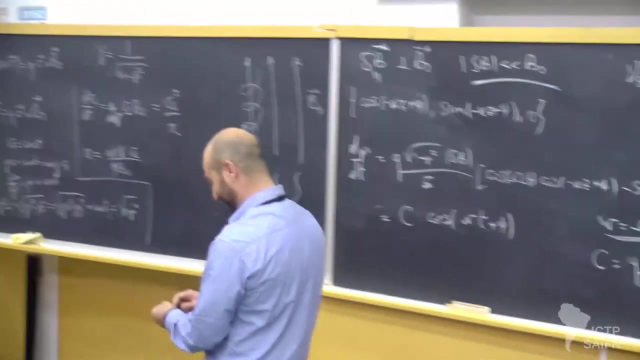 the notes so that perhaps this will show How to say Dissepate: naturally Okay, naturally okay. thank you, nonetheless, there is some time for a few questions. if you have them now, you want to add something, this is gonna be nice. just just a. of course, everything has been said already, but just it's interesting. 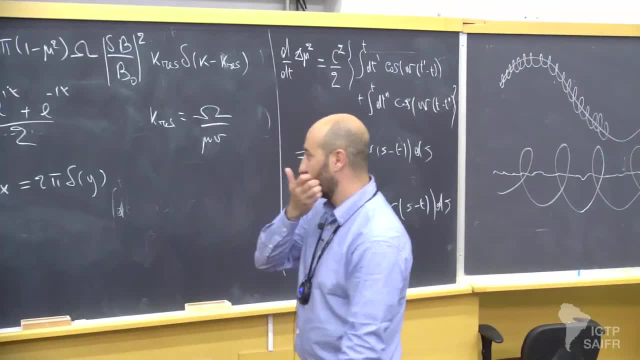 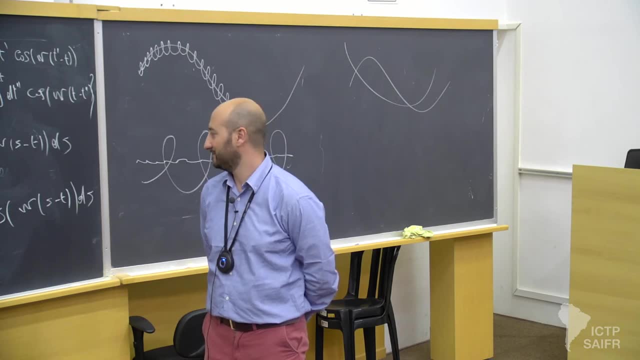 that if you use this expression that Pasquale wrote, and you can ask yourself- you know, I put the numbers in- and then you want to ask how long would it take to have a deflection of order, unity of this thing, and you do it for typical. 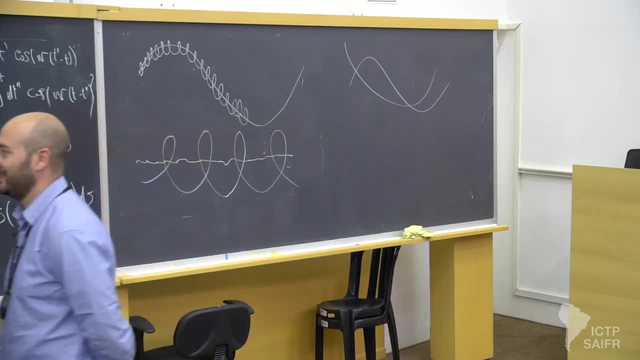 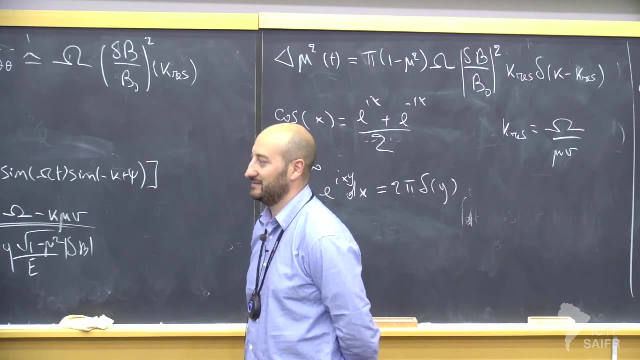 parameters of the galaxy, you need this number to be of order 10 minus 6. so the perturbations that we are asking about is a pastor, 10 to 10 to 4. say yeah, then to 3, 10 to 4. so it's tiny correction and it. 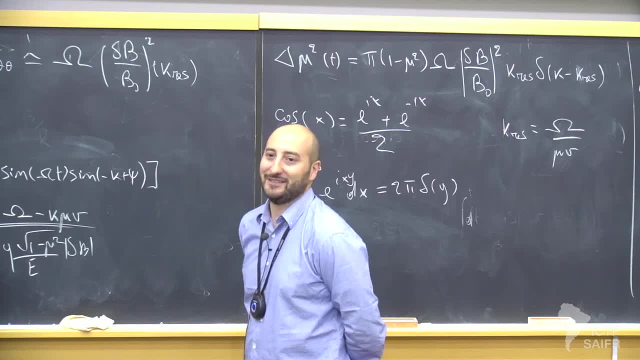 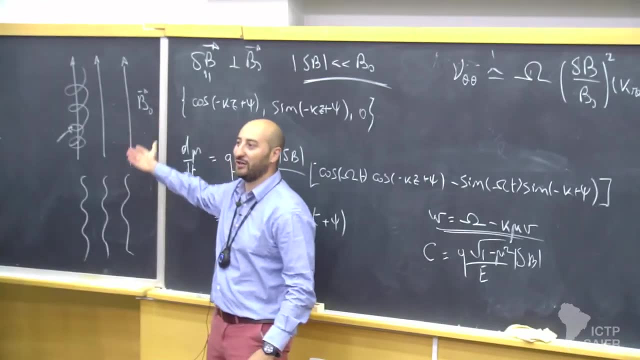 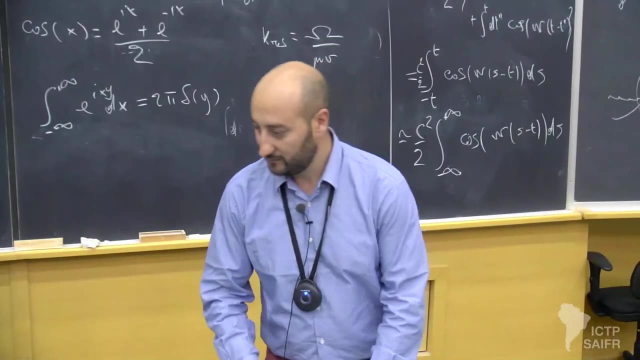 leads to a gigantic effect. so basically, there is almost. it's almost natural to expect that it will propagate diffusively. you have to arrange for unrealistic natural fields to not to not to generate this kind of motion. and again, in terms of numbers, Pasquale described this: 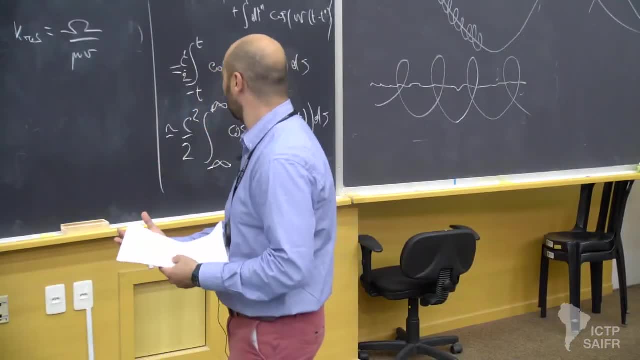 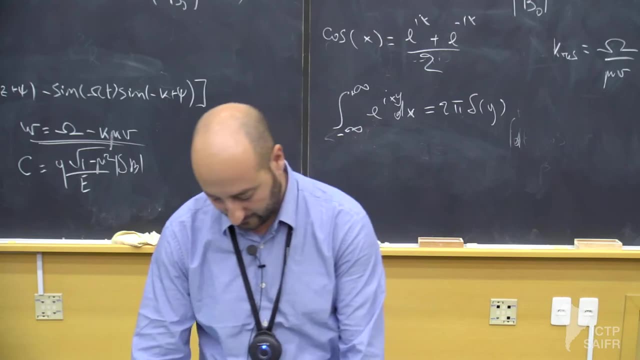 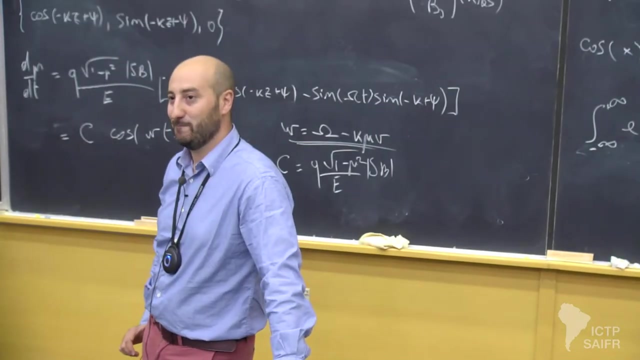 the random motion, the random interaction in the beginning of is the talk of this lecture and again you can ask yourself if you use the parameters that Pasquale's gave you. it's now a race, but say one particle per cc or cubic centimeter in the galaxy and ask: 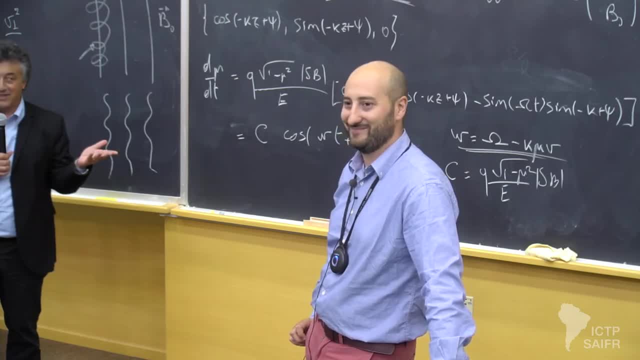 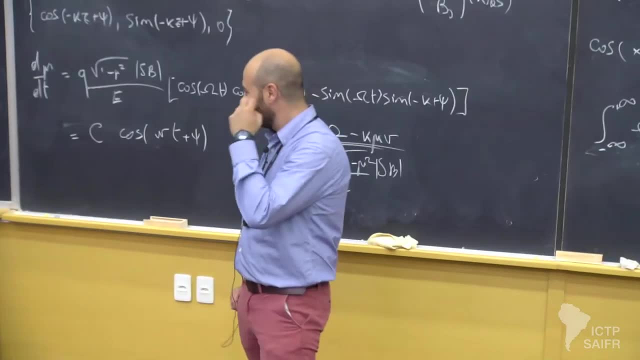 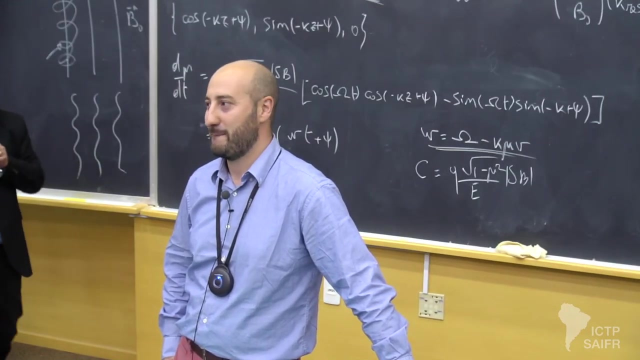 yourself how much would it take for diffusing on that scale, and you will easily find that it scatters the first time on andromeda. so an effect of one part out of 10 000 on the field leads to a gigantic effect, and collisions are totally, totally relevant in this business. yeah, 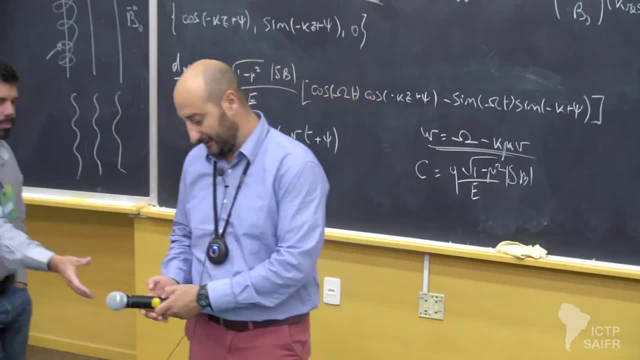 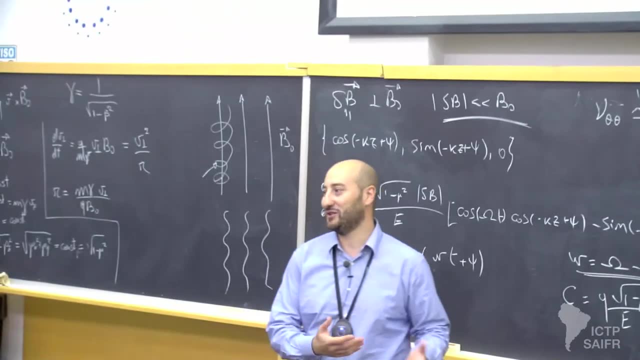 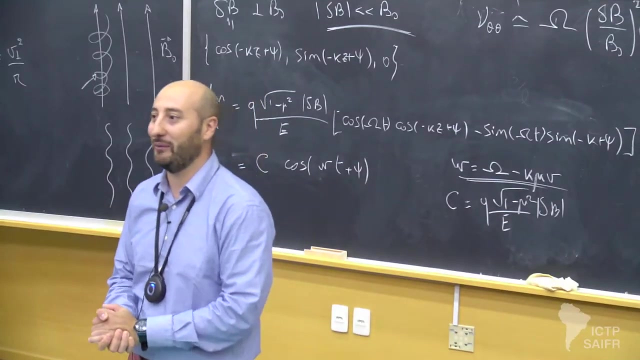 yeah, yeah, it's, it's perfectly correct. so this is another manifestation what i told you. so the conditions in the galaxy are so different from the conditions on earth that what is the only type, basically, of diffusive process that you experience in typical phenomena on earth is not going to. 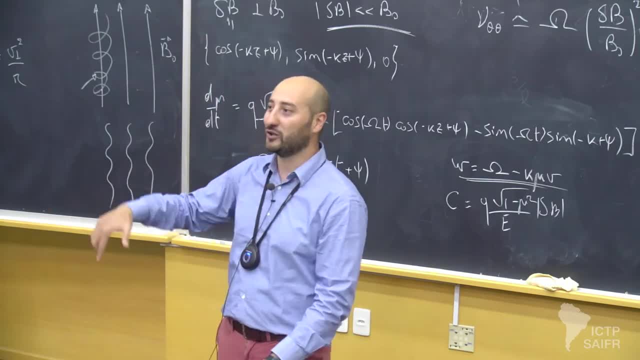 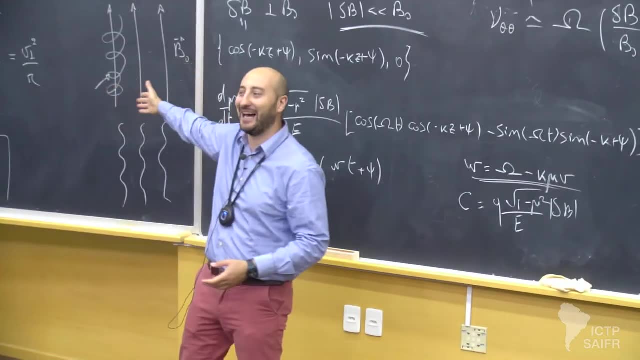 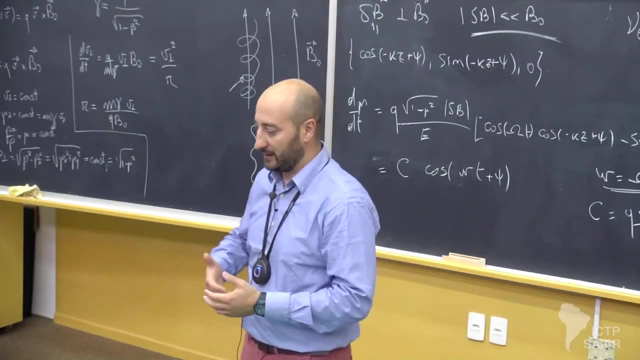 happen at all in the in the galactic environment. on the contrary, a type of of phenomenon that you have to work hard to reproduce in the labs on earth happens, happens quite naturally in in in our galaxy. it's not only related to that, but actually to more broad class of. 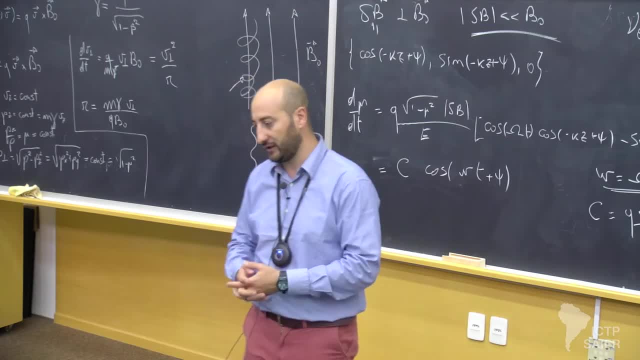 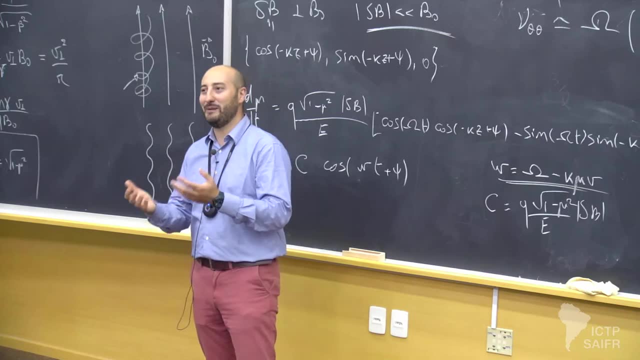 programs in physics. actually there is a whole branch which is sort of laboratory plasma astrophysics, where people try to emulate some conditions which are very, very, very hard to to encounter in normal life you, and which seem to be very typical, on the contrary, or astrophysical objects. so there are many efforts. 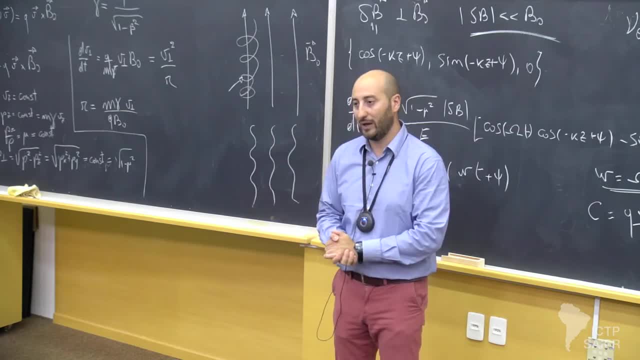 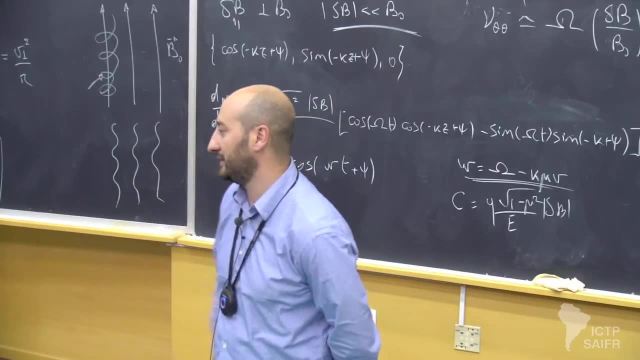 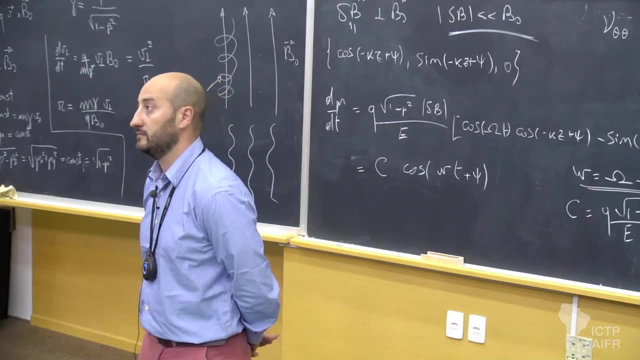 in plasma, in plasma physics, trying to, to, to have a laboratory counterpart of many of these ideas. so i i'm not an expert on that, but just to mention that this is a very, very active field of research. there is still time for one or two questions. don't get intimidated. did i intimidate? 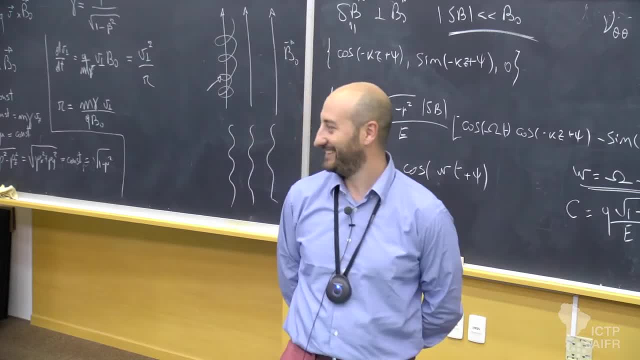 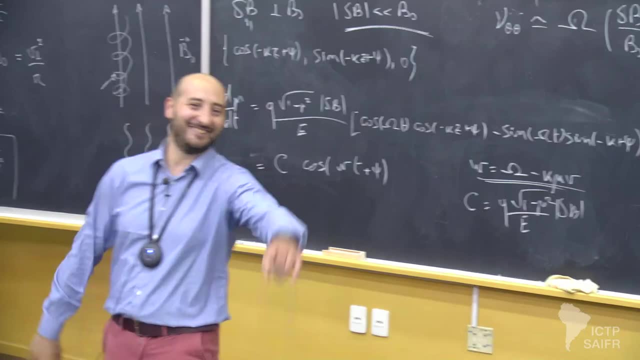 no, i don't think it's you. come on, otherwise we're not good. there is a one question there: you are the hero that is sending everybody to lunch, otherwise you would know you, there is you to take them to these labs and you take them to other places. 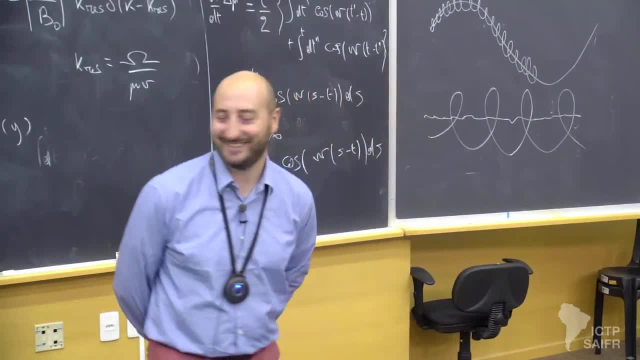 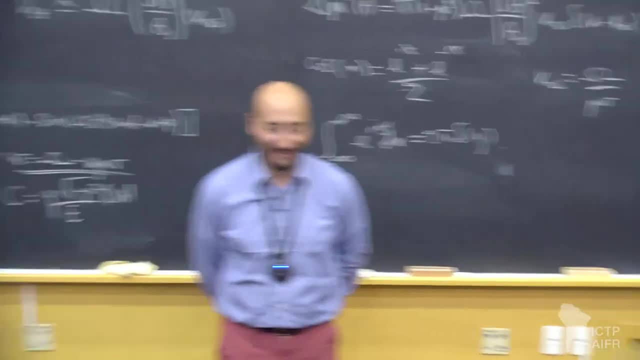 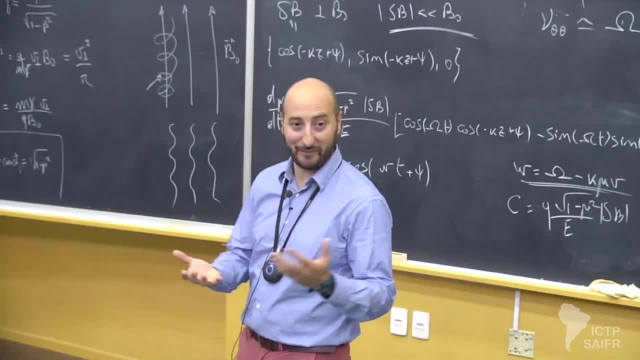 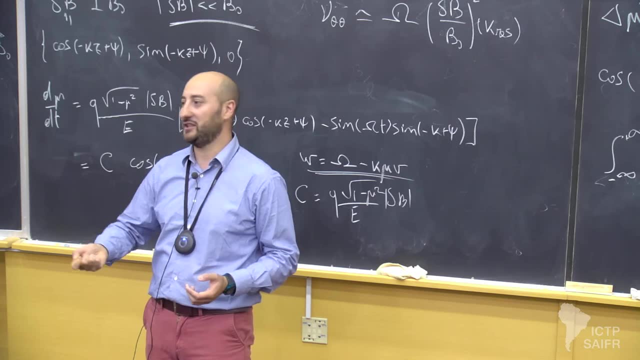 okay, as i said, i'm not an expert on that. one of the key issues in a in a practical environment room wool gay in a practical environment in the lab is that you must be sure that there are no collisional targets at a density which is disturbing your whatever collision. 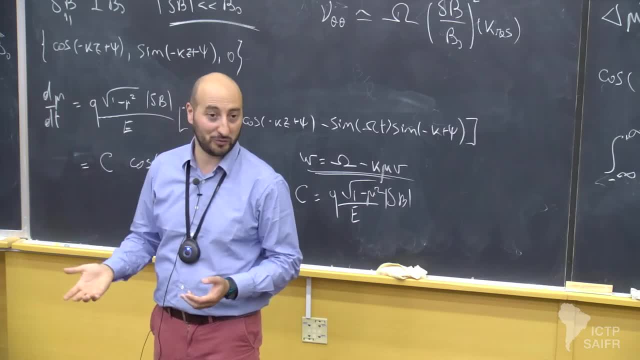 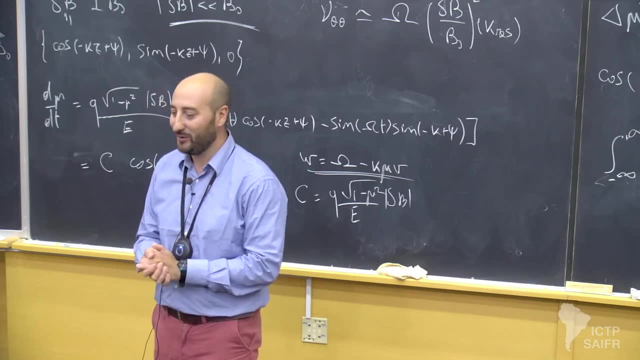 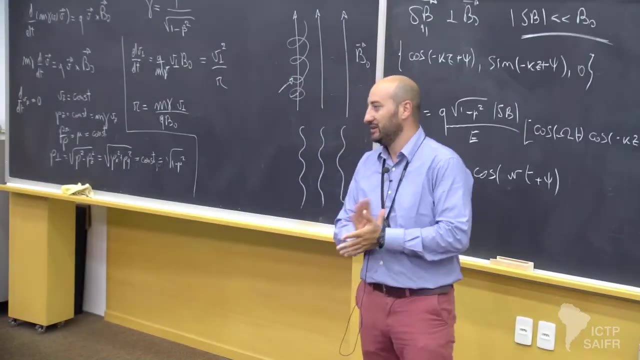 less system you want to study. so in general they only last for a very short time. that's what I know. so I think it's the past the last 10 years or so that this has become sort of realistic. but again what happens is that you lose your. particles, because they start hitting impurities or residual gas senior in your system relatively fast. so this is, as far as I know, the most limiting, the practical limitation of your reproduction. on the other end there are others, so for instance the high temperature could be a limitation in some cases. 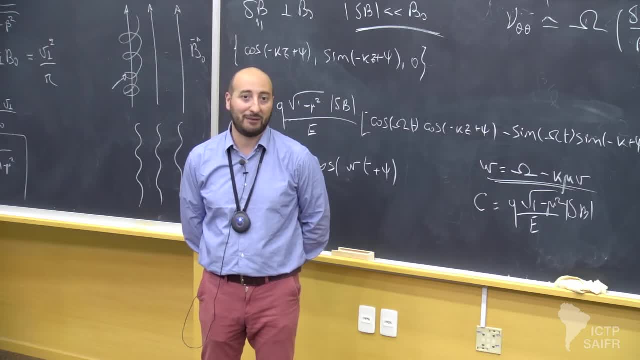 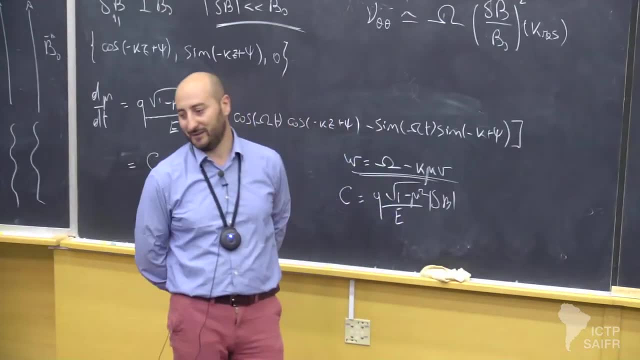 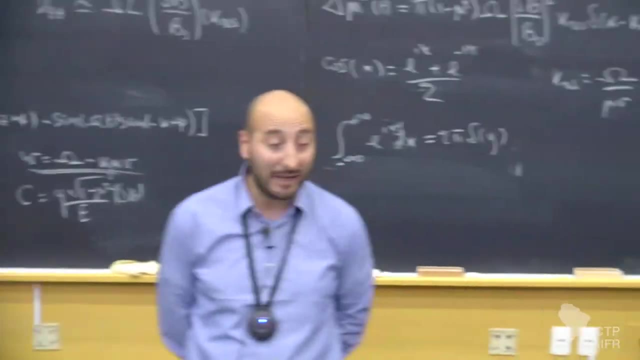 I don't know. Of course you must use some rescaling, because the field strengths we are talking about here are very, very low. So you must have some rescaling of your values. But apart from that it might be OK. another difference might concern the type of plasma that you might want to consider. There are astrophysical situations where you have electron-positron plasmas and this is not so cheap and easy to reproduce in a terrestrial one. So, OK, it's not a one-to-one correspondence. 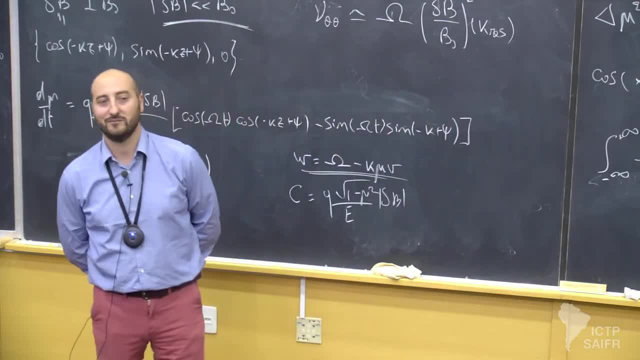 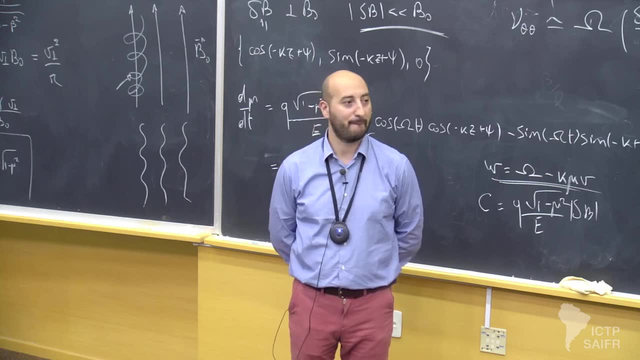 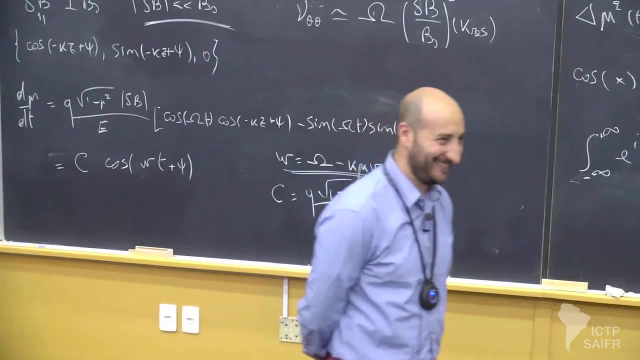 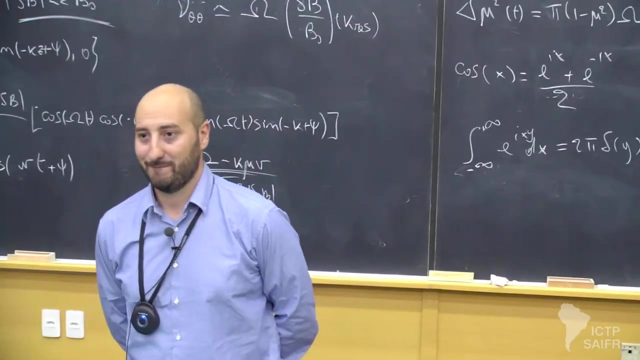 but yeah, there is some. One more question. We're not leaving by the time that the class is scheduled to leave, so you better ask a question. So how well do we know the magnetic fields and the anisotropies? 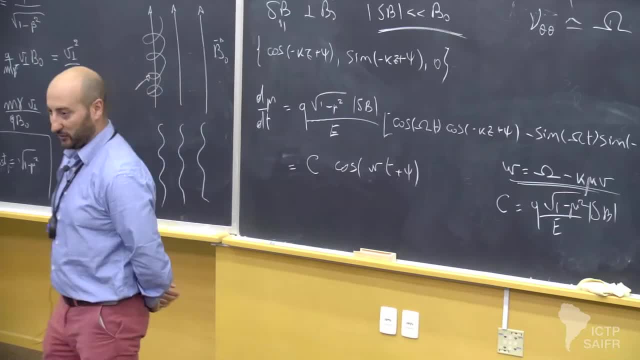 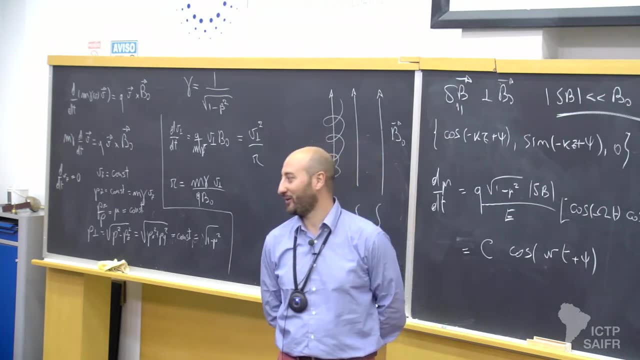 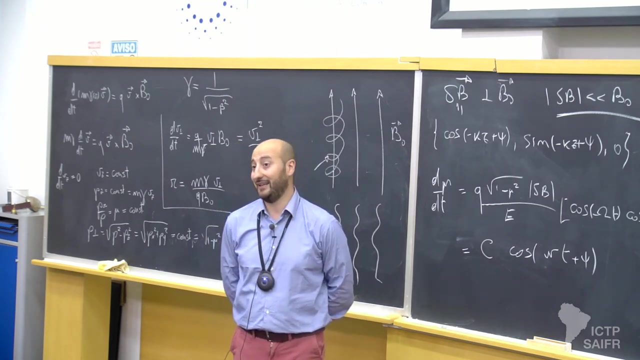 How do we measure it? OK, very, very good question. So the answer is quite badly for any reasonable person on Earth working in a field different from astrophysics. On the other hand, compared to other fields like the extragalactic space, et cetera, 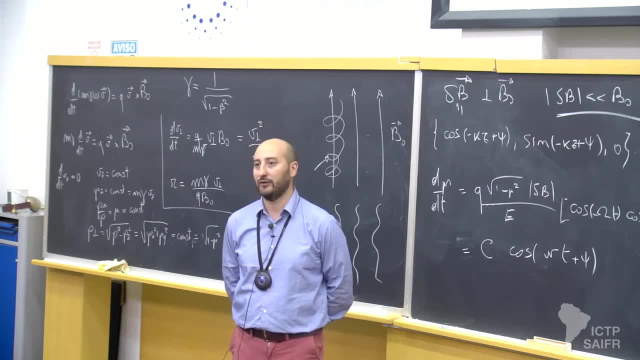 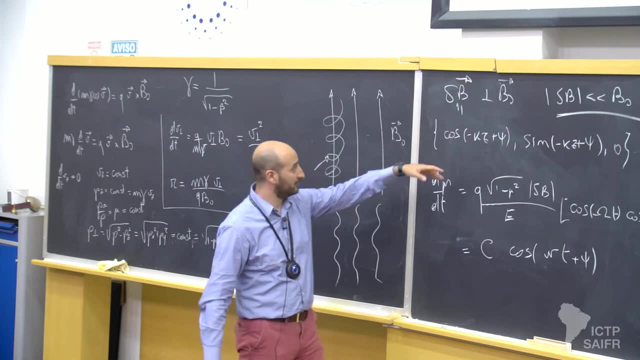 we have some idea of, let's say, what the magnetic field of the galaxy is on, say, kiloparsecs case. So the regular field, this B0 here is. first of all, it's not really a homogeneous field. 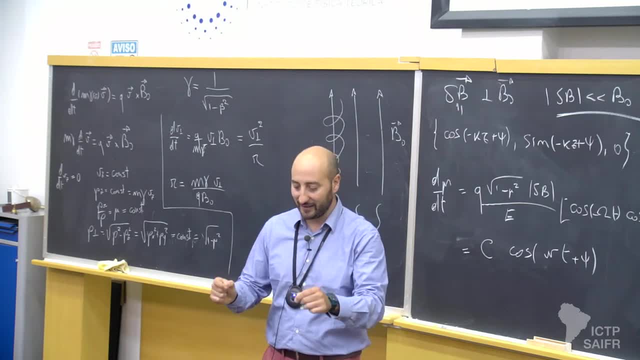 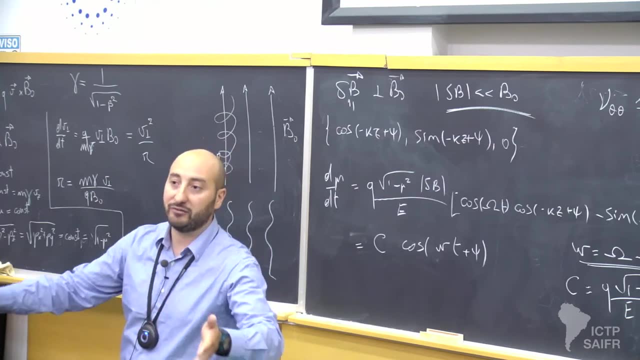 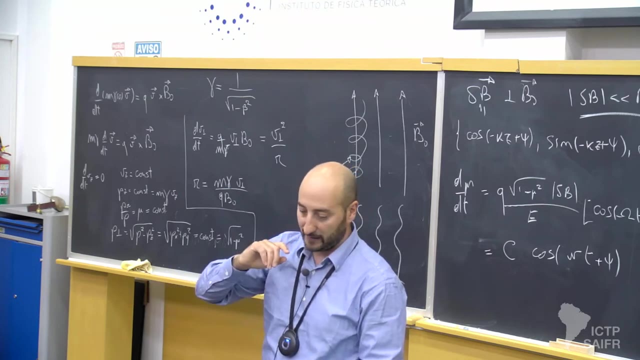 What I'm talking about homogeneity here, is homogeneity on the scales of interest for this microphysics to happen, So over hundreds of parsecs, it does follow, for instance, the spiral arms, the field in the disk. On the top of that there are perturbations. 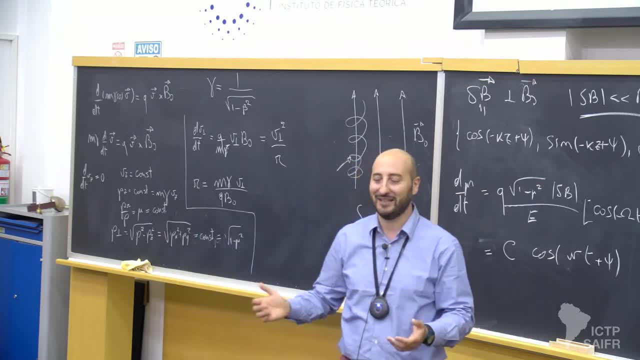 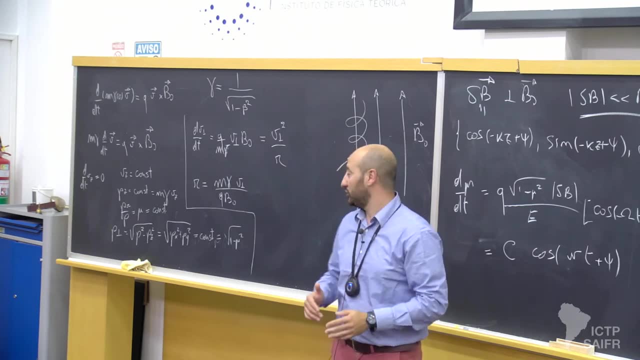 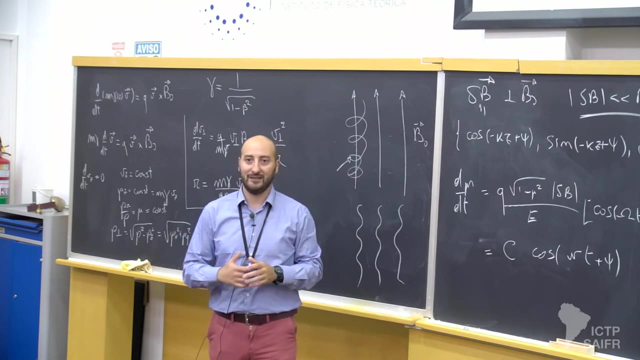 there are fluctuations. turbulent field is typically named The turbulent field, however, is turbulent on many, many scales. OK, So the tricky part is to know the turbulence at the right scale here. OK, So at very, very large scales actually. 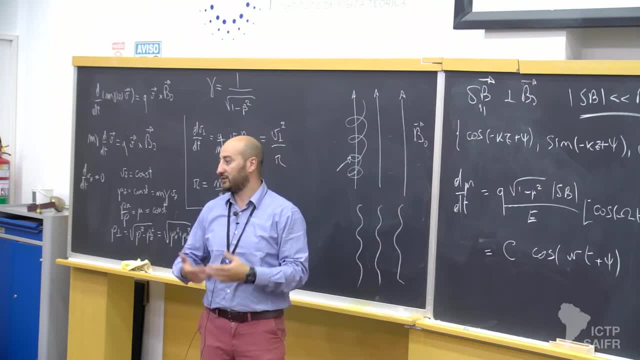 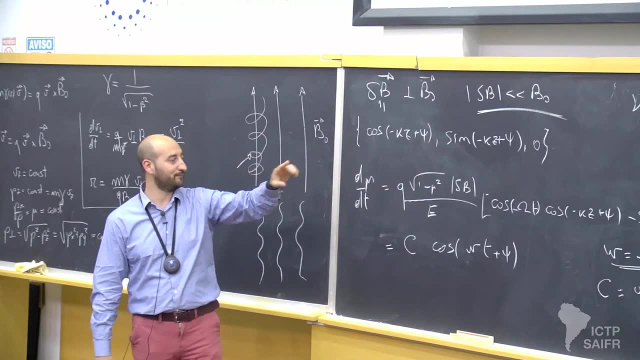 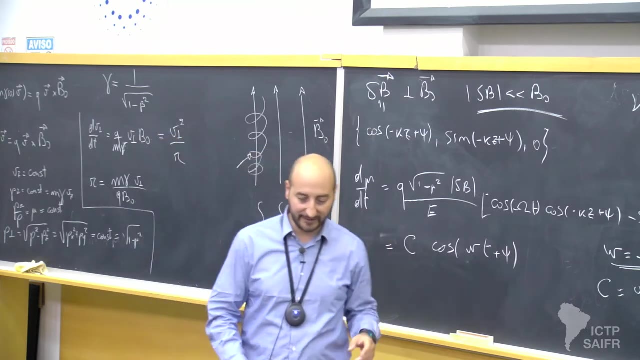 the delta B over B is not small, It's of order. maybe one, OK, at very large scales, At low scales in- let me get this right- in low scales, in physical space, not in key space, large key. there are some informations, I think from scintillation. 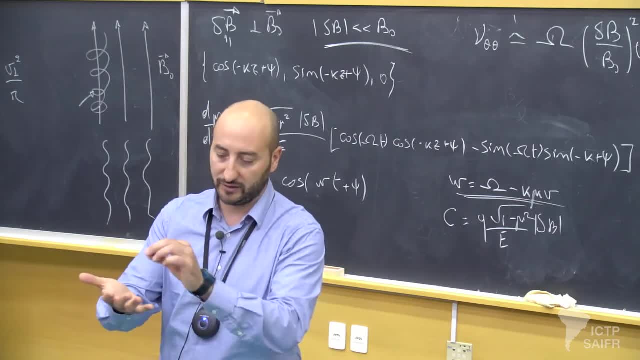 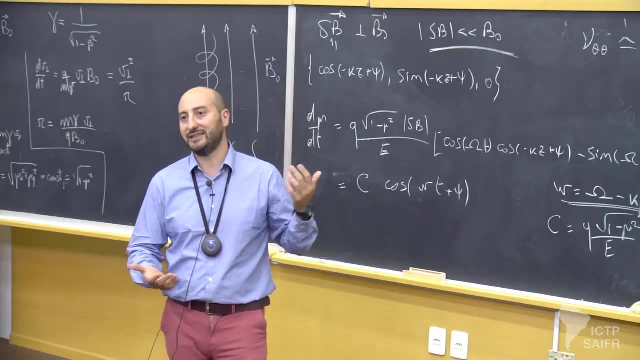 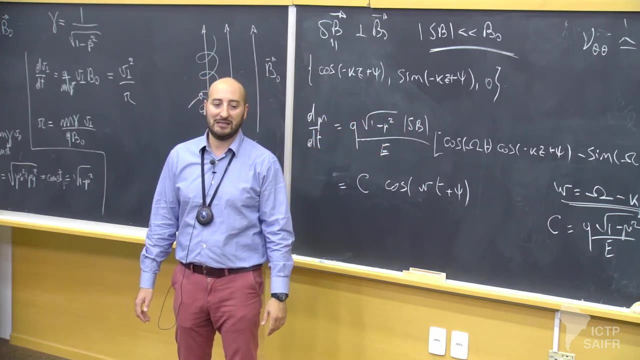 from probes of the interstellar medium, and some of them are, as far as I know, are consistent with this delta B over B, which is below one, Well below one, but non-vanishing, Actually, for phenomenological studies. 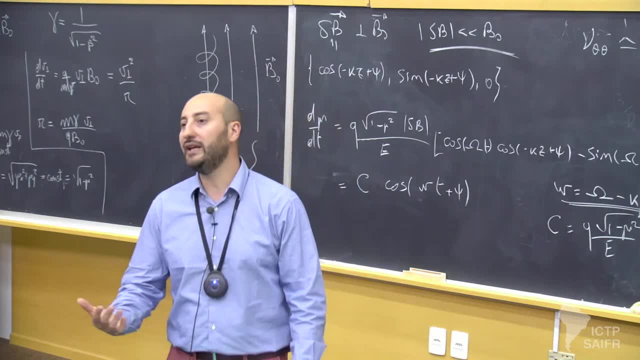 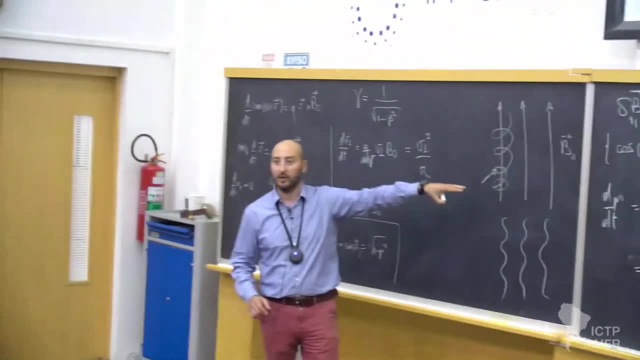 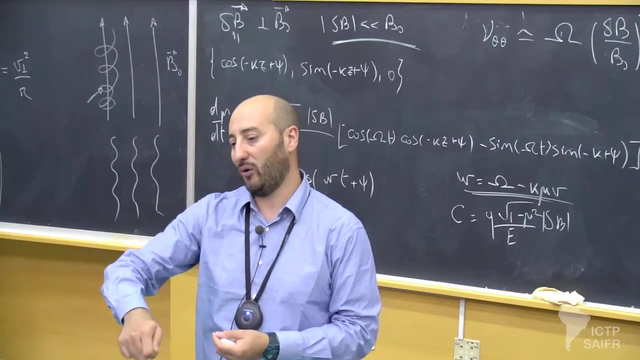 this is something I will come back later on. You don't really need that because, in any case, you are not going to describe a situation very close to this. You are going to describe a sort of average diffusion over something that maybe is the sum of many macroscopic domains. 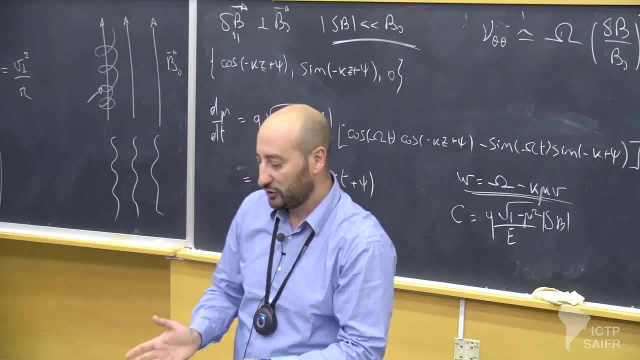 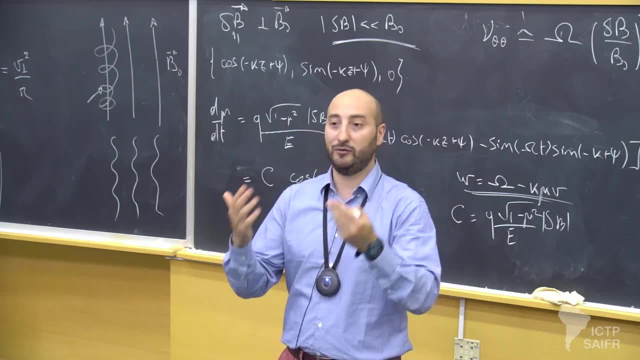 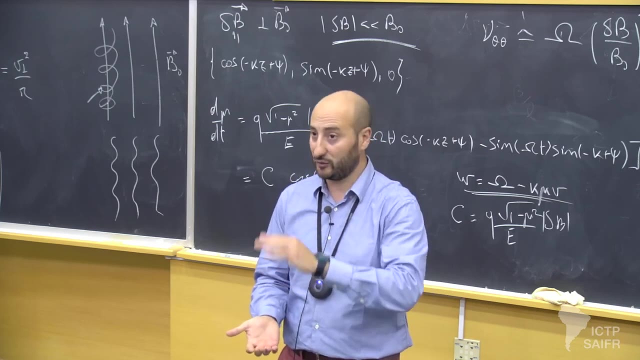 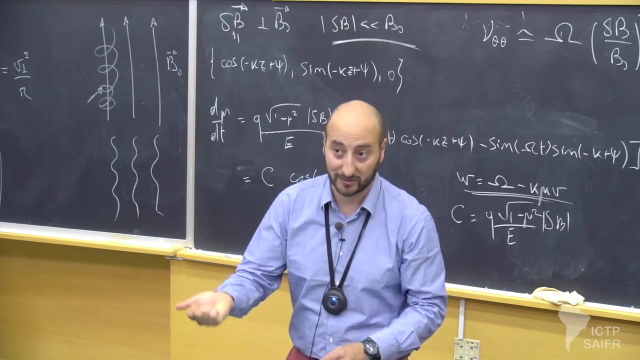 each one as a regular field. So you will get a sort of isotropic average diffusion coefficient, which is a macroscopic object, is a phenomenological object which is very hard to link to the microscopic, strongly anisotropic diffusion tensor, because it's a tensor in general. 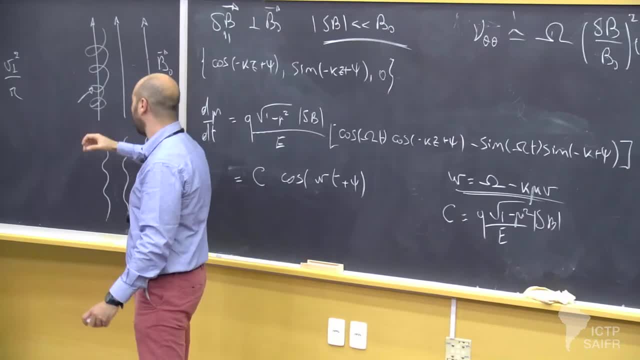 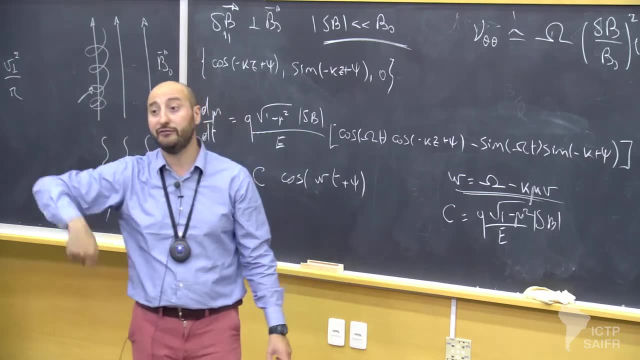 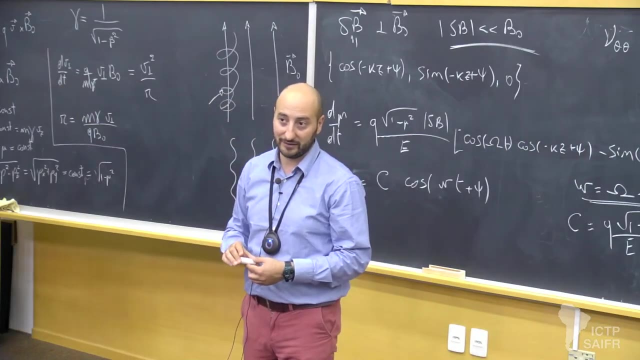 You see immediately here- but one can argue more in detail in the next lecture- that in this model the diffusion along the field line and the diffusion across the field line are very different. So it's much more efficient in one way than in the other. 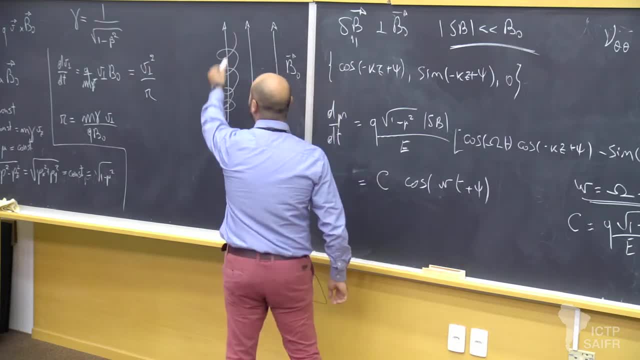 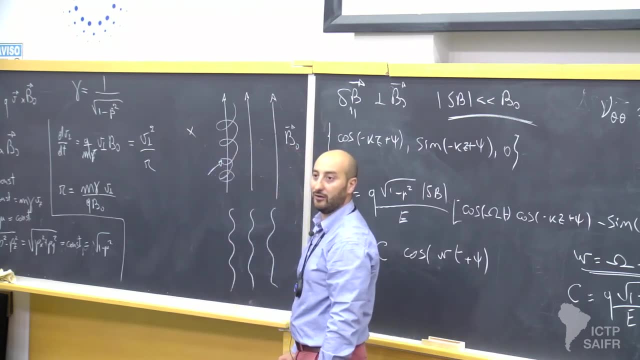 And so if we were, had we been in such a situation? okay, so let's say that we are here and this is the real configuration of the field. well, you know a source here of cosmic rays. we would never see it. 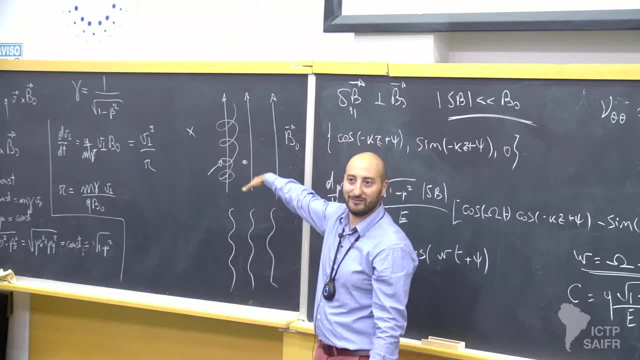 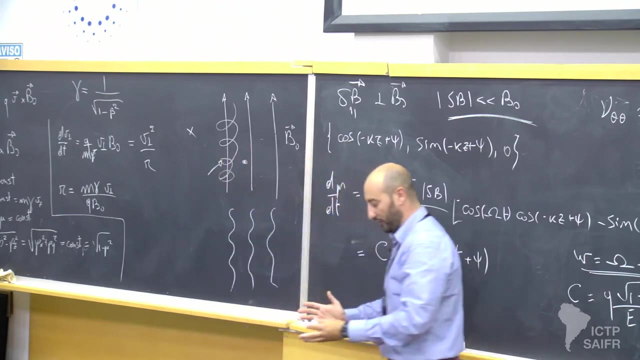 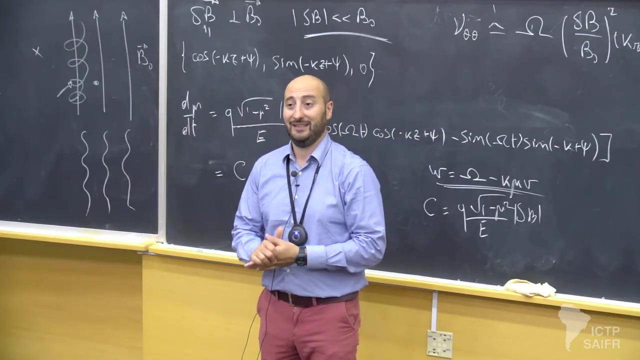 We would never see anything like that, because the time scale for this orthogonal propagation is much, much longer. So the true situation is that there are field line connecting and turning over scales which are typically of 100 parsec, and the fact that we see roughly isotropic cosmic reflux is another. 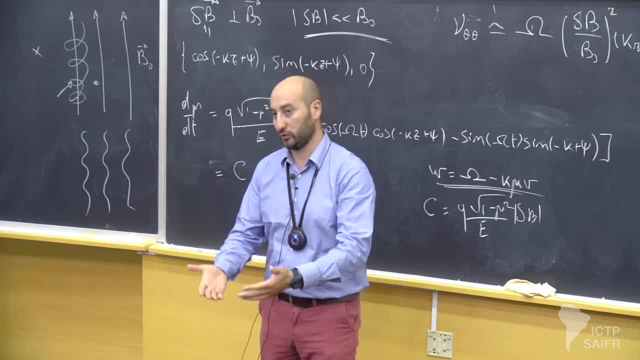 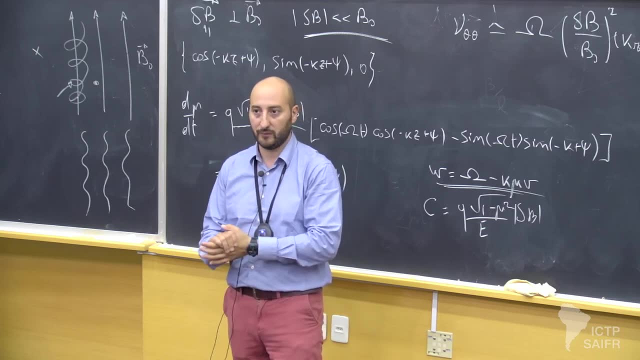 way to infer that Most likely there are many sources contributing to the cosmic ray that we see on Earth. Otherwise, we should see some anisotropy. Okay, You would see completely isotropic here Here. yeah, but probably you would see nothing in the center. 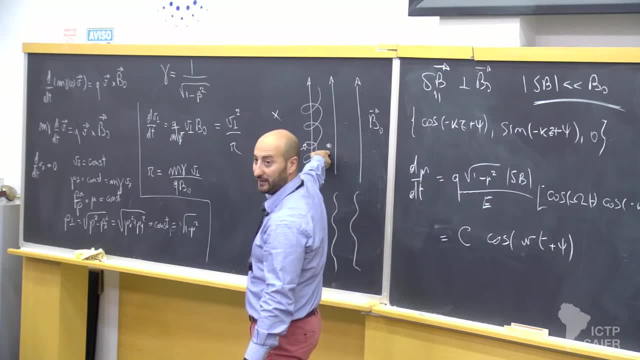 It depends on the numbers. This is a sketch, But it could happen that the time scales for okay. there are two problems. One is to assure isotropic flux, The other is to make sure that say the diffusion time scale. 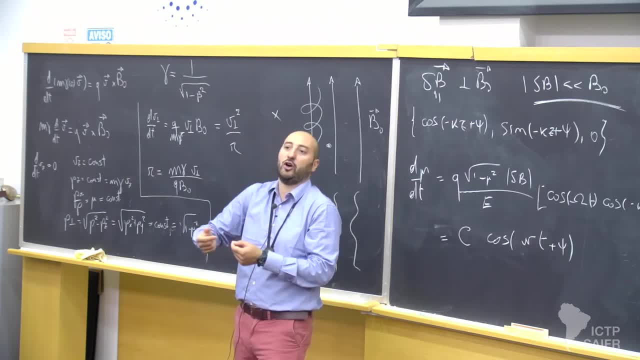 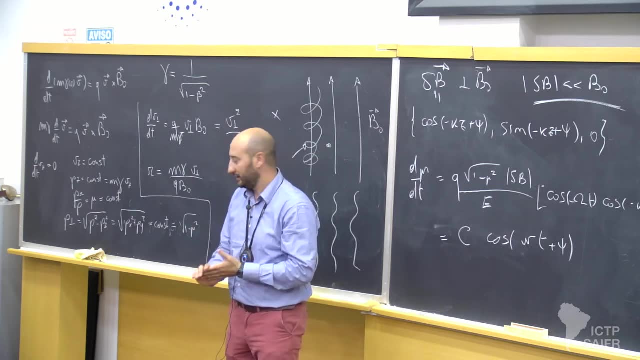 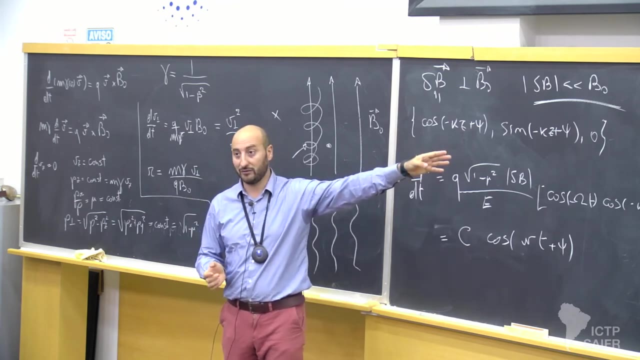 from a source to you is shorter compared to, say, the lifetime of your source or the lifetime of the galaxy or whatnot. So these depend on what happens to the, both to the microscopic fluctuation around the regular field, but also on the shape. 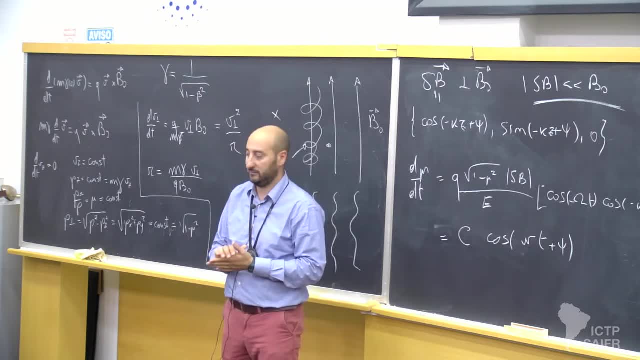 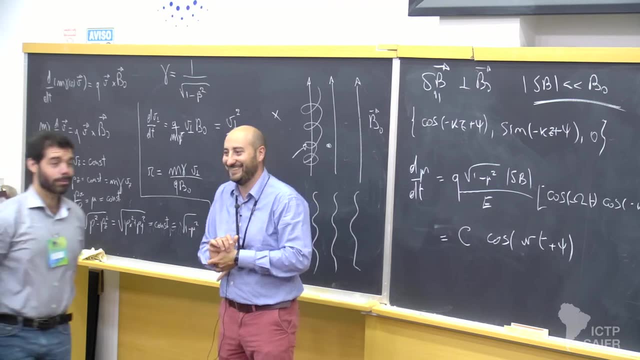 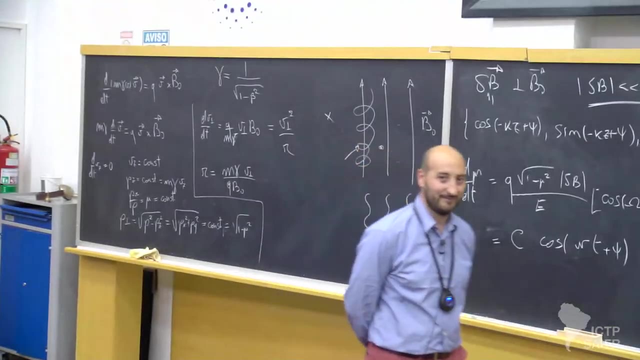 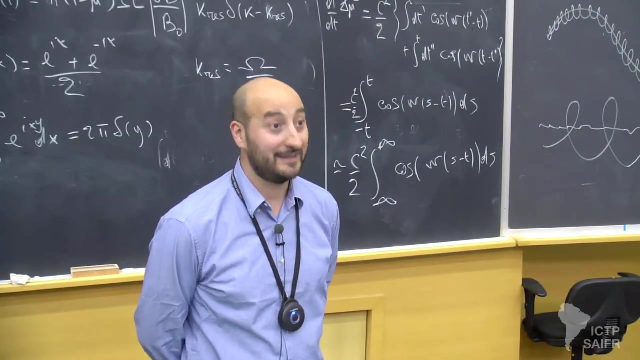 of the regular field around you. So Do you feel like taking one last question and keep the answer within three minutes? Yeah, It depends on the question. The displacement of the particle is thought as a current Produces another magnetic field. Can it be thought as a new perturbation? 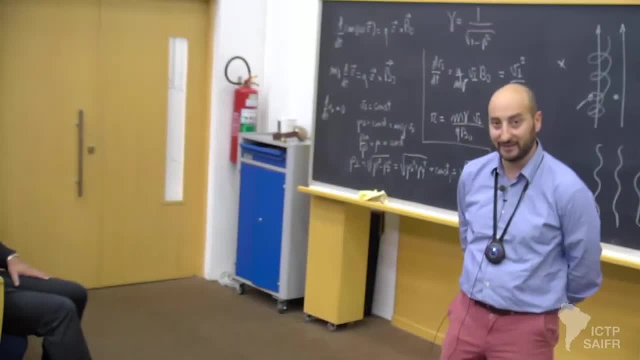 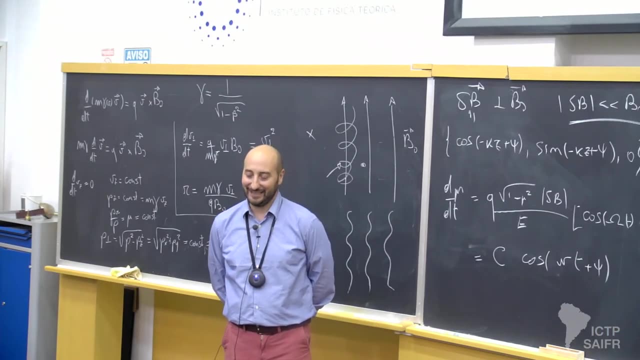 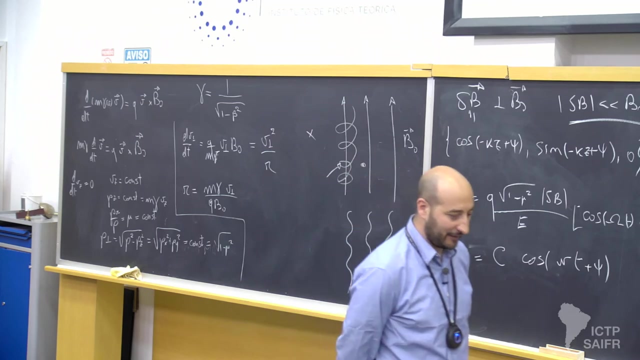 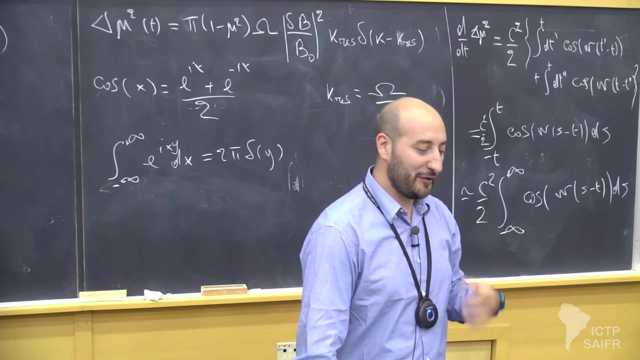 Yeah, In general, cosmic rays do produce a current, And okay, So we will see next lecture more in detail. that, okay, there is a typical current associated to the. this is the movement of a single particle. okay, First of all, there is one complication. 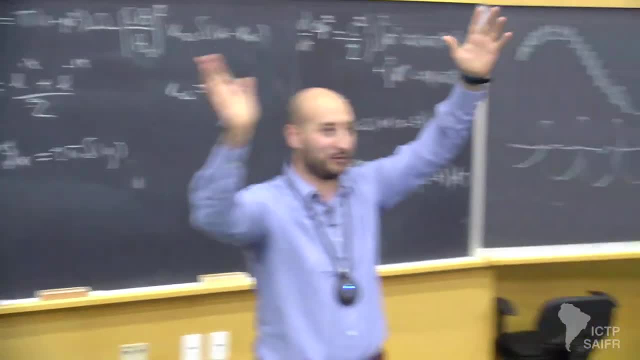 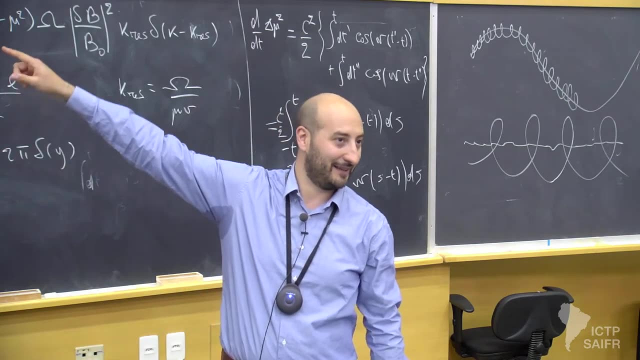 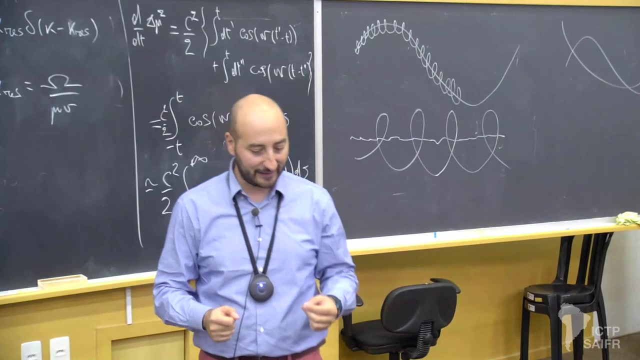 that in general, you will have particles coming from many sources all over the sky. So in reality there is not a single source there and that. So, macroscopically, The current is a sort of average. first, The second thing is that there is a trend. 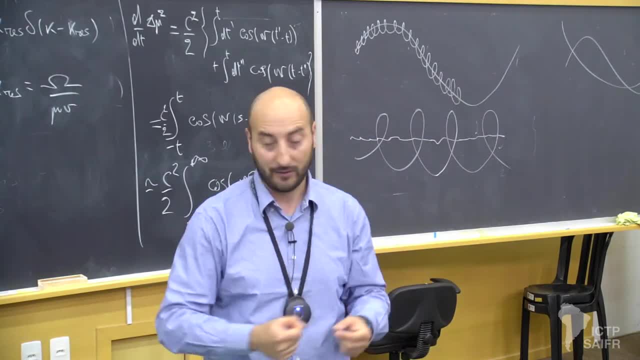 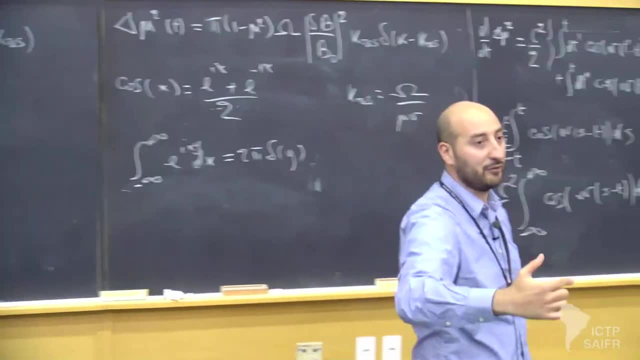 in isotropizing the cosmic rays. Okay, This is basically inferred from here. What I'm saying here is that there is a rapid- relatively rapid for astrophysical scales- change of direction. Okay, Now, this is a 1D approximation. 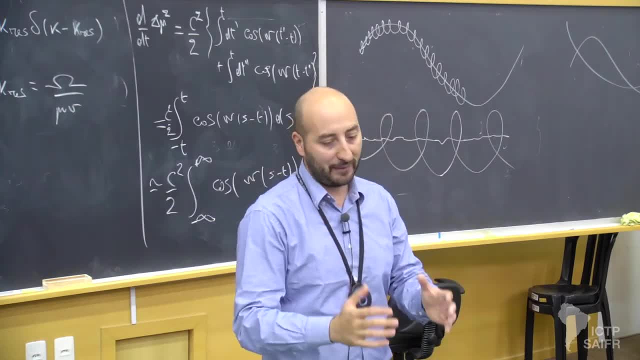 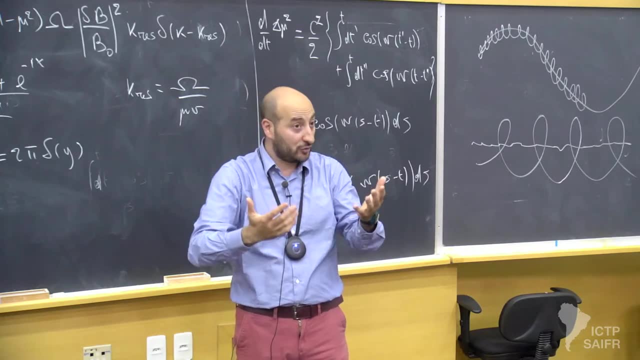 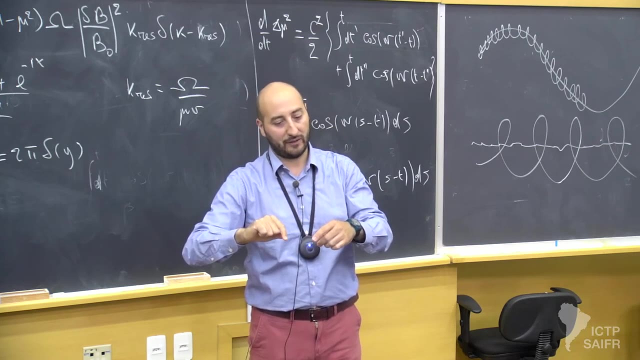 You should generalize this to 3D. So overall, what happens is that even if you start with a source which injects Ballistically a flow of particles away through, there is a current, But quite rapidly these cosmic rays won't move anymore. 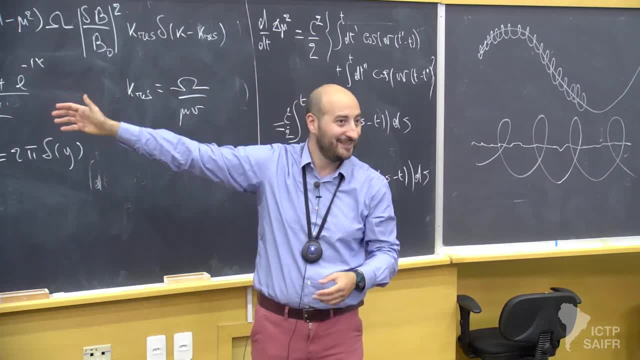 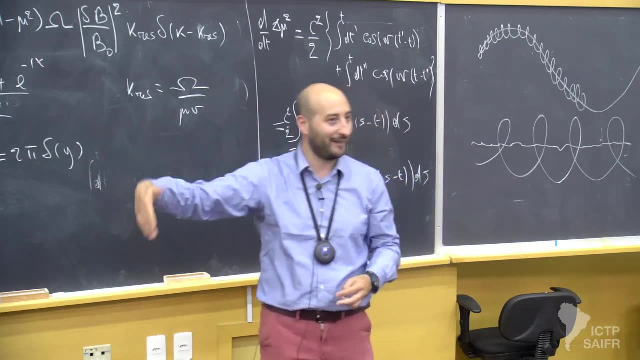 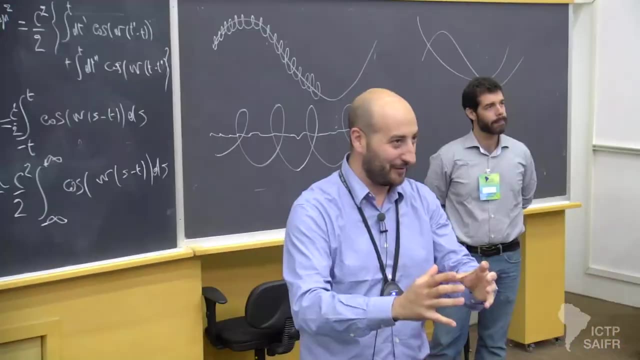 in a coherent way at velocity c, But they will basically reach a much lower velocity, which is of the order of the Alvin velocity. you will see in the following, And even there you're right: Microscopically there is a current 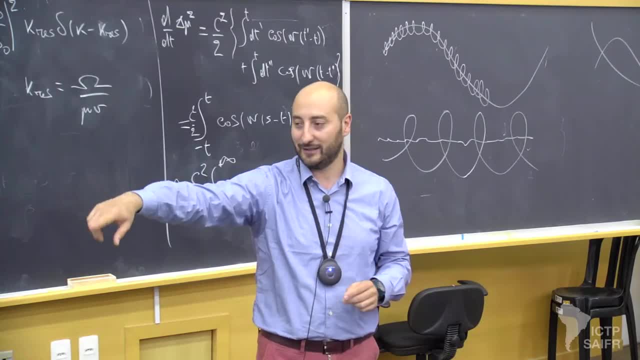 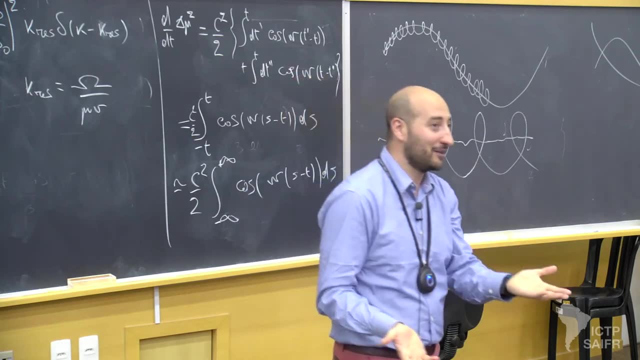 This current is instrumental in filling the loop that Pasquale was mentioning before, Namely, this current acts as a source, because a current in Maxwell's equation is a source right, A source term. This will act as a source of perturbations. 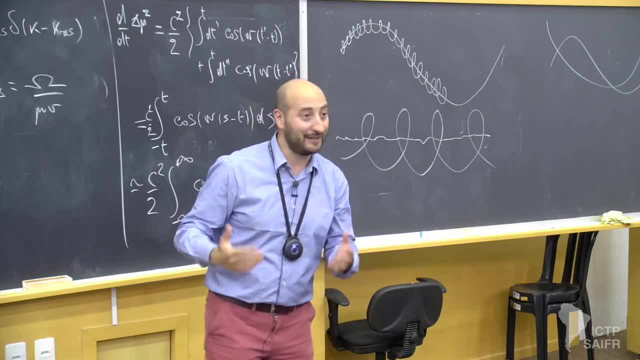 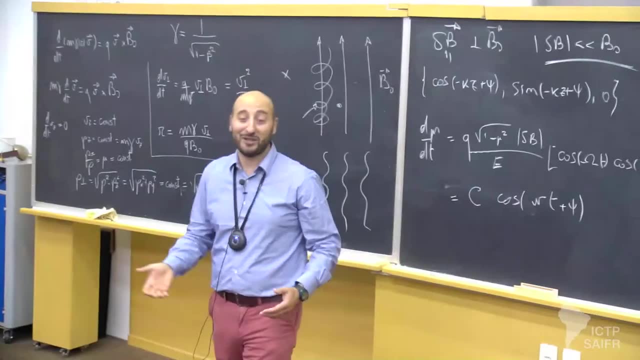 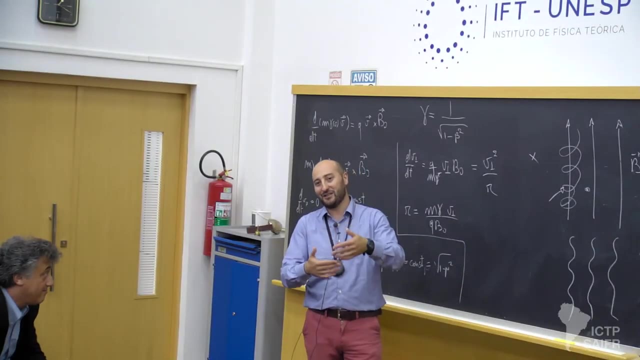 in the electromagnetic field. So in reality, I didn't tell you where these things come from, These wavelengths And actually, cosmic rays, they don't. They don't. The cosmic rays are among the sources of these wavelengths themselves. Now we start touching the idea. 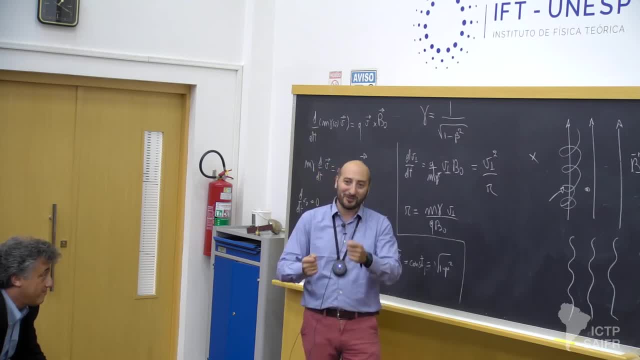 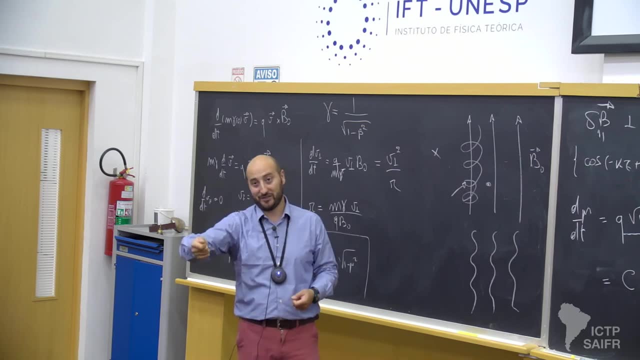 that the whole problem is nonlinear, It's coupled. So the cosmic rays, through currents, they can excite perturbations in the electromagnetic fields. These perturbations themselves act as a target for the cosmic rays diffusing, And this whole problem is usually not. 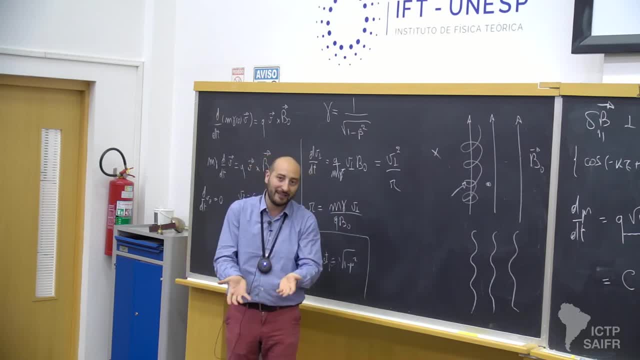 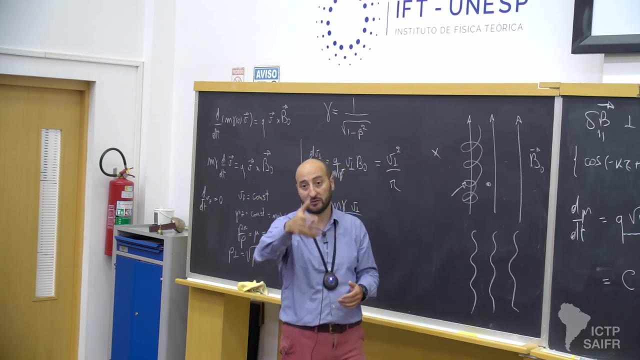 treated in numerical codes or et cetera. It's still actually subject of actual research. So trying to understand some features: how, for instance, can this be involved into particular shapes of the spectra of cosmic rays that we see at the Earth?